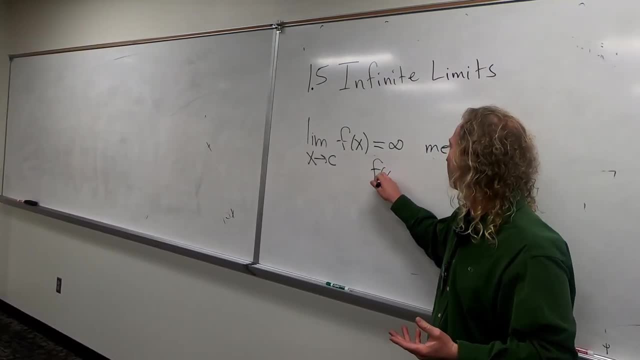 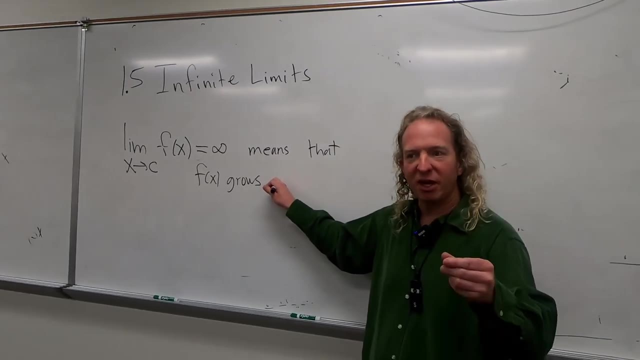 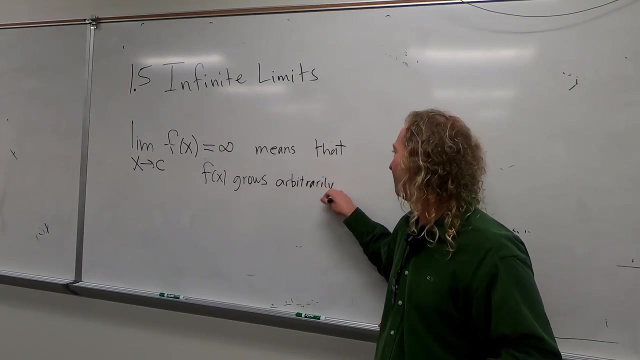 I'll say it a more precise way. It means that f of x grows, and the term we tend to use is arbitrarily large. That means it gets big. how big, As big as you want. So it grows arbitrarily large. Or you can say it grows without bound. You can also say it without bound. 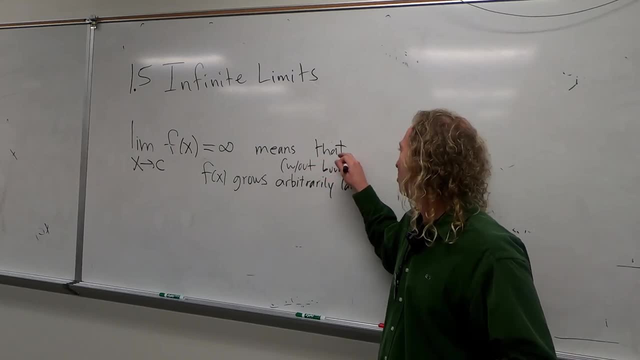 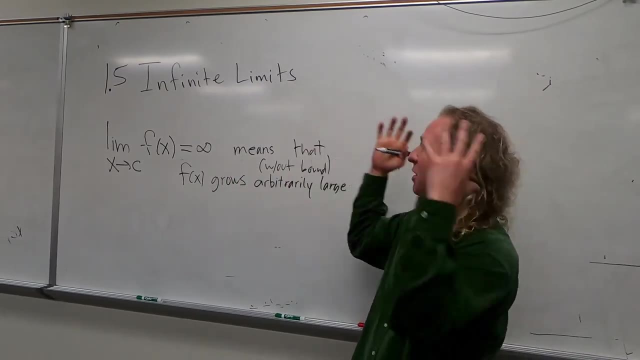 Or you can also say: it just gets big, So grows arbitrarily large, grows without bound. it gets big. In my mind I think big, big, Big is an easier word to say. in your mind Big, it's one syllable. 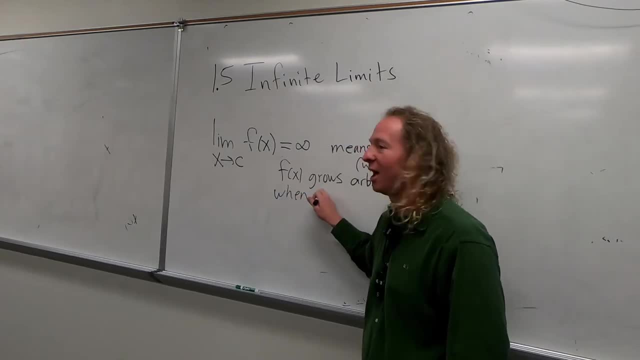 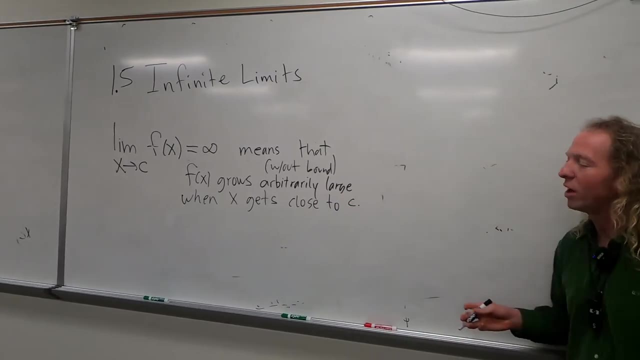 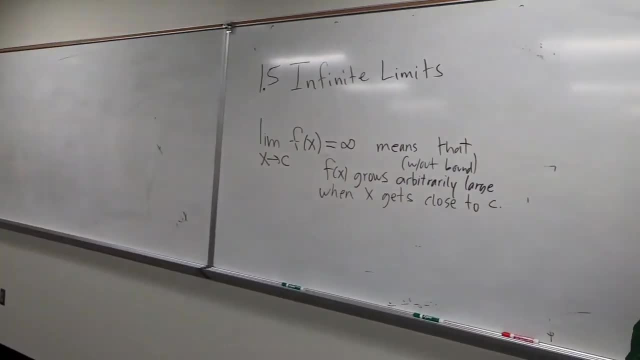 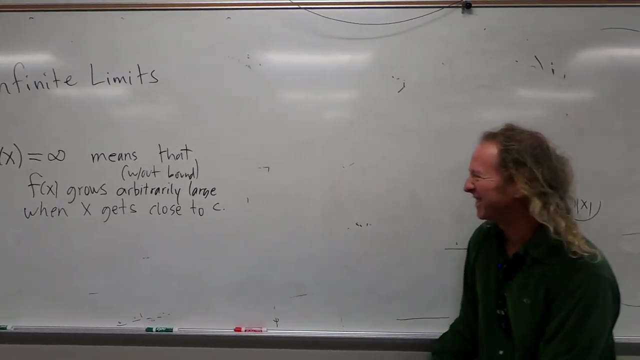 I'll say: don't show work, so you'll know. So you'll know. if it says no work is necessary, you'll know. it's these, You'll know. hey, we're people, it's filling in, It's so good. 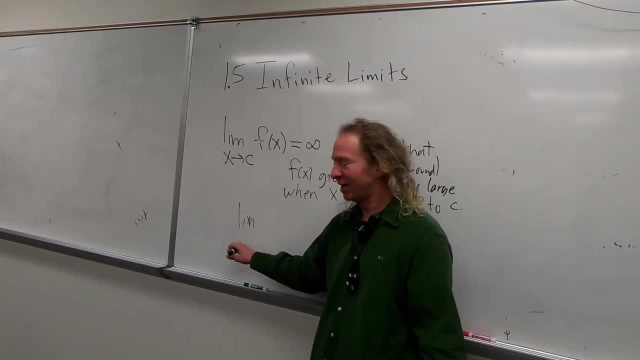 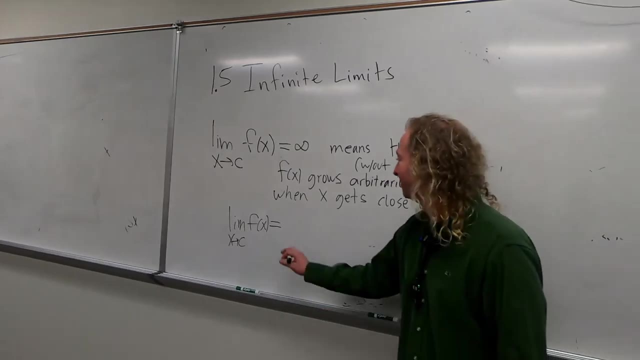 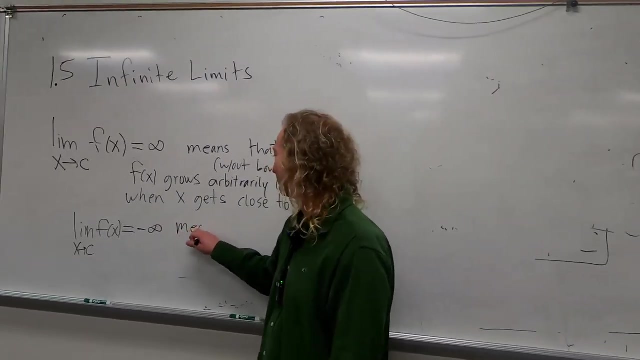 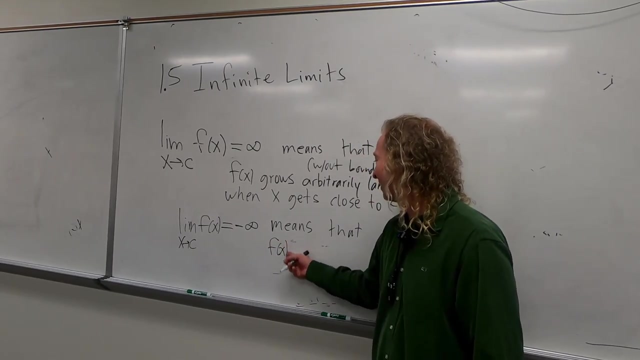 Hello, okay. and then the other one is limit: x approaches c, f of x equals negative infinity Equals negative infinity. This means that f of x, f of x- I put an s there- f of x gets small when x, so it grows, it decreases without bound. 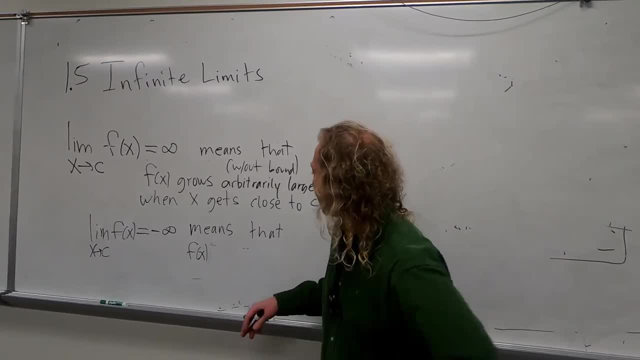 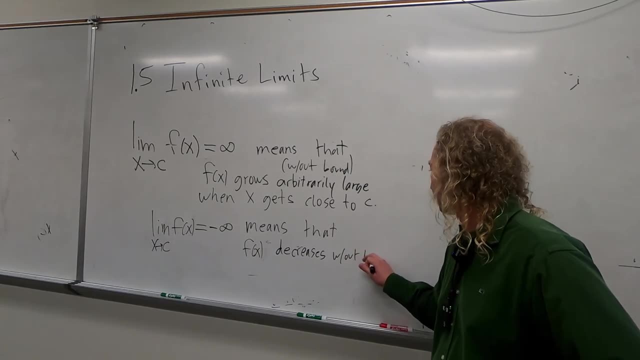 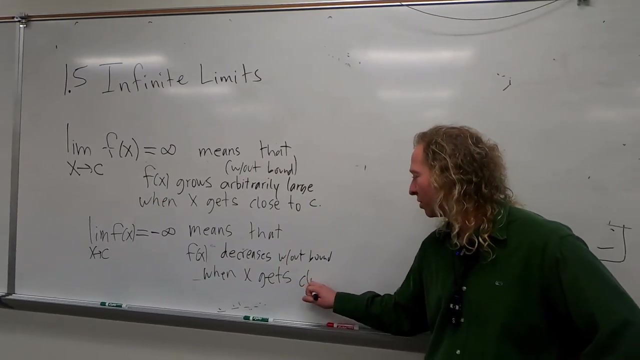 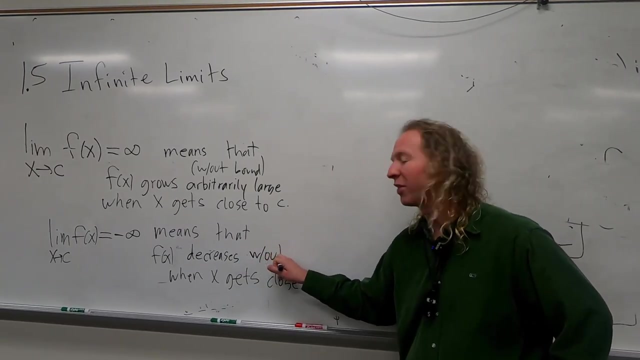 It gets arbitrarily small. So I'll just say f of x decreases without bound when x is close to c. when x gets close to c, gets close to c. So it decreases without bound, without- I'll improve my handwriting- without bound, without bound. 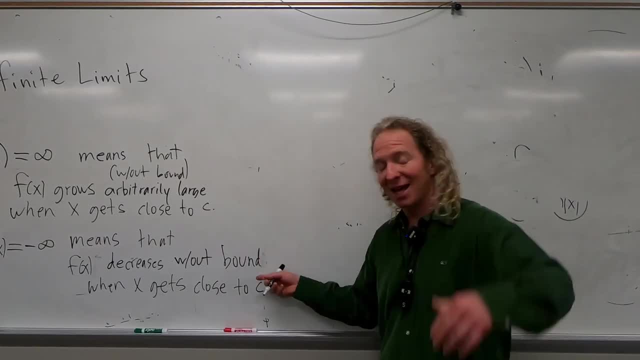 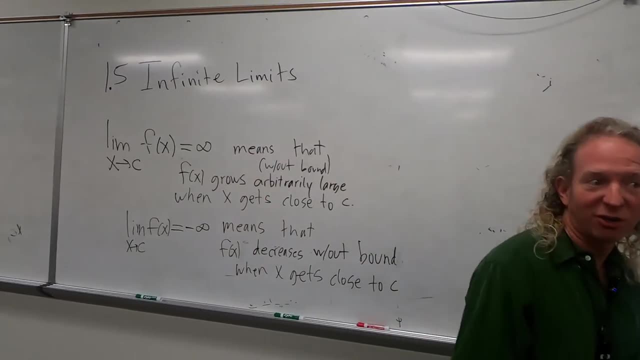 Or you can say it gets small. I just think of it. as it gets small, it goes down forever. So basically, this means the y value goes up forever. this means it goes down forever. That's it. that's the whole section in theory, almost. 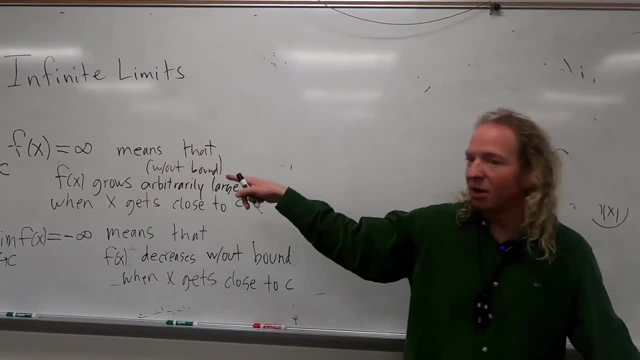 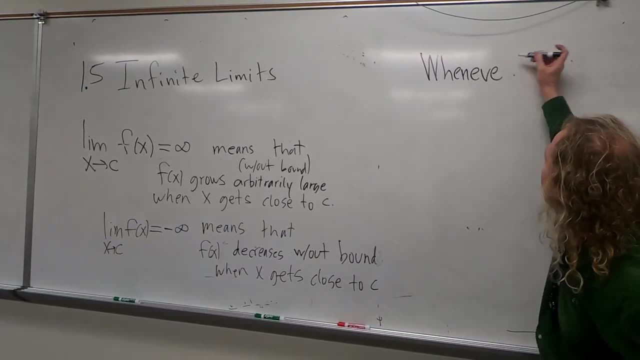 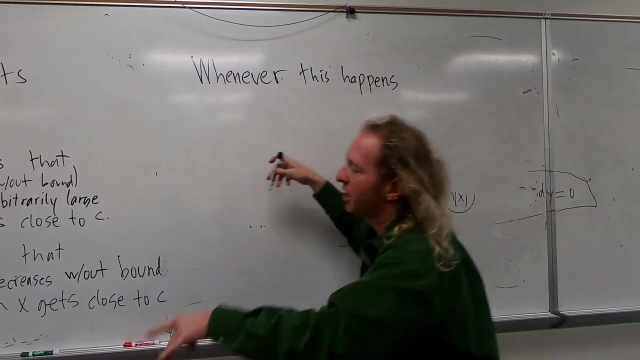 So whenever this happens, whenever this happens, we have a vertical asymptote at x equals c. So whenever this happens, including the one-sided case- So let's say you approach c from the left, That still gives us a vertical asymptote. 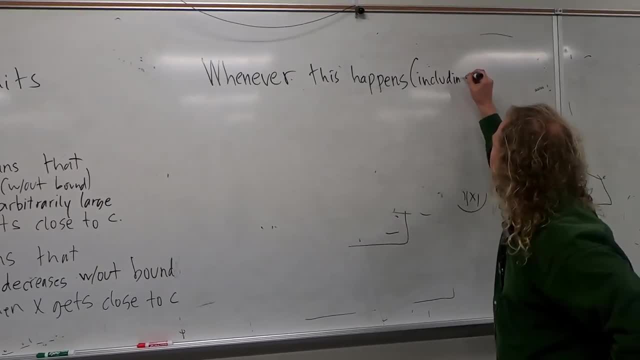 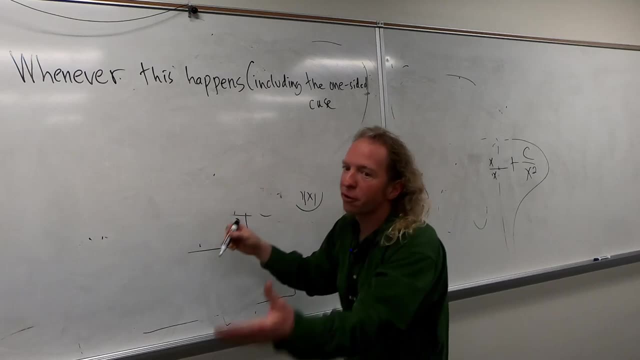 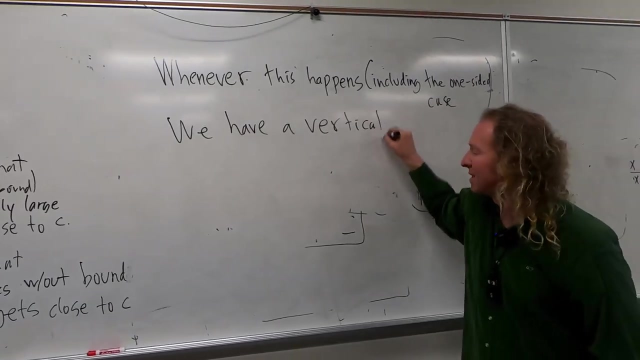 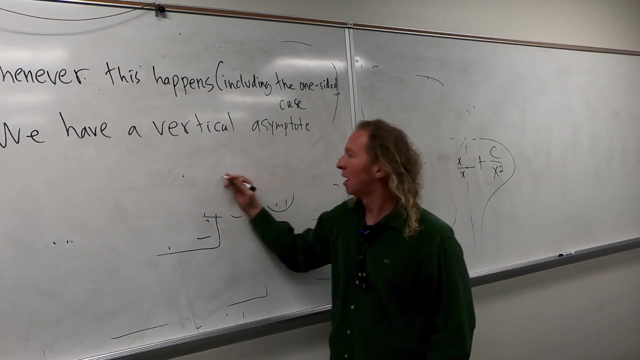 including the one-sided case, The one-sided case. We have a vertical asymptote. We have a vertical, a vertical, a vertical asymptote. We have a vertical asymptote, asymptote, asymptote, Big word: A-S-I-M-P tote at x equals c. 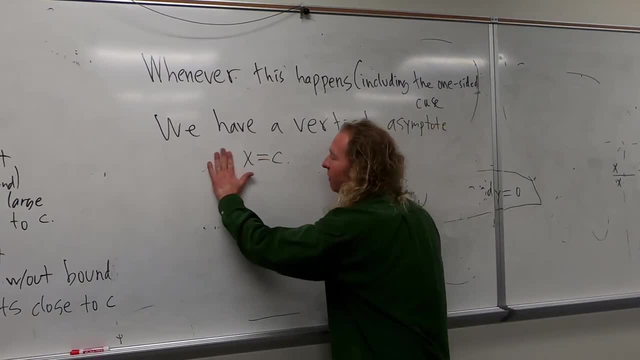 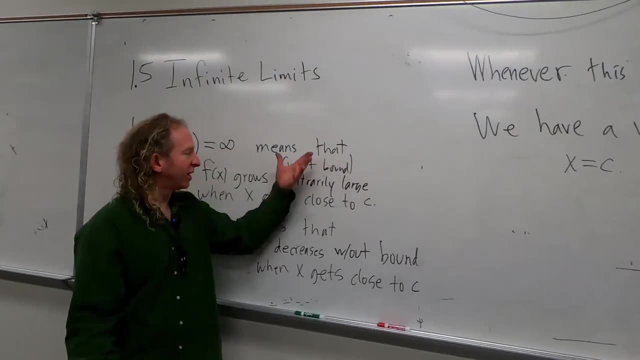 So x equals c, rather is the vertical asymptote. Let me just say vertical asymptote, x equals c, because it's not at x equals c, it's a line, right, It's a vertical line. So whenever you get infinity, you're going to have a V-A right. 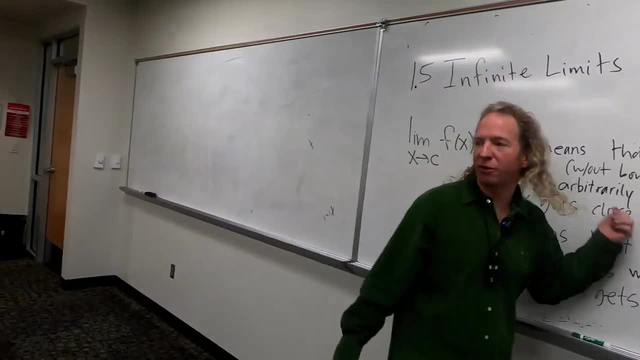 You're going to have a vertical asymptote. okay, You're not going to be using this to find vertical asymptote. It's too much work. Most of the time, you'll just look at it and you'll know. I think it would be. 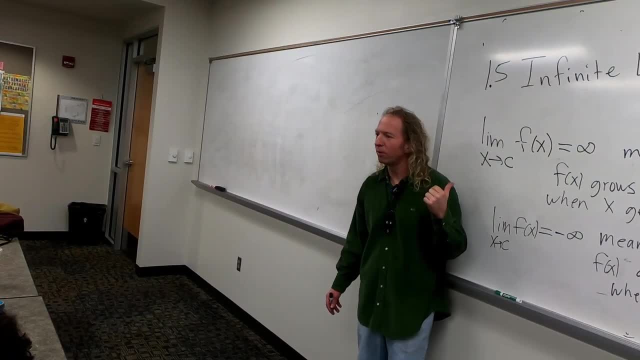 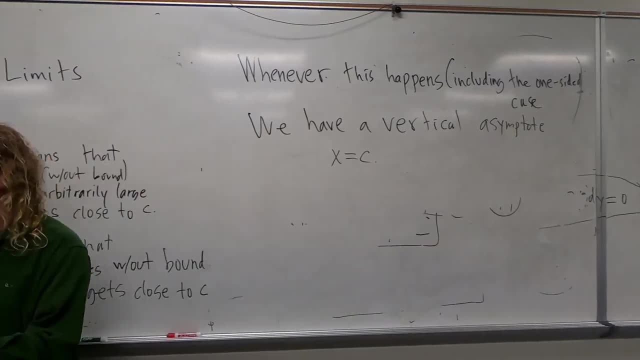 I think we were doing it before, weren't we? With the removable and non-removable. Do you remember? were vertical asymptotes removable or were they non-removable? Non-removable, Yeah, but what about holes? Removable? 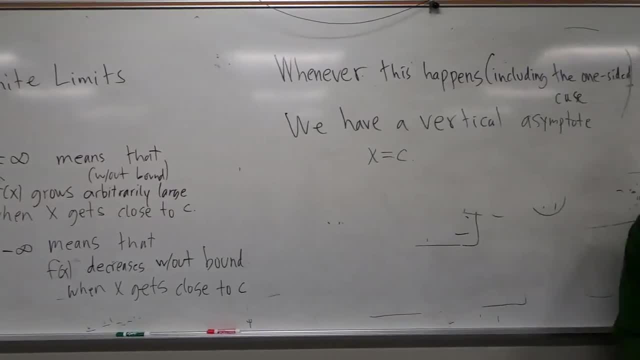 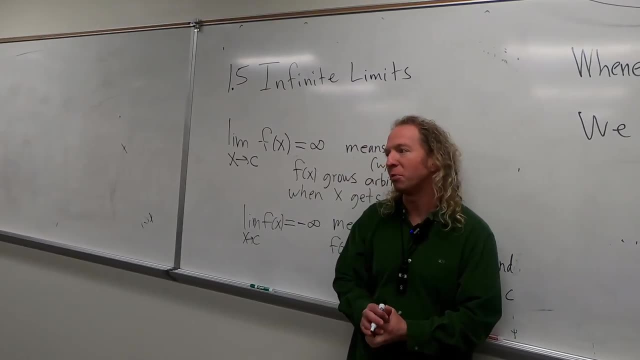 There you go. You got five points on the test, right. That will definitely be on there no matter what. So typically when you're studying too, like if you just go over the examples from class, you will be set like for the most part, right. 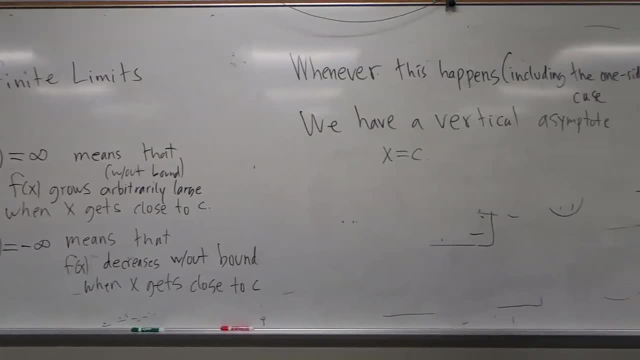 It's stuff from class. We did a lot of hard ones too, So not all of the hard ones will be on there. I mean, we did a lot of stuff. Last time was insane. We did, I just felt insane. 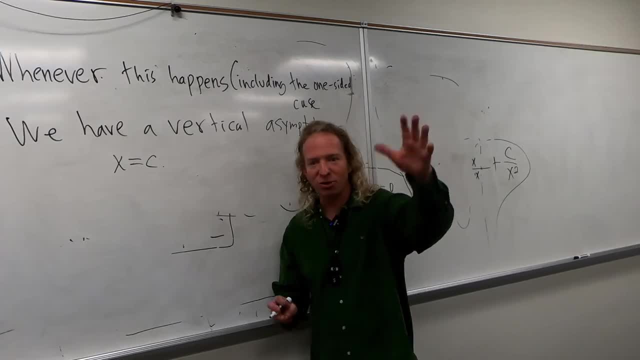 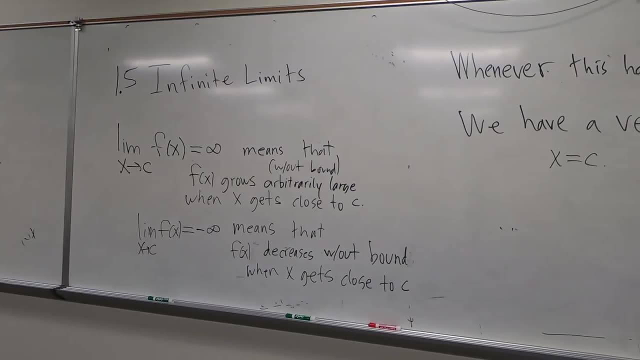 We did so much math. There was no break, was there? It was like: I'm sorry, Today will be much shorter, Like don't worry. So like oh, Okay, let's do an example of a test question. 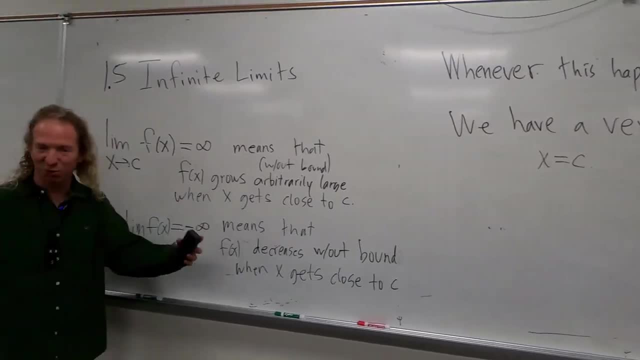 Let's just start right away with like something that you'll see on your, because your test is next week. I feel like, oh my God, It's like we just started right. It's like why is there a test? 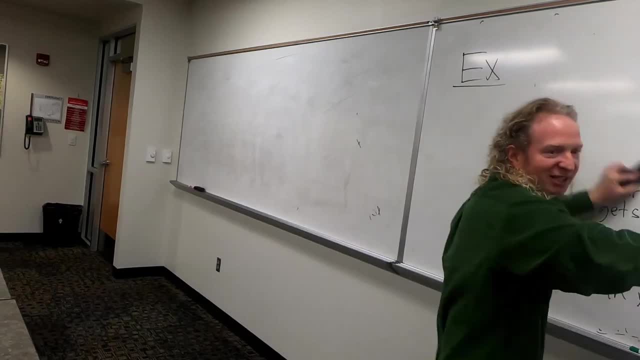 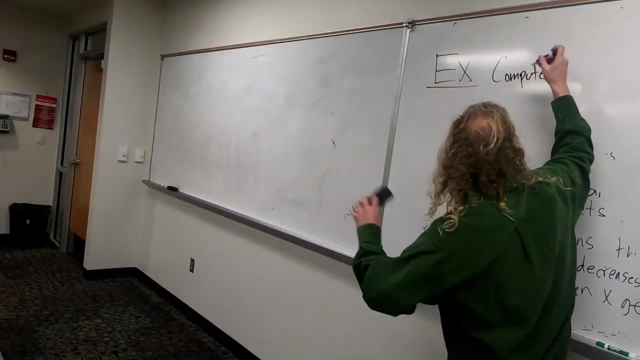 So on your test you'll have a question like this. It'll be like: six or seven parts, okay, Lots of points, Yeah, and it'll say: compute Now if possible. it'll also say: you know? 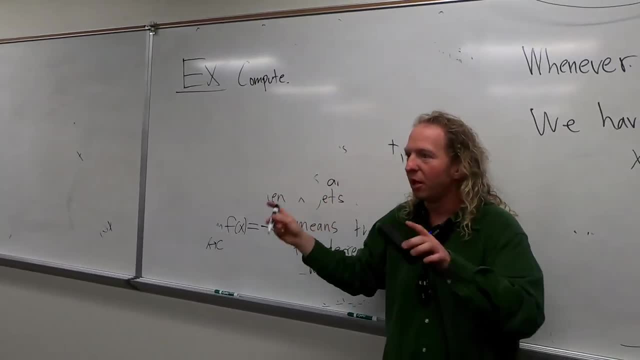 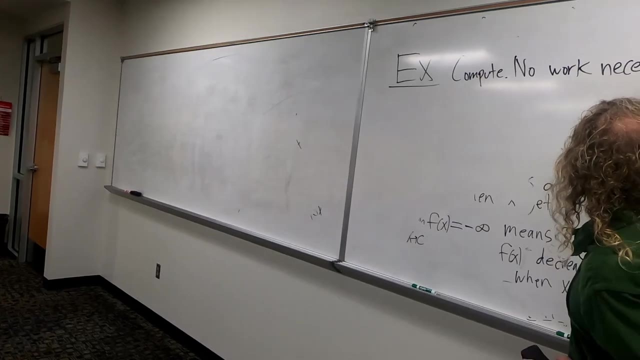 use infinity, negative infinity and D and E when appropriate. It'll also say no work necessary. I specifically will say this: Okay, so because I'm not going to grade your work. Why? Because there's no nice way to show the work. 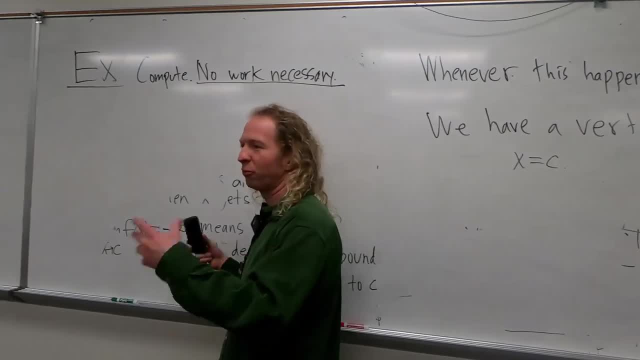 The work is actually incorrect, right? The only way to compute these limits is like to prove them using, like the definition, which we're not going to do, So we're just going to do whatever to get the answer, So A. 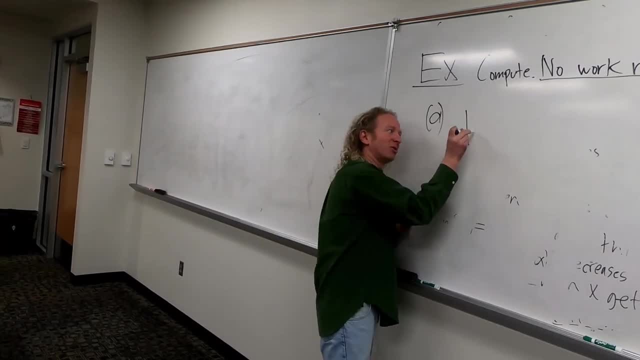 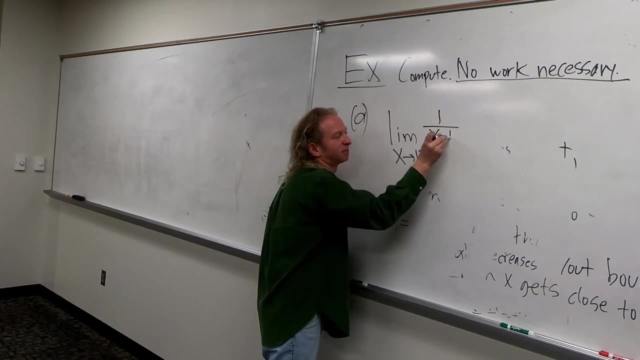 It's kind of fun. So just keep in mind it's wrong. So limit, as X approaches 1 from the left of 1 over X minus 1.. I don't know what the answer is. I haven't thought about it. 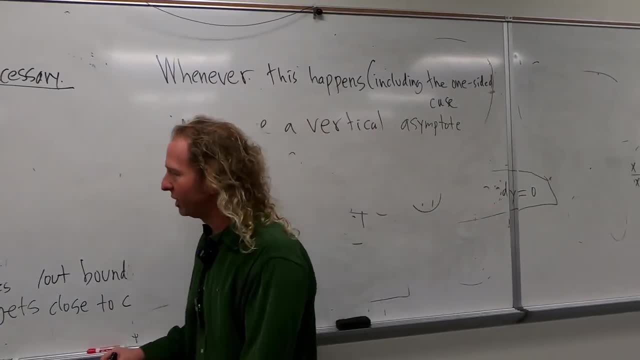 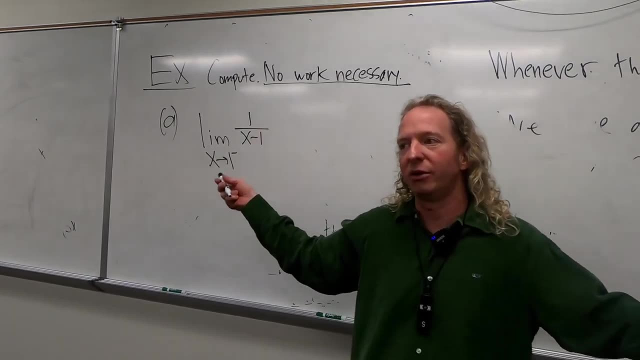 But you could put it in your calculator and graph it and try to get the answer. If you plug in 1, it fails right, Because you get 1 over 0, right, You get 1 over 0. So it doesn't work. 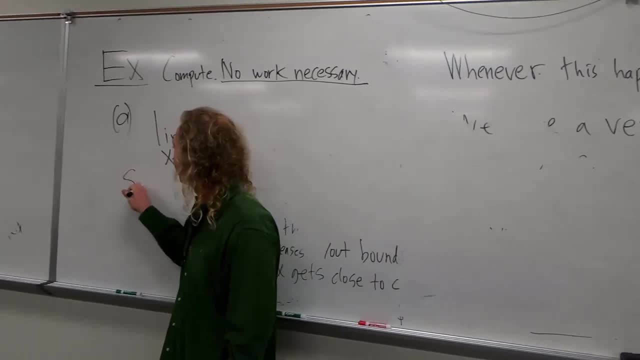 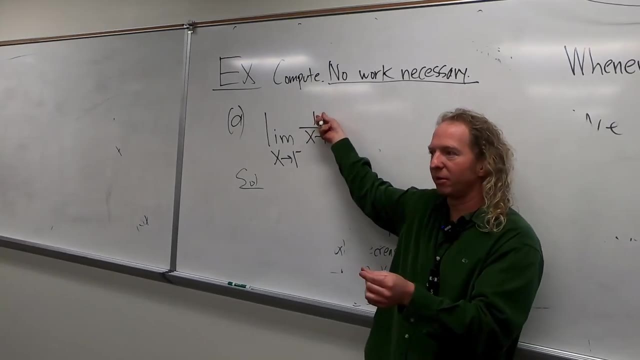 So how do you do it? Okay, Let's see So solution. So you have to think about it. So I think about it as a fraction. So, no matter what, up top 1 is a positive number, right? So you have a positive number. 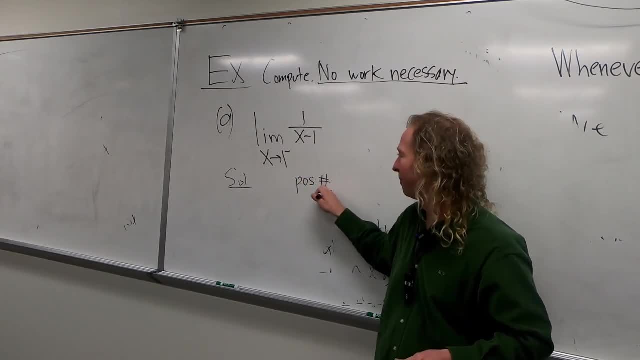 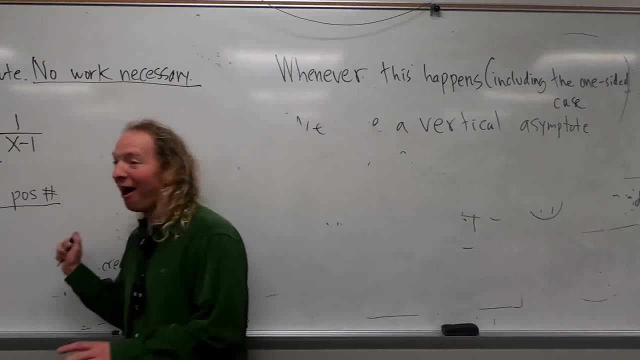 So you have a positive number, I'll put POS number- POS means positive Positive number- On the bottom. you have to figure out what's going on. So I like to draw a little picture. So I'll come over here and draw a little picture. 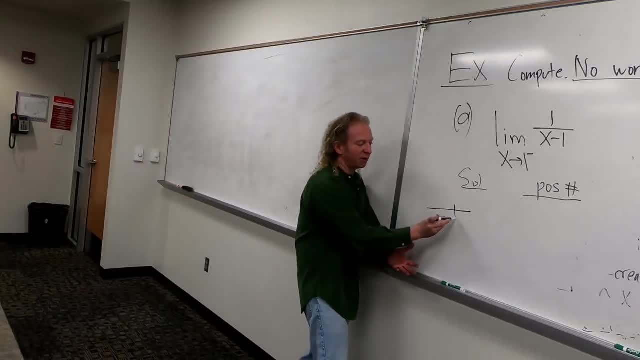 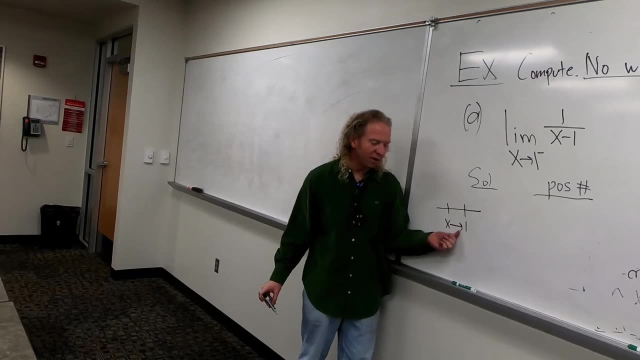 So here's the line, the X axis. Here's 1.. We're approaching from the left right, So we're going this way. So I just like to plug in a number that's really close to 1, but smaller, So like .99, right. 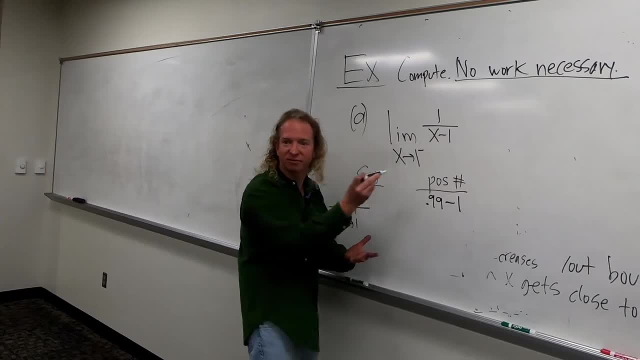 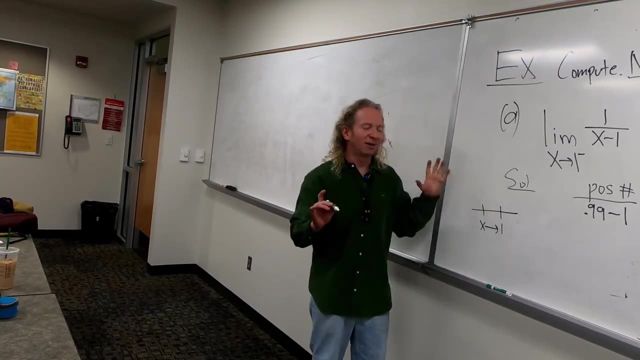 So like .99 minus 1, right? So we're just writing down our thoughts, right? You can do it in your head if you're feeling like a rock star, But I know, yeah, I don't like doing stuff in my head. 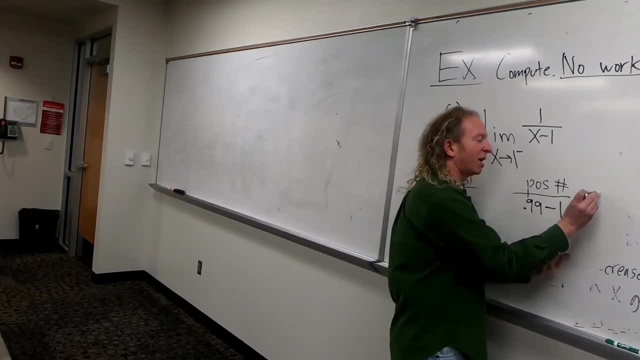 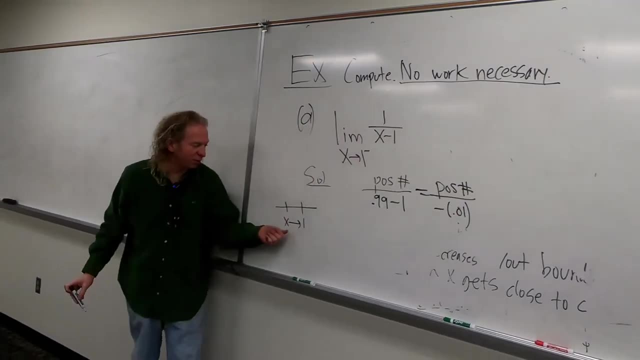 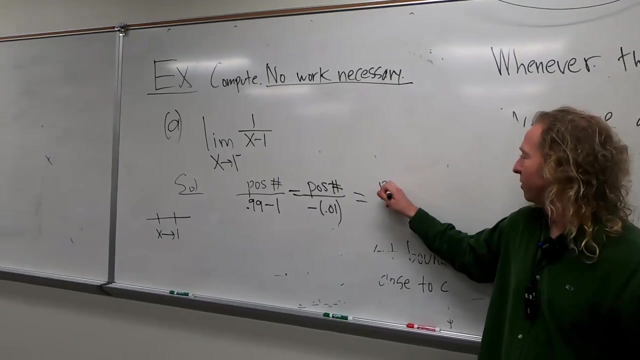 Not too much, So positive number in that. So then this is positive, Positive number over negative, and then it's .01, right? So I just made up a number. You could use any number: .9999.. So basically, you have what you have, is you have a positive number. 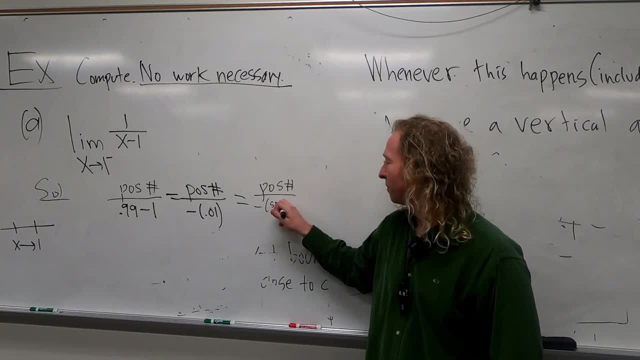 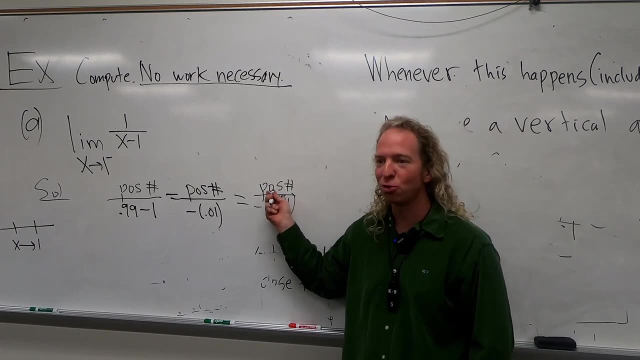 Then here you have a negative and then you have a small number. So a super small number That says super. You can't see, I don't know if you can see, It says super small, super small number, It's a super small number. 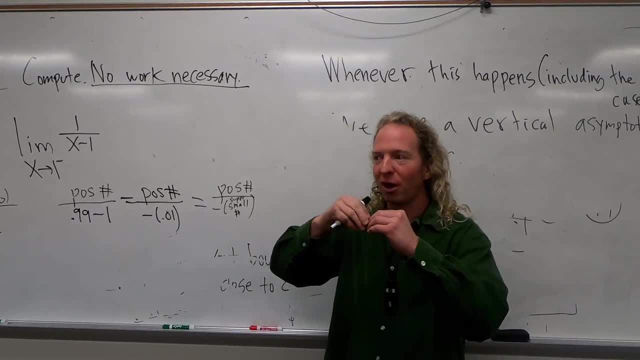 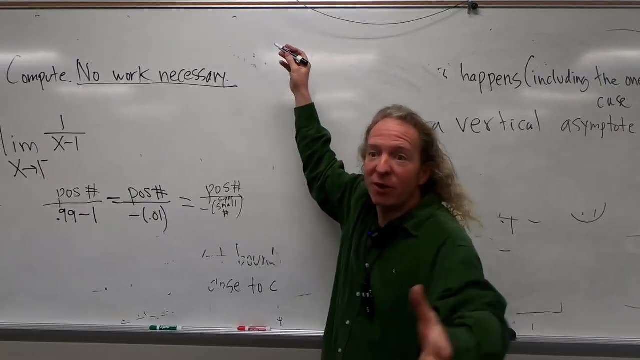 So if you have a number Over something super small, I don't even know what happens to it, What happens to that fraction, It gets what Really big Yeah. So if you don't know that, think about this. If you have like, if you have like 10. 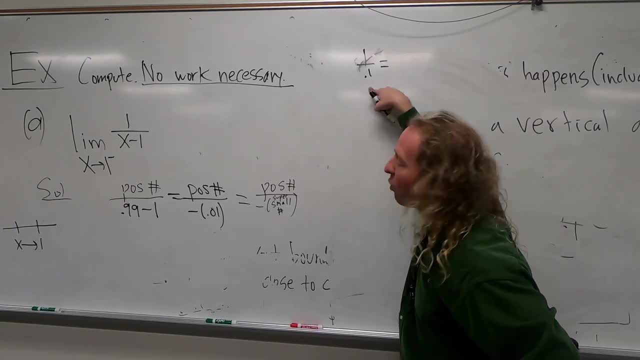 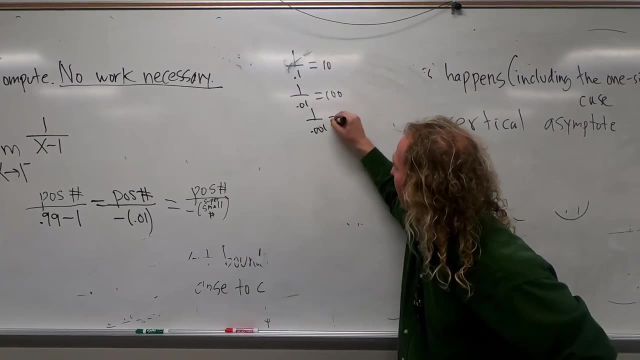 If you have 1 over .1, that's actually 1 over 110.. That's 10.. If you have 1 over .01, that's 100.. If you have 1 over .001, that's 1,000.. 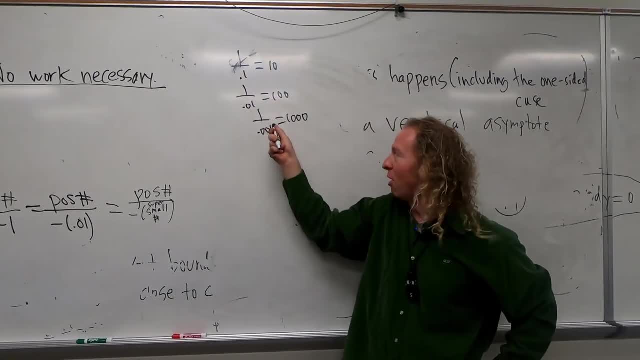 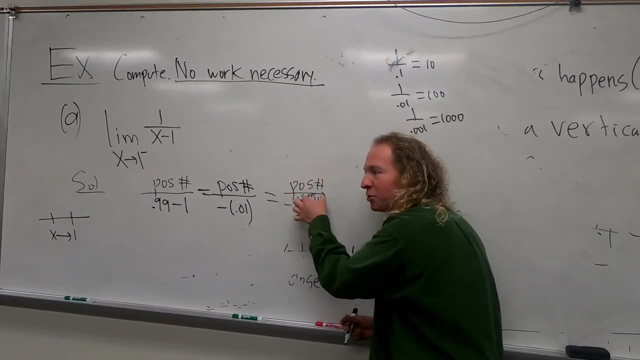 I'm going to stop there because it gets too confusing. But when the bottom gets small, the thing gets big. So small on the bottom, big fraction. So this: you have a positive number over something small. So this is big and it's negative. 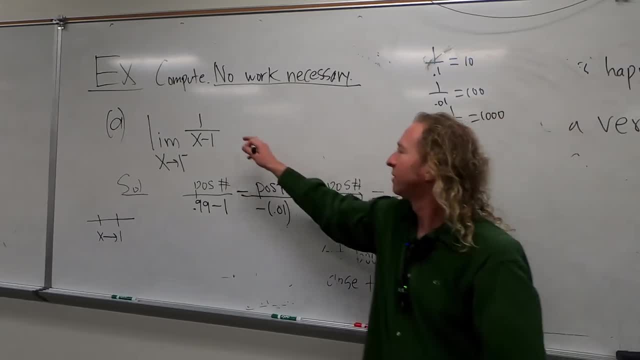 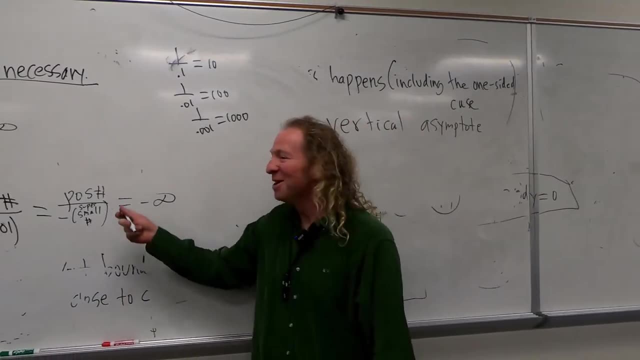 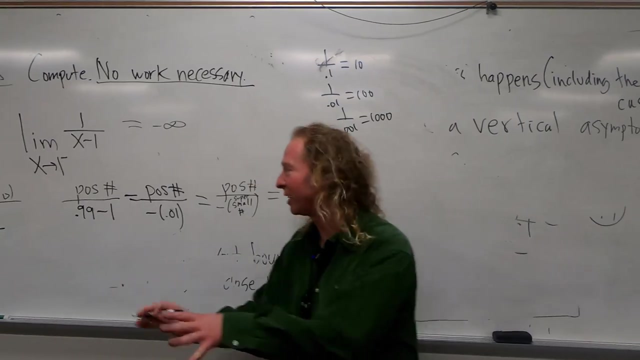 It's big and it's negative, So it's going to be negative infinity. Hey, what's up? Bring it in. So does that make sense? No, A little bit. No, No, I'll go over it again. So the top is a positive number, right. 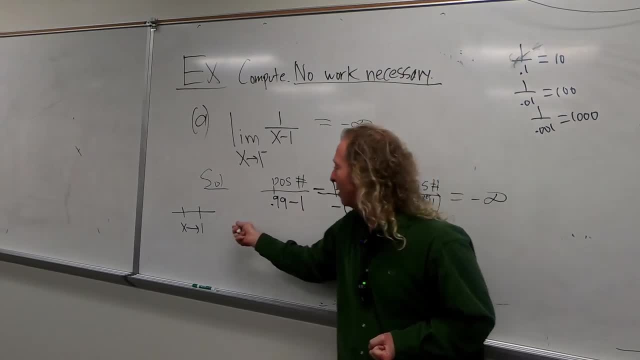 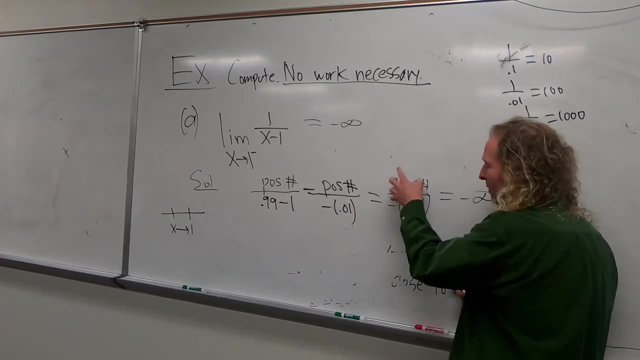 And then you just take the bottom, You just take any number you want that's smaller than 1.. Because it's approaching from the left, So like .99.. So .99 minus 1 is negative .01.. So you have a positive number over something super small. 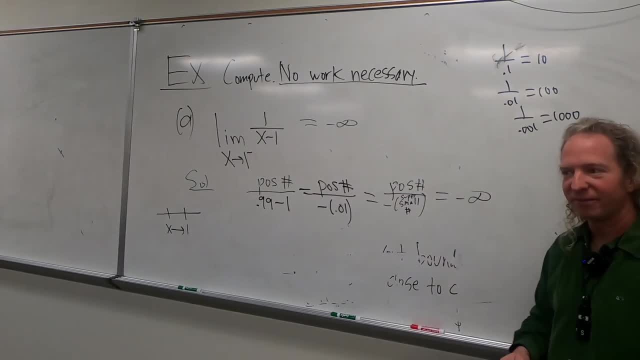 So that's big. Then you have a negative, so it makes it negative infinity. That's it. Let's do another one. We're just going to keep doing these until you got it. Let's just do more. Let's just do more. 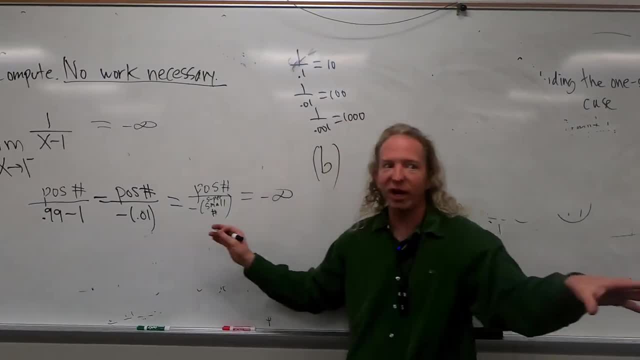 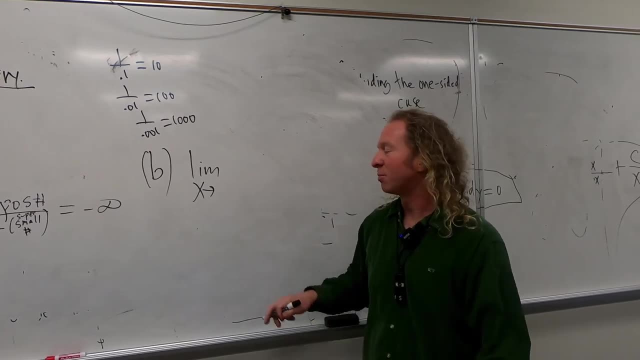 B, B, B. And again, the work doesn't matter. Like you could do whatever, right You can draw a picture of a horse, It doesn't matter. I don't know why I said that. Let's approach. Let's approach 2.. 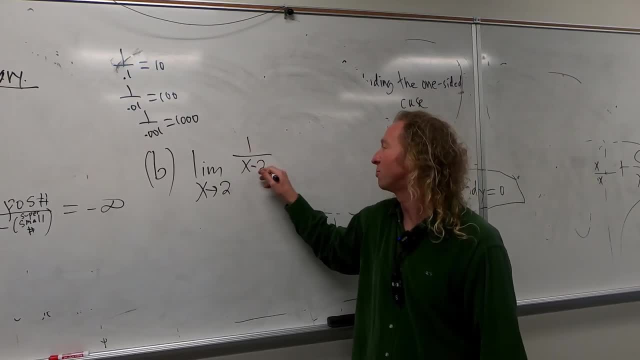 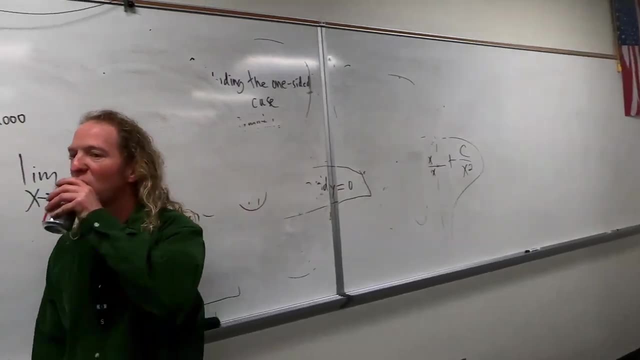 Let's keep it simple: 1 over x minus 2.. And let's approach from the right. The homework is kind of weak, It's all right. I mean this is a little bit harder. Like these are better examples: Infinity. 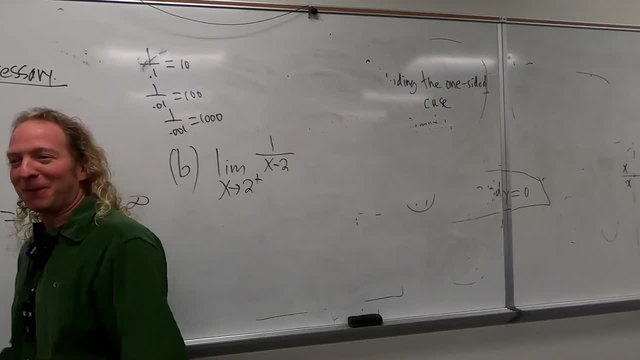 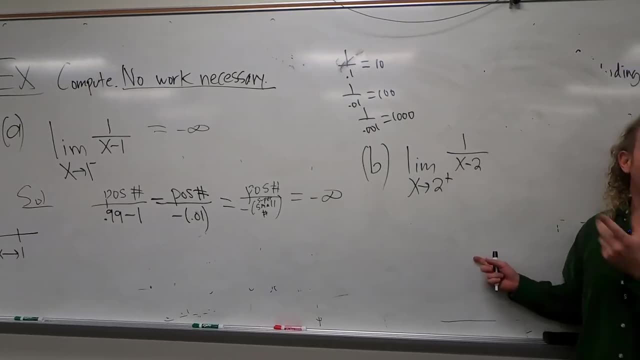 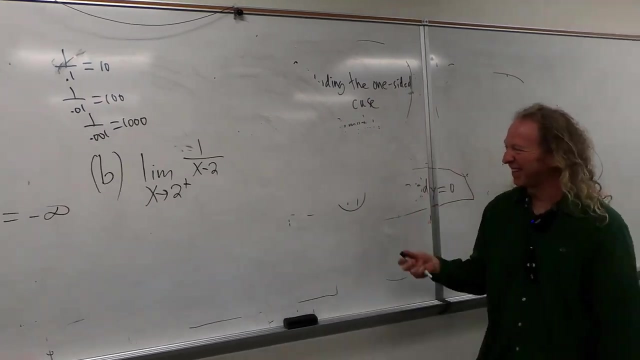 Very good. So John is saying so. if it's approaching from the right, it's positive infinity. Yeah, in these cases, but if I do this game over, Yeah, No, no, Yeah. Good John Thinking, Good work. 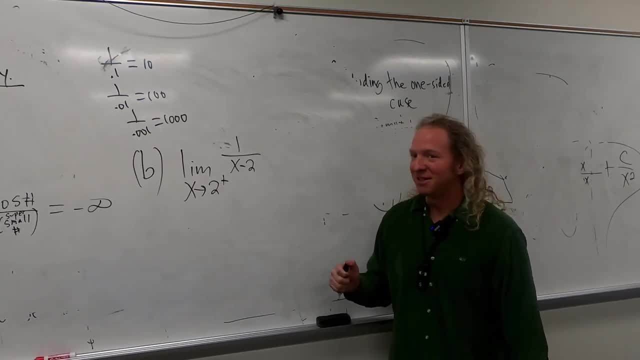 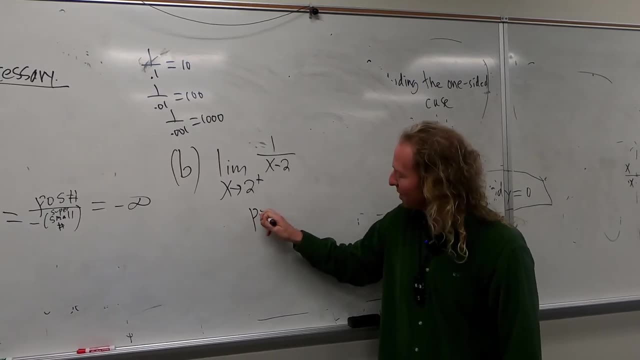 Dennis, No, No, no, Don't tell me, I'll figure it out. So let's work it out. So positive number- I should know Positive number And we're approaching 2.. So here's 2.. And we're approaching from the right. 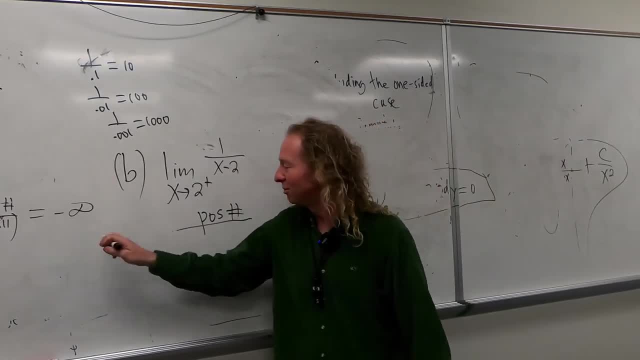 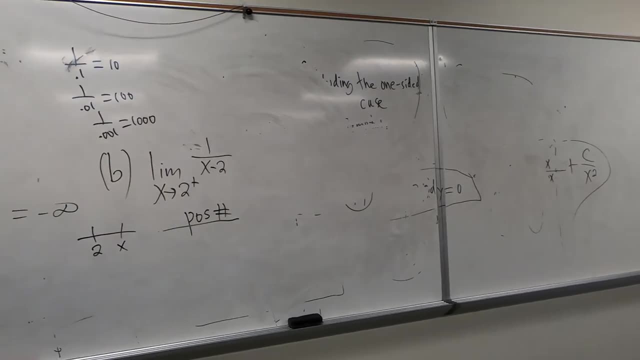 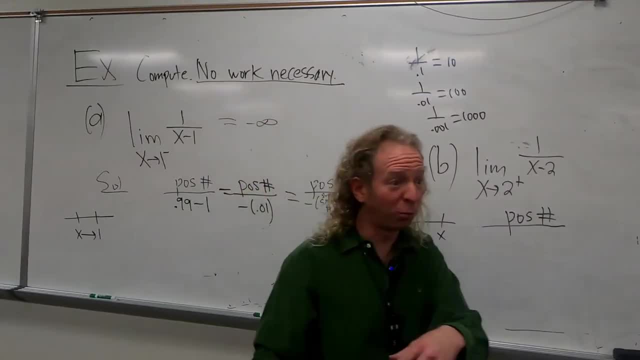 3. Well, it's really close: 2.1.. Or 2.1 or 2.01.. I'm really close, Yeah, So 2.01.. You can do 2.1, too, But I'll do 2.01 minus 2.. 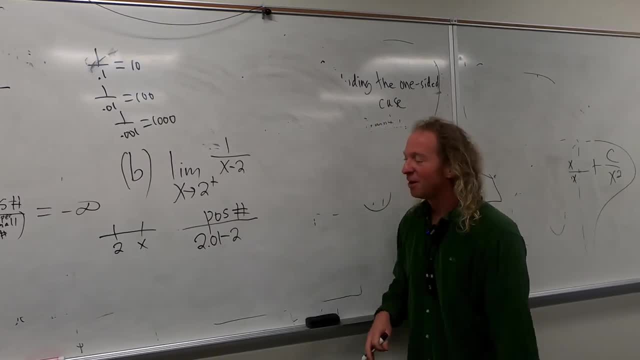 You'd have to do 2.0001, but it doesn't matter. So this is a positive number And this is .01.. This is .01.. .01.. So you have a positive number over something small. That means it's big. 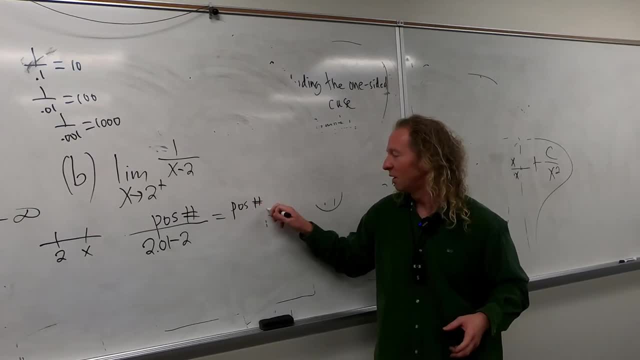 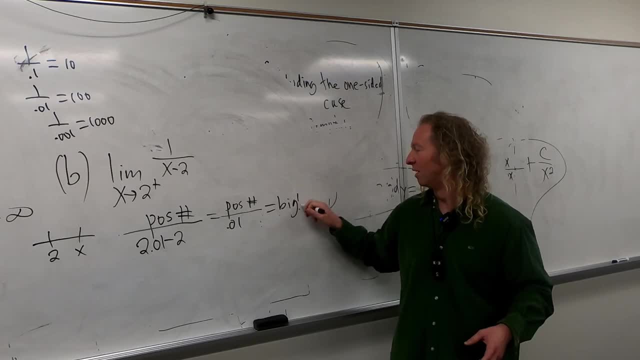 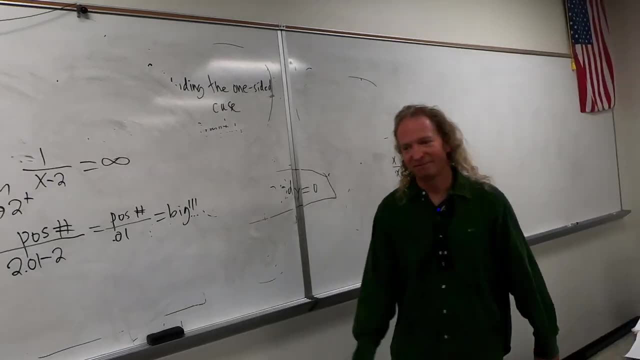 2.01. 2.01. 2.01. 2.01. 2.01. 2.01. Right, Right, So it's infinity. That's it, That's it. 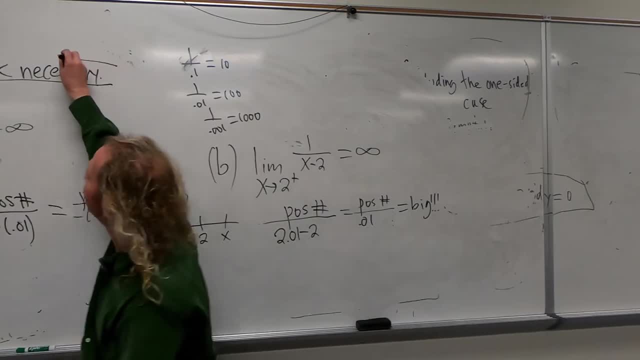 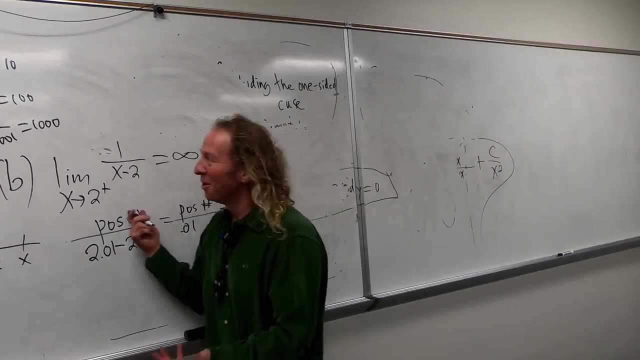 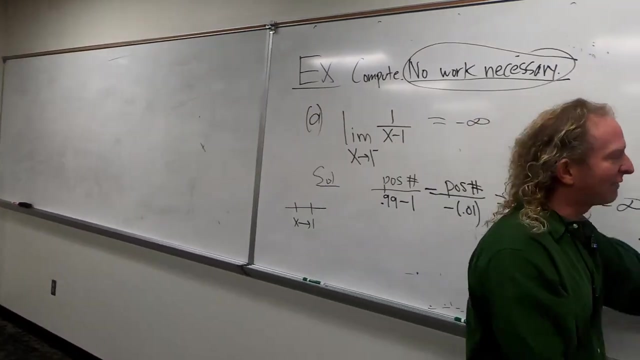 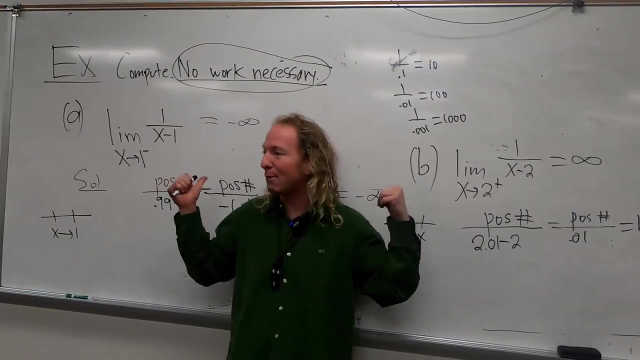 So I can't mark it wrong on this one And that will help you on the test because you'll know it's this type of problem when it says that's huge. 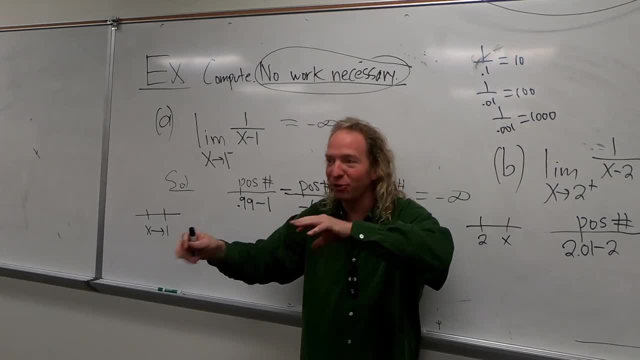 If it says solve analytically, those are the ones where you have to factor. Don't put D and E on those. No, that's bad. You want an answer on those? All right, let's keep going. Let's do more. 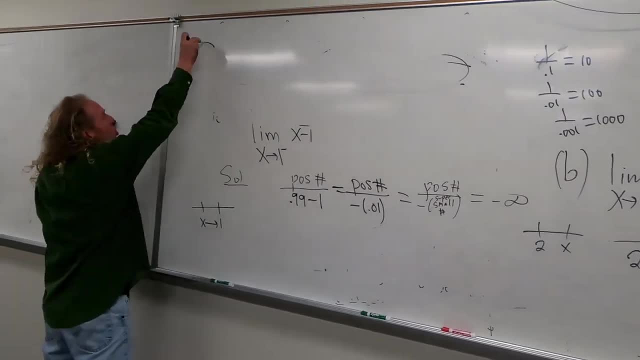 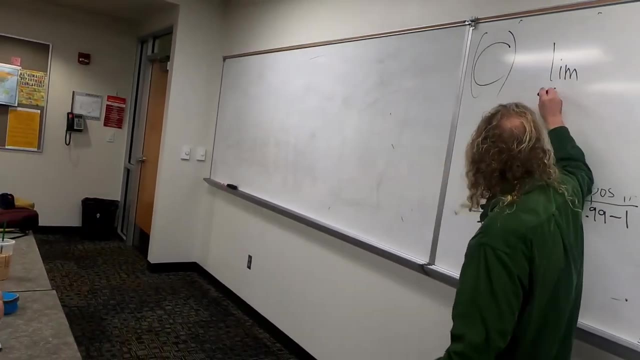 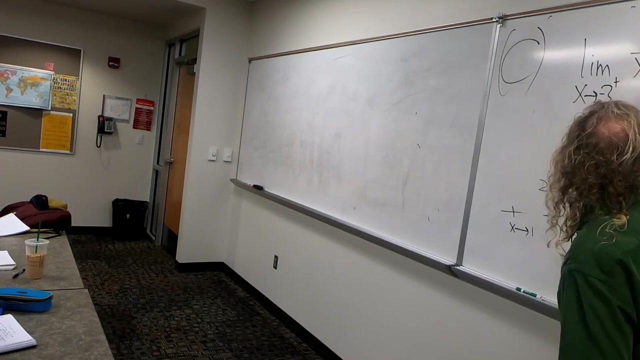 I like these. I haven't done these in a long time. I don't know C. Here we go. Oh, I know I know Limit Ethan Like the furniture. Sorry, Let's keep it simple for now. Do you all want to try this one, or should I do it? 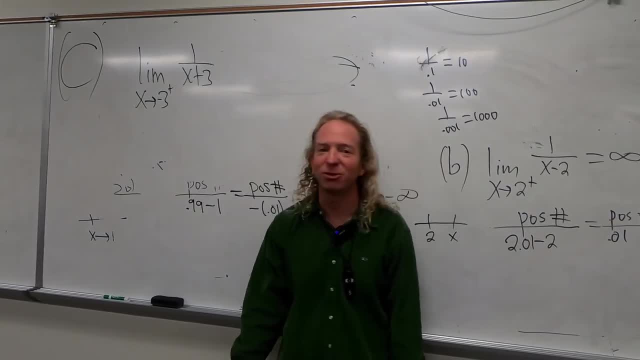 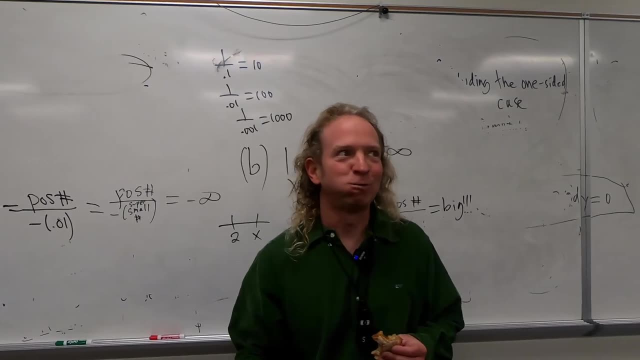 You want to try it? Okay, All right, try it, Try it. Take your time, Try it. I'm going to try it. So many people here, It's like perfect attendance. Nick Jason, Is that the chair? 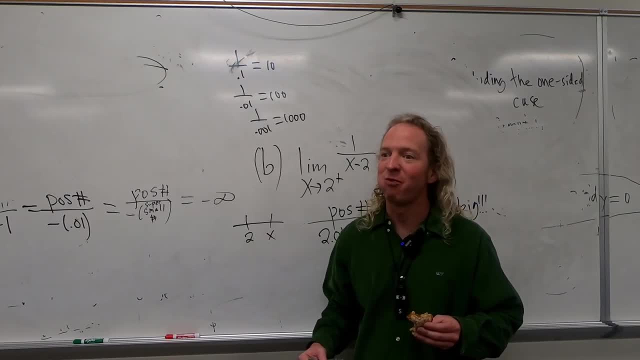 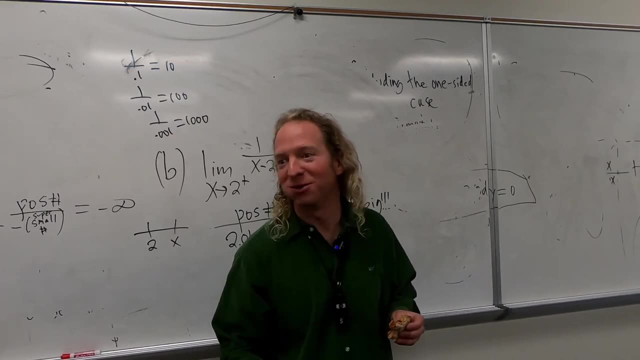 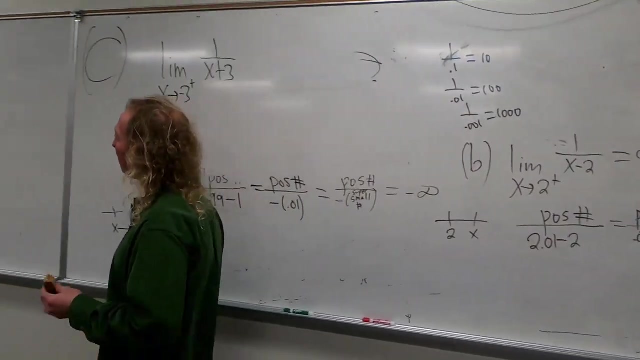 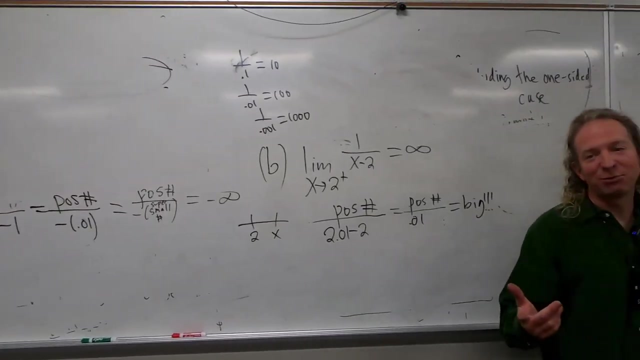 Jeff. No, it's not Jeff, It's not Jared, It's not Jason. John Jono Jordan- I guess I picked Jordan to be tall Like Michael Jordan. I had a guy named Jordan in my class last night. 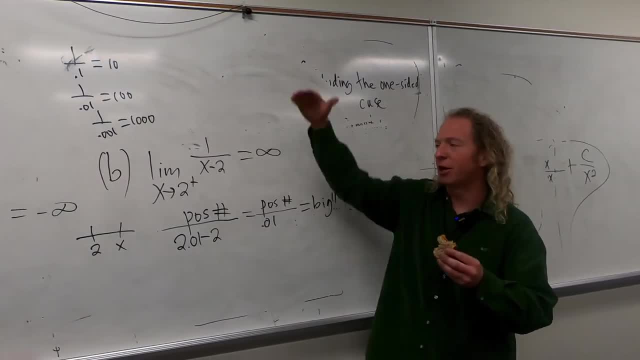 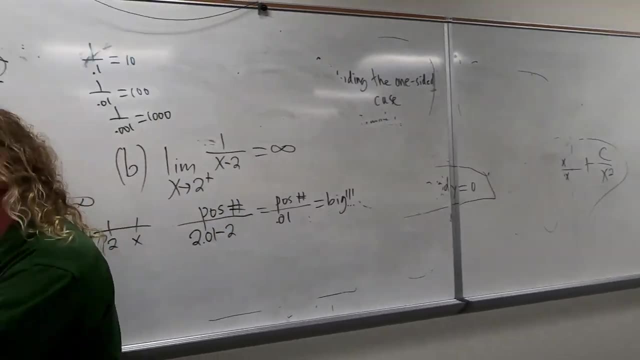 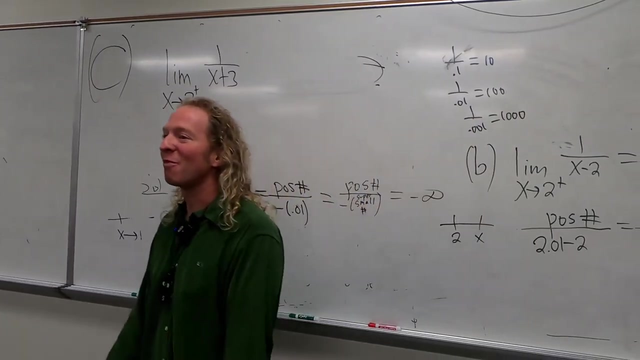 He was really big. He was like tall Giant, Giant. You got it. I haven't even thought about it yet. Hey, all right, Welcome back Anyone. what answer did you all get? Infinity, Okay, let's try it. 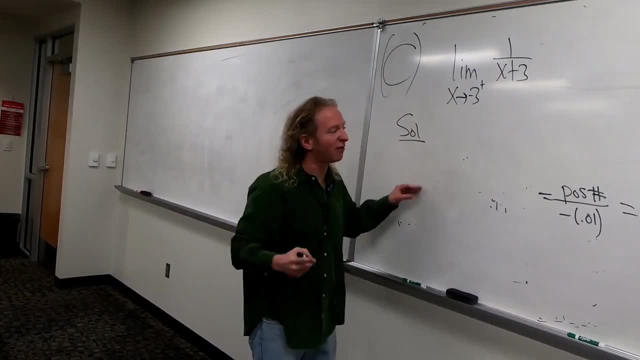 Let's try it, Let's see So. solution: Some people have a really hard time with this. I've had students in the past- really good students. They get A's. They take Calc 1,, Calc 2, Calc 3, DE. 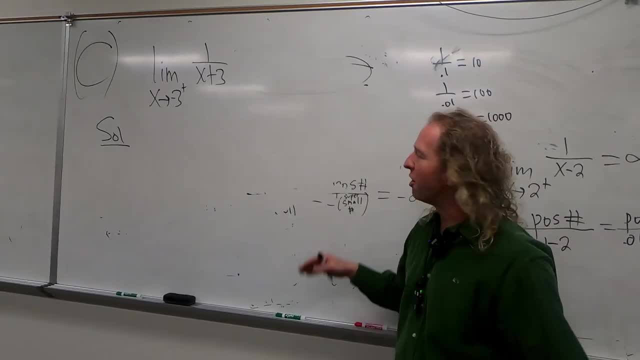 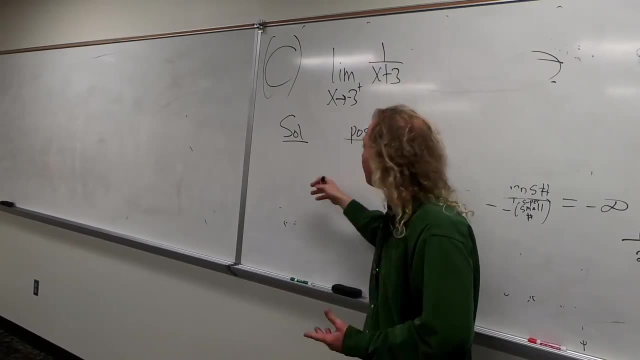 They get A's in all the classes. But this, Like I never understood this. It's just certain types of math are harder sometimes. So it's a positive number up top, because it's 1, right And then. so here's negative 3.. 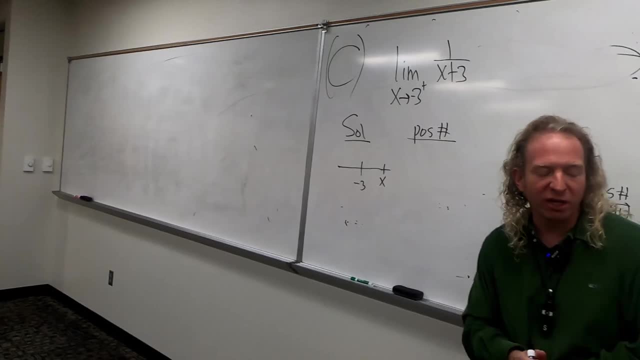 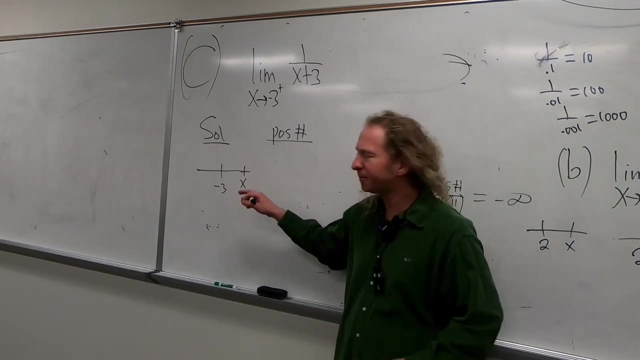 We're approaching from the right, So let's see Bigger than negative 3.. So negative 2.9.. Yeah, so negative 2.9, right, That'll work. So negative 2.9 plus 3.. 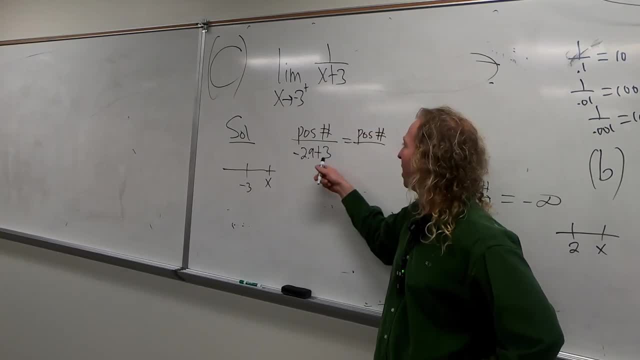 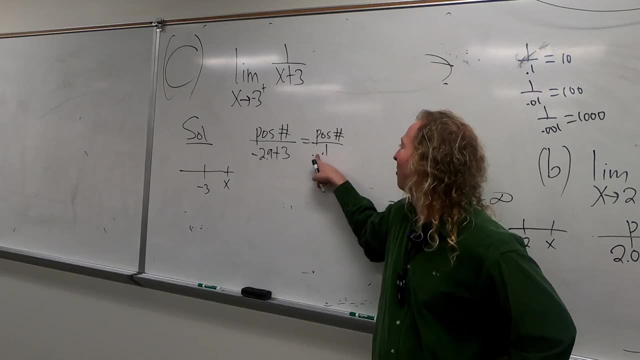 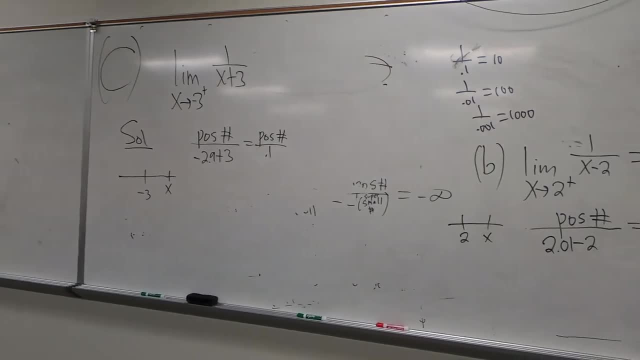 Is that a mistake, Even though I guess it is, Because I mean, none of the work is right anyways. No, I'll give you the point. Okay, I don't have a pen so I can't write it down. 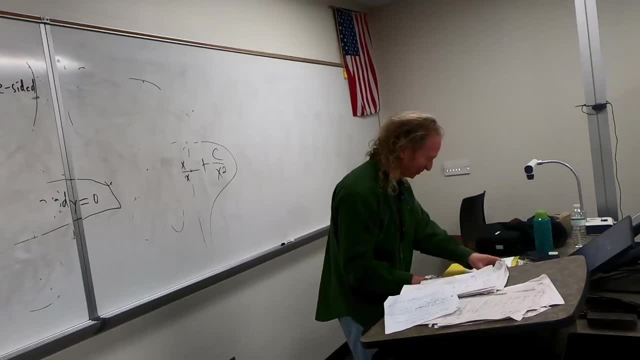 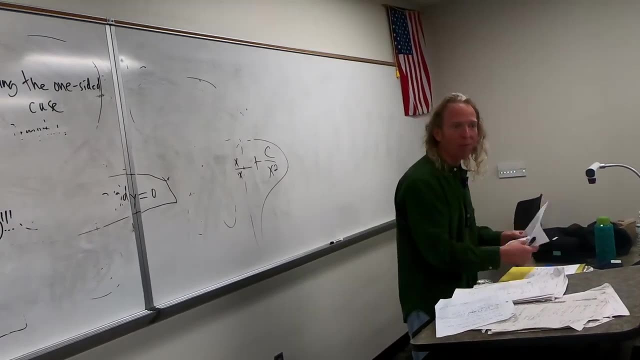 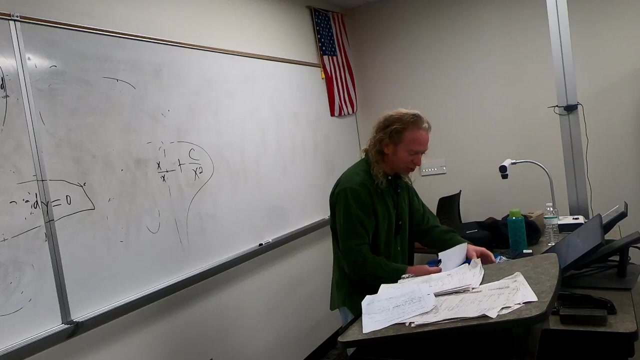 Okay, just throw it. Thanks, I'm bleeding, I'm kidding, I'm kidding. Do you all have any points for mistakes in this class? You do, Really, Really. Three, Three Ryan. that's the wrong class. 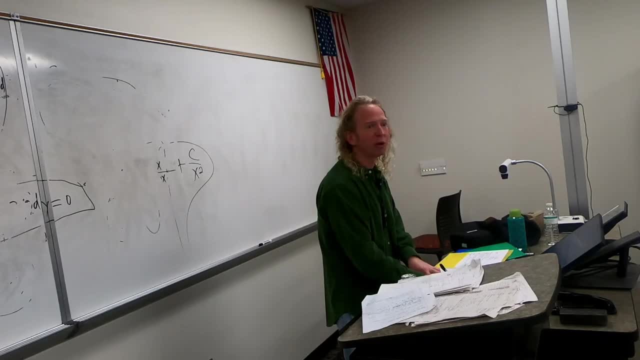 I see the names: Logan. Who's Logan? Oh, Logan, I'm sorry. Logan, I'm sorry You have two, John has one. And who got that one? Was it everyone? or, just Okay, everyone? All right, everyone gets two points. 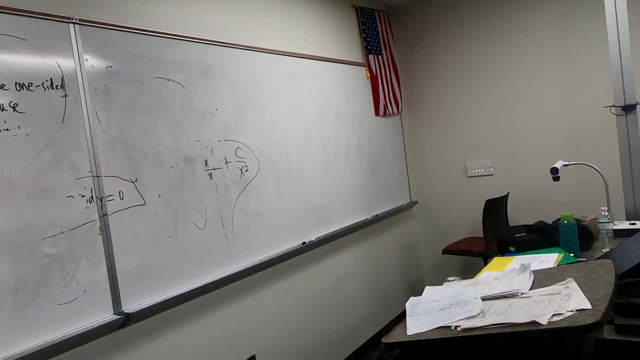 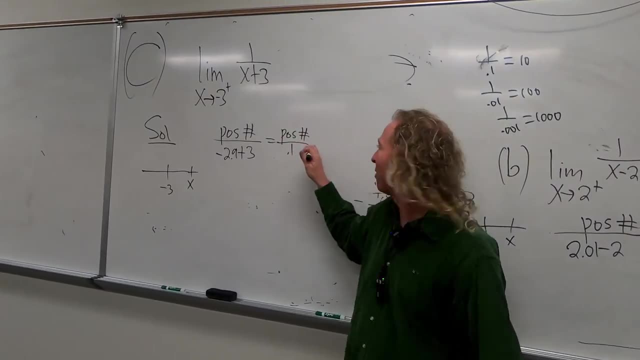 Here you go, Logan, I won't throw it. Good work, Thank you. Thank you. So Yeah, that's good. You might need the points. No, So it's going to be infinity Positive over something small. 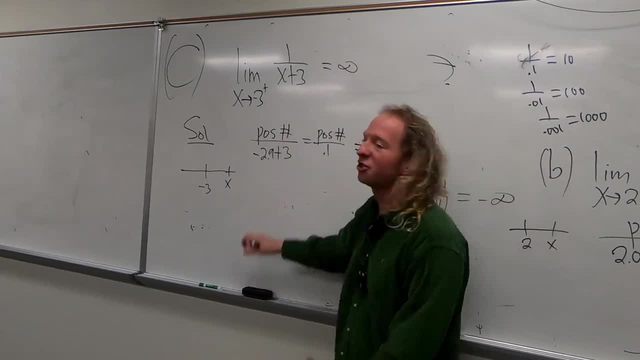 So this is big, So it's infinity. Good, Let's do another one. Let's keep going. We'll just do as many as it takes, right? Let's just do a bunch of these. So, because you want to get all these right, 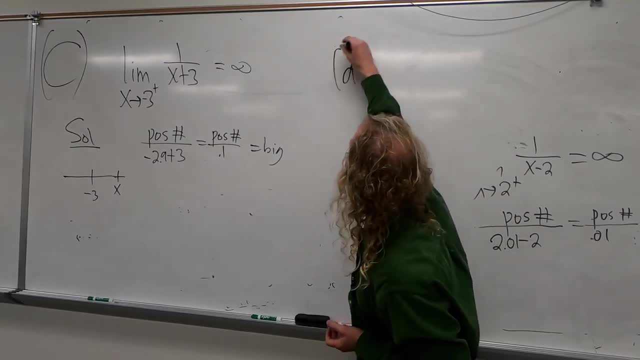 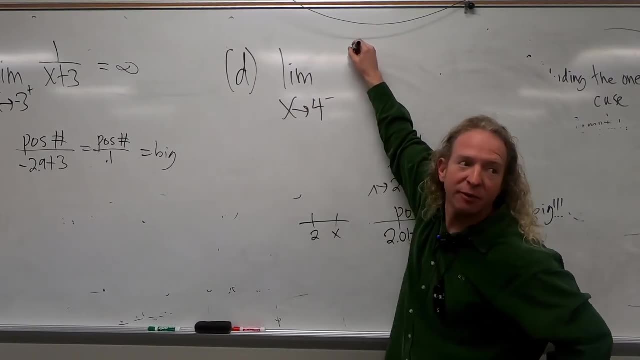 This is like 15,, 20 points on a test: right A, B, C, D. Let's try this one. I'll help you with this one: Four from the left And it'll be. oh, let's be weird. 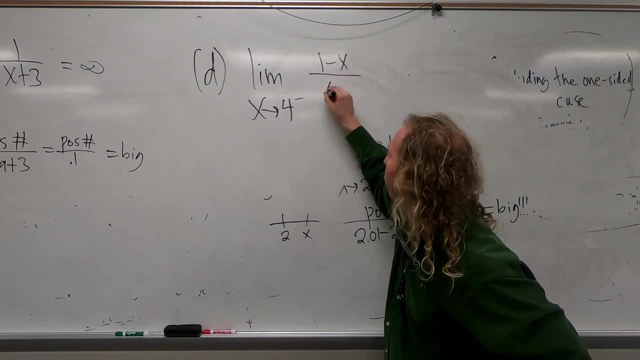 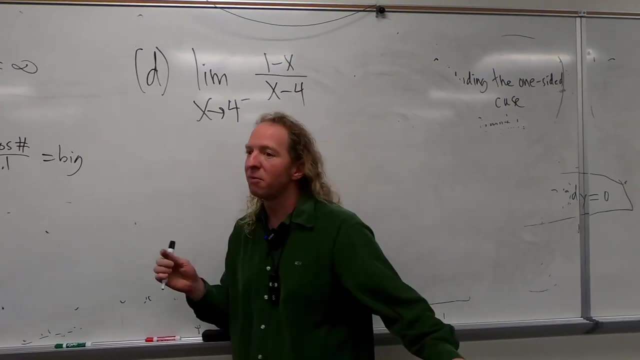 One minus X over X minus 4.. I'll work this one out for you Over X minus 4.. So 1 minus X over X minus 4.. So you can actually plug in the 4 in the numerator this time. 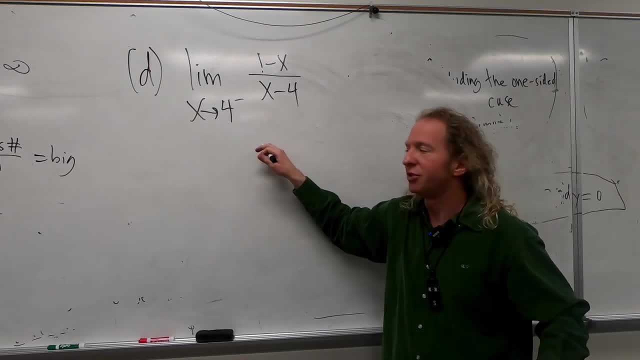 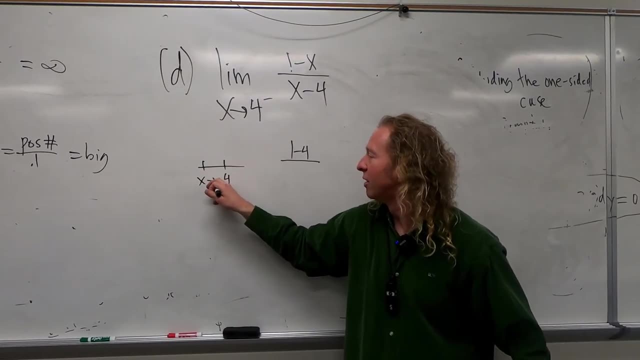 So you get 1 minus 4.. So you get negative 3, right. So you get 1 minus 4.. And then think about 4.. So from the left, This is so bad, Like we're plugging in different numbers. 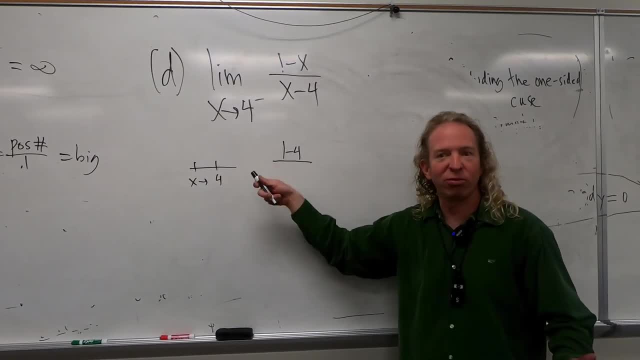 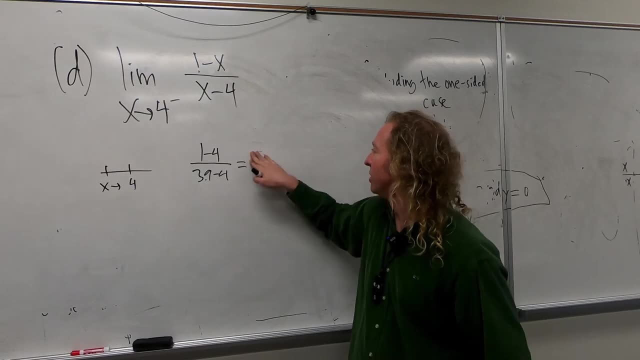 It's just so bad. 3.9, right, 3.9 would work. So 3.9 minus 4.. It's just so bad, Negative 3.. So I'm just going to put negative number. 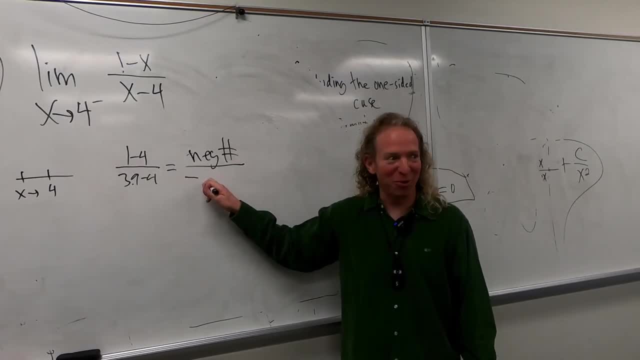 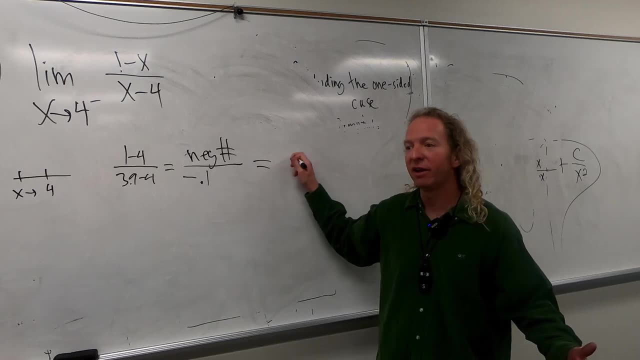 And then on the bottom, it's going to be negative 0.1.. Didn't mess up that time. Negative 0.1.. Oh, negative, and negative becomes positive. So what's this going to be? Infinity, You got this. 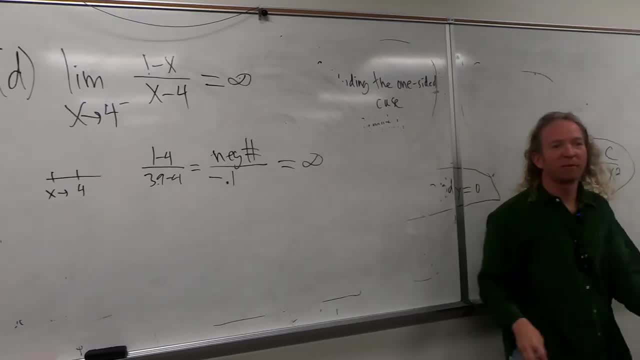 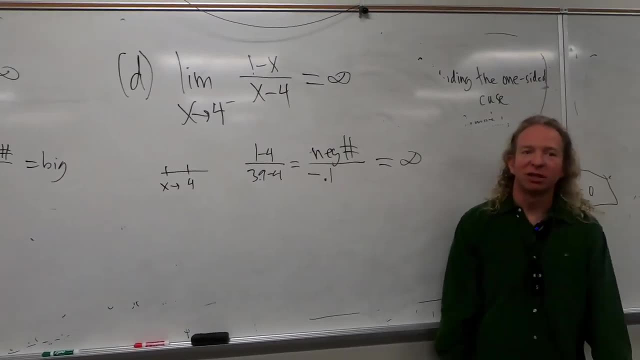 Infinity. So it helps give you some intuition. Yes, sir, You have 1 minus 4.. I know I'm being really bad. I'm plugging in different numbers, which is super wrong. Yeah, it's just all bad. 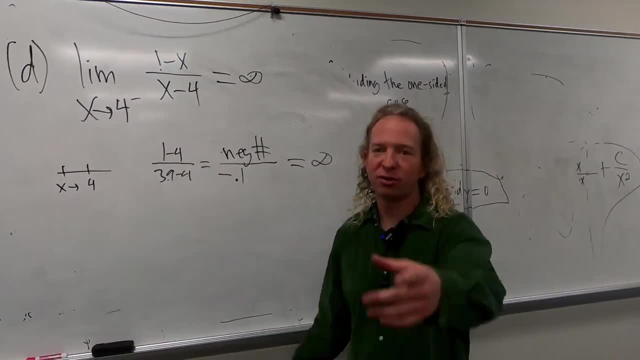 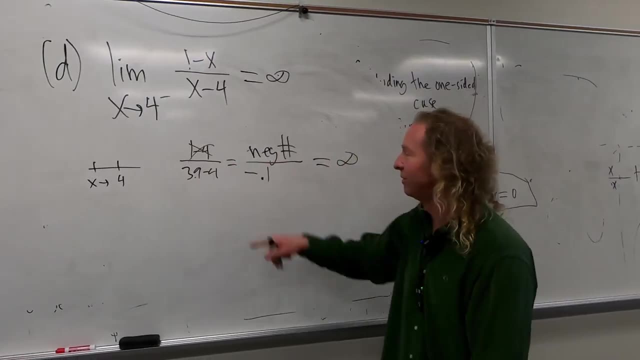 Yeah, It should be 1 minus 3.9.. It should You should. Good, Yeah, it should. I mean, I feel bad, I'm not going to, I'll just do that There. Negative number, That's more correct. 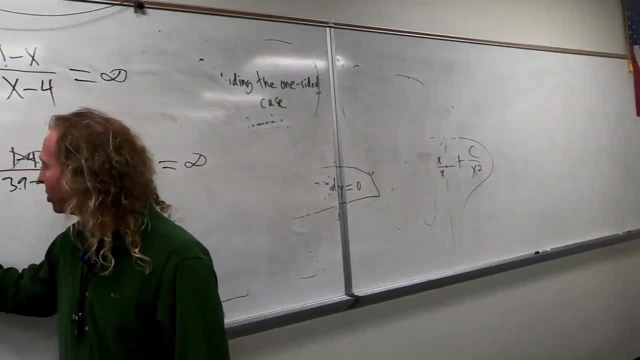 Even though none of it's correct. So it's infinity. Let's do another one. E Check this one out. This one's really interesting Limit- This is our first one like this. X approaches 2 from both directions. 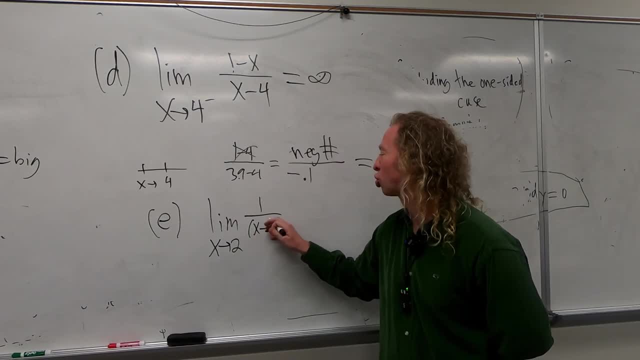 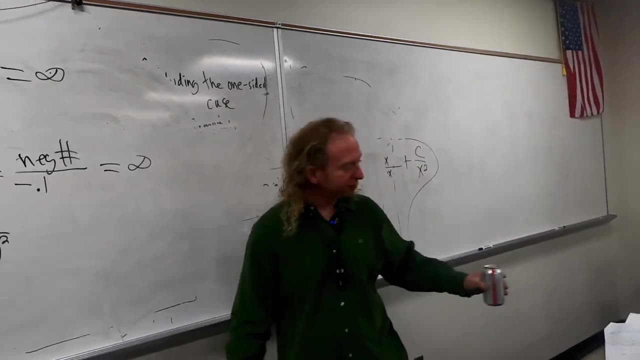 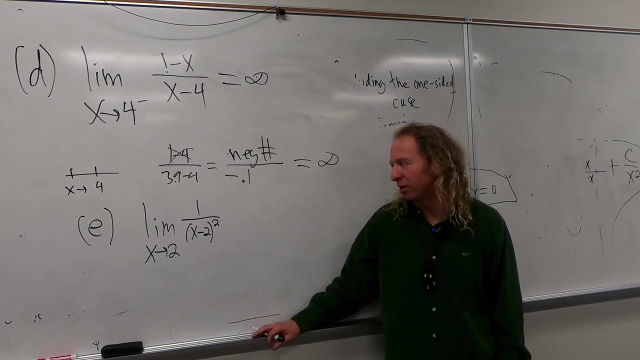 Okay, Yeah, Yeah, X minus 2. squared, Yeah, Squared. The nice thing about doing one section a day is sure some sections are intense, but like this one, this one's. after that we're almost done. We have a couple more things. 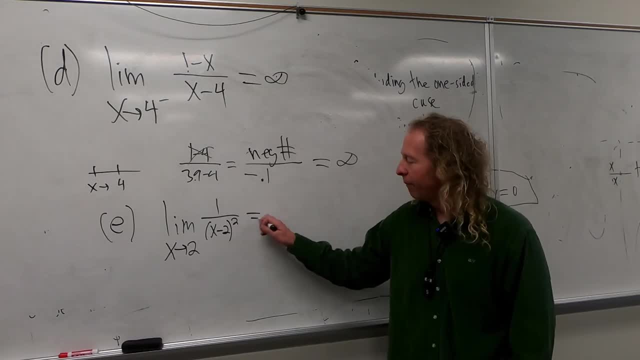 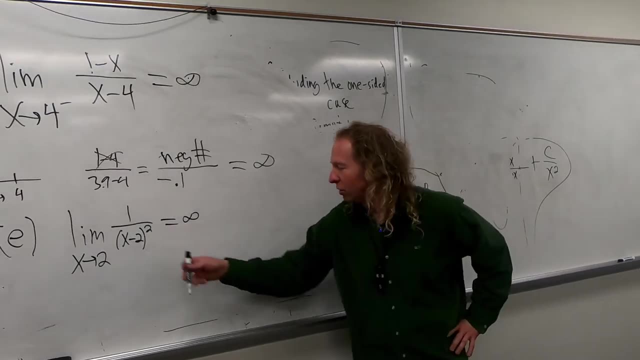 Positive infinity. Yeah, The answer is infinity. Yeah. Two ways to think about it. One: you can put it in your calculator graph it. Two: you know the graph and you can do it in your head. Three: You can plug in anything you like. 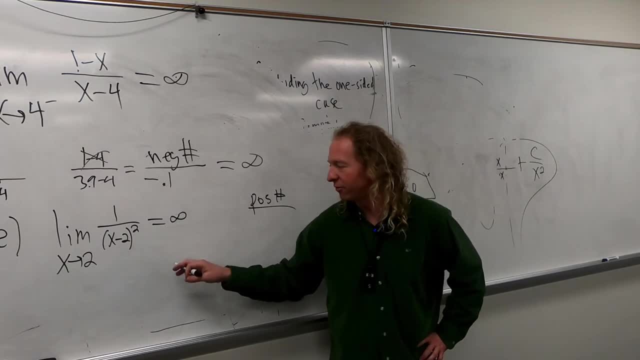 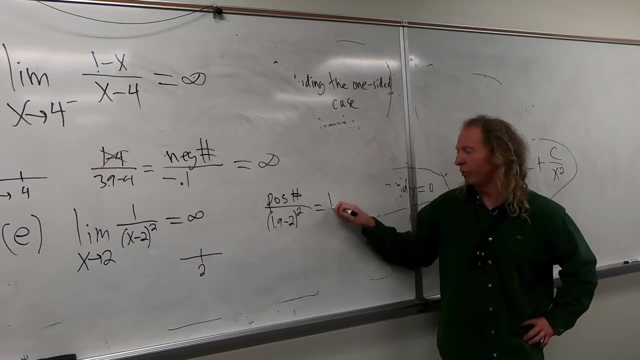 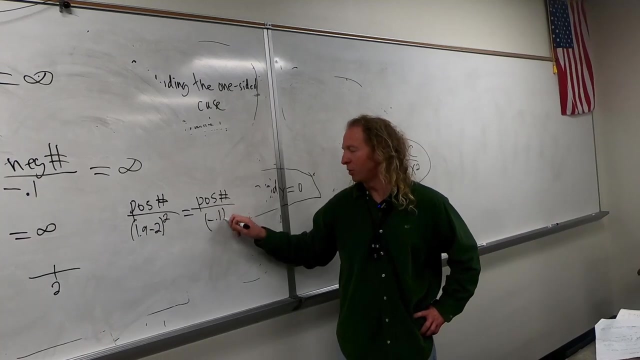 You have a positive number If you approach from the left. if you do 1.9 minus 2, you get a positive number, And then you get negative 0.1 squared. When you square a number between 0 and 1, it becomes even smaller. 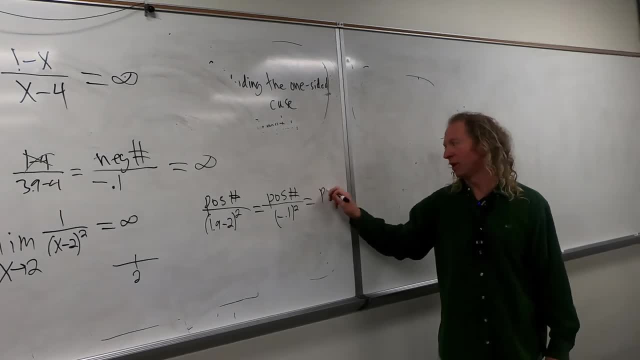 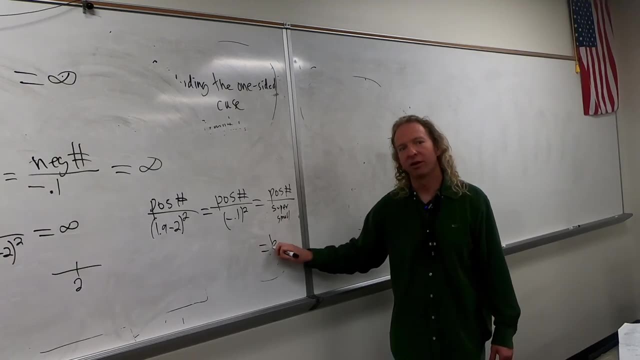 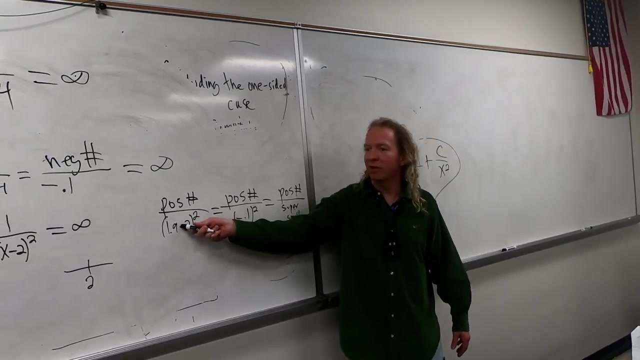 So this is going to be a POS number over something super small. So it's big, So it's infinity, So it's infinity. So when you square it, it becomes positive, no matter what. Yes, Reese. 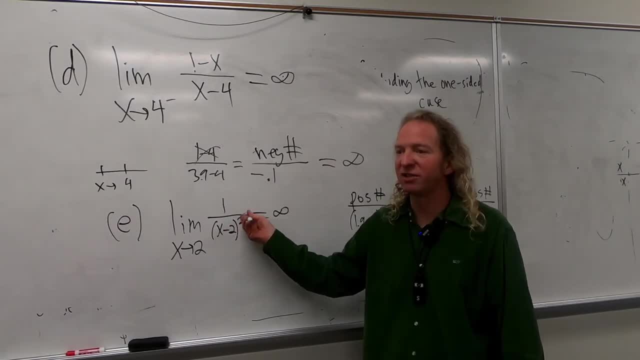 Yeah, because it's squared. Yeah, You just say, hey, no matter what you plug in, it's going to be positive. Yeah, That's even better. Yeah, That's even more pro. Yeah, Totally Yeah, Mm-hmm. 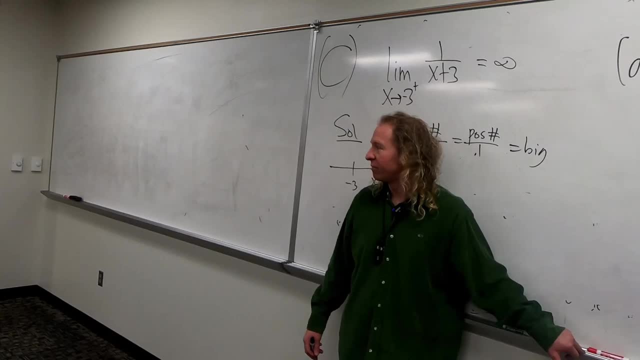 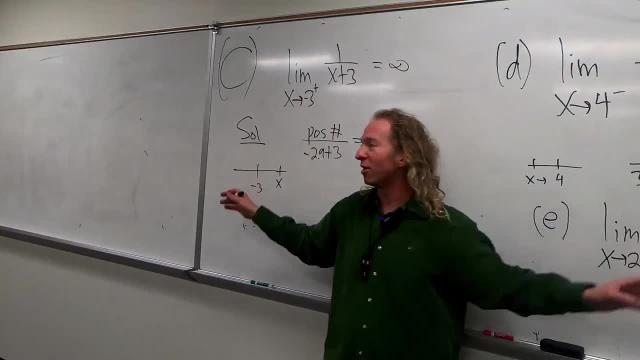 But no work necessary at all. Yeah, You don't have to show any work. Mm-mm. Yeah, You can do anything. You can graph it in your calculator. If you have a calculator, you know how to use it. You can put this in there. 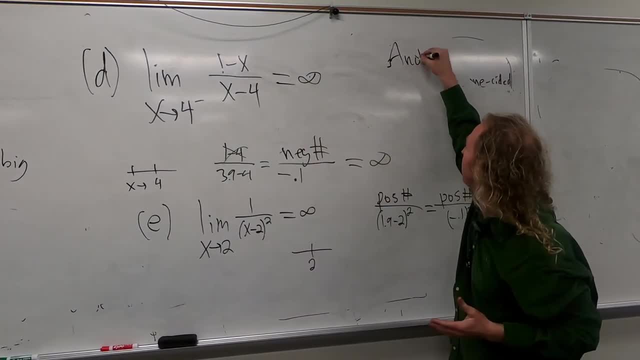 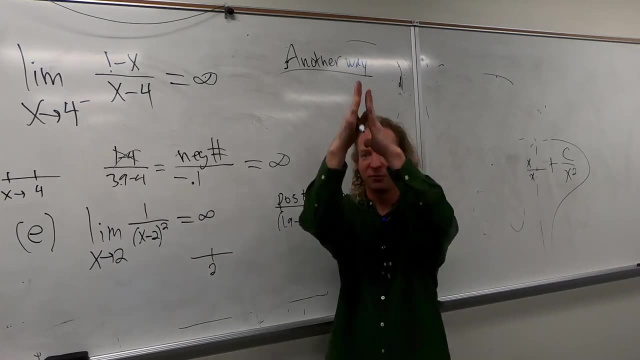 If you graph this in the calculator, watch this Another way, Check it out. I've never talked about this, ever, ever. I don't know why, Because I'm bad. This is the volcano function. That's how I memorize it. 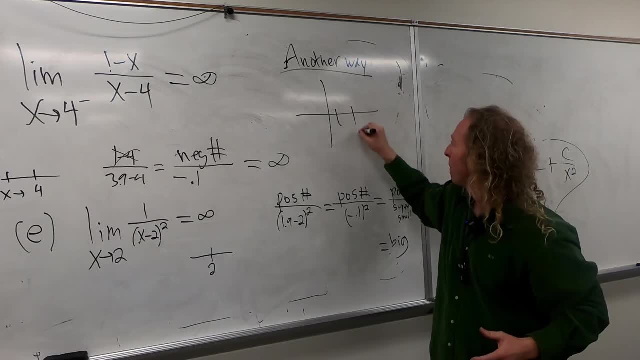 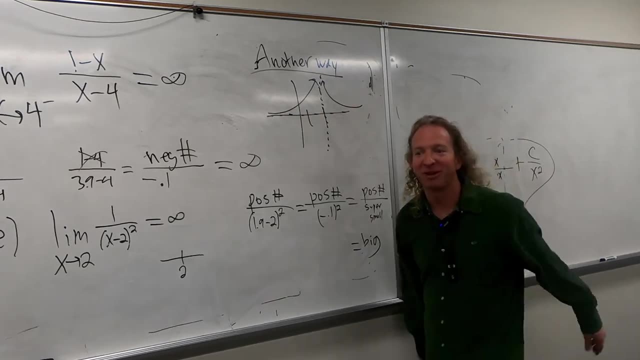 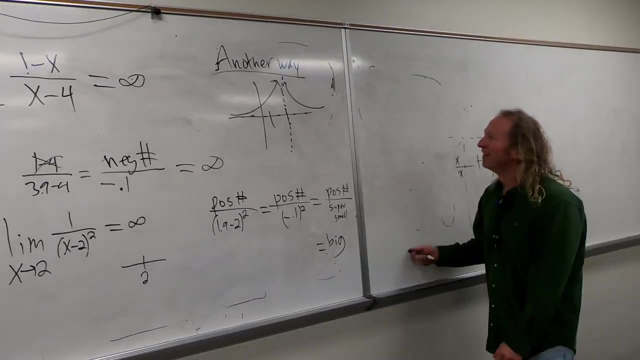 And it's shifted to the right by two, So it looks like this: Okay, So it just goes to infinity, right? Do you remember this from college algebra: The volcano? Yeah, yeah, I don't know. I haven't taught college algebra in a while. 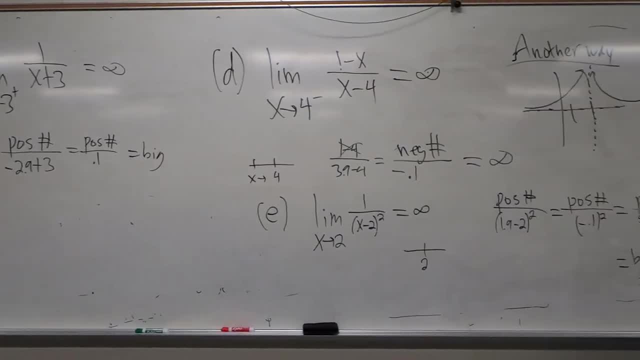 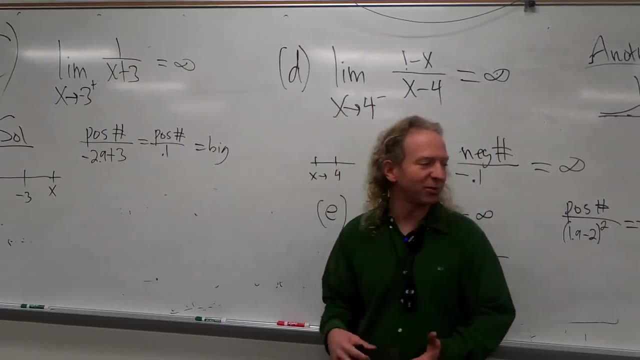 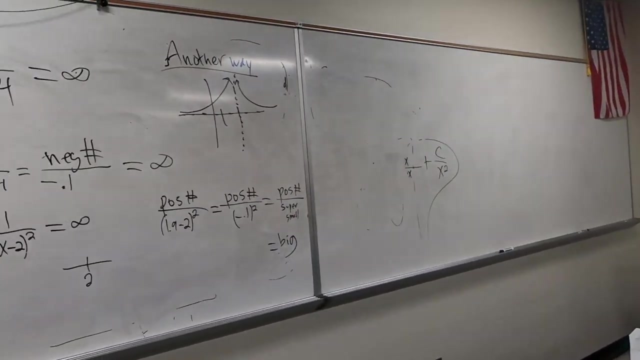 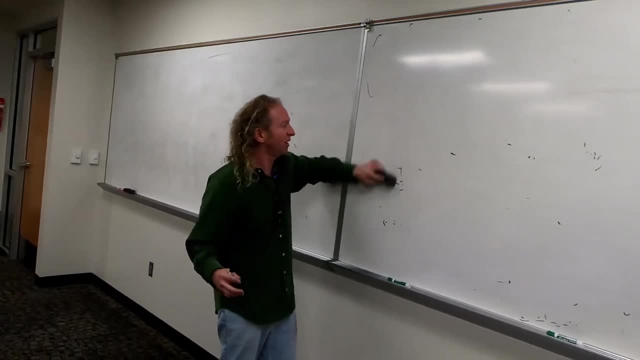 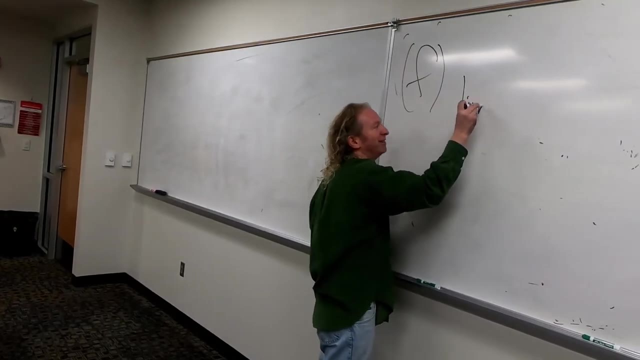 Check this out. Let's just go: nuts A, B, C, D, E, F, F. F is next right, F, F Failed. No, I'm kidding, Limit, Let's approach, let's approach. 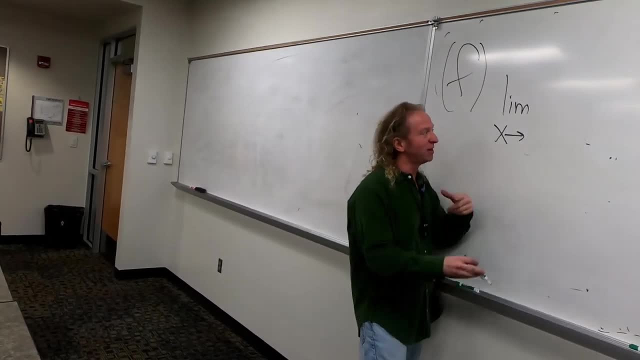 This one's really hard. This one I might be in the homework. There used to be a teacher. He doesn't work here anymore. He's a friend of mine And I ran into him in the hallway one day And he goes: hey, check this out, man. 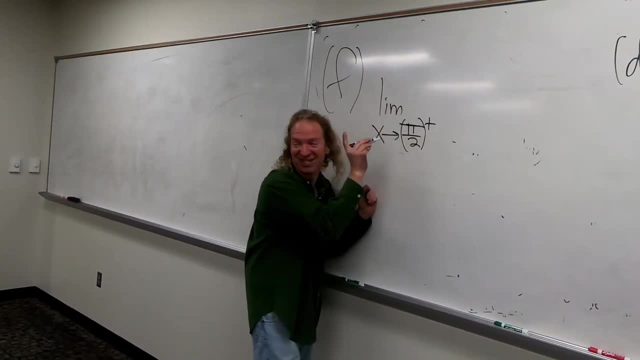 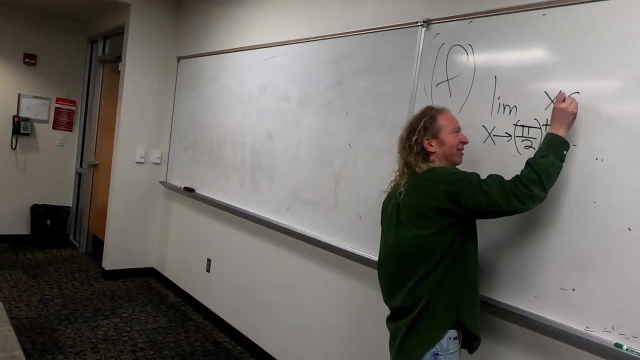 And he gave me this problem. Yeah, this is really evil X. what's worse than cosine Secant? It's ridiculous. It's about as hard as it gets. We'll do a couple of these until you get it too. 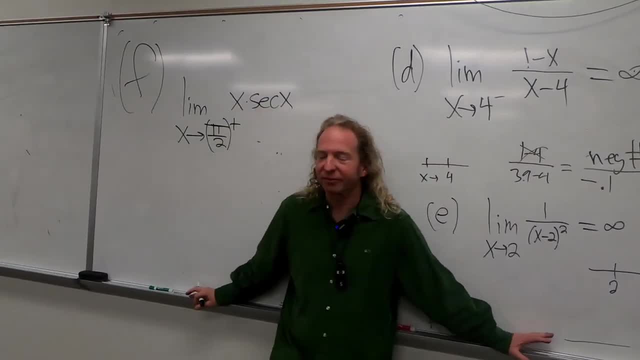 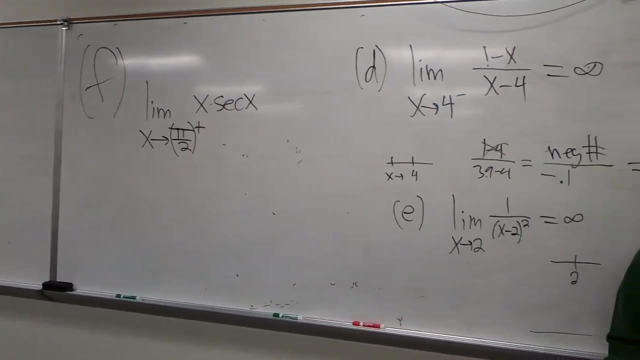 So throw a trig function in there and it makes it a little bit harder. So secant is one Over. what function Do you all know? Cosine, yeah, And if you don't know, it's okay. There's a really easy way to memorize it. 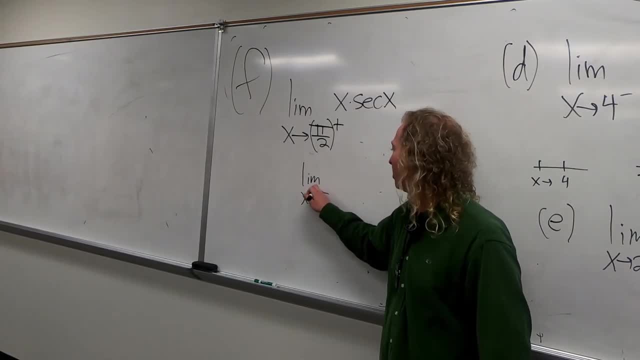 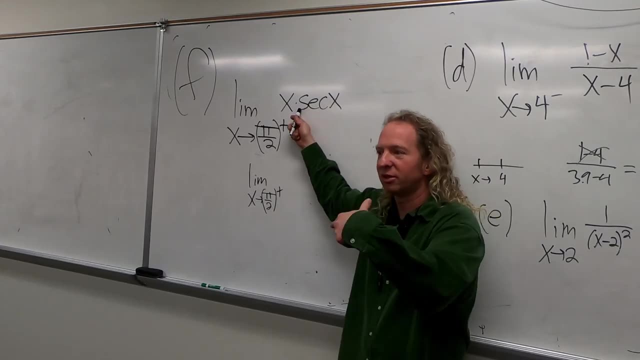 At least the way I do it is. I know it's one over the one that starts with the other letter, So it has to be cosine Right, because it starts with a, C, And then cosecant is one over the other letter. 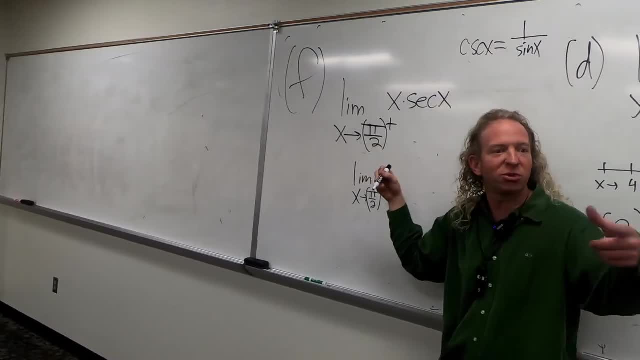 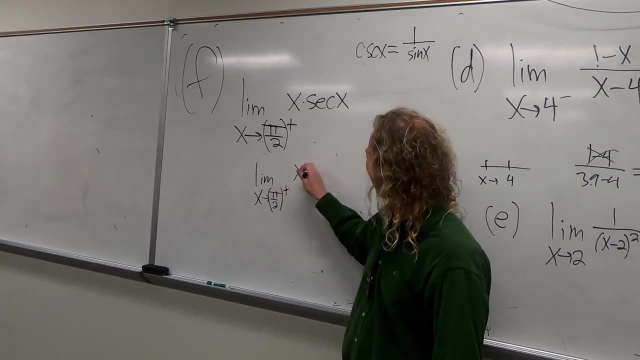 So, sine, yeah, That other letter trick is really good. Is that how you all do it too with the other letter, Really? Oh, so I'm not alone in my weird Good, good, good, It's great. 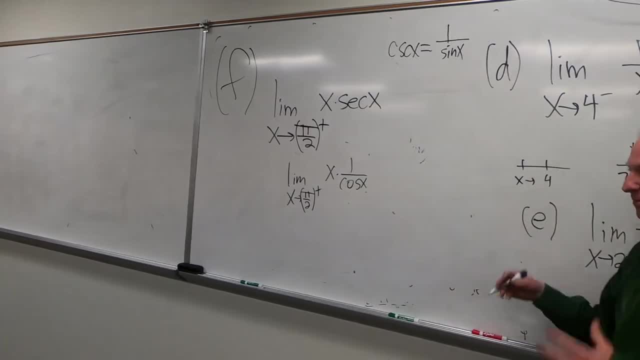 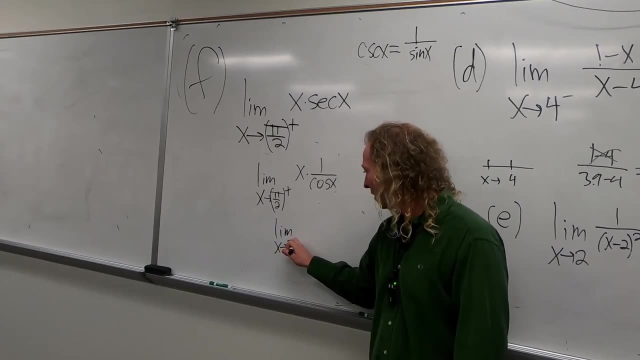 It's amazing how humans are similar deep. I'm going to rewrite it again. That's bothering me. I'm going to write it like this. So, basically, we are rewriting it in a way that will allow us to think about it a little more clearly. 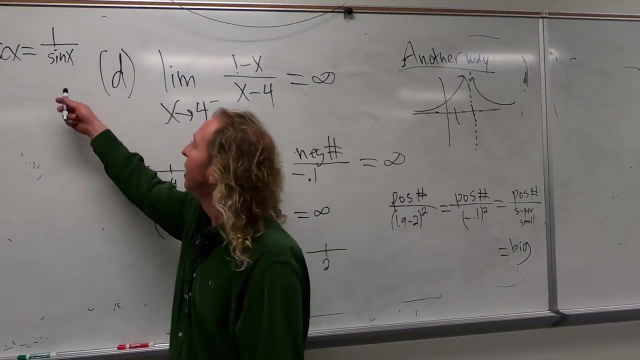 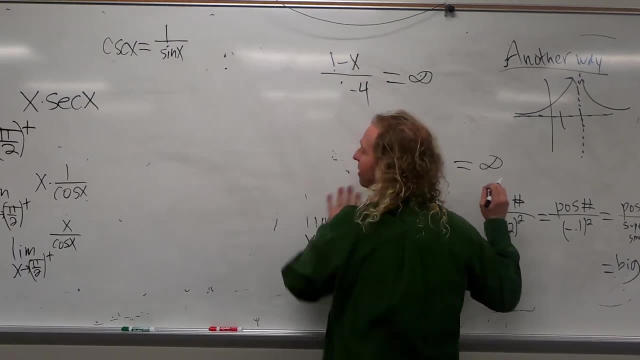 So if it was cosecant, it would be one over sine Right, it would be one over sine. Okay, So up top it's going to be simple, right? What type of number are we going to have up top? Positive or negative? 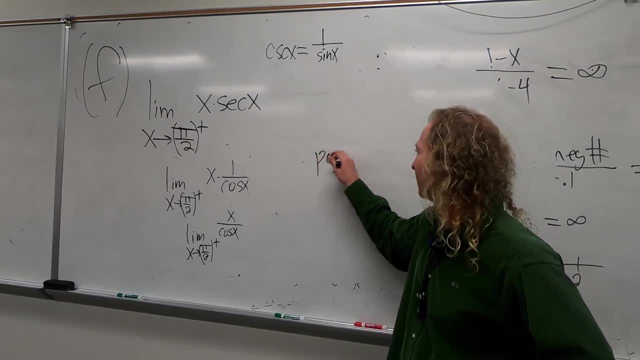 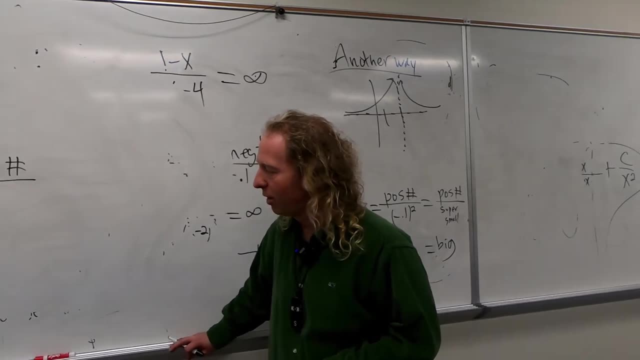 Positive, Yeah, positive. So I'll put POS number. Okay, The bottom part is tough. I guess there's two ways of doing it. You could use the unit circle. I'll try to do it that way. I'll struggle with that, but I think I can do it. 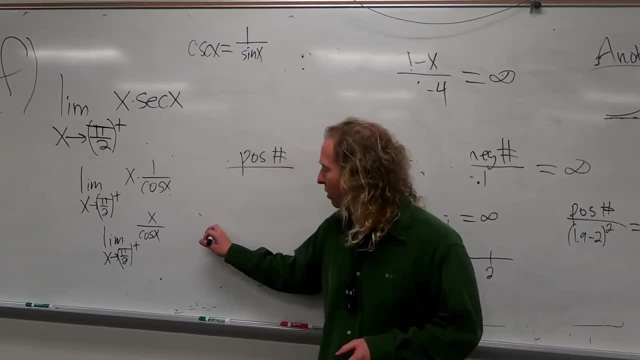 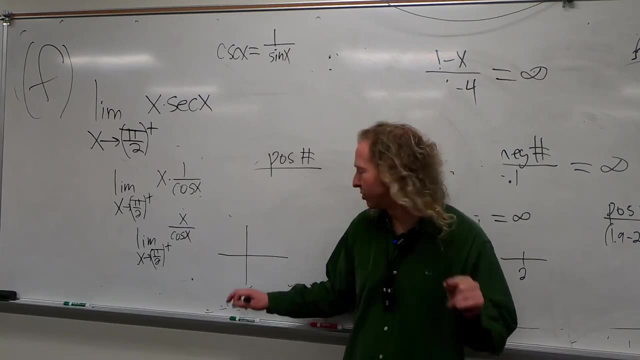 The graph might be easier. Think about the graph of cosine. So the graph of cosine. if you don't know it, just memorize one point: What's the cosine of zero One? So it starts here, right, Sine starts here. 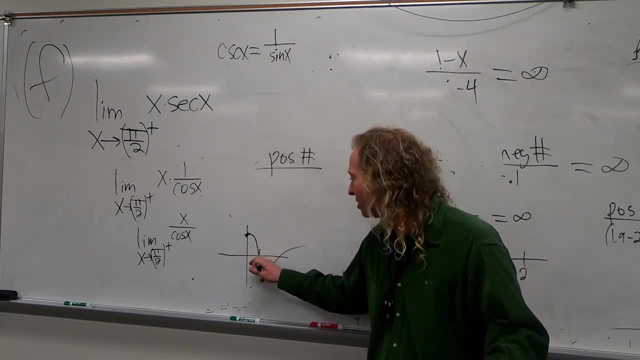 And then it's a wave, so it does this, Okay, And then you know that this is pi over two, Because cosine of pi over two is zero. I have that one memorized. So this is the graph of cosine, right. 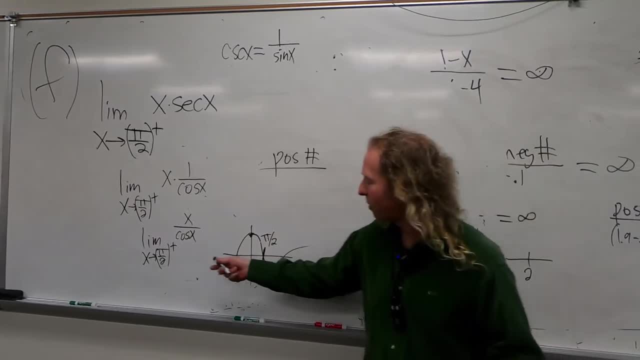 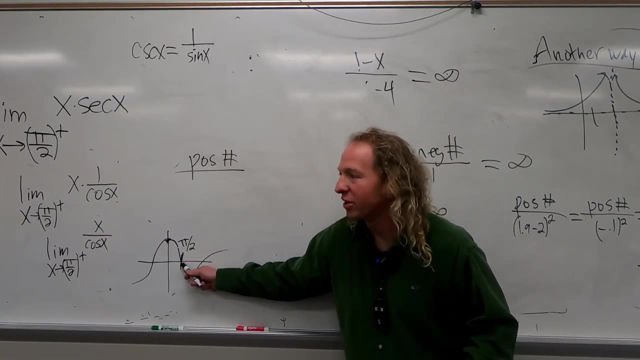 This is cosine x. Okay, So x is approaching pi over two from the right. So x is coming from this way, right? So are the y values negative or are they positive here? Negative, Negative, So it's negative and it's super small. 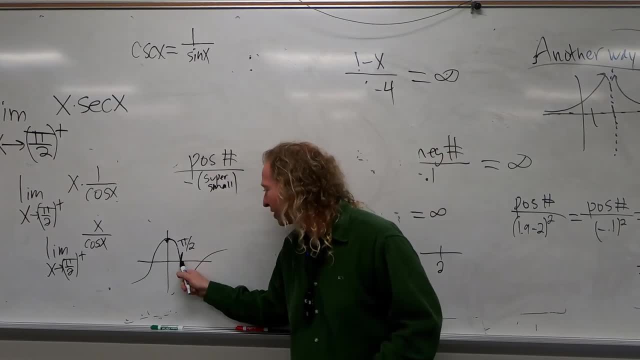 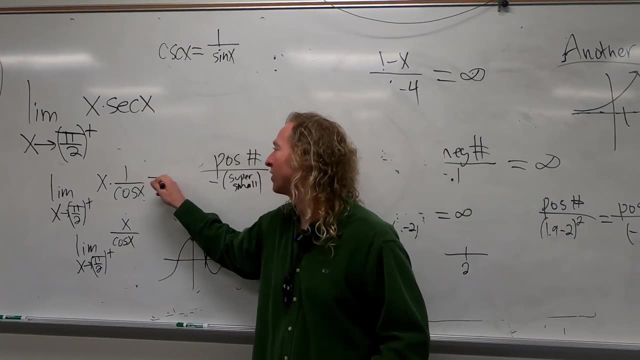 The reason it's super small is because it's really close to zero. It's like negative 0.0001, right, So then this is going to be negative infinity- Really slick. Yeah, the guy who showed me this, I remember. 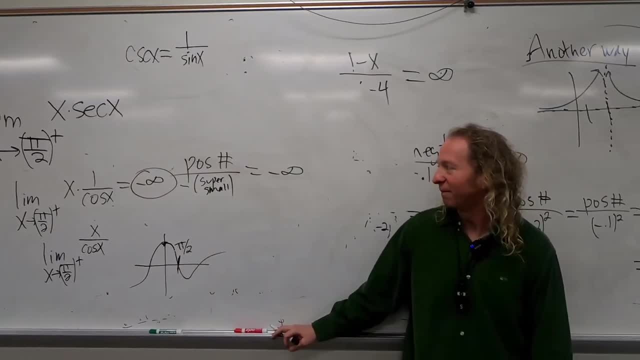 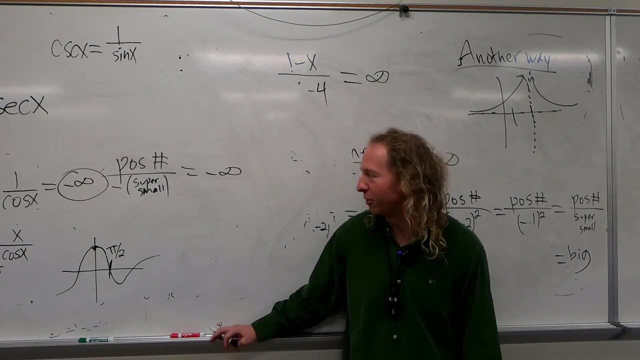 because, yeah, really, really slick. I wonder what happened to him. I used to have his phone number but I had to get a new phone, So, yeah, Yeah, Really sneaky. He's like check this out. 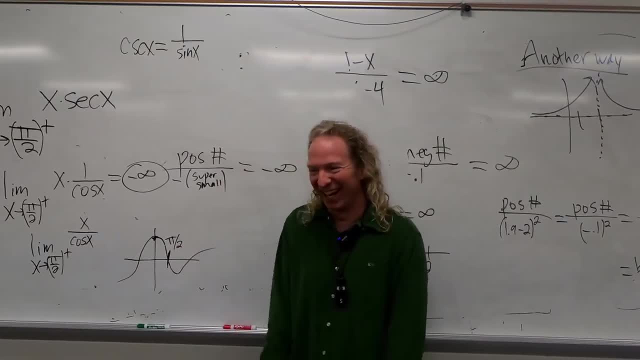 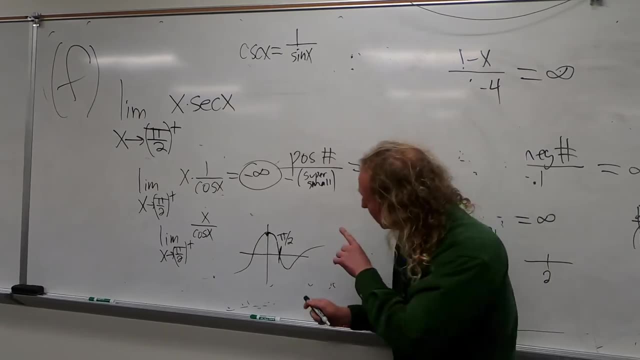 I'm going to put it on their test. I'm like whoa, Like it's hard, right, It's really sneaky. Any questions? Yes, Why is the bottom super small? again, Like I mean negative. 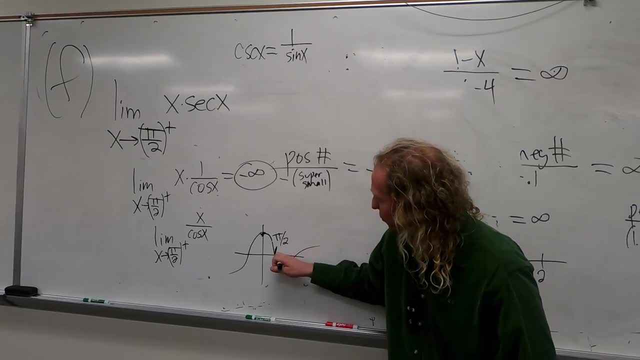 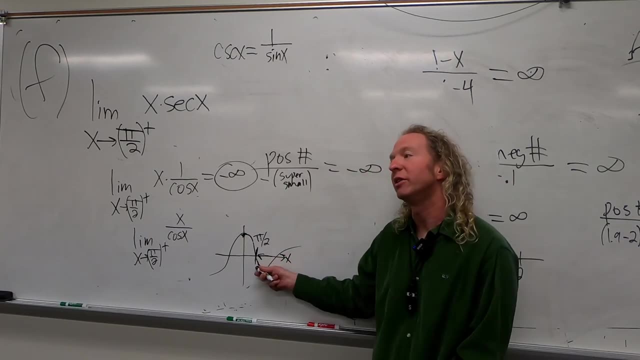 Good, Because okay. so this is the x is approaching pi over two from the right right, And so the y values are here where my marker is. So you see, this is the x-axis. So all these y values are negative down here. 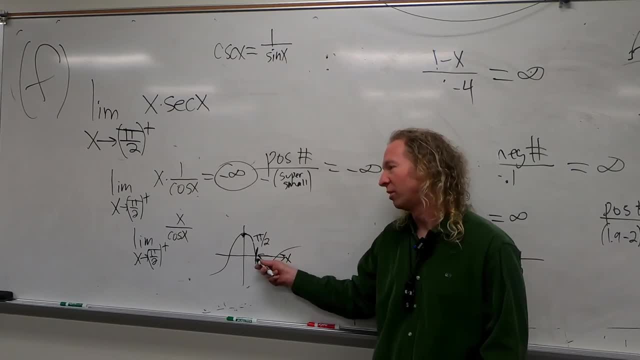 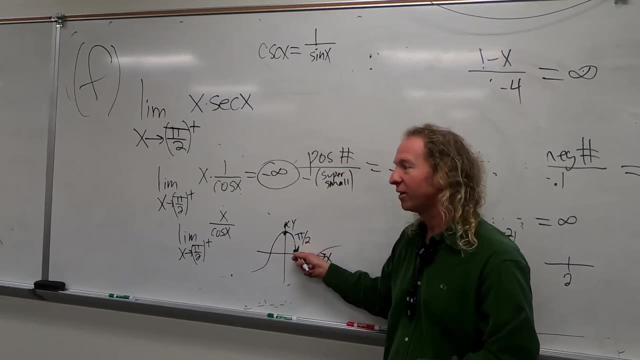 That's y Right And they're getting close to zero, so they're small Right, Because this is the y-axis. So these are positive y's. So if it was from the left it'd be positive. Yep, Good question. 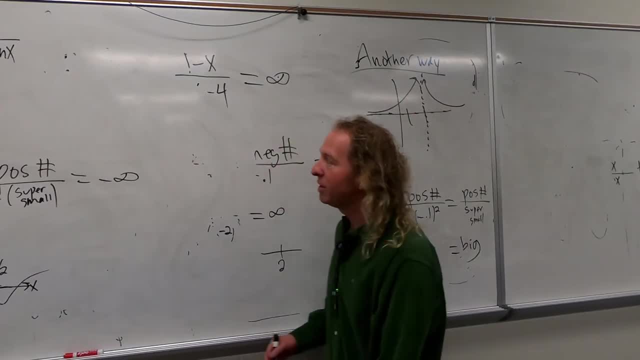 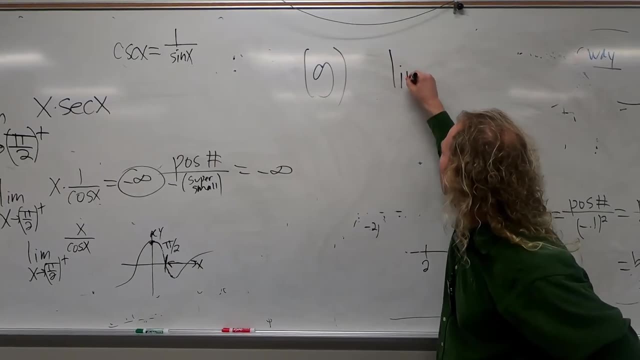 Good question, Let's do another one. Let's do another one, Let's do one more: A, B, C, D, E, F, G, Let's try limit x approaches. Let me look at the homework for ideas, because oh, I know, I know. 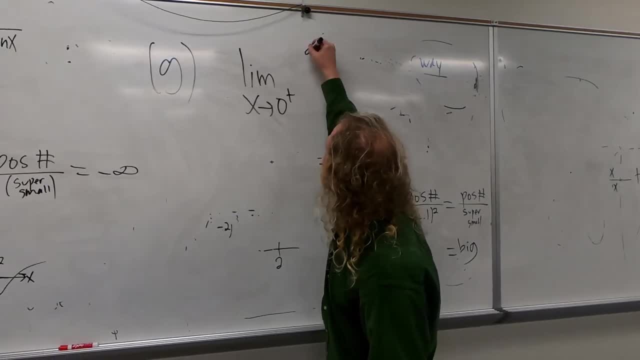 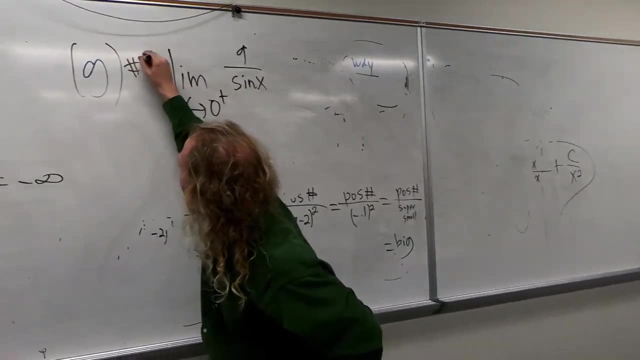 This one. This is in the homework. It's perfect, It's perfect. This is number Number 15 in the homework, Number 15.. Do you all want to try this one, or should I do it? Let me do it. 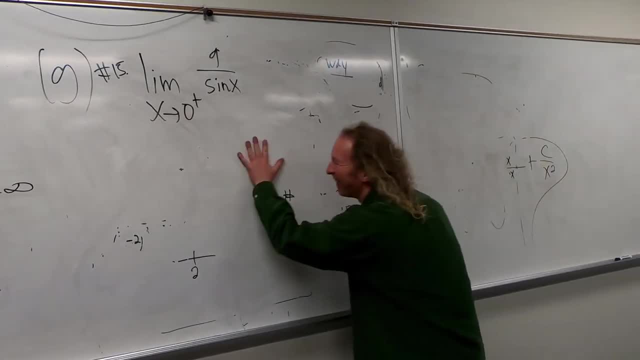 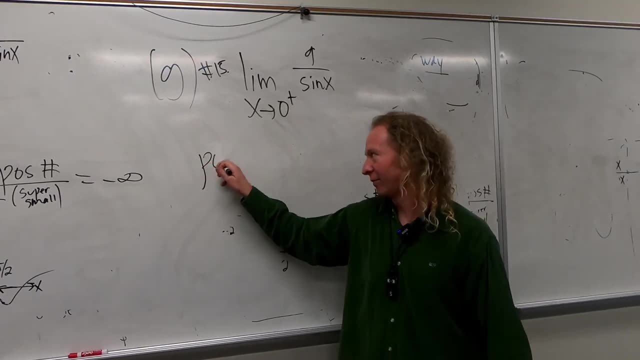 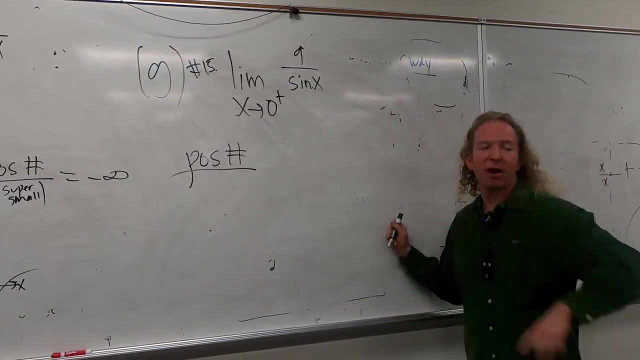 Okay, All right. It's okay, All right. So up top we have a POS number Right, So that's easy. So positive number up top. This one's not as hard as the secant one. And then we have to think about sine on the bottom. 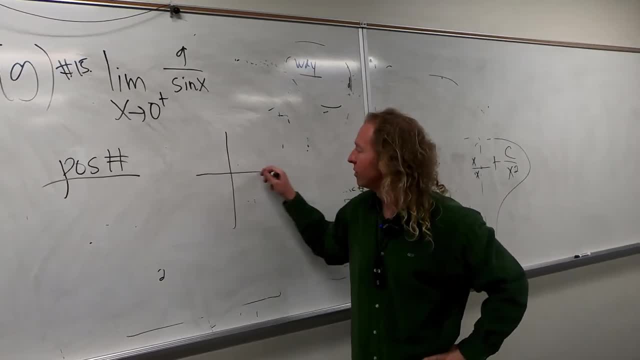 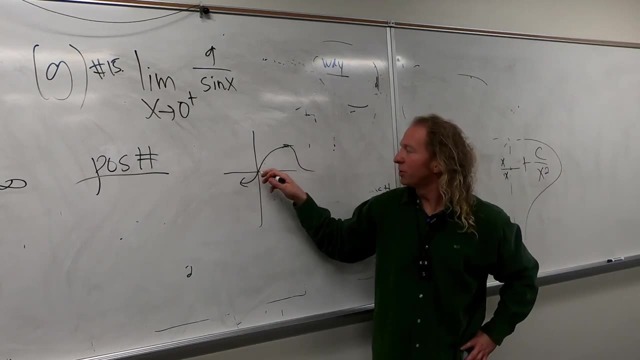 Sine of zero is zero. So let's draw the graph of sine. So it looks like this, and et cetera. It keeps going. You know that's a terrible graph, but yeah, So here's zero. So we're approaching from the right. 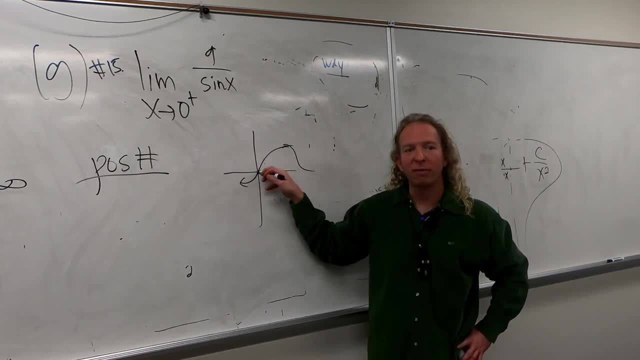 So the y values, when we approach from the right, will they be positive or will they be negative? Positive, Yeah, positive, right, Because they're up here. So it'll be super small and positive. So it's just infinity. 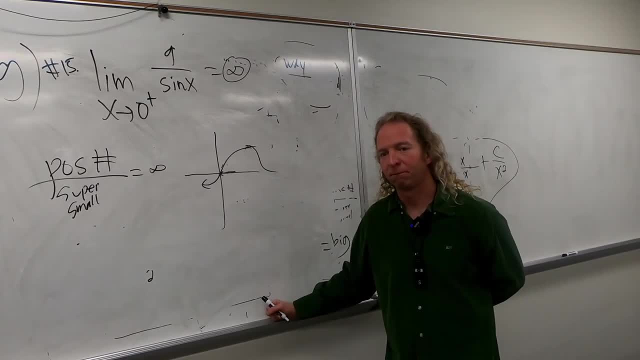 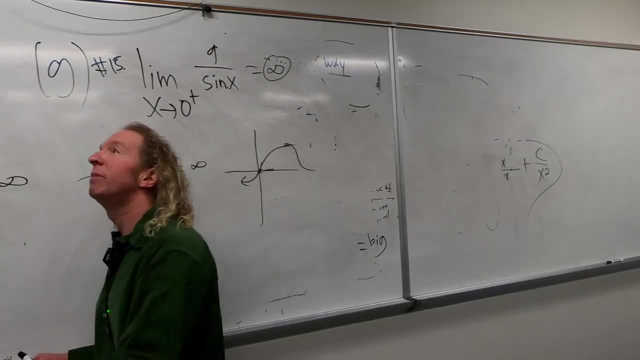 Yeah, So if we have super big in the denominator, is it going to be negative infinity, since it's an infinitely long denominator? No, Oh, super big in the denominator, So like x, Yes, Yes, We haven't done that though. 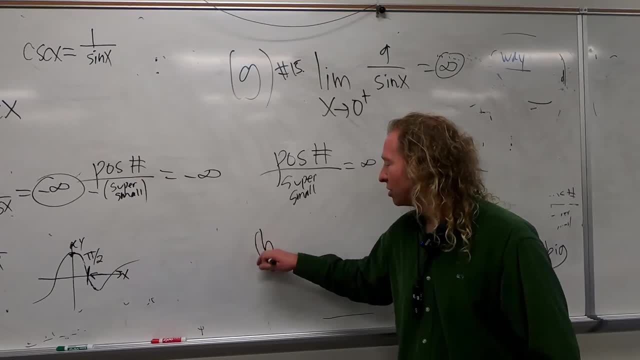 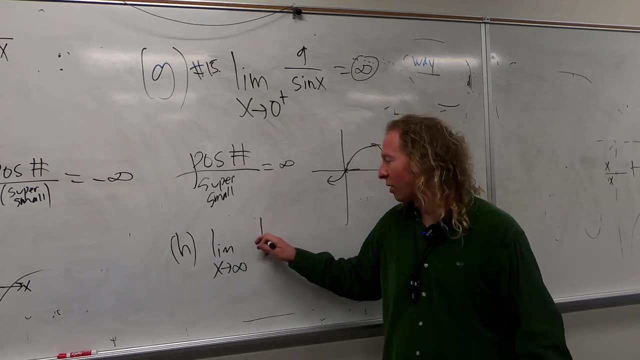 But yes, just for fun, because we talked about it. H, Not on the test, but let's say we haven't done this yet. You see a lot of this in Calc 2 and in Chapter 3 in this course. If you have like 1 over x. 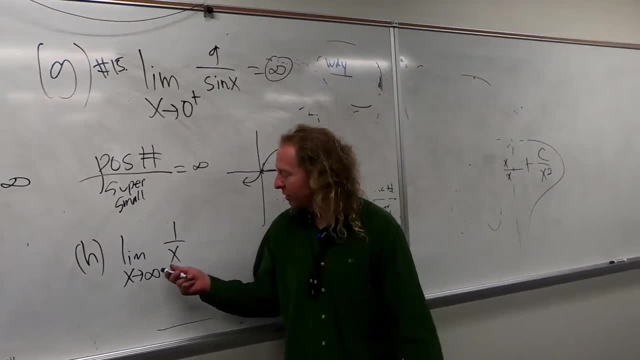 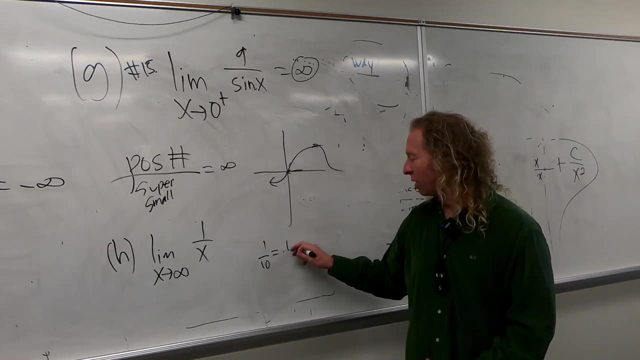 Yeah, Yeah, this would be 0.. We haven't talked about this yet, But basically, when x gets really really big on the bottom, the fraction gets really really small. Think of it as like 1 over 10 is 0.1.. 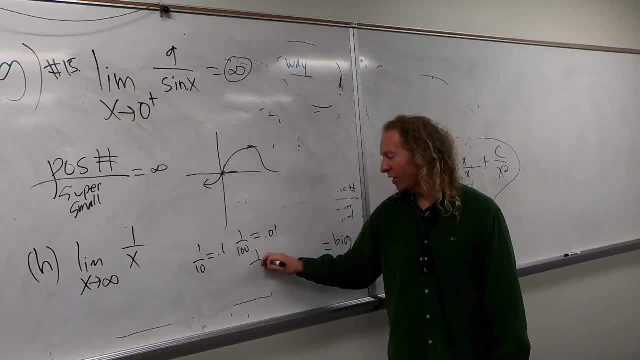 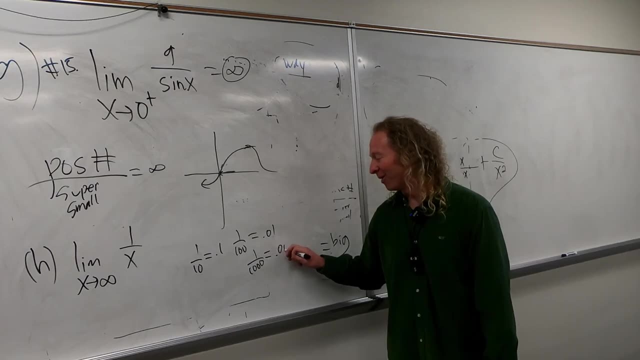 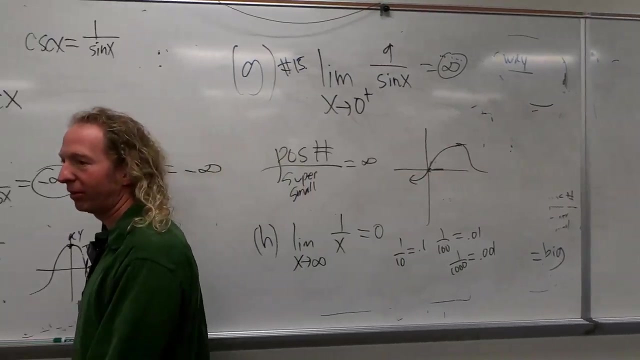 1 over 100 is 0.01.. 1 over 1,000.. I almost messed up- is 0.001.. So this is 0.. Yeah, Yeah, Yeah, that comes up later a lot, That's a big deal. 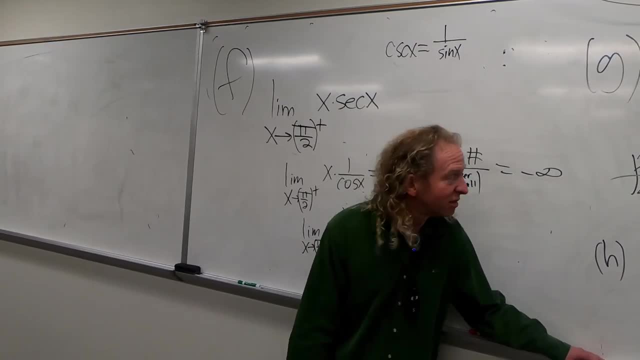 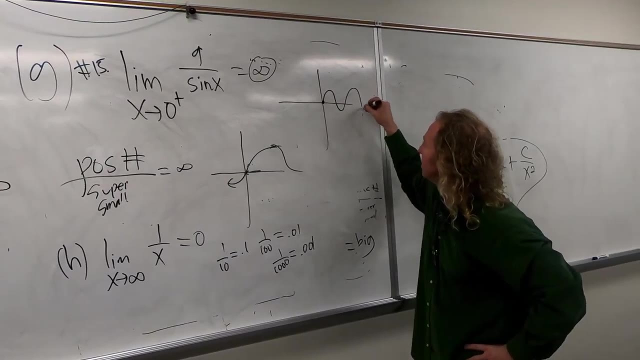 Yeah, Does the sine graph go down into the negative zone? It does. Over here It looks like this: So sine of 0 is 0, and it does this, doesn't it? Yeah, So how do we know? like from the right. 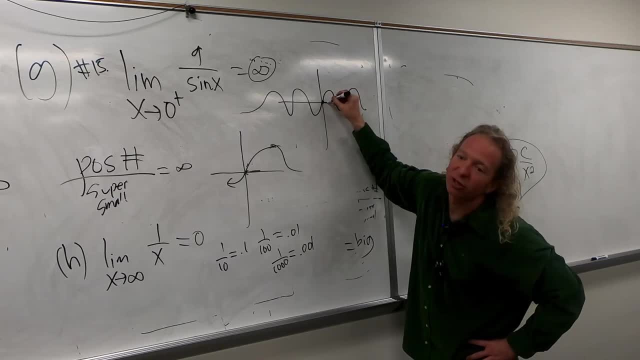 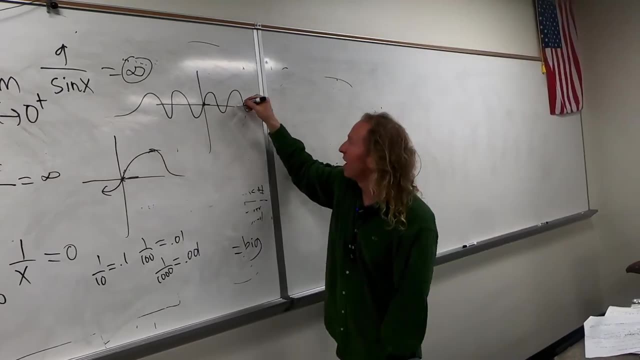 Coming from the right. Yeah, Oh, you're here. You're really close, Oh, okay, So it's just right. Remember what Ethan asked. He had a really good question. He said: wait a minute, How do you know if you're coming from this way? 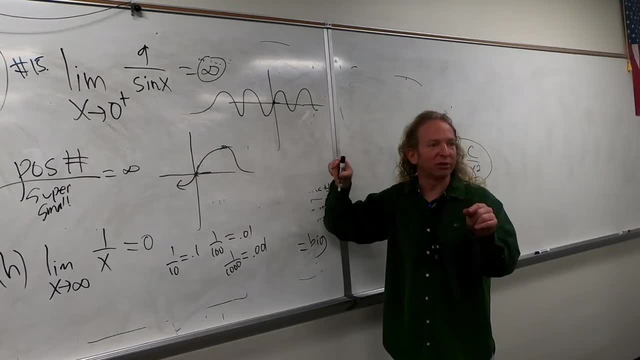 How do you know it's not up here or down here? right, You have to be really, really close, How close, As close as you can possibly be, How close as you can possibly get mentally so there, Good question, Ethan. 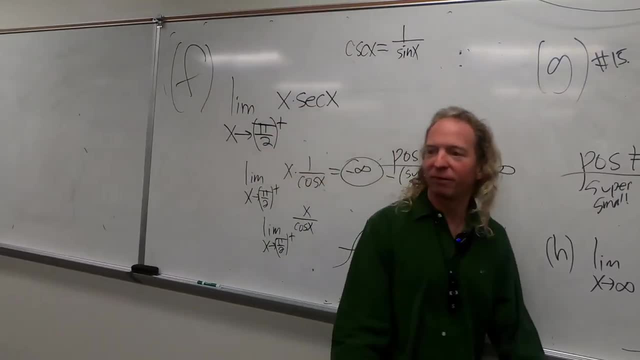 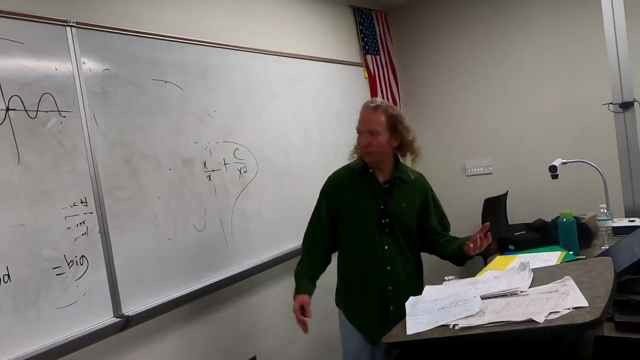 Very good question. Yeah, Yeah, Good. It's really good, Good, Good stuff. I like this. I don't know why. Oh okay, What's this? What is going on here? We should do 16.. Let's do it. 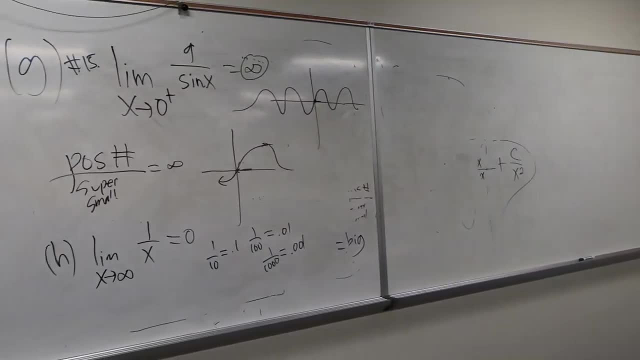 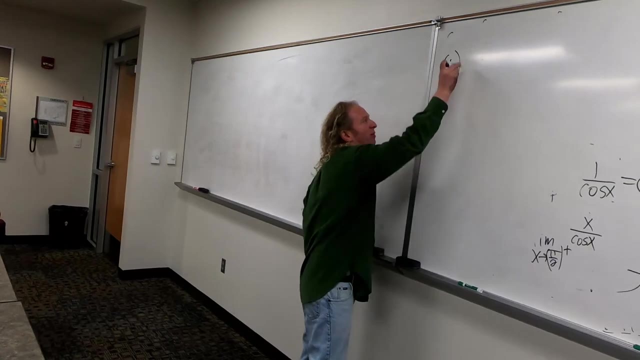 X approaches pi over 2 from the right. So this is A, B, C, D, E, F, G, H, I, J, K, I, I, I. It's a pirate's limit X approaches. 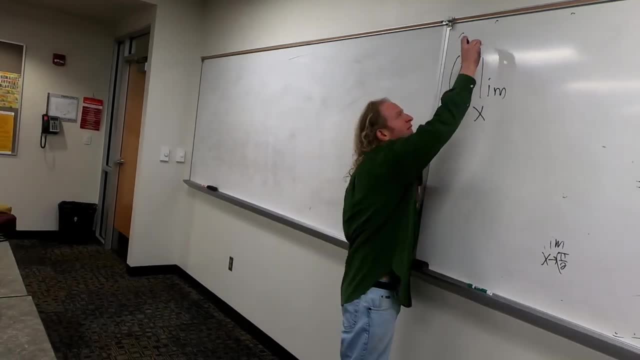 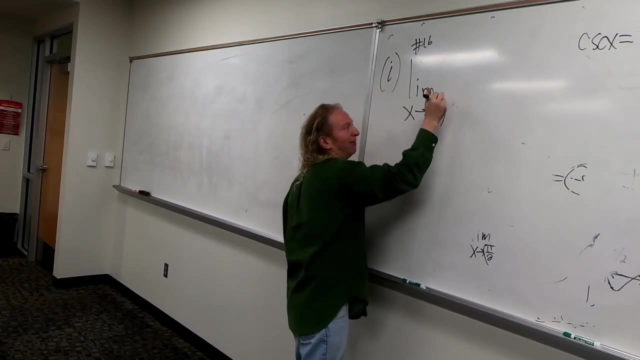 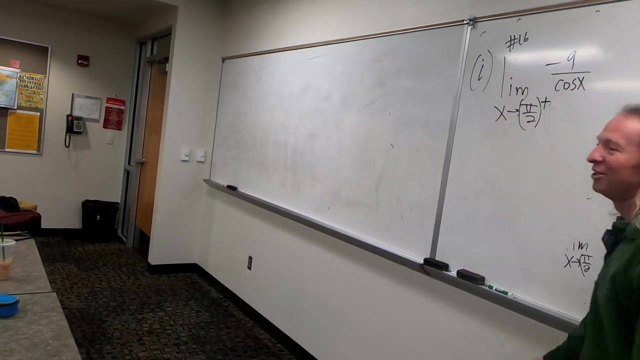 Anyone have the homework? Does anyone have the homework up 16? From the right, And what's the oh, What's the uh? All right, Do you all want to try this one? You should try it. You should try it. 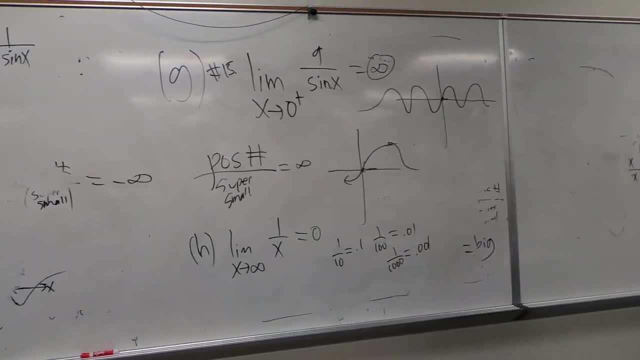 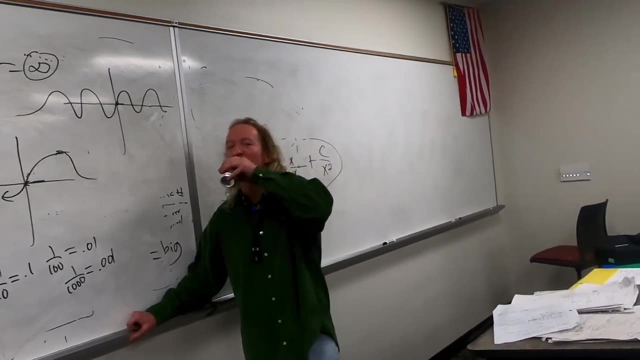 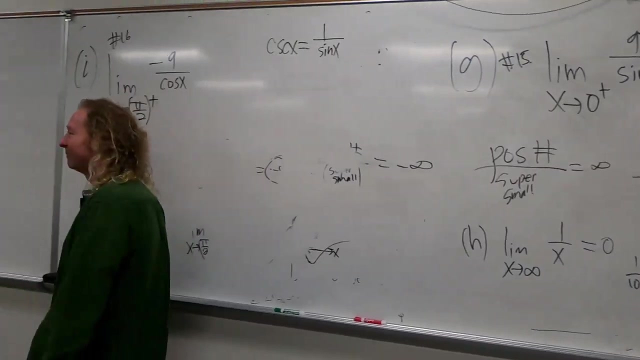 Yeah, try it. I believe in you. You got this, Try it, Try it. You got this, Aaron And not. uh, Sorry, Judah, Judah, You're sitting somewhere else today. Oh, What'd you get? 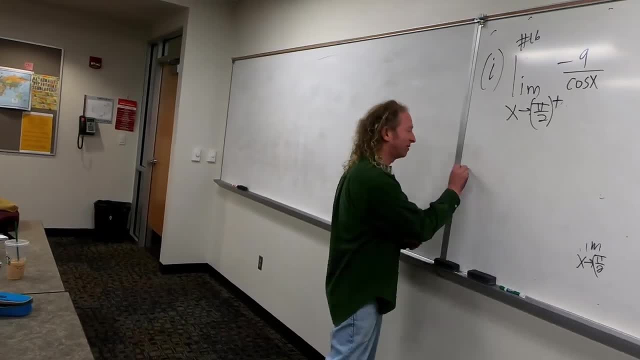 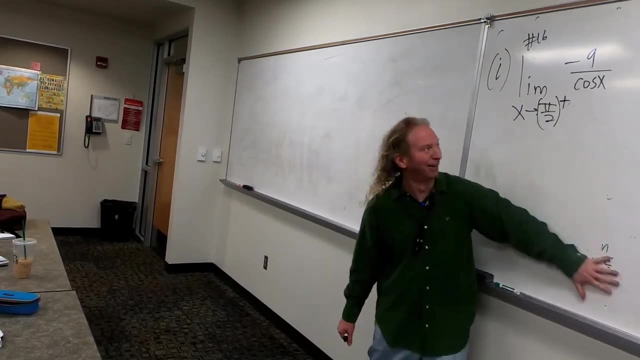 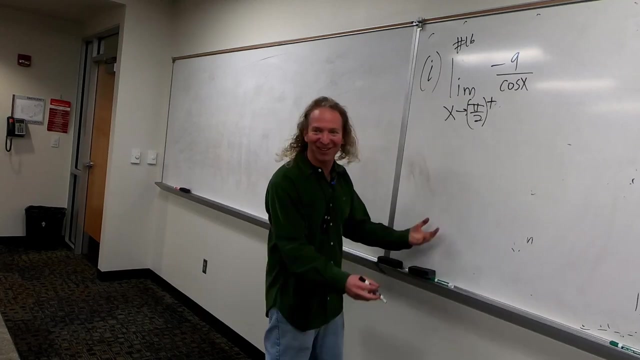 Negative infinity. Okay, That's one possible answer. I mean, I don't know. I don't know, It's wrong. Oh, It's positive infinity. You all figured it out Really. Oh, it's so good. All right, let's work it out. 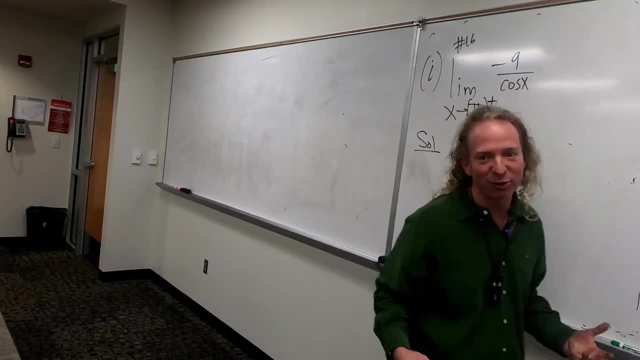 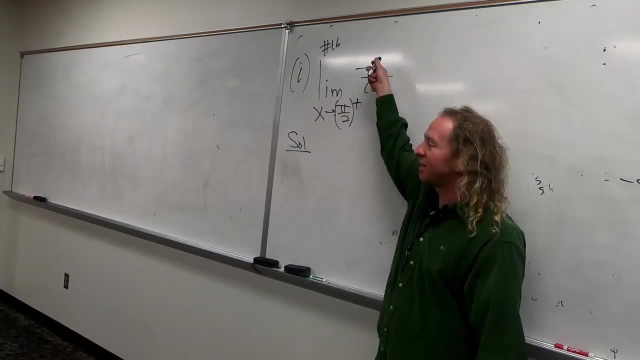 I can't believe you're getting this. This is like A massive source of confusion. This is probably like the hardest problem in the entire section. It's like a calculus killer. So let's see Up top. it's a negative number. 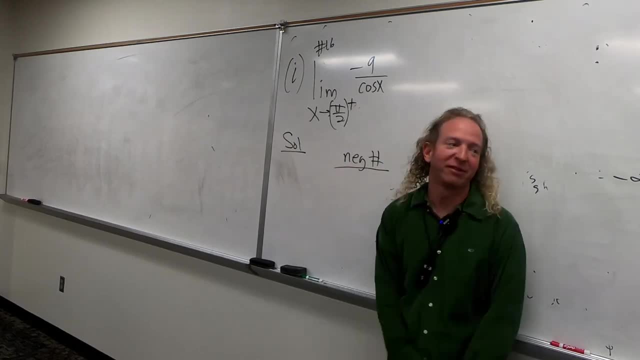 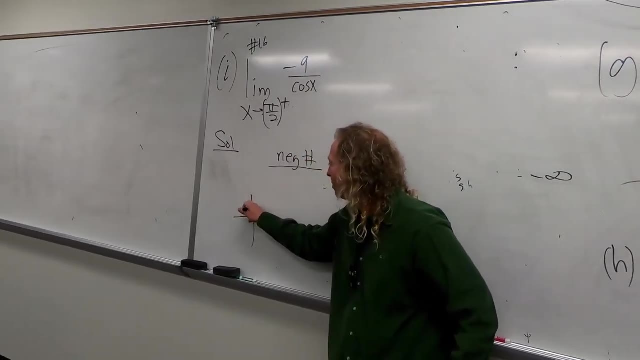 So negative number On the bottom. I've got to think about the graph of cosine, Let's see. So I've got to draw it. So cosine of zero is one, So it does this, So this is pi over two. We're approaching from the right. 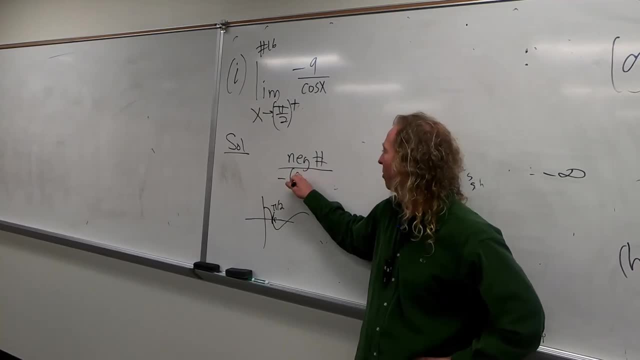 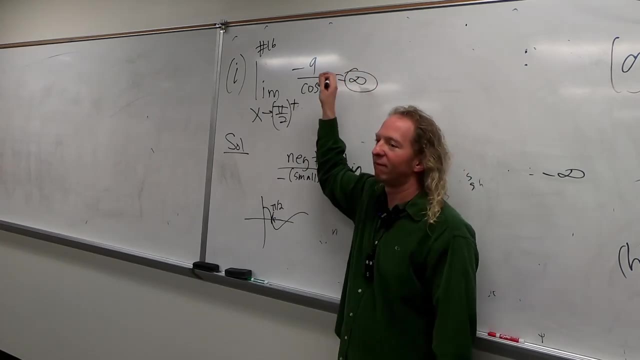 Ah, So it's negative and it's super small. So it's negative and small So that means it's big, So that means it's infinity. Yeah, yeah, This here. Yeah, yeah, I did it really fast, Okay, so check it out. 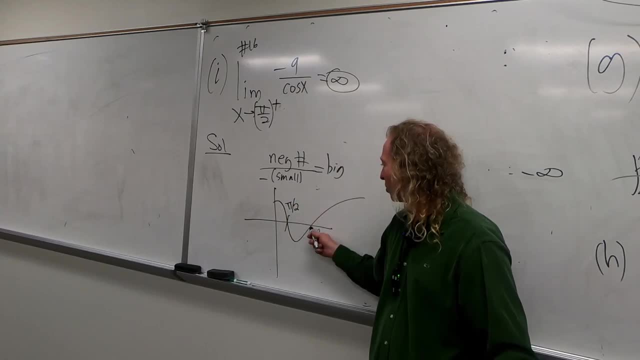 So here's pi over two, So we're approaching pi over two from the right. So the y values are negative down here, right, Yeah, see how it's negative here, Yeah. And then so it's negative and small Negative, negative. 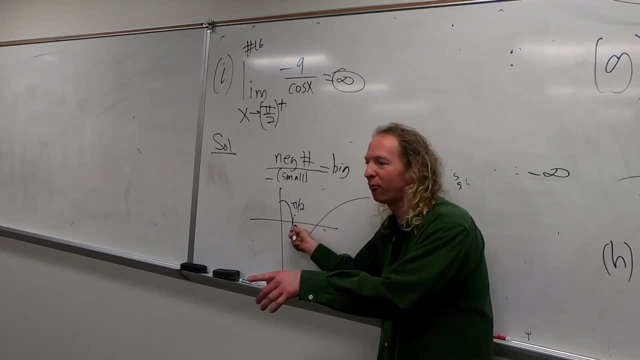 It's positive, so it's big. If it was over here, it'd be positive, right? Yeah, right before, like Ethan was asking, It's tough, right, It's tough, It's tough. You think you got this. 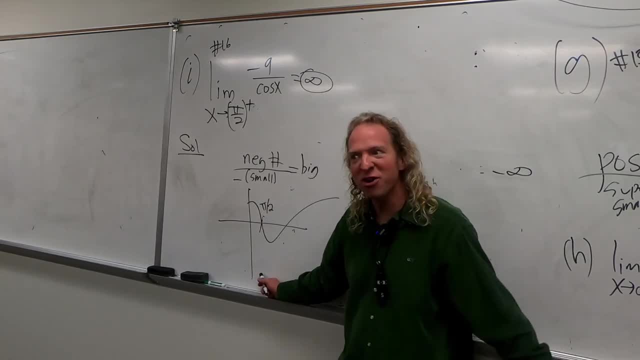 You want to do another one. It's up to you. Let's do another one. Another one Good A, B, C, D, E, F, G, H, I, J. I really want to keep seeing you right. 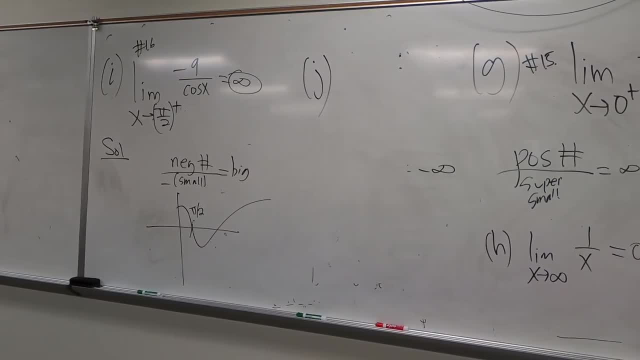 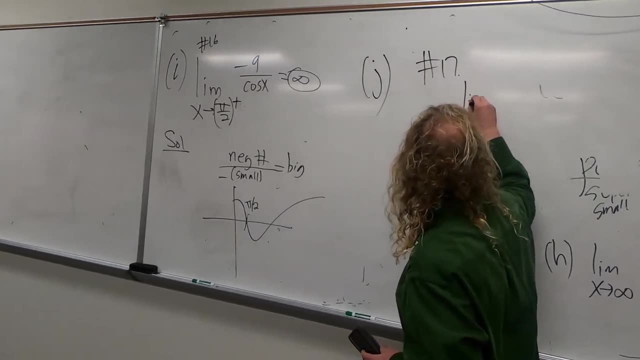 L M N O P or K L M N O P. Whoa, What's going on here? We should do 17.. It looks really good. I'm almost at the time of the hardest possible problem. 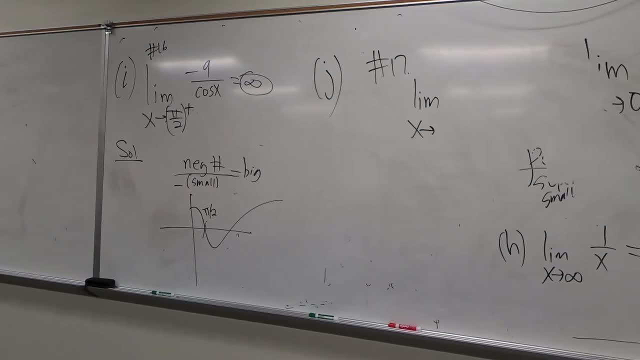 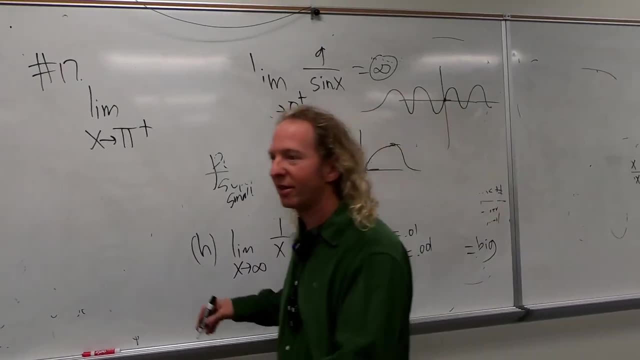 This is ridiculous. I hadn't even looked at the homework until now, actually, So I assigned it. If it's bad, I can always delete it. See, that's the thing. It's a nice thing about homework- online homework. 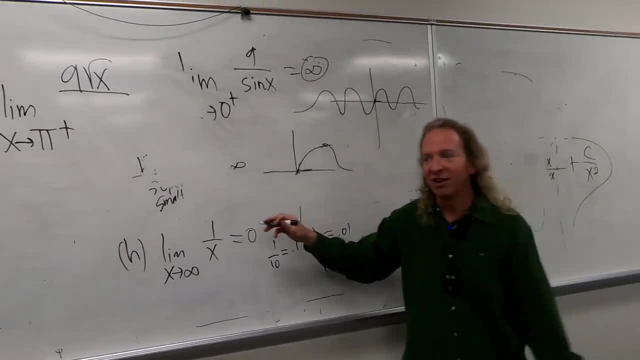 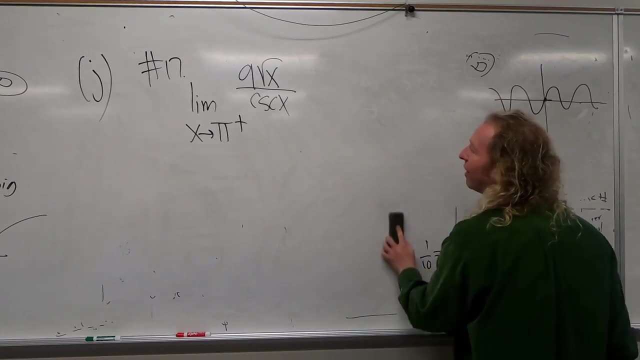 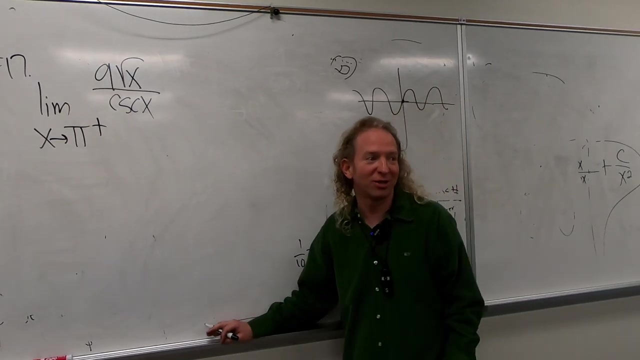 It's really easy to unassign it. I just hit a button and it's gone. Cossy context- Oh, this is kind of interesting. Maybe I should do this one for you, Because I mean, or do you want to try it? 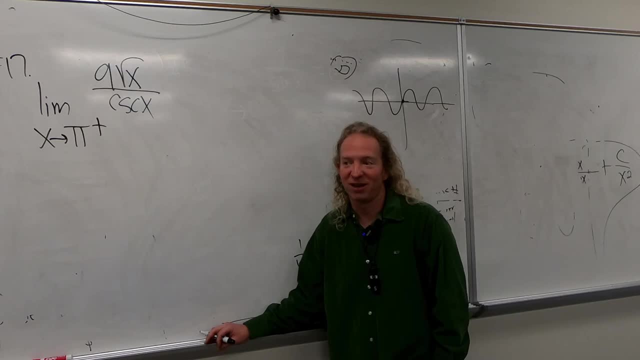 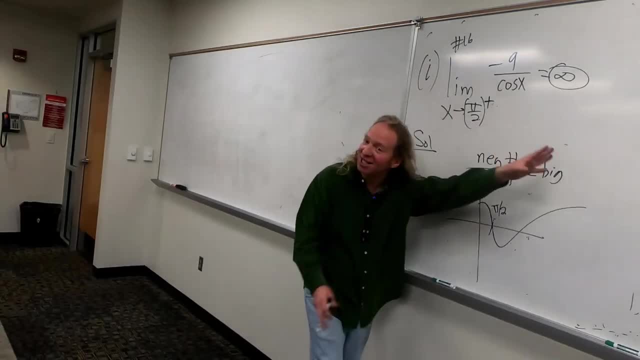 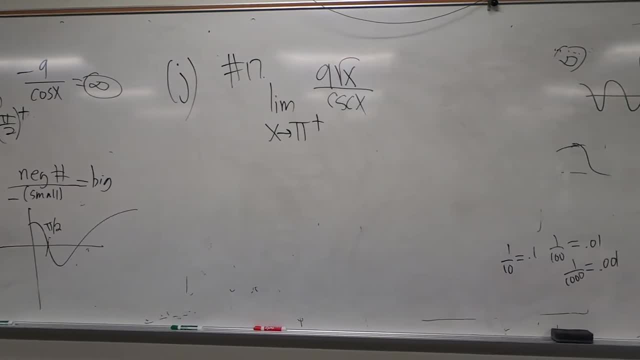 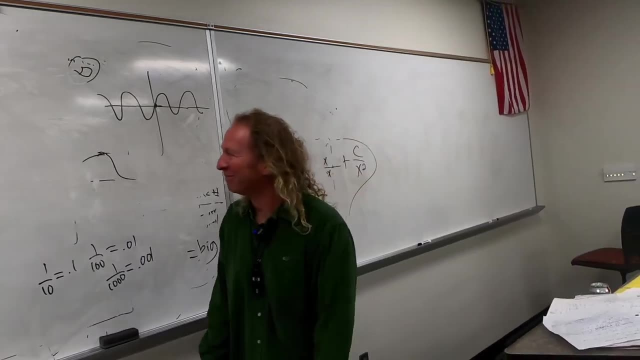 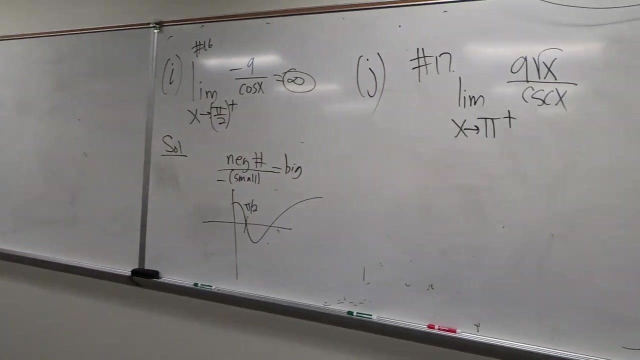 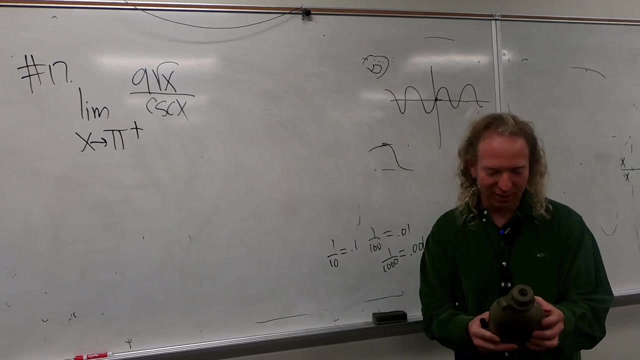 I'll try not to. I wouldn't intentionally do it. I'll put it out. Hey, did someone leave a canteen here? Wow, For water only. do not apply canteen to open flame or burner plates. I'm going to leave it. 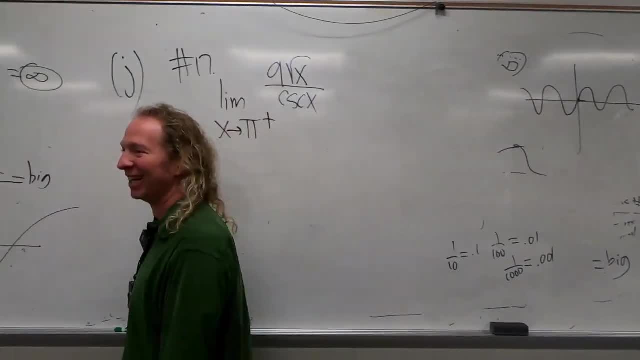 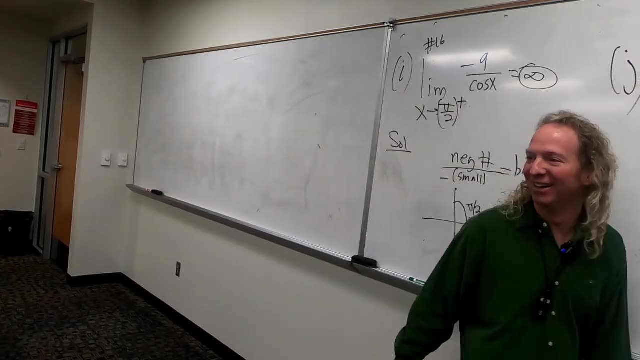 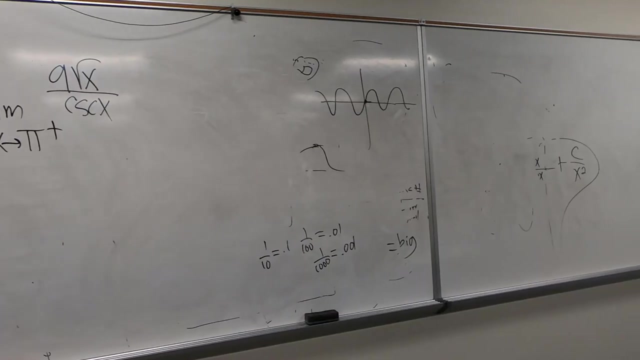 Must have been someone from my other class. It's hardcore. It's like Go live in the woods. Did you get it, Logan? You did. I don't want to say it. What did you get? No, it's wrong. 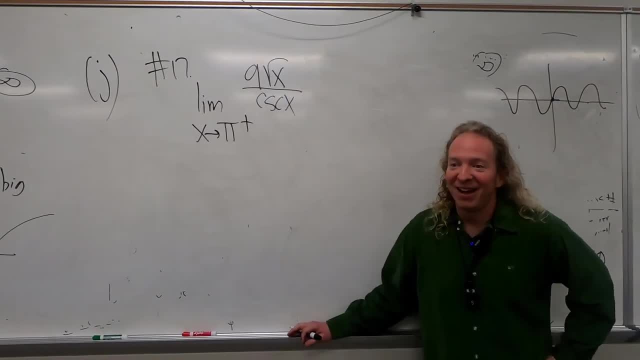 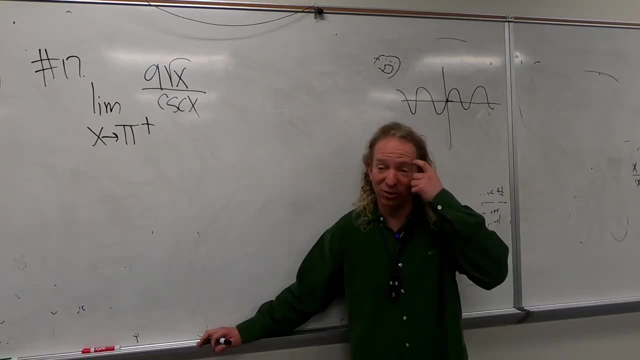 It's wrong. Yeah, see, that's why I was like: Did you get it, Judah? Did you get what Logan got? Huh, Jordan, That's a point right? No, Anyone, Anyone get the answer. 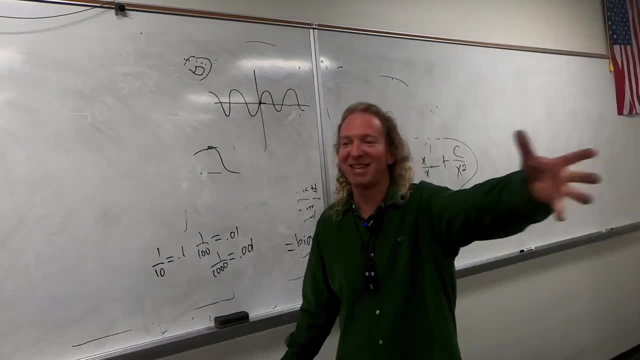 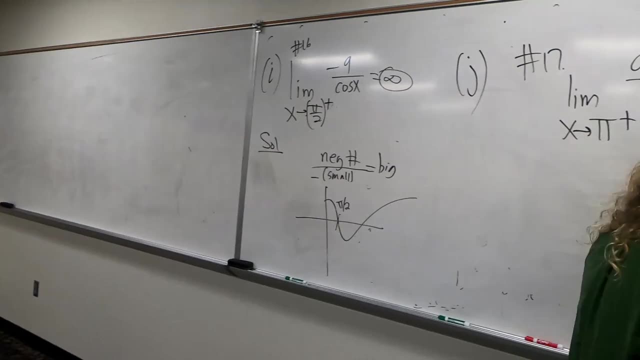 Anyone. What did you get? It's zero, It's zero, It's zero. Oh, We thought about it, but then we were like, no, No, it is zero. Good Judah, Good Yeah. So this is evil, because you actually do get an answer in this case. 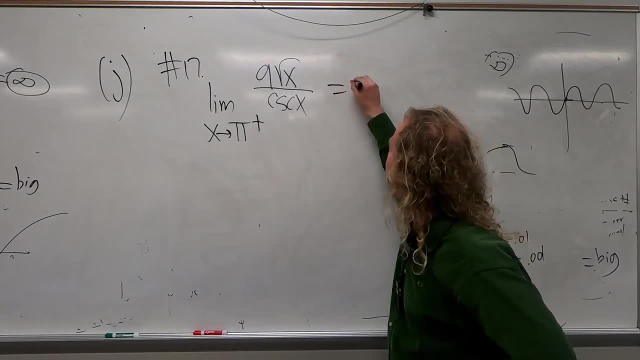 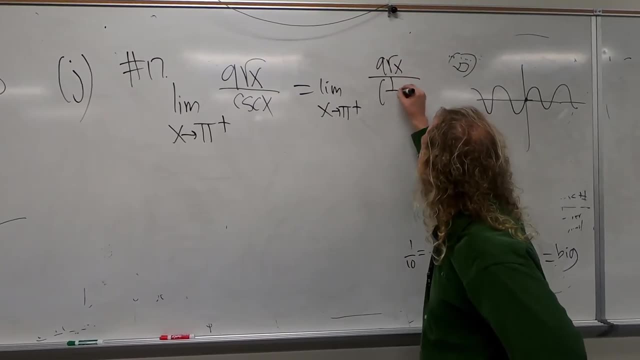 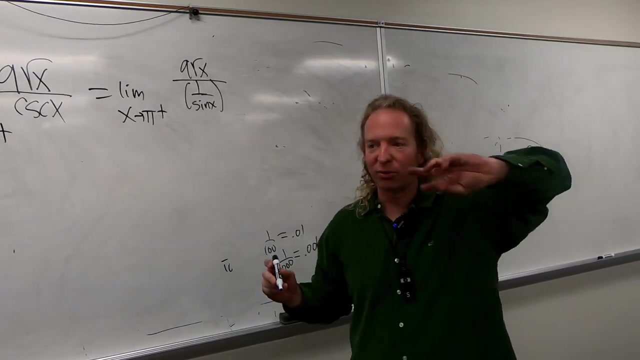 Watch. So cosecant is one over sine right. You can actually show the work in this case, which is kind of evil because the question says: don't show work. And then when you divide, When you divide by one over sine, you really multiply by the reciprocal. 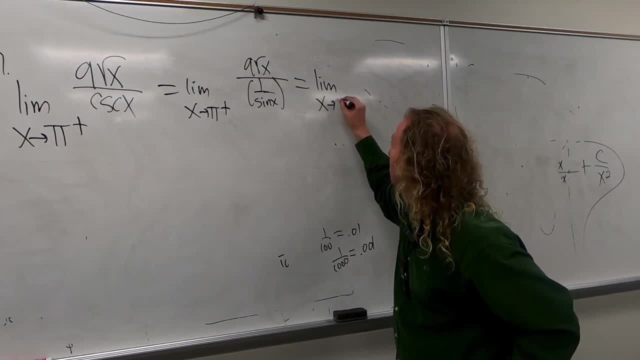 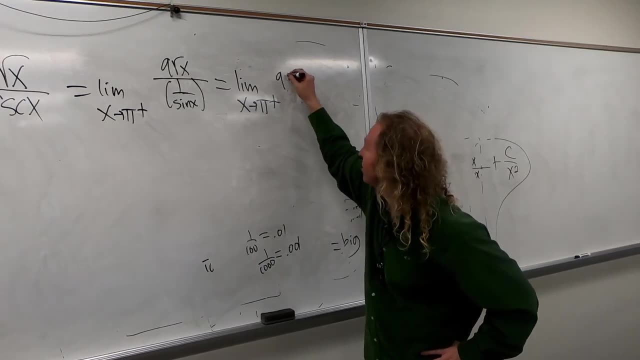 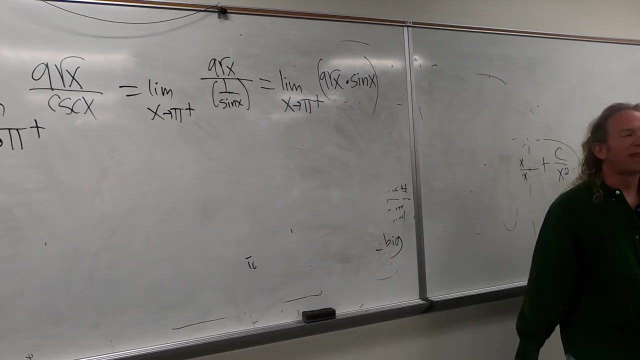 Yeah. So if I give you a question like this on your test, it would say: show work right. There is one like this, I think, with cotangent in one of the previous sections. So this is nine square root of x times sine x. 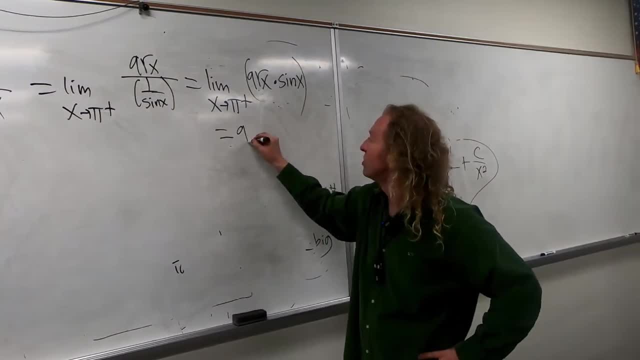 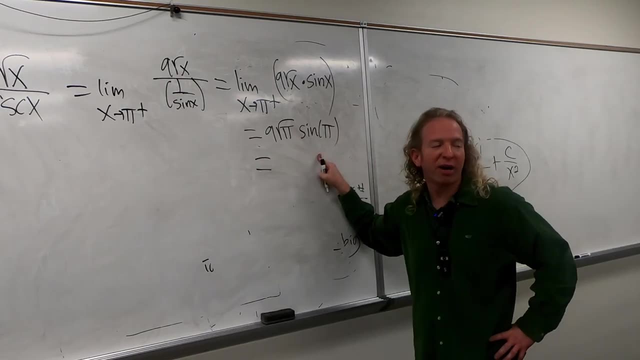 And then now you can plug in the pi so you get nine square root of pi. Who cares about the one-sidedness of it? It's ridiculous. It's like they put it in there on purpose, just to be tricky. Sine of pi is zero right. 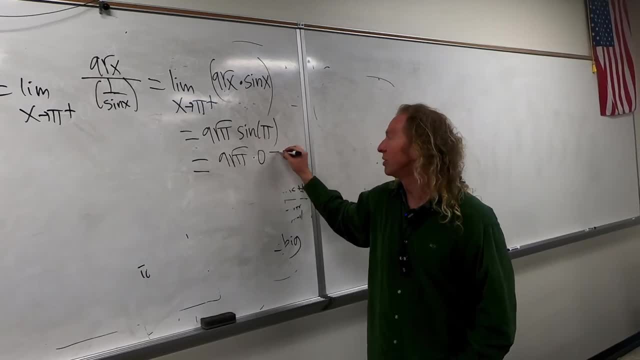 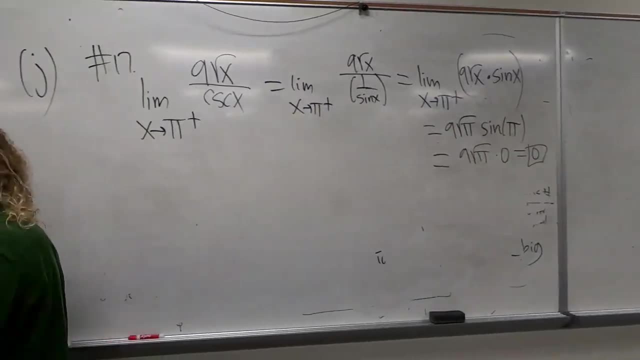 This is nine square root of pi times zero. so you get zero. So kind of a nice problem. but again, I will not purposely try to put this mixed in. I haven't. It's happened before in the past like a typo. 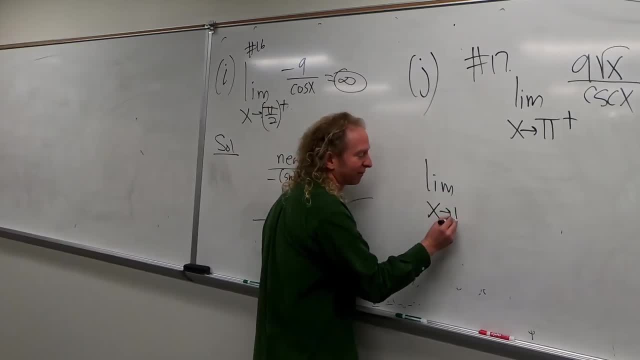 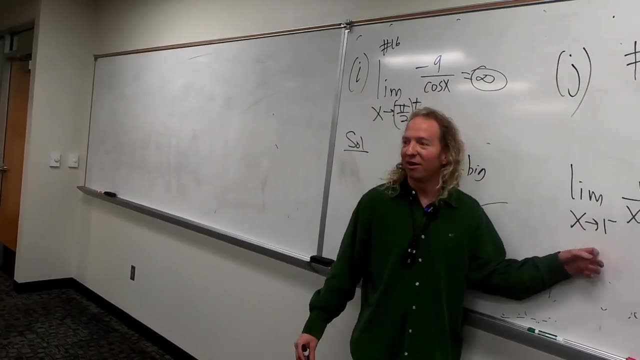 Like accidentally one semester. I did this right because I was in a hurry, because you know, I just wanted to make the test and do something else, You know And then so you just plug in the one Right. But people were pretty like oh, infinity. 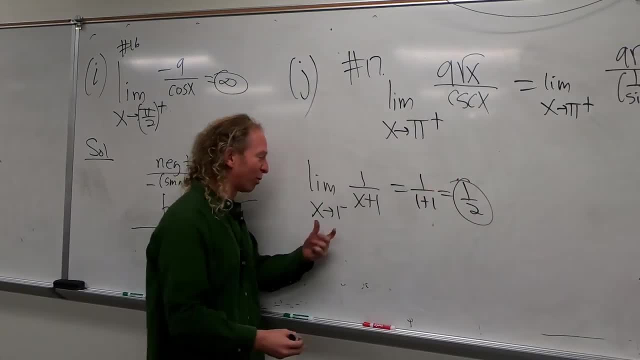 You're like no, You're like no, And I was like, oh, it's a typo. I'm like, oh, they're smart, right. So I just like a few people got it wrong. That's kind of evil, though, right. 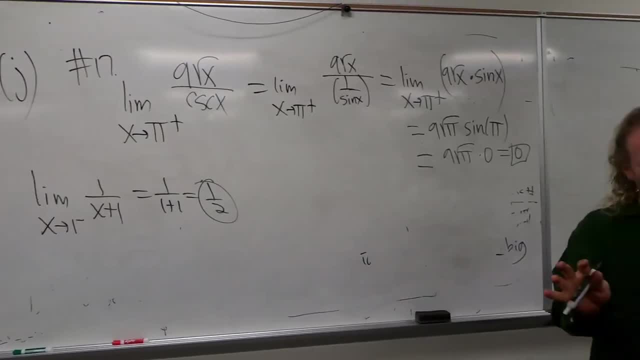 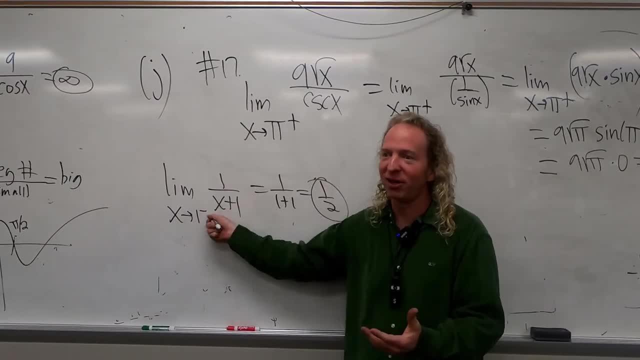 you plug it in and you plug it in, and you plug it in and you plug it in. It's kind of evil, though right, Because you get so used to the infinity and negative infinity then you forget you can actually plug it in, right? 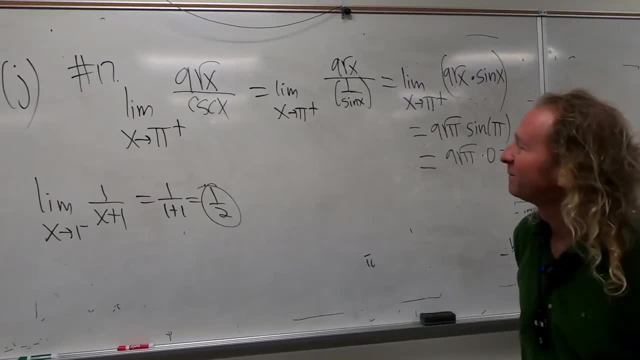 Yeah, So for number 17,. I did it using the co-seeking graph. Like, if you approach pi in the co-seeking graph it's going to be infinity, positive infinity. so I think, over positive infinity it's zero technically. 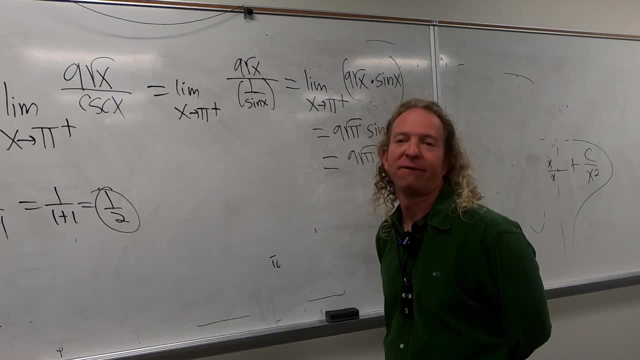 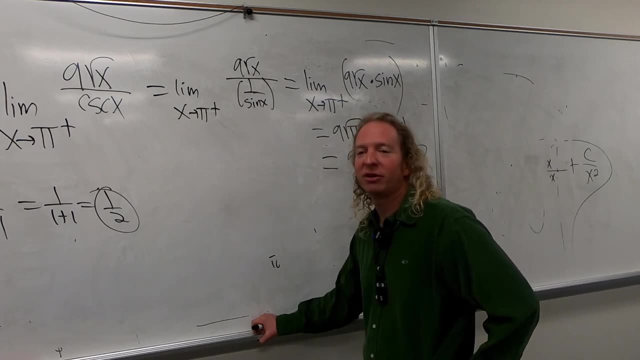 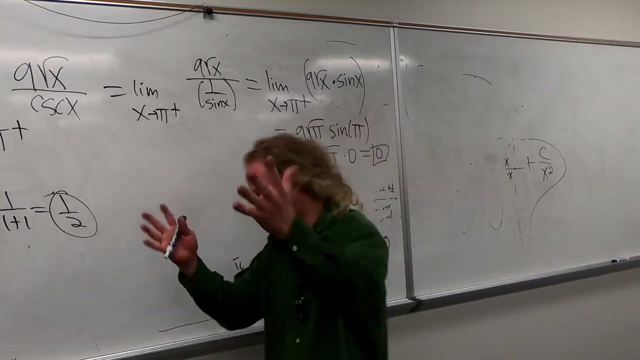 All right, Very good, But you still get. That's beautiful. Yeah, That's great, That's amazing. No, It's really deep. No one does that. That's like Analytically, though you do have to show work. 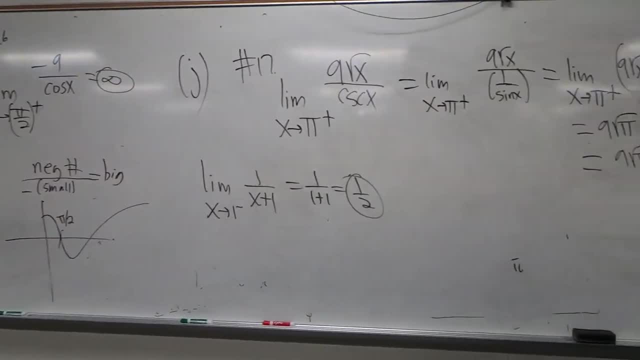 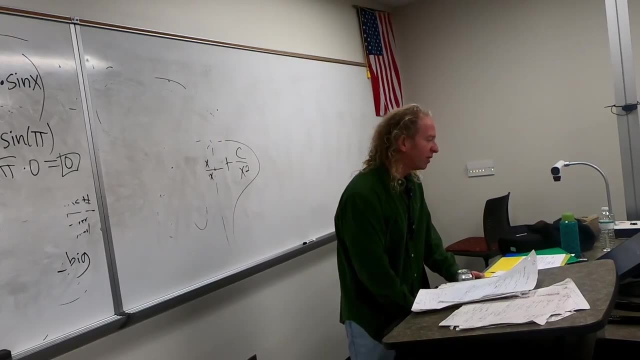 That's the only thing. Yeah, like you have to show some work, Like, yeah, All right, let's talk about something else: Vertical asymptotes. I think you've seen these before, So let's do a couple vertical asymptotes. 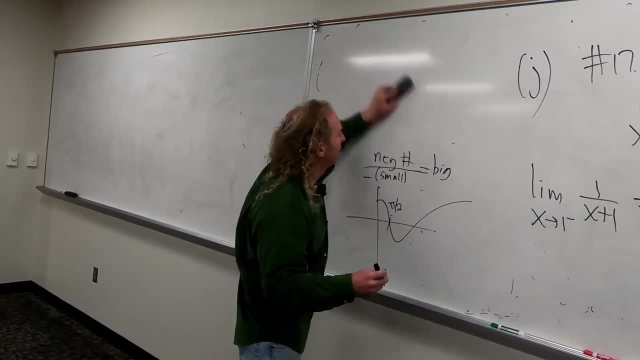 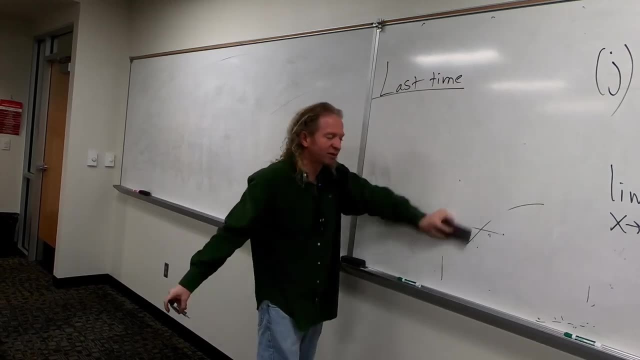 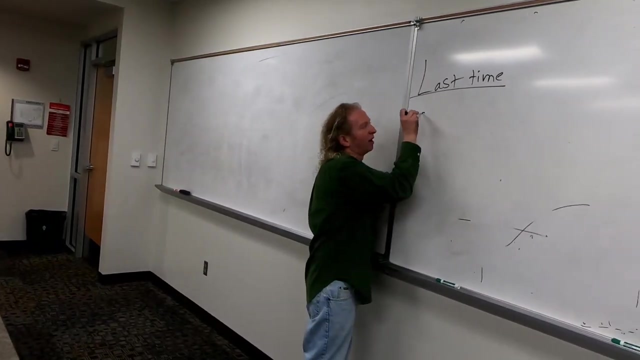 So, yeah, let's do it. So last time we had this formula involving sine and cosine, which was very useful. We're just going to do it again today. Why not? It's probably on your test. Sine x is equal to 0.. 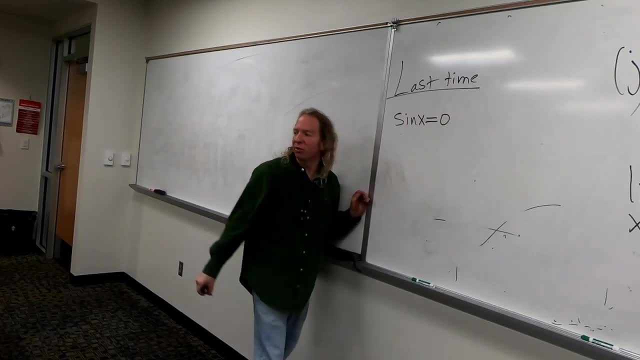 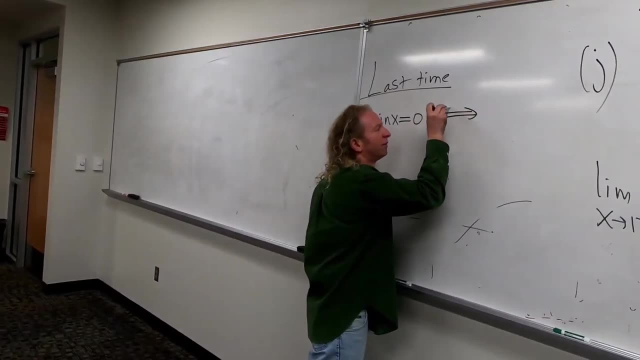 Remember this with the k pi. I'm going to do it again. This is the same thing as saying that x is equal to a multiple of pi. That means it's k pi. So we're just going to do it again today. We're just going to do it again today. 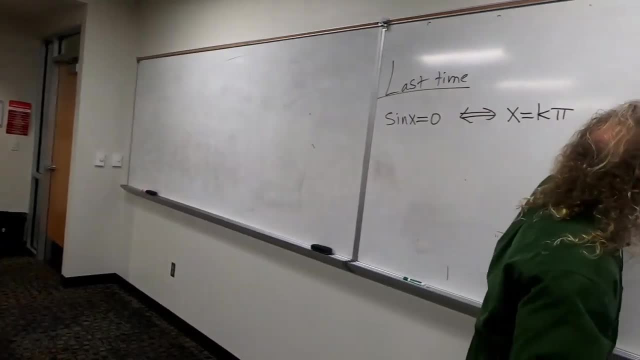 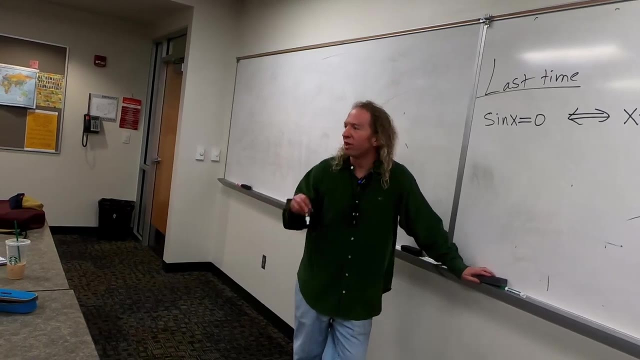 We're just going to do it again today, And there was something we had to say about k. Do you all remember what it was? It's an integer. So you can say where k is an integer. Did I show you the other way of doing it, the fast way? 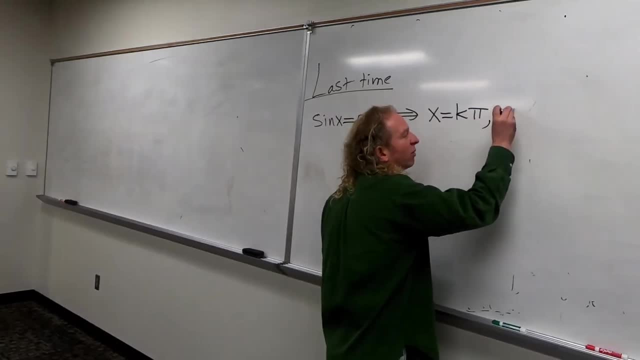 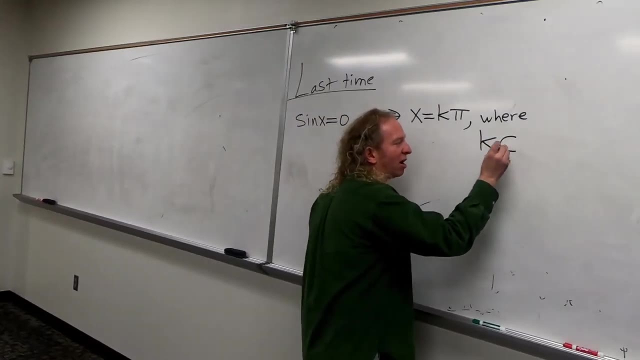 Remember that. So I'm going to do this instead. where k- and then we use this symbol here- belongs to, this means belongs to yep. and then the z. Remember the z like this, the fancy z Z. 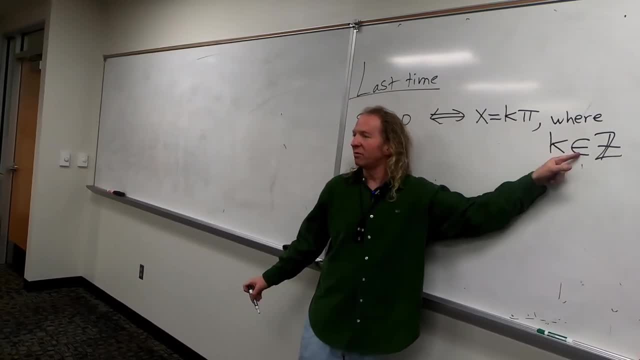 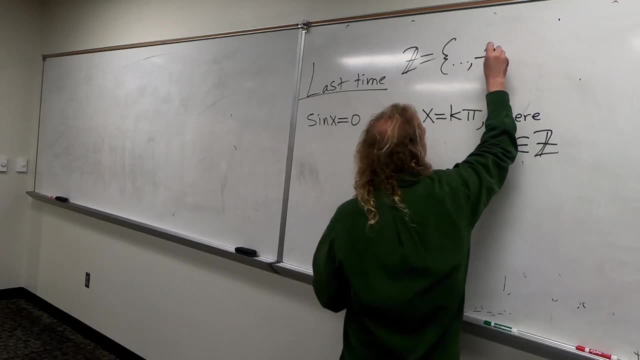 So k is inside this set, k is an element of this set. What is this? Z is the set of all integers. This is worldwide language, right? Math people say. I mean some people will say math is like another language. 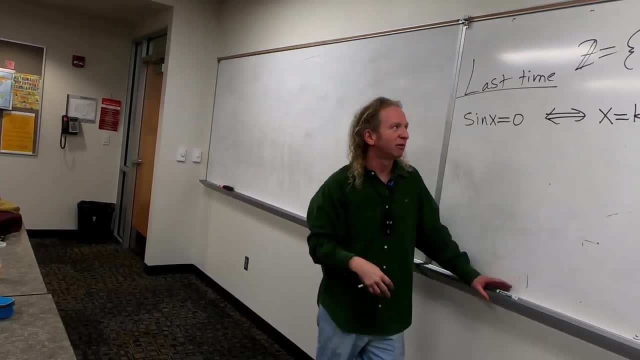 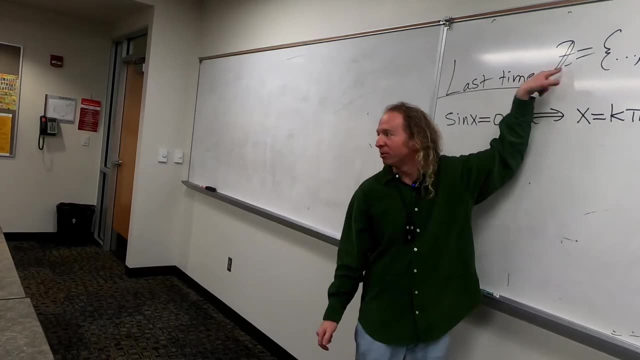 It is. it is except languages I think are harder Like. it's probably harder to learn like Japanese right than it is to learn this, because there's more letters and they form words. This is just one symbol. 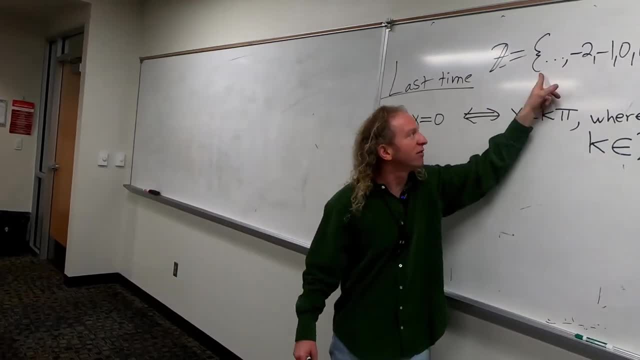 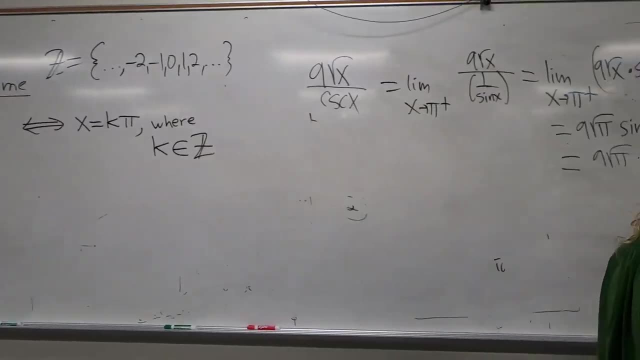 So this is the set of integers. So this means k is one of these numbers, right? So the word they use, z, because I think in German the word for numbers is salen. I think That's what it says in Wikipedia, so I don't speak German. 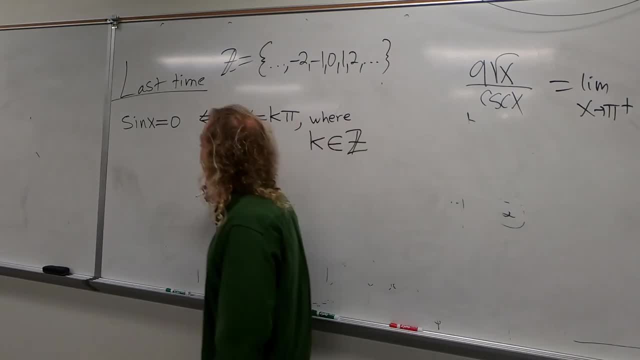 I just know that. so and a bad word which I can't say. So, and then we have cosine of: does anyone here speak German? Anyone? No, Okay, I was hoping you'd say it the right way, but okay. 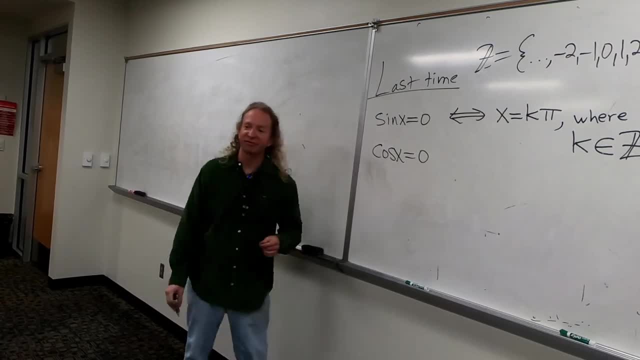 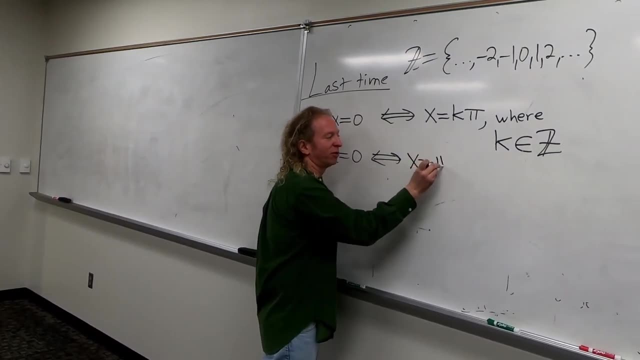 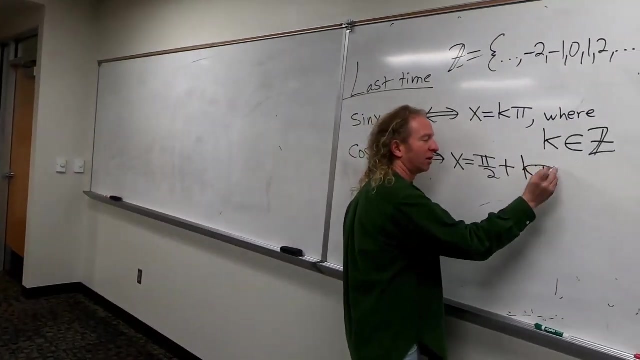 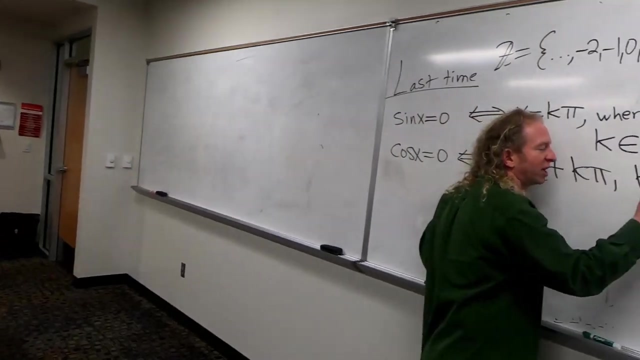 So cosine of x is equal to zero. This is equivalent to saying, you know, x equals pi over two, plus plus k, pi, plus k pi. And again where k is an element in the set of integers. So very, very common notation. 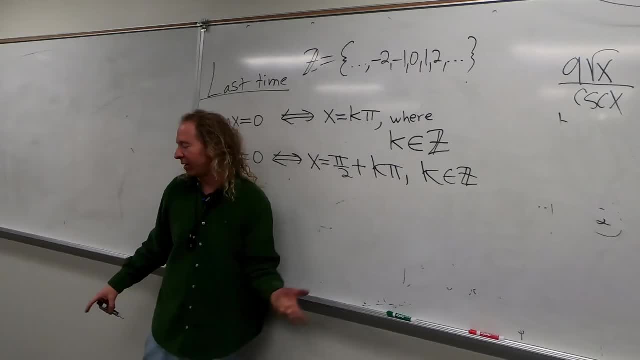 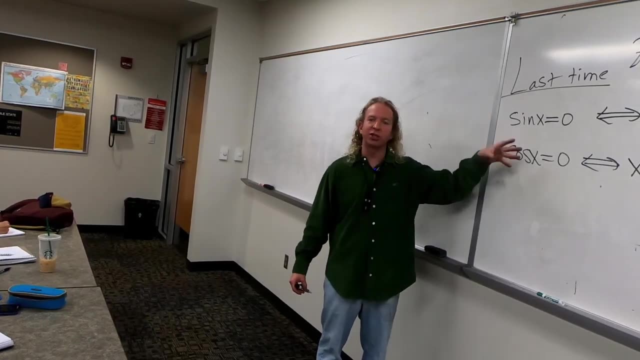 If you're wondering where you learn this, you learn this in like a discrete math class. if you're a computer science major or if you study math as a major, you learn it in like a logic improvement proof class for math majors. 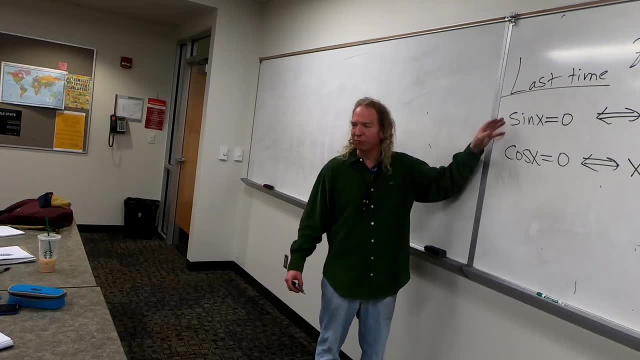 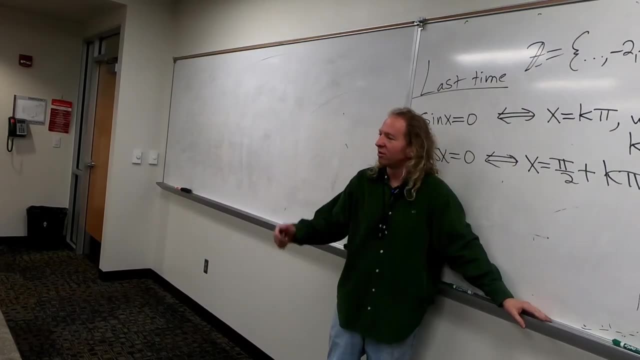 But otherwise you don't really see this right. Maybe you might touch on it in intermediate algebra. Has anyone ever seen this before today, Like before this class? Where have you seen it? Just Just around, Just around In logic-improved books. 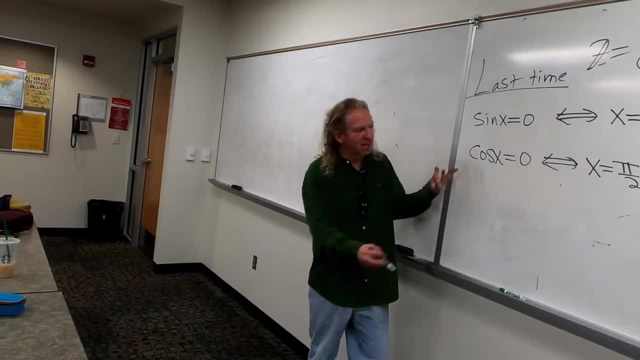 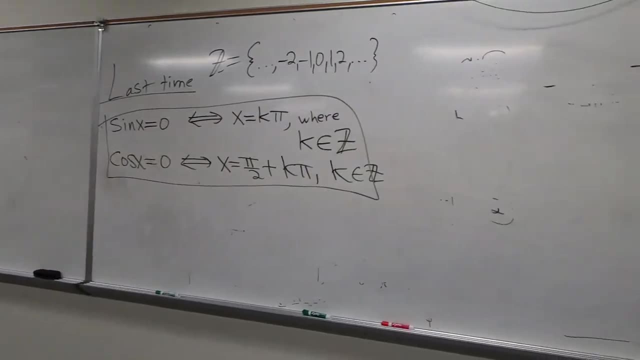 In logic-improved books. Yeah, was there a men's class? Okay, yeah, Mm-hmm. Yeah, it's not something that's typically taught. Most of the classes here, like all these calc classes and stuff, they're typically they're geared towards people. 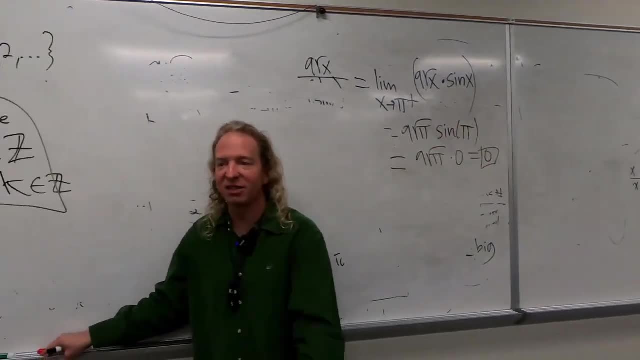 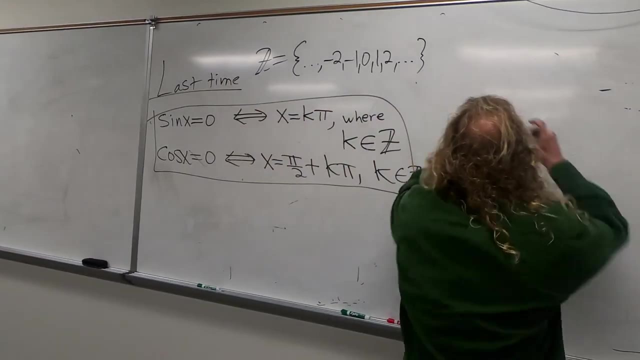 who are going into engineering right, Physics, science, stuff like that. So we do a lot of like a different type of math, more calculus. Okay, So let's find some VAs, Let's do it So find. 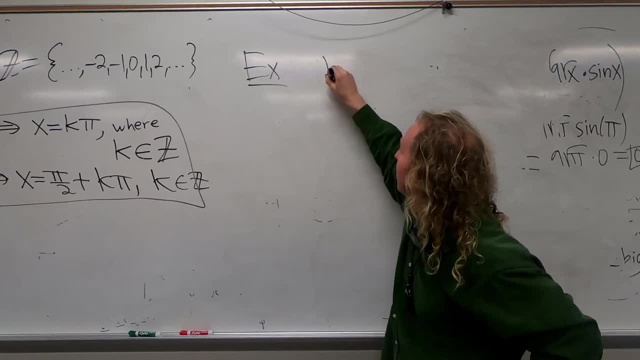 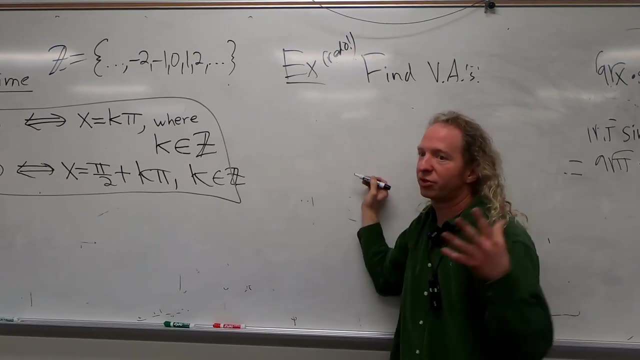 So find, Find some asymptotes, So you'll have this on your test. So find VAs, So redo these examples, right? So find VAs, So redo. Redo the last example too, right, When you're studying for the test. 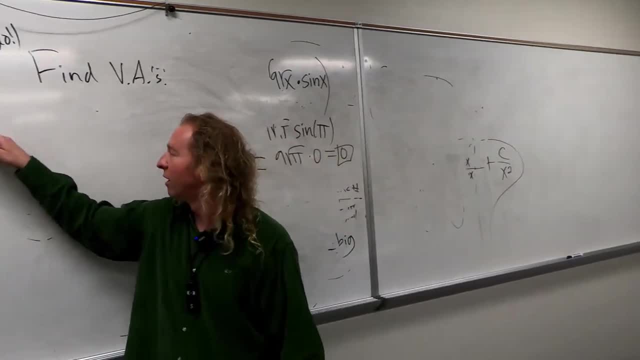 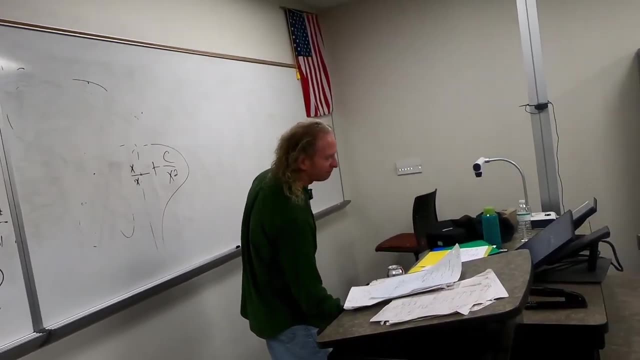 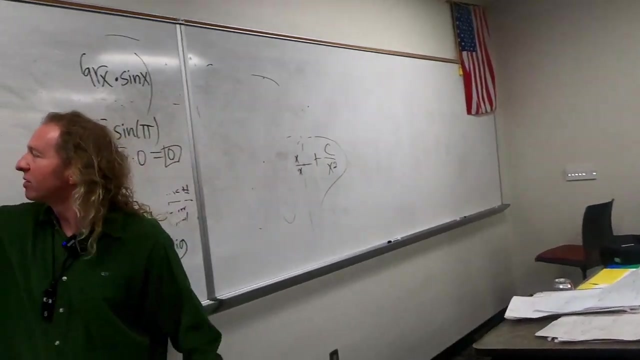 So find VAs, So A. So maybe there's one in the homework that's decent, Like test level. No, those are all weak, Mm-mm. No, Yeah, Or I guess this one number nine. So this is number nine from the homework. 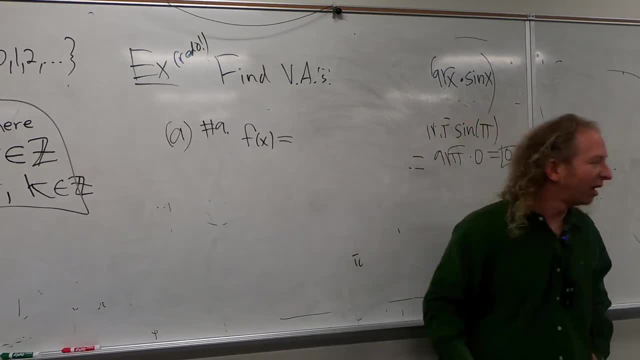 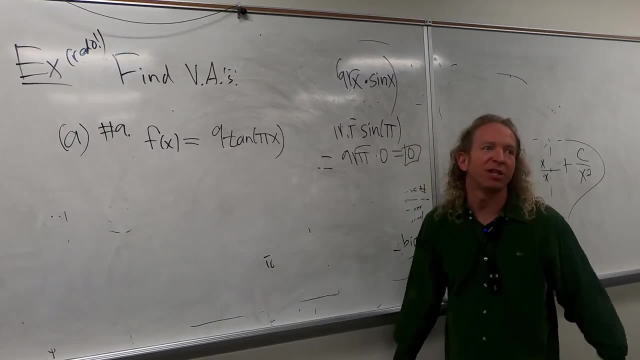 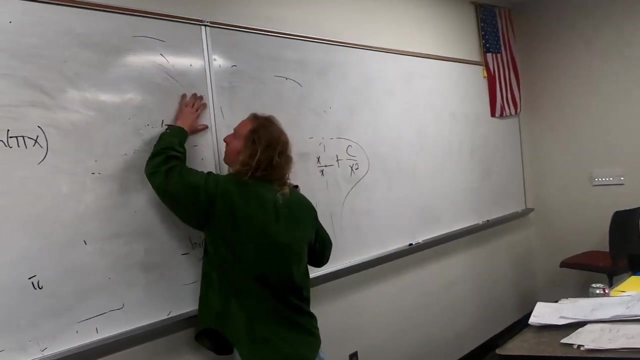 F of X equals This one's okay. Yeah, it's pretty good. It's got a nine there. It makes it look confusing. Tangent of pi X. Tangent of pi X. All right, So when you're looking for VAs, just think about. 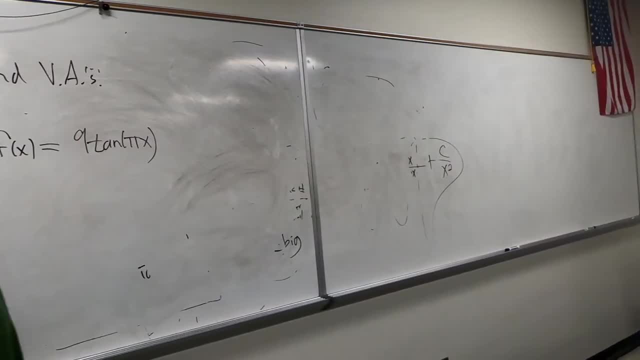 Whenever it's a trig function, think about what's on the bottom. You don't have to write it down, but you can. Yeah, It's not question. nine, It's eight. Oh it's eight. Yeah, eight, Are you sure? 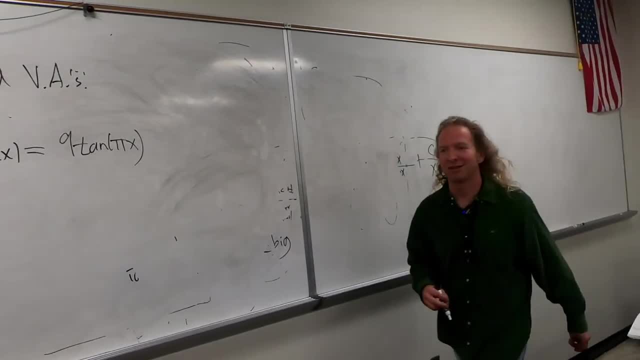 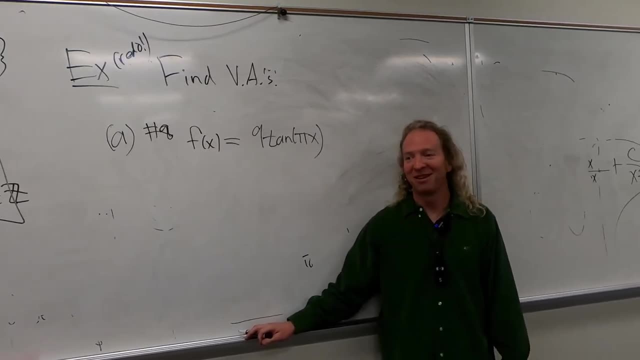 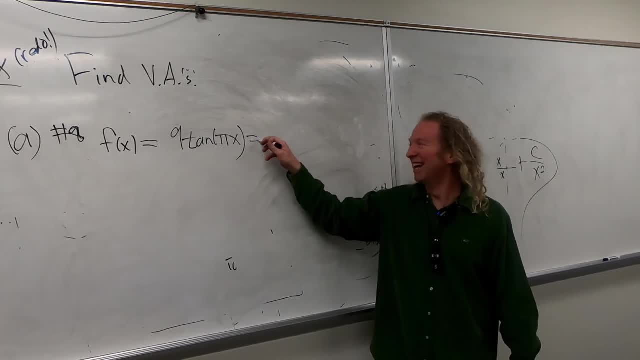 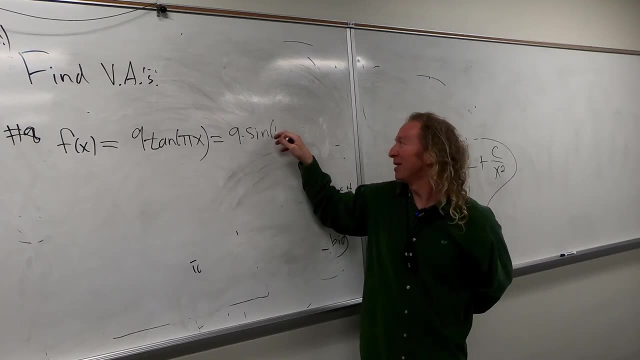 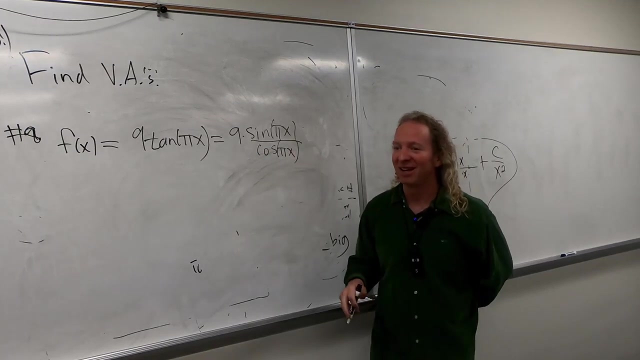 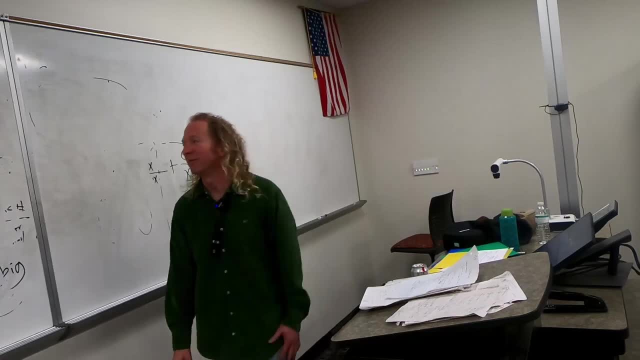 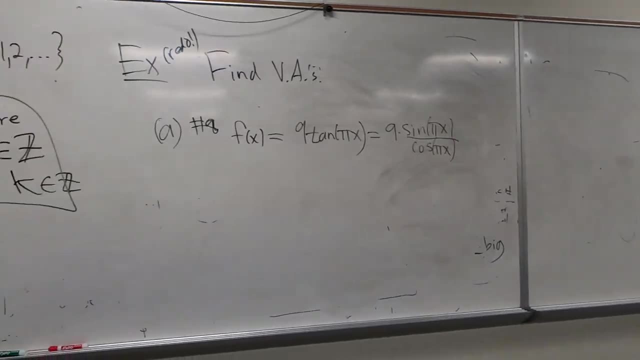 A point. It's good. It's good, It's your life. It doesn't affect me, right? Doesn't? Yeah? No, No, No, No effect on my life, right, It won't matter in 30 years. 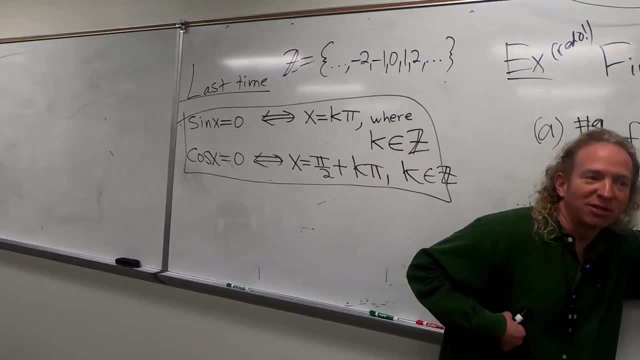 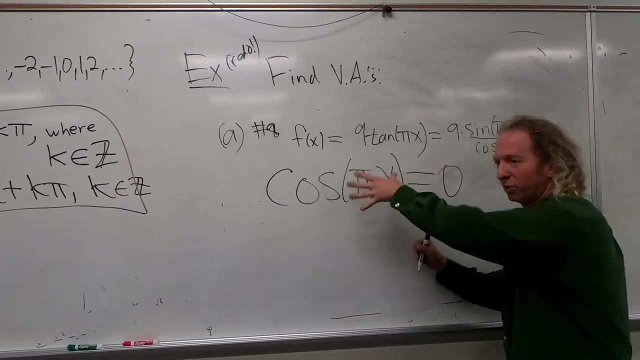 Okay, This is a fraction, So we want to know when the bottom is zero. right, That's what it has a VA, So you take the bottom and set it equal to zero, All right, You want to know when. That's what you want to know. 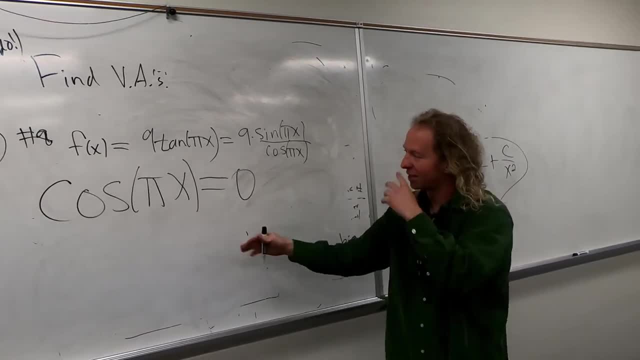 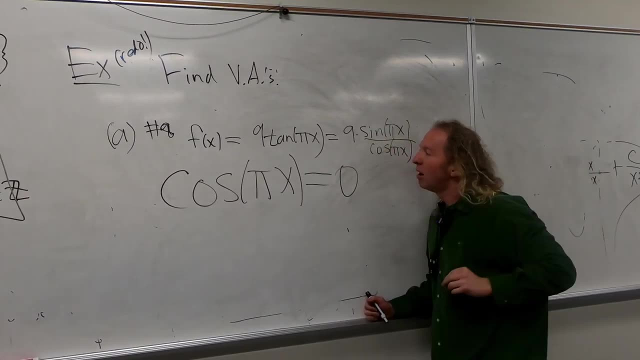 You can show where You can skip this step right. You can go straight to the next step. So cosine of pi X is equal to zero. So let's see What happened here. What happened to the nine? What happened to the sine? 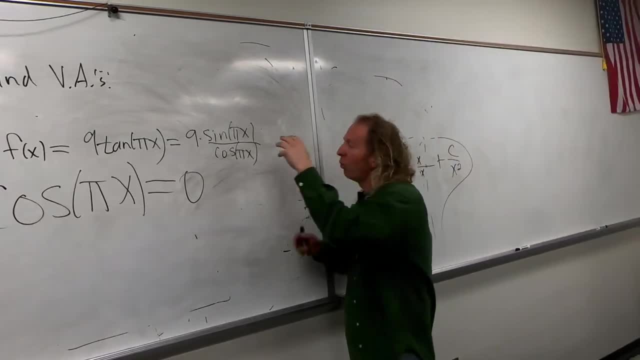 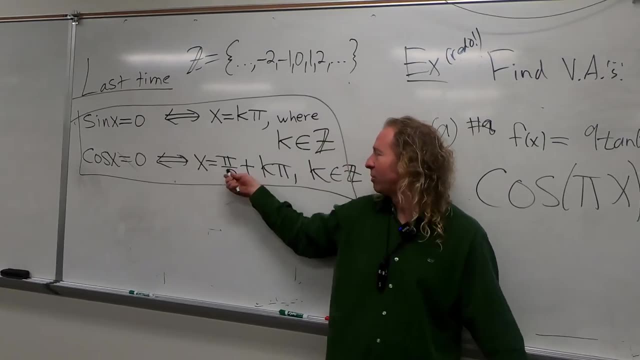 Well, it's a logical move. It's like we're thinking: when is this undefined? It's undefined when the bottom is zero. So cosine of X equals zero when X is equal to pi over 2 plus kpi. right? So you just take this right. 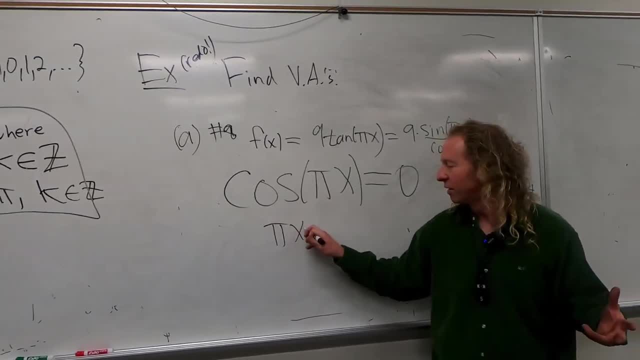 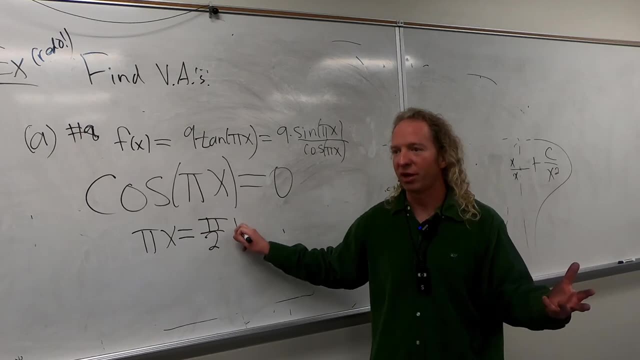 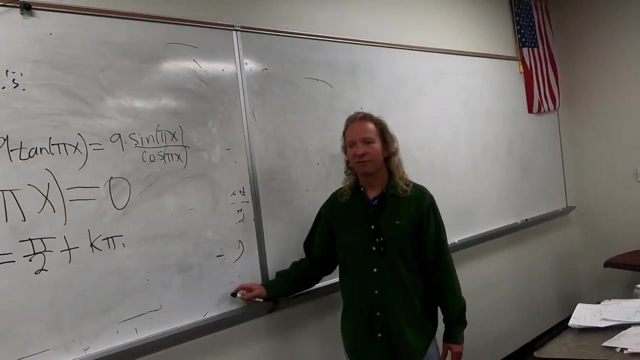 This whole thing right? So pi X equals pi over 2 plus kpi. Any questions on that step? You want to see how we did that. So when I'm taking the test- because I have to take the test too, because I have to- 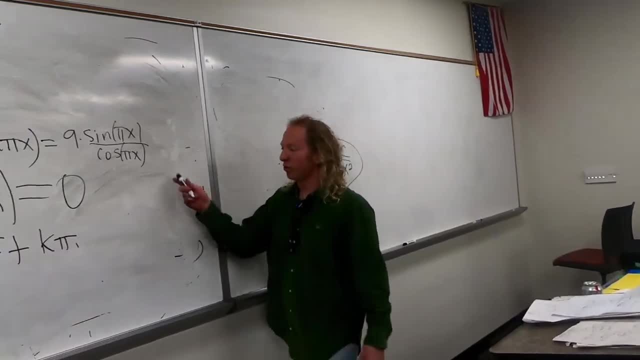 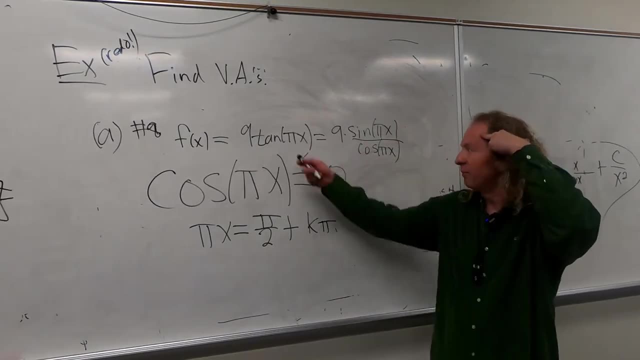 grade it. I need the answers, right. I don't do any of this. No, Why Right? I just say: oh okay, Tangent is sine over cosine, Oh, cosine's on the bottom Right. So you can skip all of this. 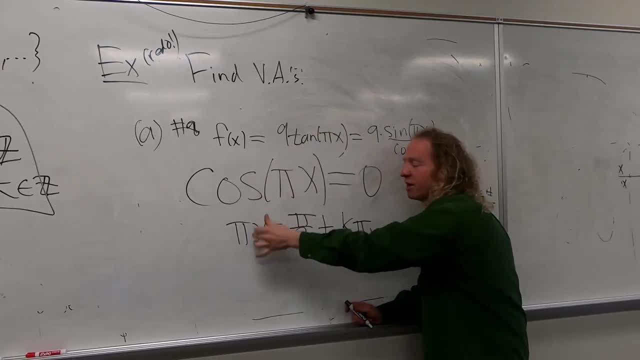 Just think about what's on the bottom. Oh, cosine's on the bottom. So just take this and set it equal to that. If sine's on the bottom, you just set it equal to kpi. You don't have to show all this work, right. 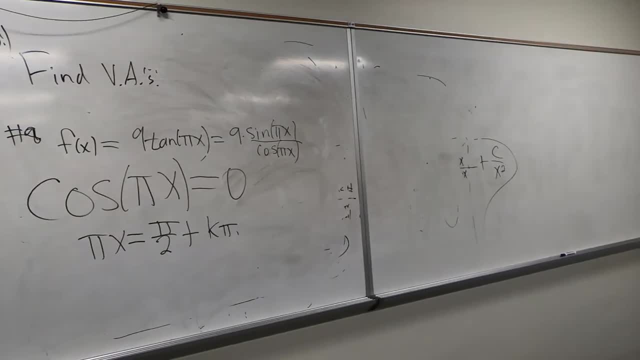 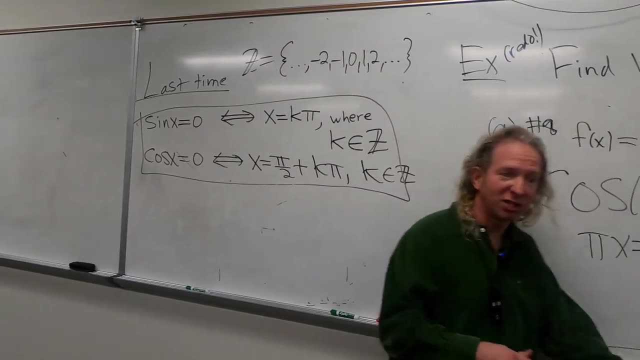 How do, Yeah, How do we solve? How do we solve for X? What do we multiply by, or divide by? Divide by pi. Divide by pi. So it might be easier to multiply by the reciprocal of pi. It's just a little bit easier to show the work. 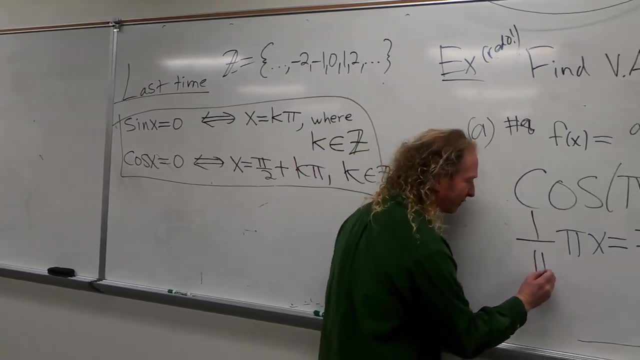 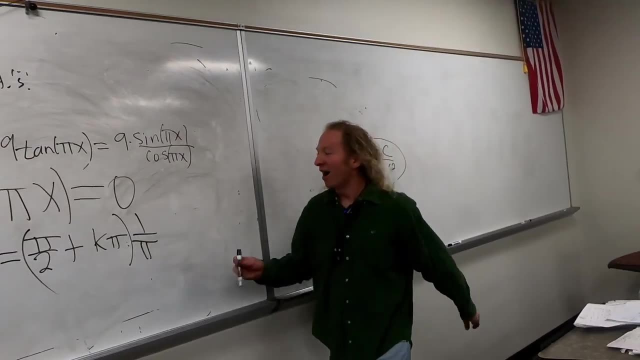 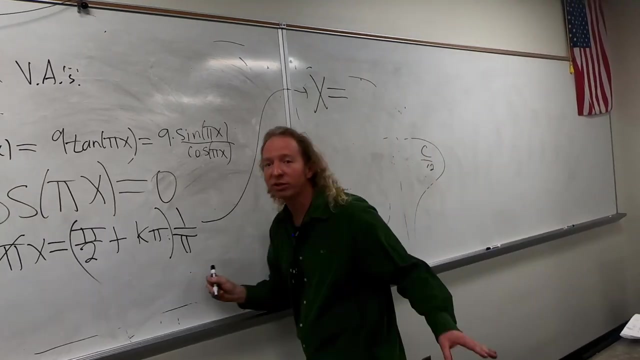 So I'm going to multiply by 1 over pi, So 1 over pi times 1 over pi. Okay, I just thought of something These cancel. So this is equal to X equals. right, X equals. It's really important to write the X because it's a line okay. 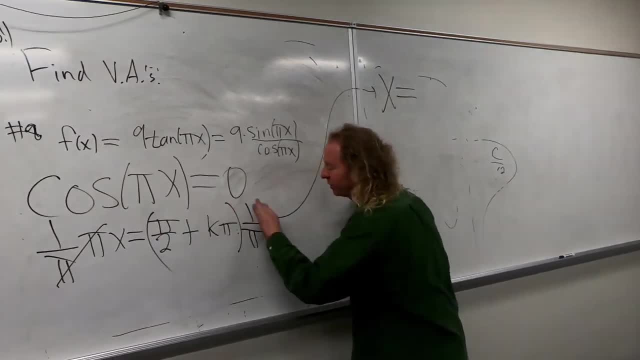 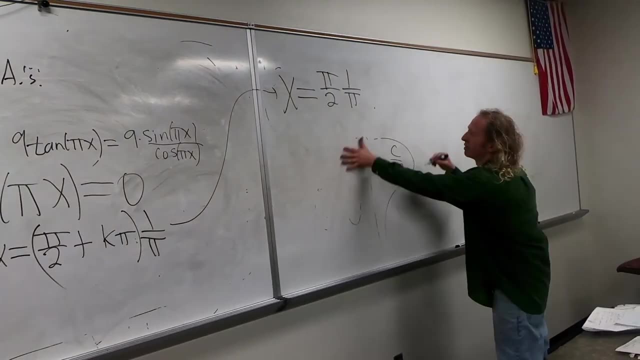 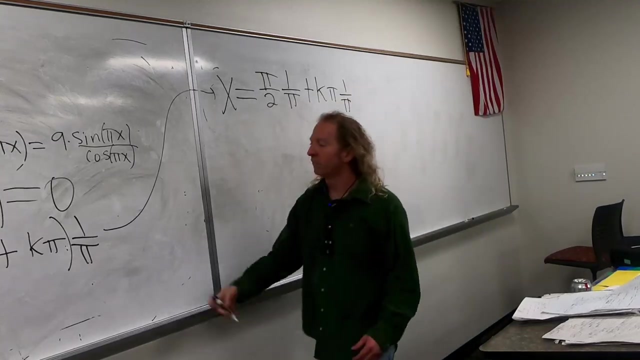 It's a vertical asymptote. I'm going to show every step: Pi over 2 times 1 over pi. So pi over 2 times 1 over pi, plus kpi times 1 over pi. Right, You can skip steps. 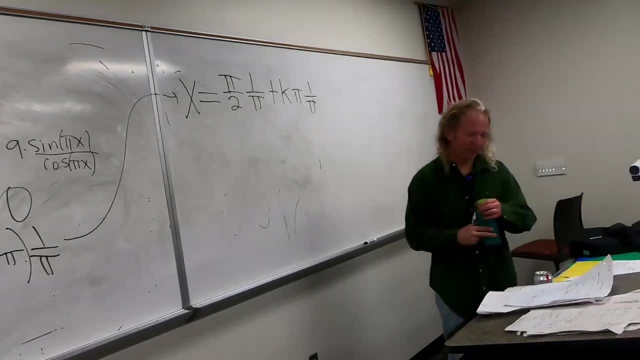 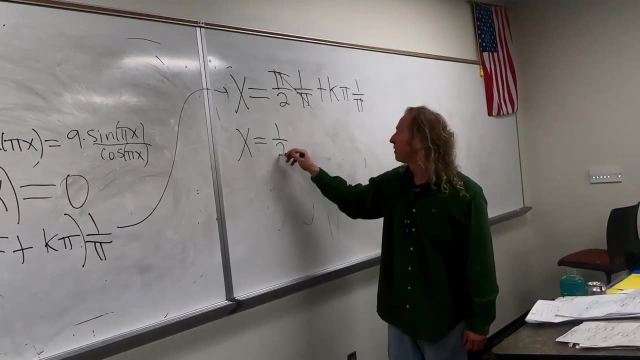 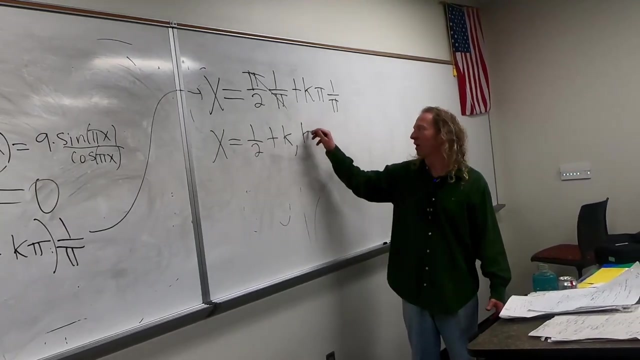 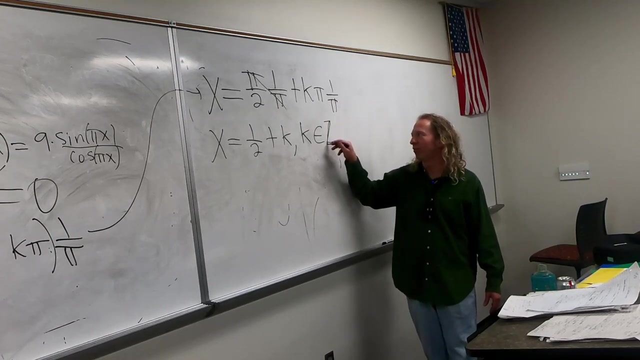 I don't like to. It's easy to mess up And these cancel. So we get X equals 1 half Plus k, And then we just have to say that last thing right. It's really important Where k is an element in the set of integers. 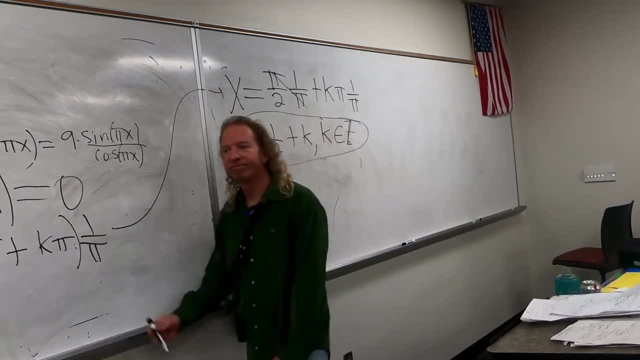 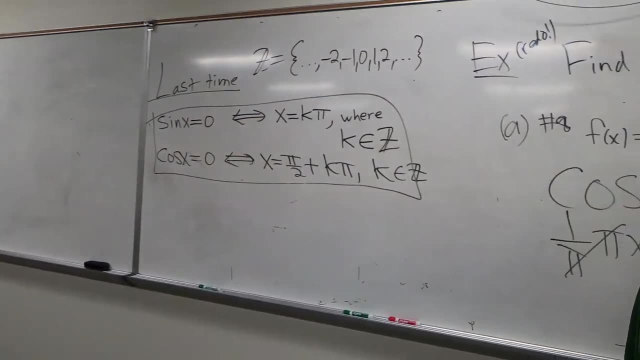 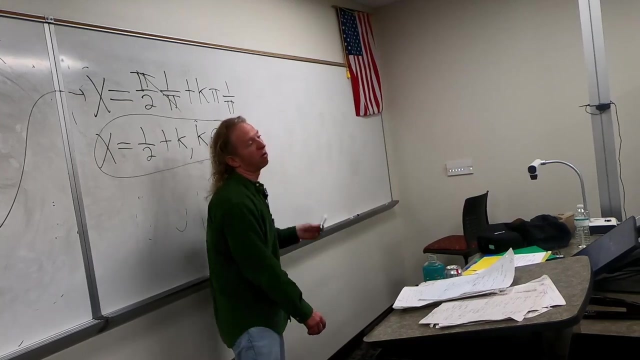 That's it. That's it, Hey, All right. Yes, Would you like to put that in the homework? Yeah, The homework actually has. Yeah, They want n, though. Oh, you mean the k part? No, No. 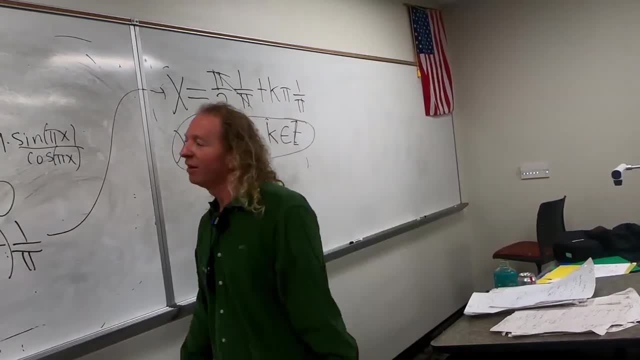 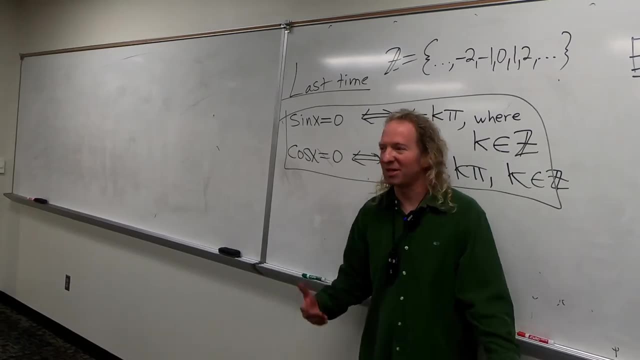 And they tell you to use n. I think. Good question, Mm-hmm. Any other questions on this one? Anyone like this stuff besides me? Anyone? Anyone like this? Yeah, It's not bad right? Yeah, It's trig, but it's better than trig. 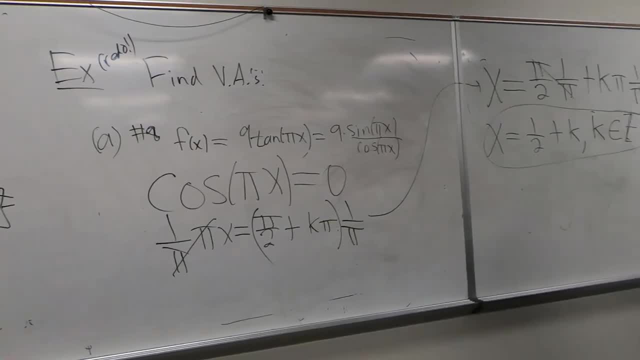 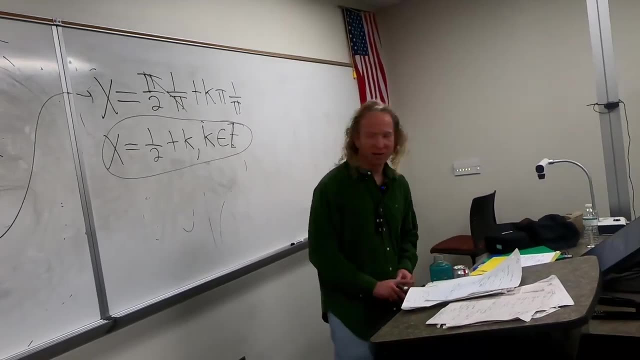 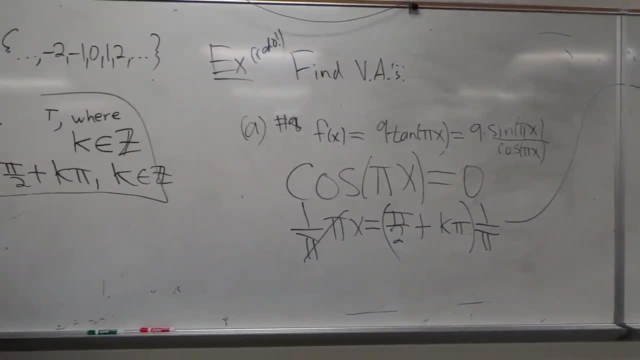 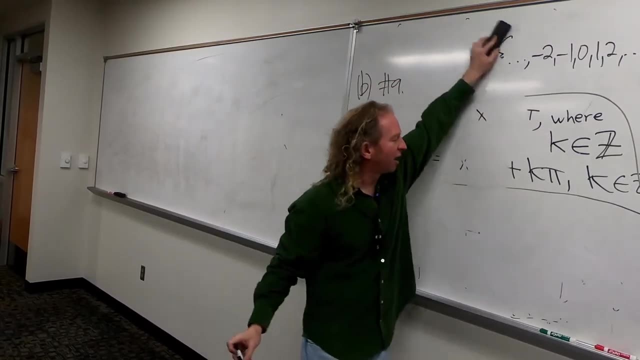 Number 1.. Number 1.. Number 9.. So b, B, B is number 9 from the homework Number 9.. Can someone read me number nine? Is it f of x or f of t? F of t. 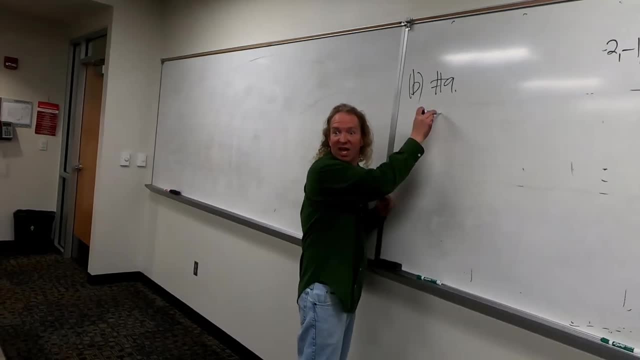 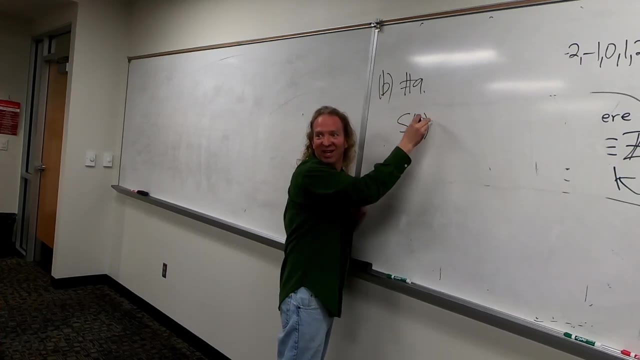 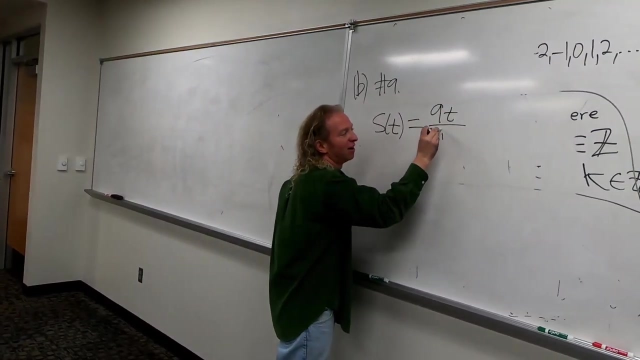 F of t. Yes, F S like in, like superman, Yes, Like this, Yep, Really. Wow, I believe you. Okay, And it's equal to 9T over 9X. Oh, And the homework wants you to use n, okay. 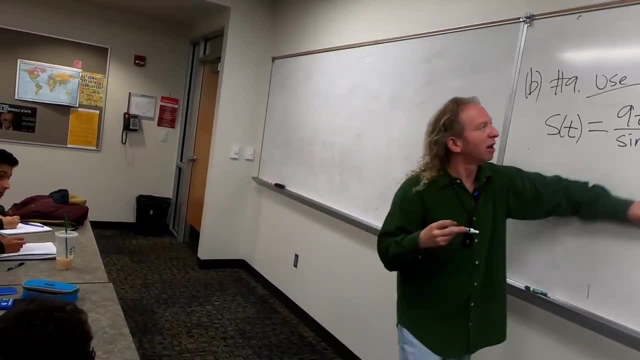 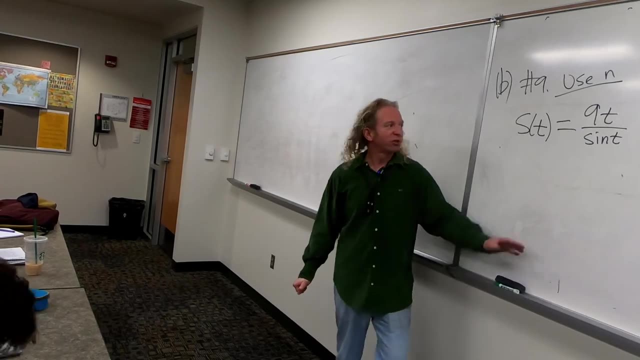 And they have a little box. you have to fill that in. I want to do this one and explain it, and then we'll do more after this. So same thing: we're looking for the vertical asymptotes. So we think about when sine t is equal to 0, right? 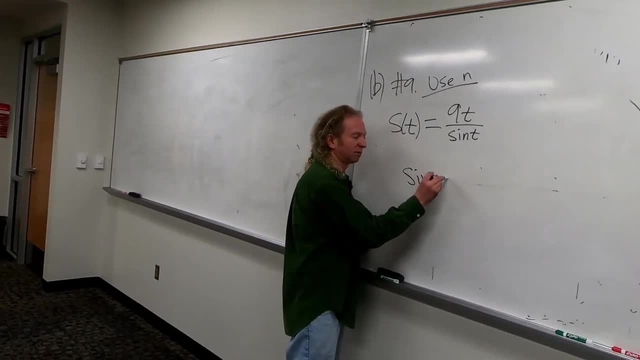 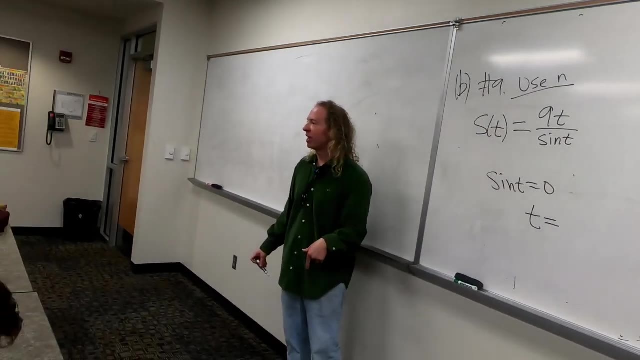 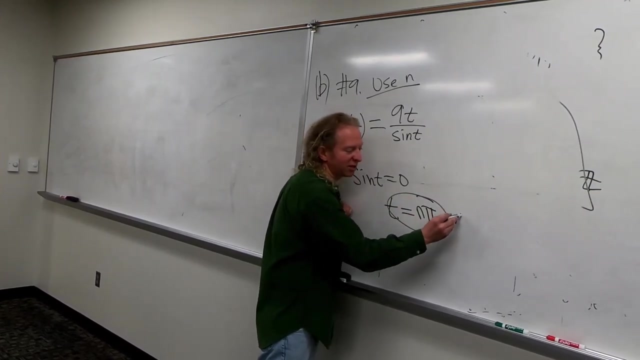 Sine t is equal to 0. when t is equal to well, it's k? pi normally right, But we have to use n, so it'll be n? pi. That's it. That's it. And then n. here is an integer right. This was a test. 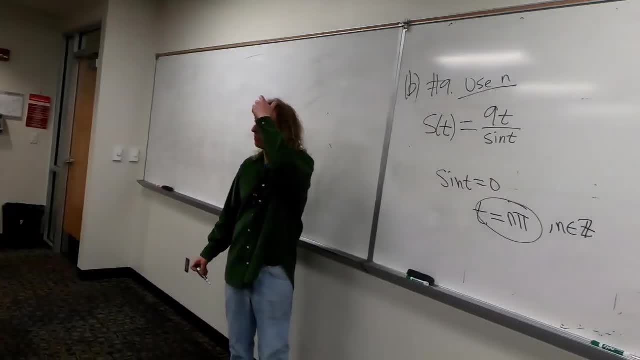 So you can use n or you can use k, It doesn't matter, right? You can use any of those letters variables. The homework has a little box, though, and it tells you that n can't be equal to something. okay, 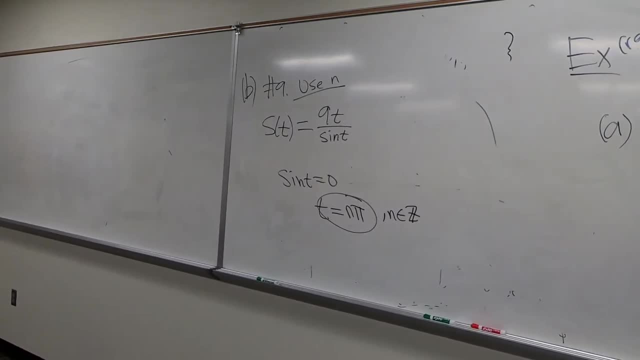 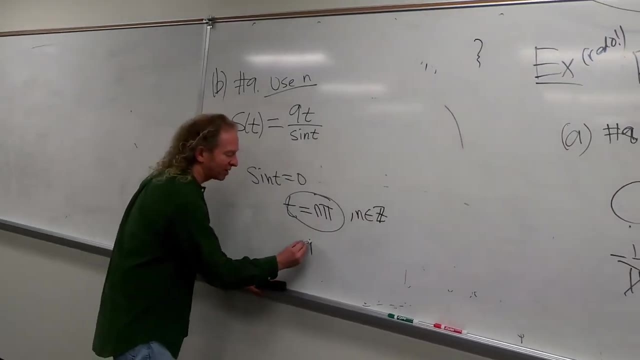 I believe n can't be equal to 0, right, n can't be equal to 0,, okay, Because if n is 0. So n here is not 0. This is really deep, so, aside, I'll call it an aside. 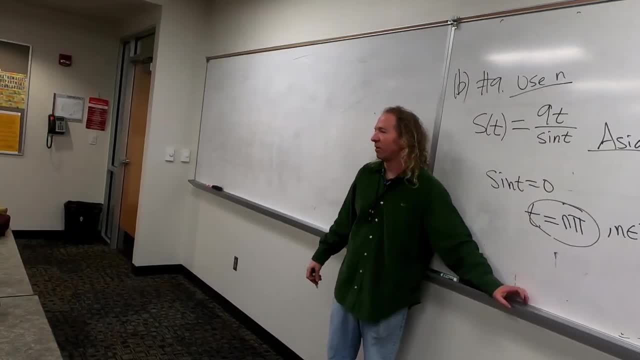 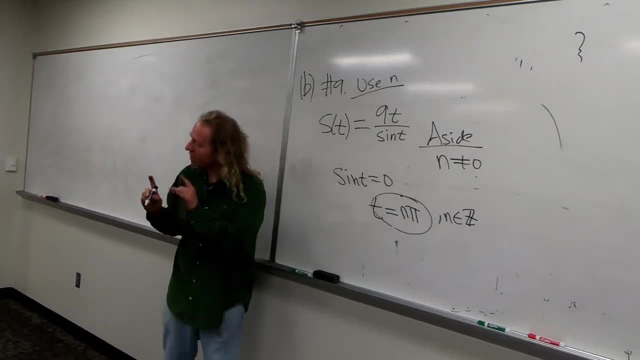 Well, first of all, any questions on this before I go over the next tricky part. Okay, the homework says that n. You're supposed to do this for the homework. Here's why, If n is equal to 0, t is also going to be equal to 0, right? 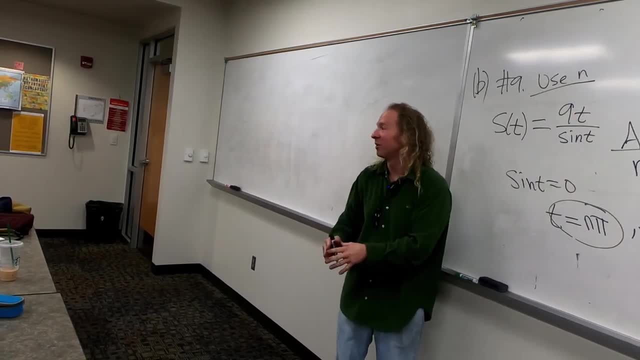 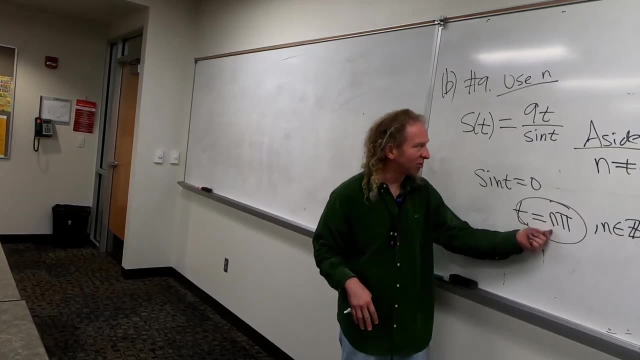 And then you'll get 0 over 0, and you're going to get a whole. okay, So it's not a VA. The homework wants VAs. It's really sneaky, okay? So if n is equal to 0, then t is 0.. 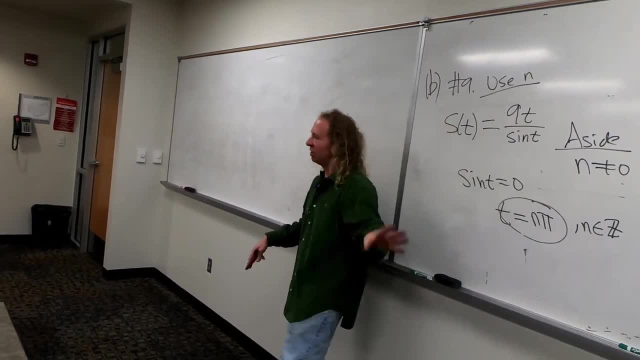 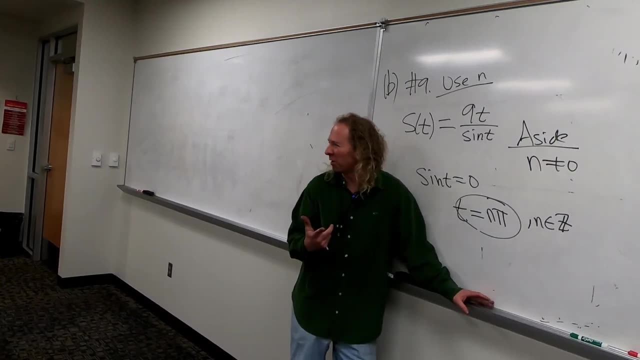 So this is 0 over 0, so you get a whole. So you have to throw that away. Don't worry, You're not going to see something that tricky like in an exam situation. That's just like The first time I saw the homework problem. I'm like why? 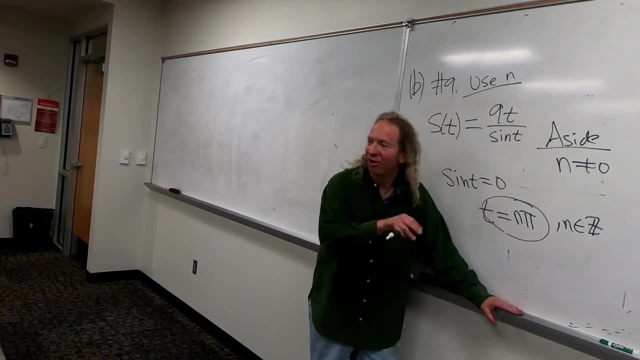 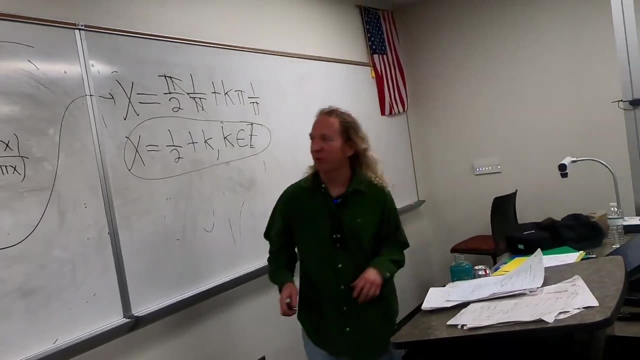 What's going on? Like what I'm like- oh, they think they're smart- Like, oh, trying to throw away the 0.. So that's that one Here. let me give you another one: A, B, C. 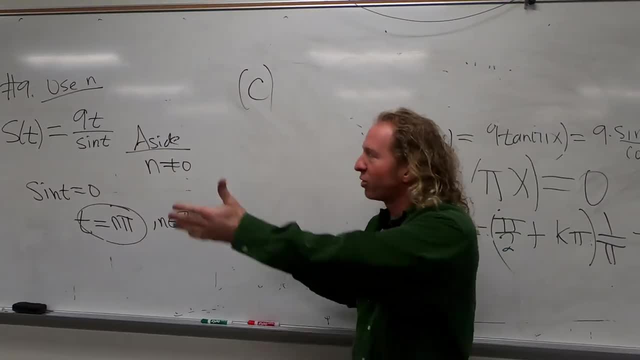 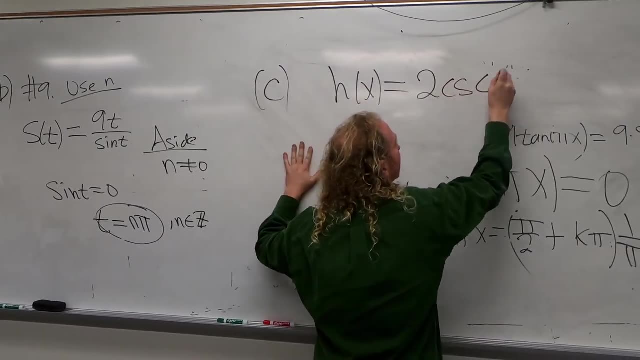 Here's another good test, one C. Oh, since we're using new letters, how about H for hard, H of X equals 2 cosecant 4X. Why don't you all try to do this? one Take like two minutes. 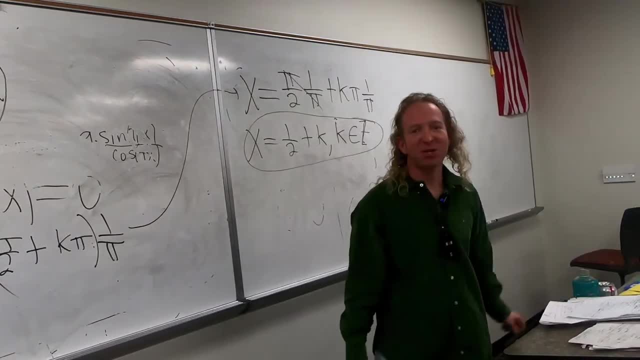 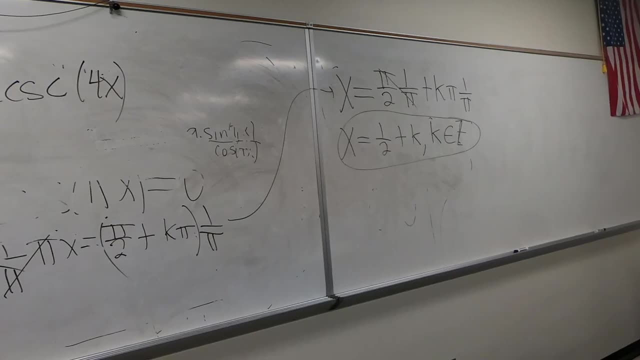 Three minutes. Yeah, Yeah, sure, It's going to follow me though. It's okay, But I'll just delete this. Oh, look, I outran it. No, it's just really weak and broken. Oh, you have to put t equals. 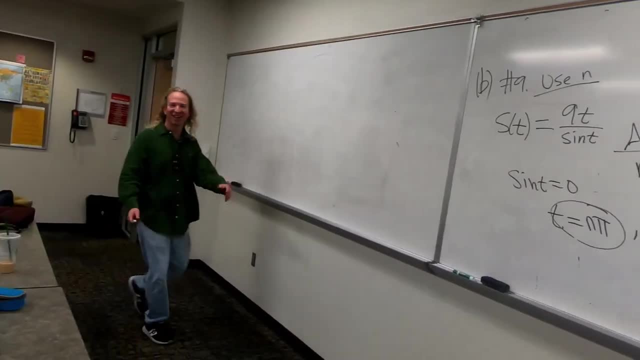 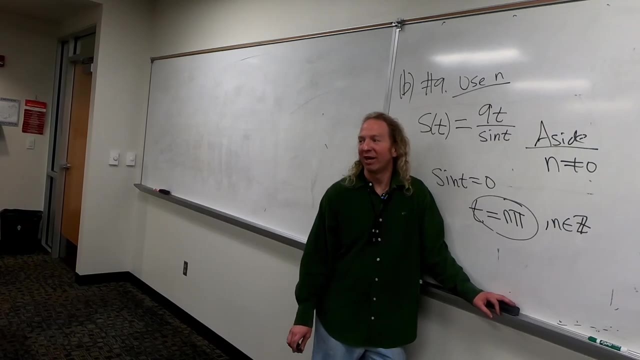 Because it's an equation. All right, It's a vertical asymptote. See, there it goes. Hey, all right, It's back. I used to have a better one. Yeah, They made me give it back, like after I borrowed it. 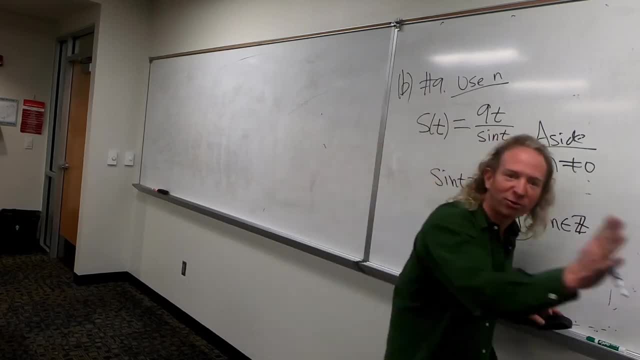 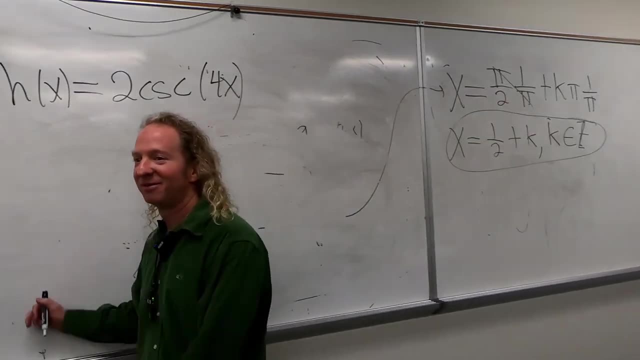 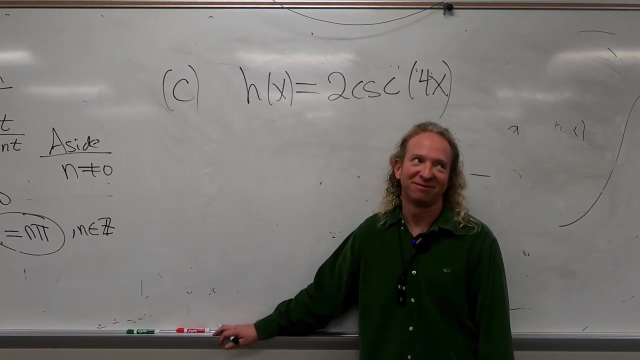 And they gave me this one instead, Like it used to be really good. It would like follow me really quick. That's not mine, So Did you get it? Did you get it? Did you get it Really? 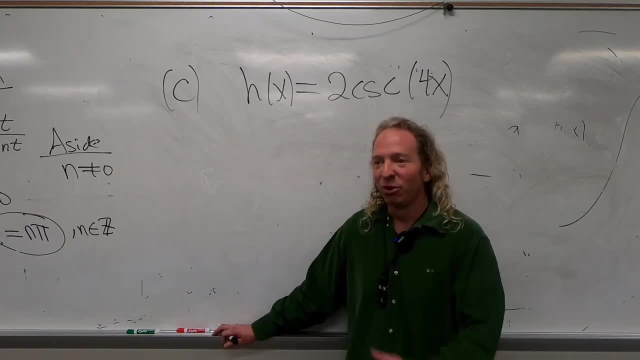 You all got it. Did you get it? What'd you get? I don't know, Oh yeah, Yeah, I think so. I think so, Right Is it? It is Yes, All right, Let's do it. 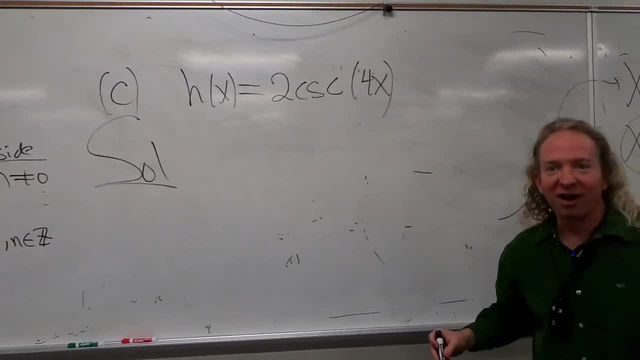 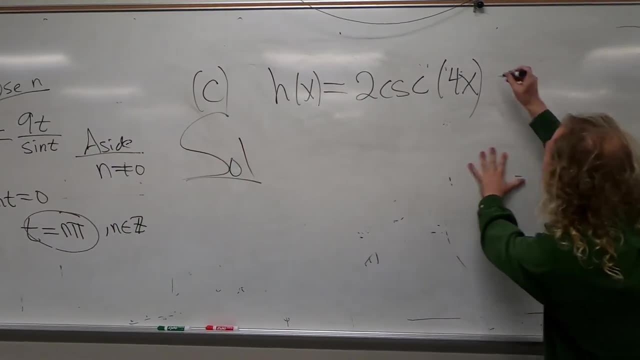 Solution. That's what I mean. Solution. So Huh, We're carrying an integer, So cosecant is one over which function Sine, Yeah, The other letter Good. So you can write it like this if you wanted to. 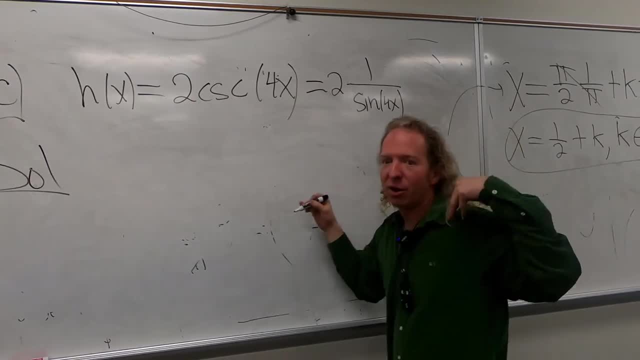 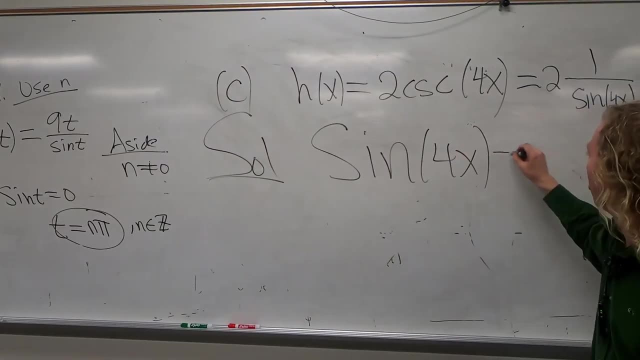 Sine of 4x. So you just think about when is sine 4x equal to zero? So sine 4x equals zero. Oh, broke the marker. It's like it went in. Okay, That's all right. 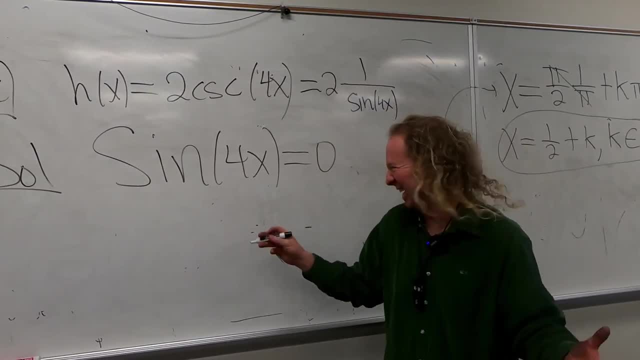 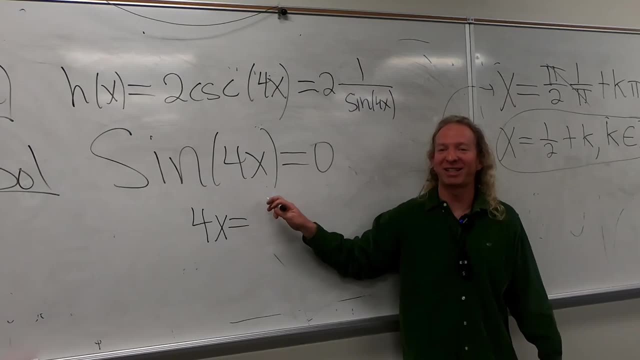 I can't use my mouth. Okay, That's really gross, right? Yeah, it's nasty. So 4x equals. So what goes here? Do you remember K-pi, K-pi, K-pi? 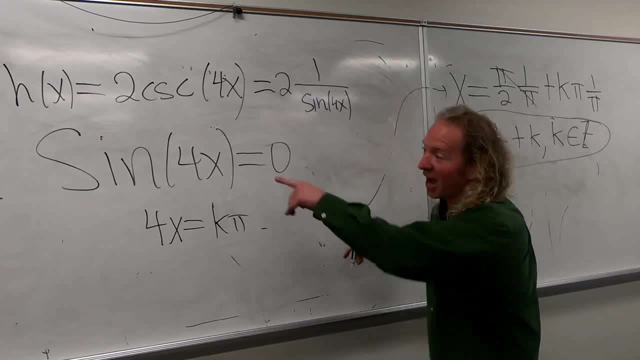 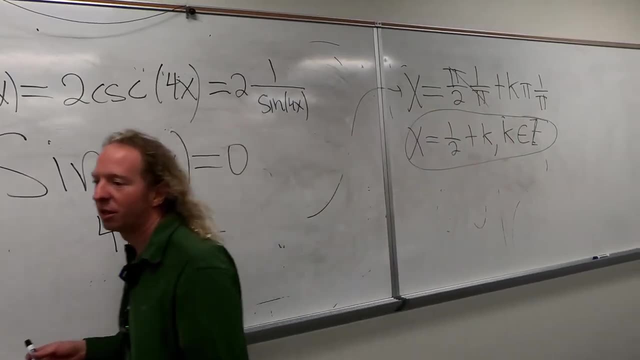 This is really useful, Not just for this class, right? I didn't even learn this in calculus, right? Yeah, It's supposed to be h-pi, or no? No, no, no, No, No, it's h-pi. 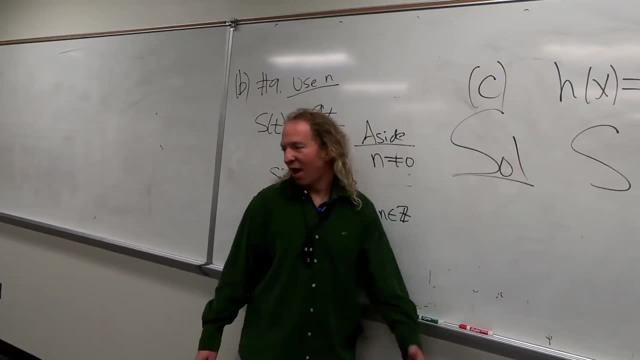 Huh, What's h-pi? Oh, that's just the name of the function. I just wanted to be weird because see, over here it was s. Oh sorry, All right, Yeah, It's 2.. It's 2.. 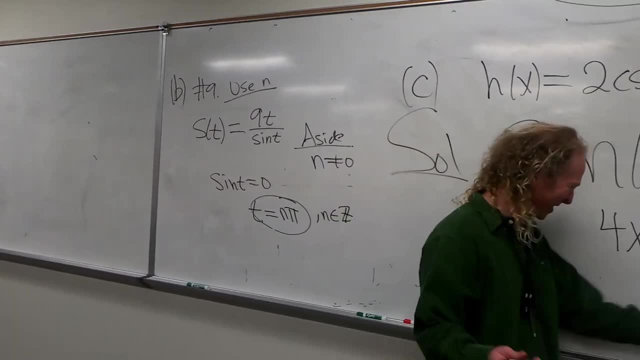 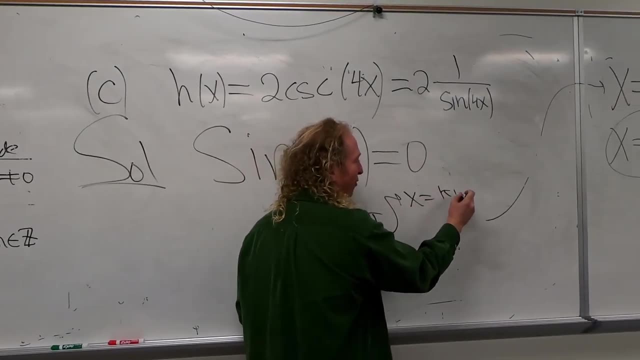 Yeah, I'm glad you asked. No, it's good It worked. I didn't need to fight. So someone would ask: So divide by 4.. So x equals k-pi over 4.. What's missing? 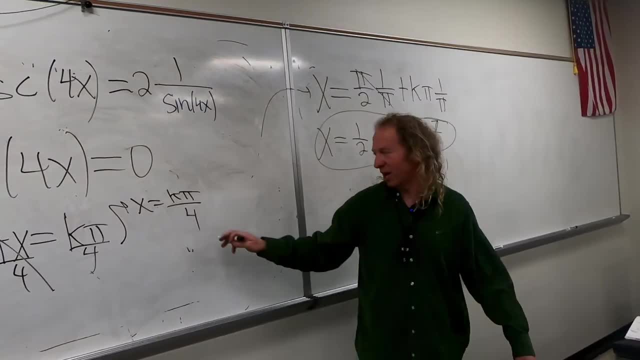 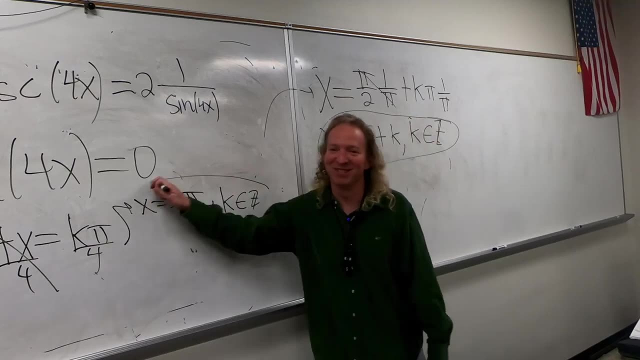 An integer Where k is an integer. Yep, So you're just supposed to say comma k is an element in the set of integers. I'm not judging. It's good. Good Pistachios are the best, That's it. 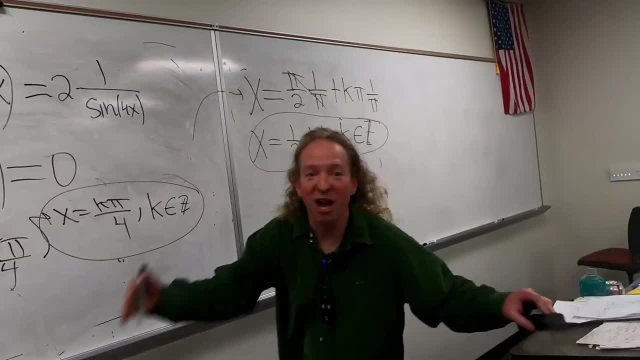 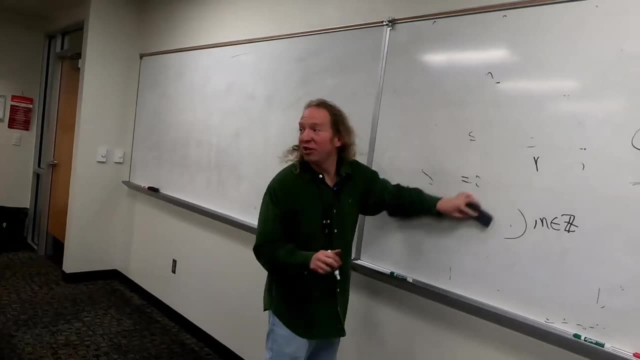 That's it. Let's do another one. Just one more, One more D. You've already done this, by the way. Oh, I thought you had a question. No, it's okay. Do you have to leave? Oh, sorry. 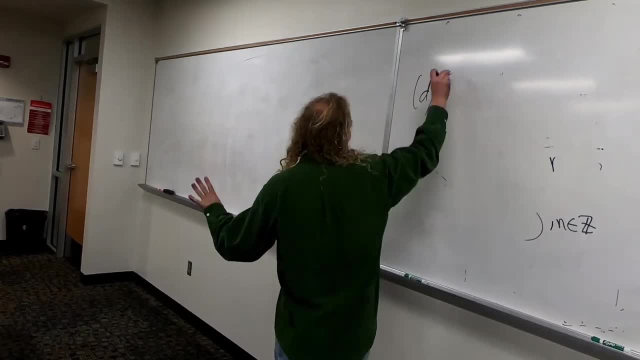 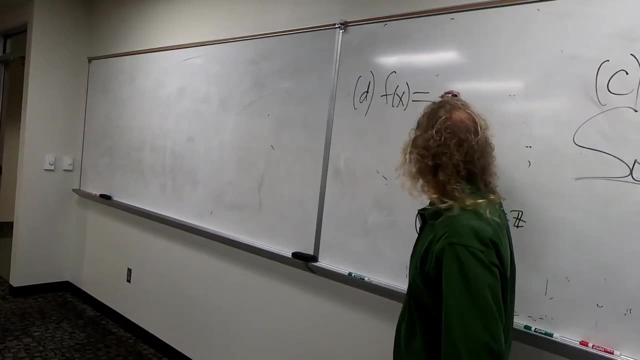 Okay, Sorry, It's really bad. Sorry, I'm sorry, That's fine. What? Oh, I didn't hear what he said. It doesn't matter, I don't know, I didn't hear anything. What did he say? 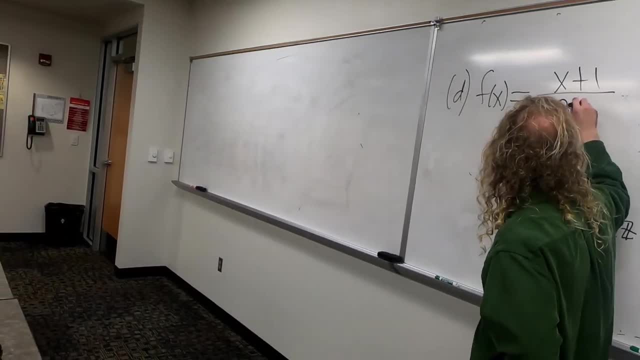 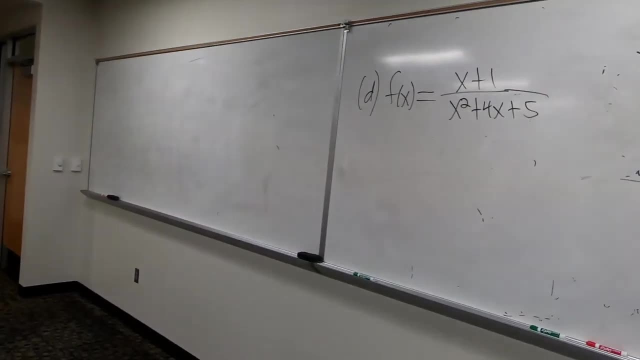 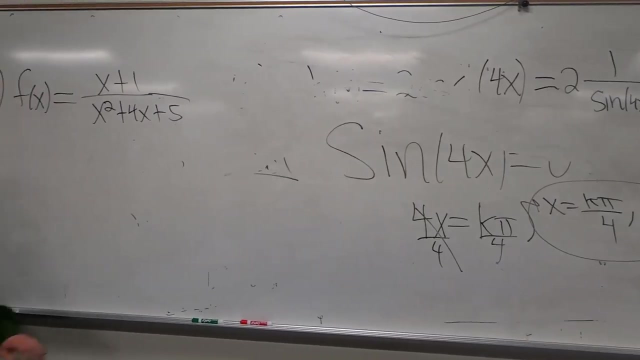 Oh, That's great. That's great: x squared plus 4x plus 5.. Do you want me to do it or do you think you can do this one? I'm going to give you like a take 30 seconds, try it, and then I'll do it. 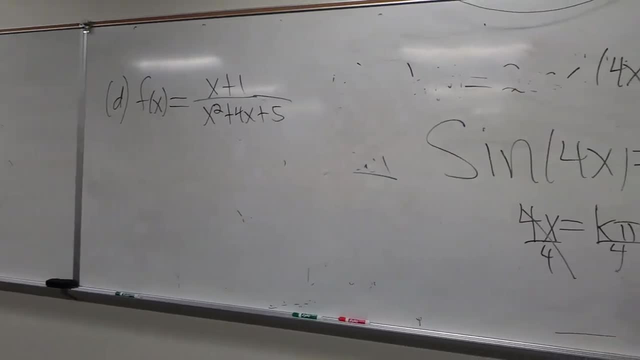 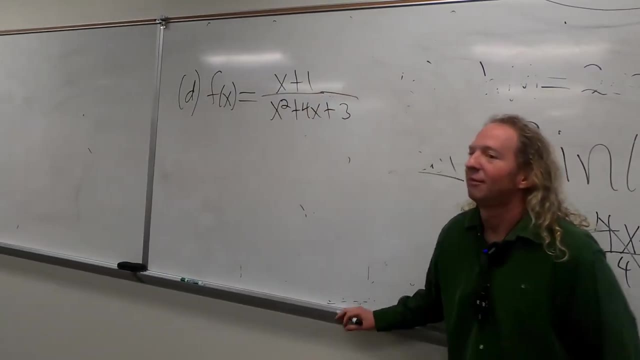 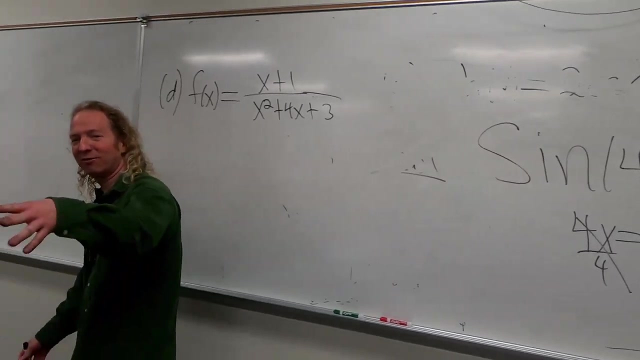 After this we'll do something else, So we did this before. All right, Yeah, go ahead and try it now. Sorry, I was like they look confused. Like I know they can factor, They're pretty good. 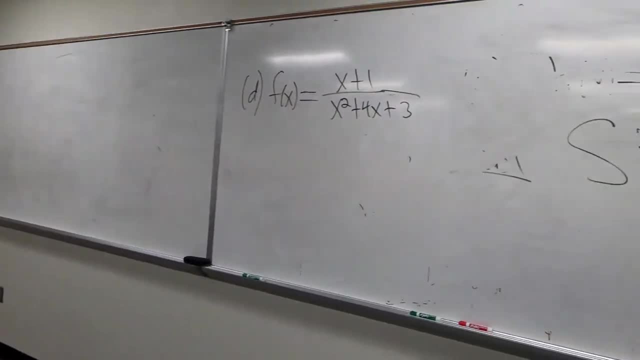 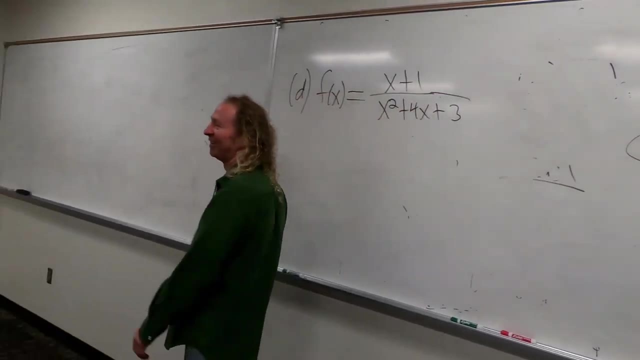 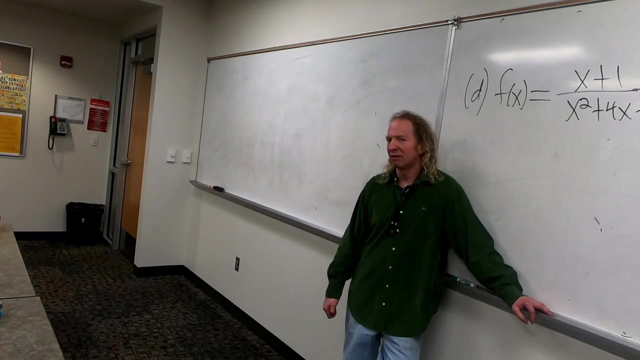 Like I'm, like, it's me, not you. You know, last semester they had a take-home test, I think for this class, Because they had the hurricane right. Wasn't that the hurricane? Yeah, I know. 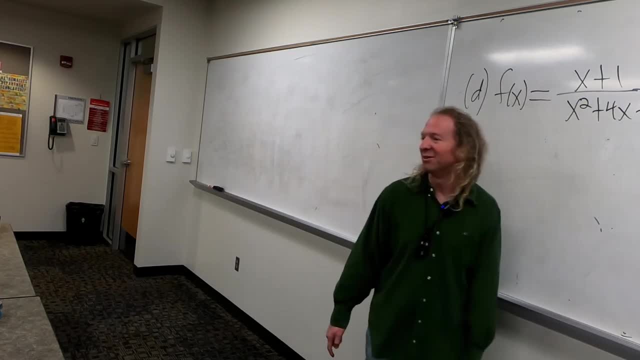 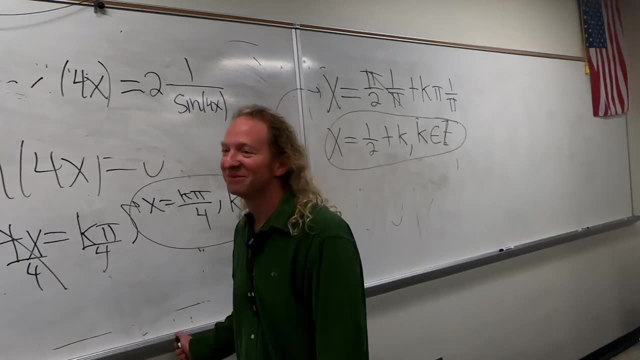 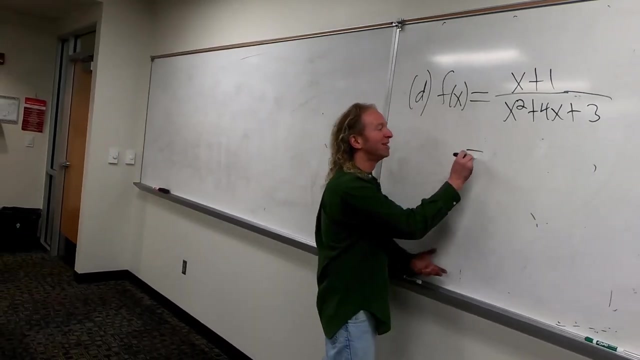 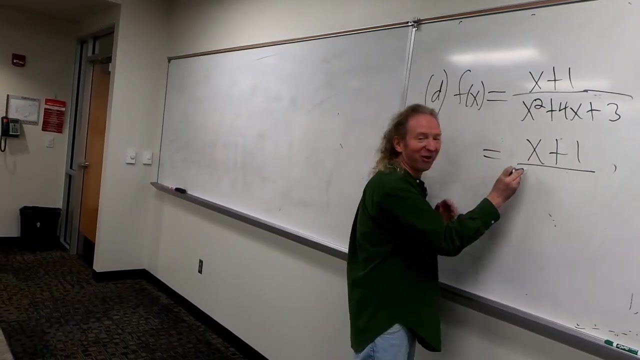 It was a little hurricane. I know, I know It's just not fair, It's just not. I'm going to do it, I can't wait. x plus 1. This should factor right Now. Yeah, now it should factor right. 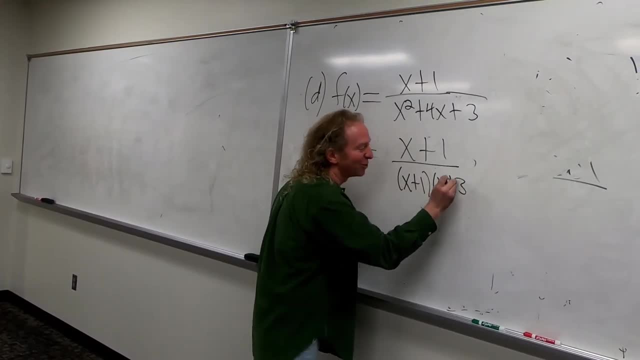 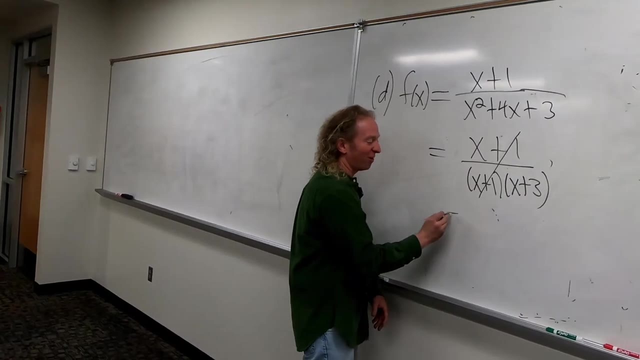 So it's x plus 1, x plus 3.. It should factor now, Is that right? Yeah, Okay, good. What cancels x plus 1.. Yes, we get 1 over x plus 3.. Then you set the bottom equal to 0.. 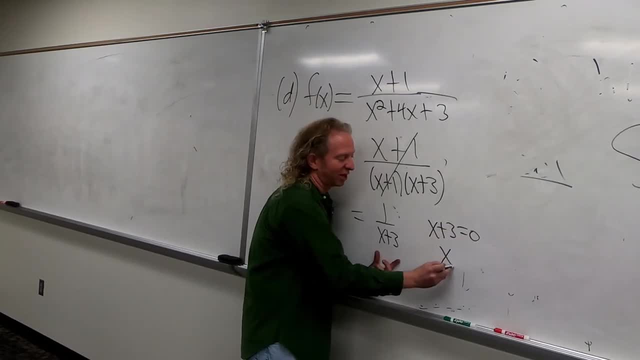 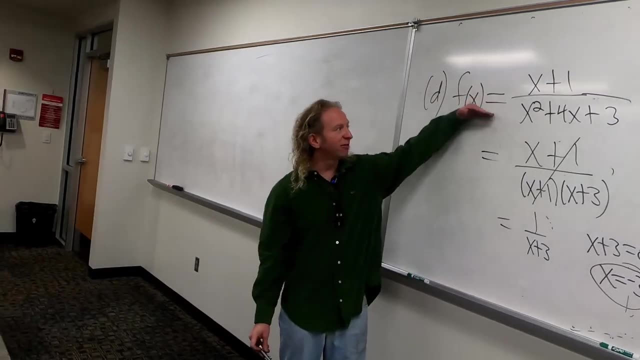 So you get x plus 3 equals 0.. So you get x equals negative 3.. It's really important to have the x equals right in this case, Because it's a vertical asymptote. So basically, to find vertical asymptotes in a rational function. 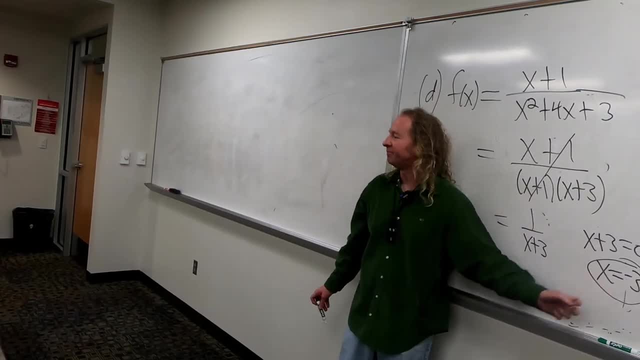 I think we've done this before. you cancel, And then you set the bottom equal to 0. And since there's no k, you don't have to put 1.. Right, It's only with the trig functions. Yes, Logan. 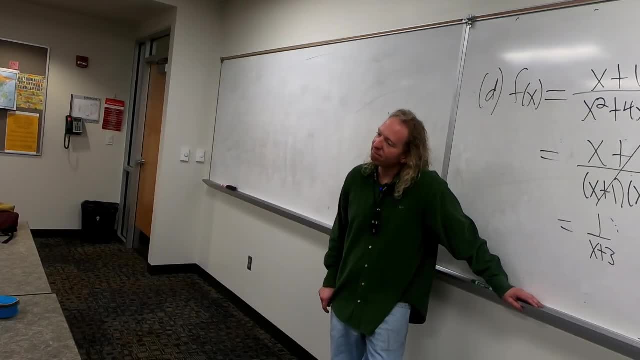 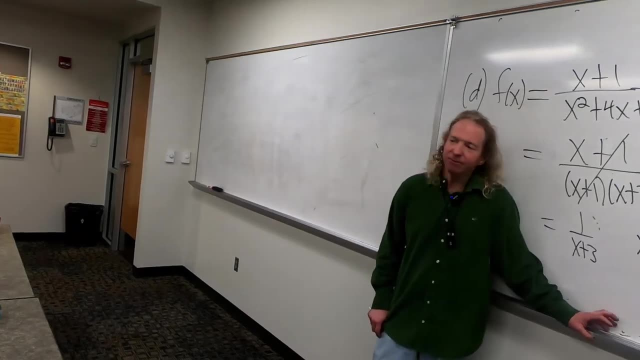 Just an offset question. Why wouldn't they put like they'll put like x cannot equal 0. Or why don't we do that with vertical asymptotes? Where Are we just identifying that the vertical asymptote is that where x equals negative 3?? 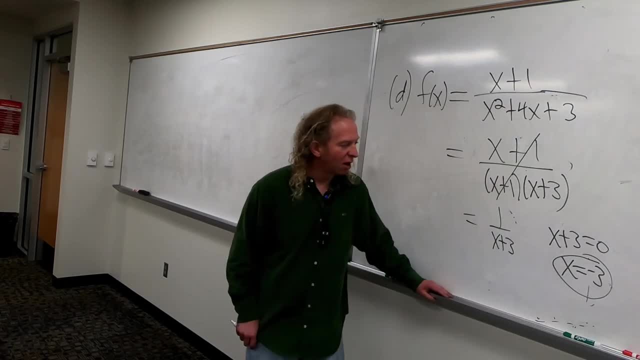 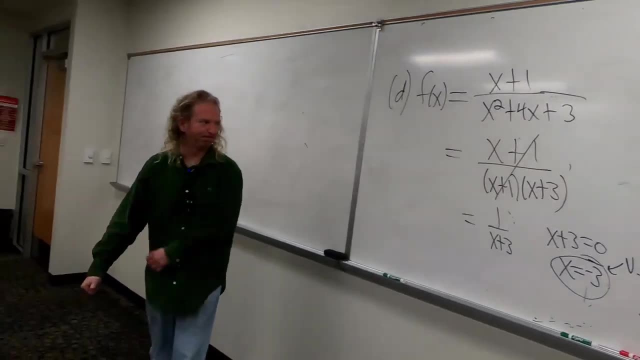 Or are we saying that x cannot equal negative 3 because it's a vertical asymptote? No, we're saying that the vertical asymptote is x equals negative 3.. Okay, Good question. By the way, what happens at negative 1?? 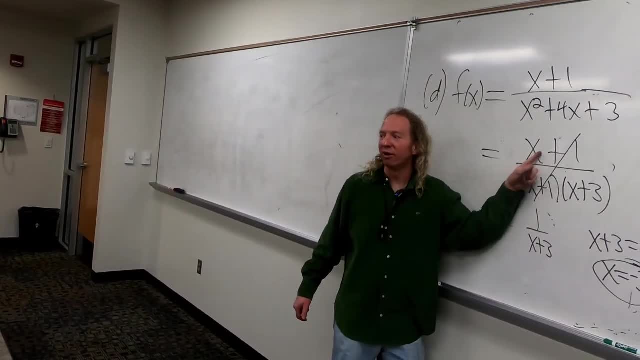 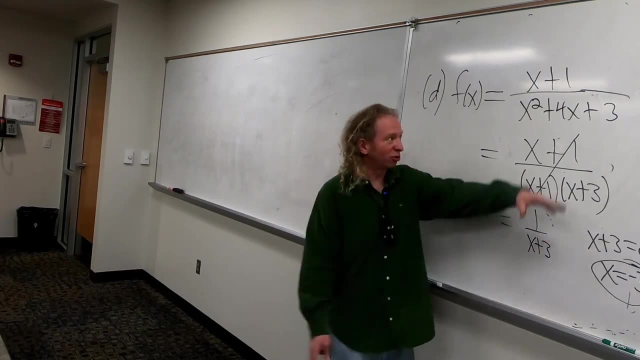 What do we have there? A hole. Is it removable or non-removable? And what about this one? Is it non-removable? Yeah, good, So that's another question you'll have probably right. So two different questions. 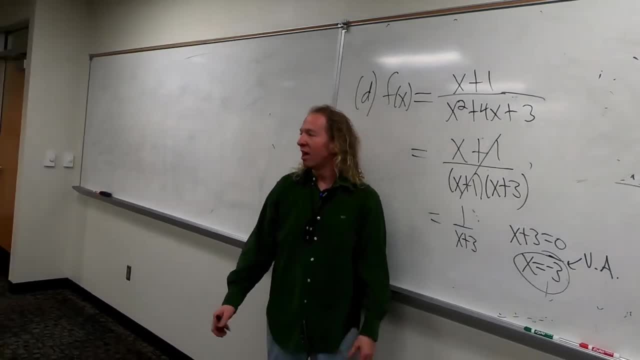 One where you have to find your VA, and then one where you just answer what you just did. And then you have the trig ones. Those have the k in them right, And then you have the limits, where you don't show work. 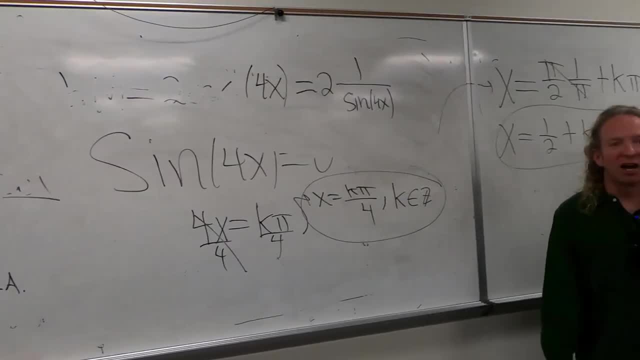 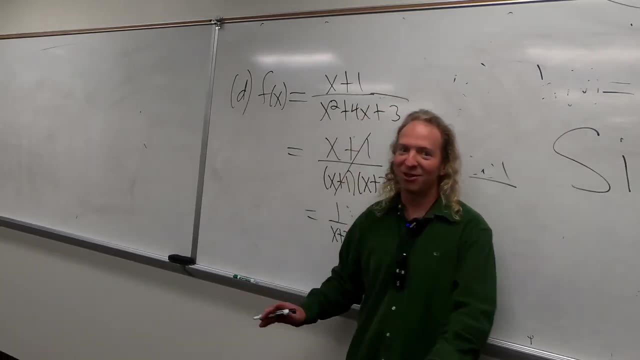 That's like 30 points right there, right. So yeah, In theory, like if you didn't do any homework and you just went over your notes, in theory, in theory, in theory, you can get 100, right. 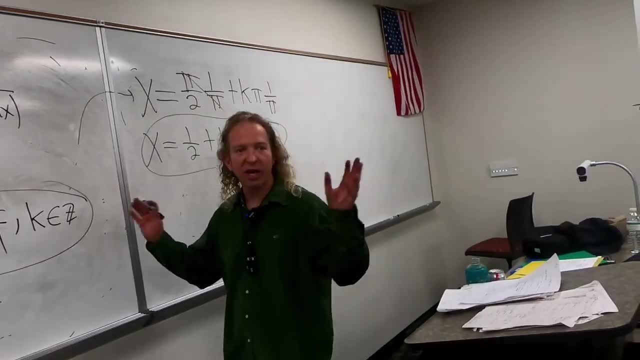 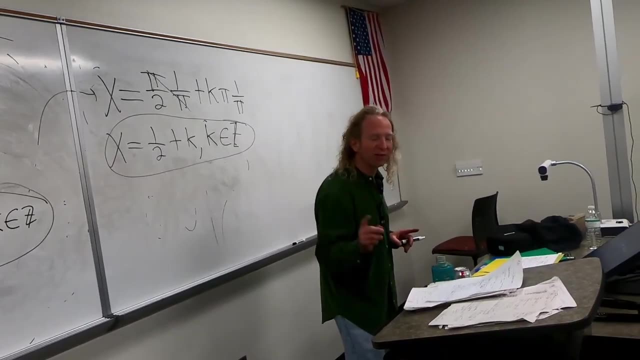 Let me show you how to do something else. okay, that's later, Just in case you want to do some homework. And I'm also going to show you how to cheat and get all of the answers to the homework in the next section also. 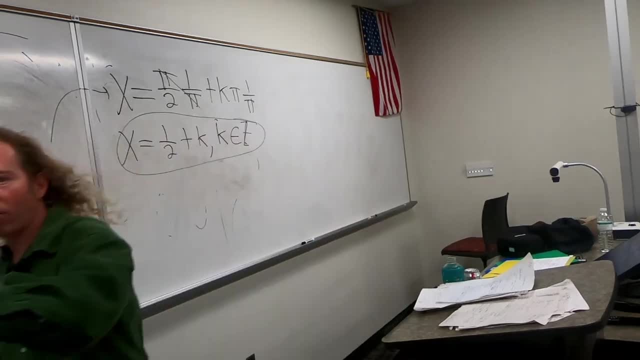 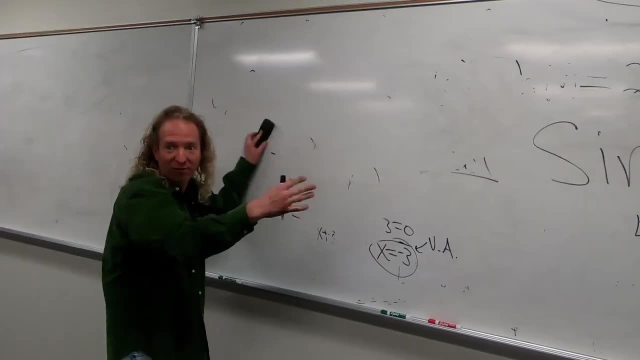 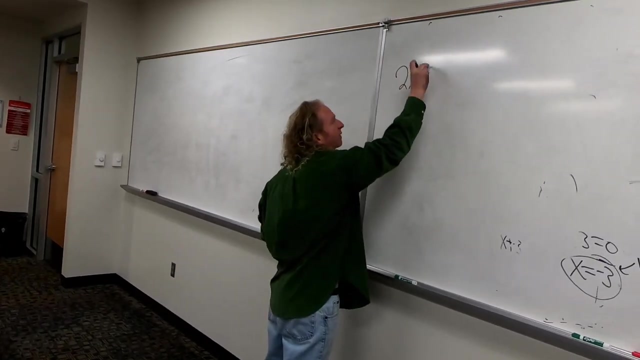 But first let me, let's do a problem. I'm going to do one problem from 2.1, so we haven't done this, so I'll pretend we didn't do this next time. Next time, when you come in, because we're done with 1.5, we'll do 2.1, like there's like 45 minutes of notes, it's deep- and then we'll do 2.1 again. we'll do this again next time because this is like a lot of points on the test. 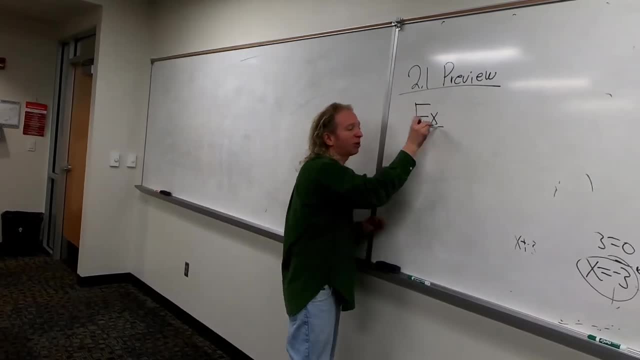 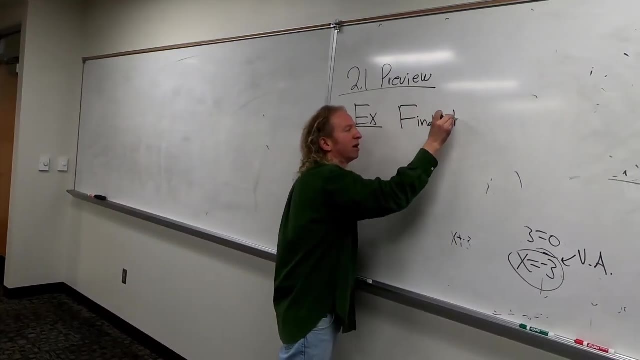 So I'm going to do, I'm going to call it an example. I'm going to call it an example and we'll say: find the. so you might not know what this is. it's okay, I'll tell you. 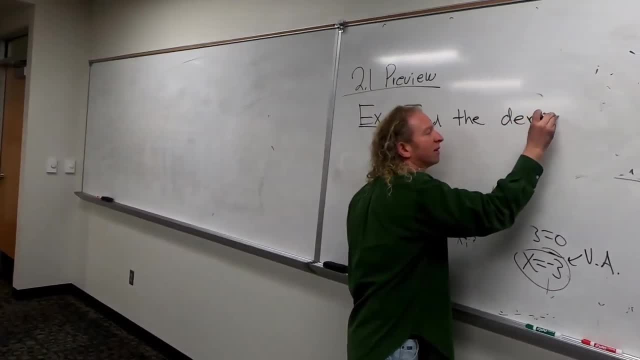 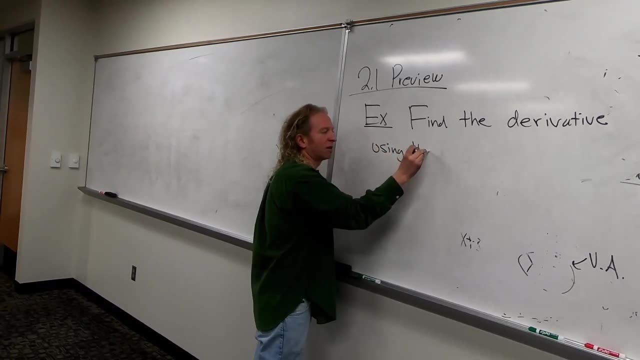 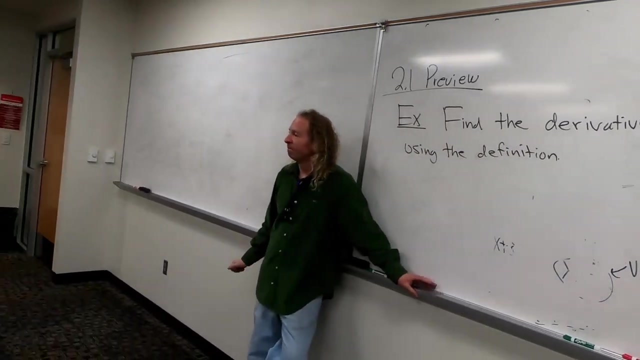 Find the derivative using the definition. So using the definition. So this is like a 10-point question on your test and you'll probably have like two of these right, Probably like two of these. 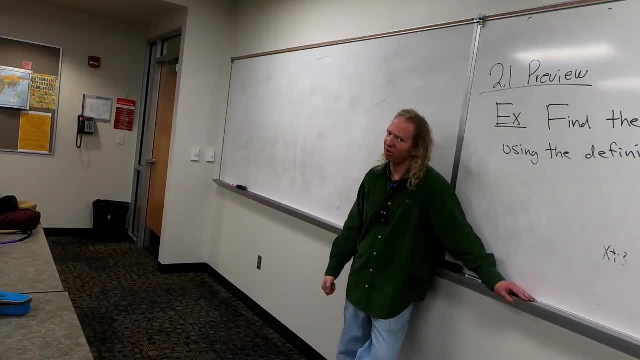 It's not bad. Most people get it right, even if it looks it's kind of hard. No, you'll get it right, Like if you study, you'll get it right. You'll get it right If you study. 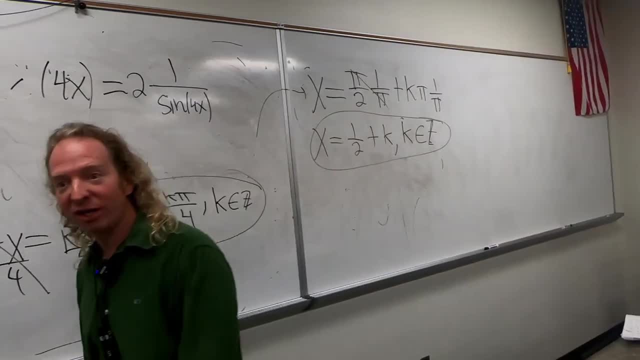 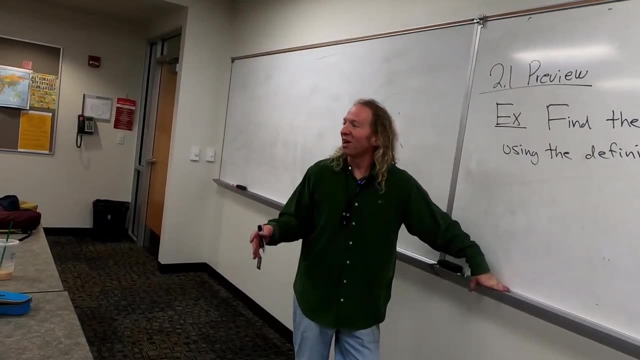 Yeah, if you study, What's your name? Austin? Really? Oh wait, no, never mind, Okay Nothing, No, it doesn't matter. There's a guy in my other class. his name is also Austin, but he was sitting over there, so I'm just so confused. 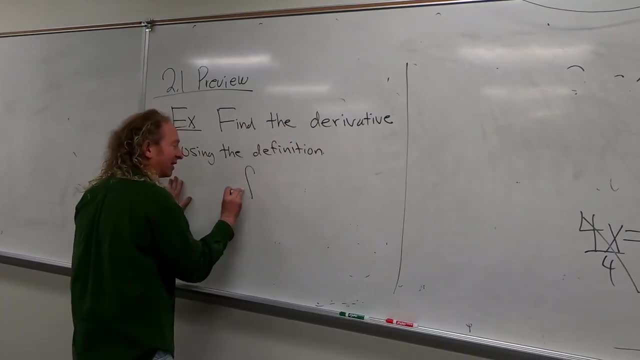 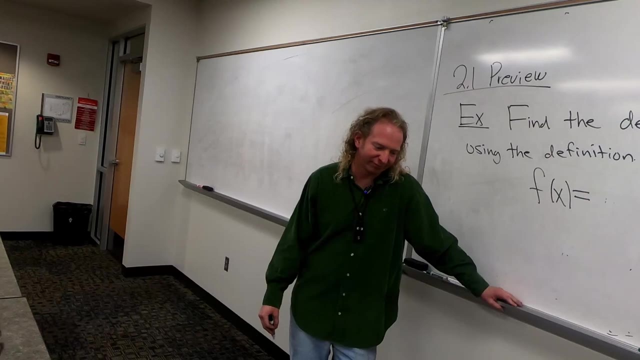 It's too many people, So the function is f of x, F of x, equals. let's see one that will probably be on the test. Okay, okay, yeah, yeah, this seems like a good one. I don't want to do it, but it's probably going to be on there. 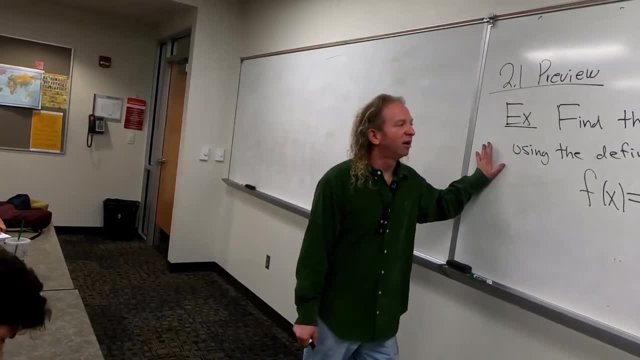 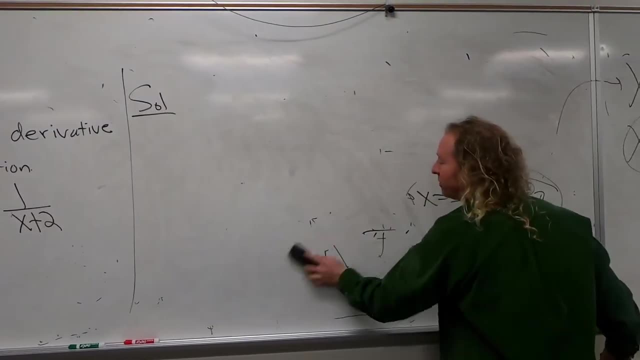 One over x plus two, So solution: All right. So, but you'll probably have two of these on your test right. Every semester. every calculus class in the entire world does this. This is like one of those problems. 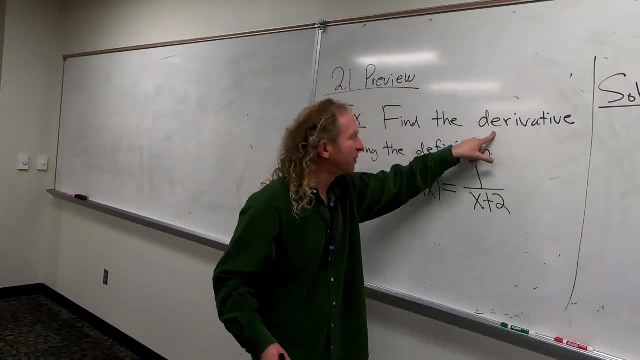 So the first, so the formula for the derivative, whatever that is. well, let me just tell you. So, if you have a straight line right, like say you have, say you have, like y equals 2x plus 3.. 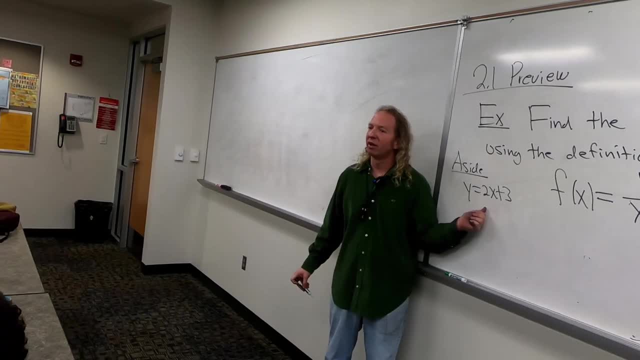 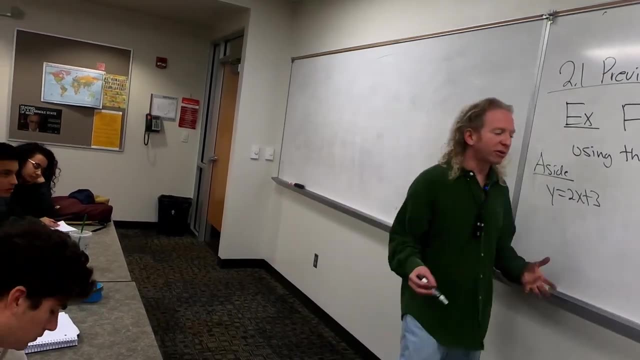 So this is mx plus b, right? What's the slope of this line? Two m is two, right. So for straight lines we have the slope right. It's the rise over run. So in calculus we talk about rates of change, right. 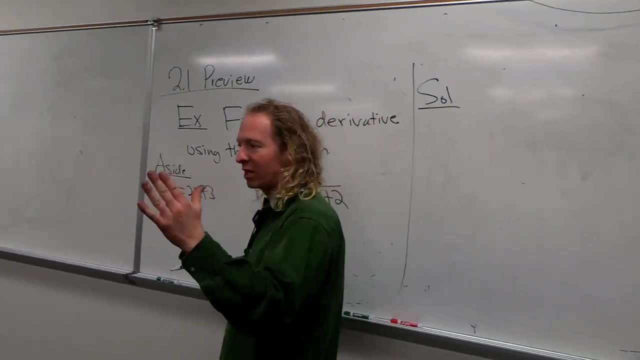 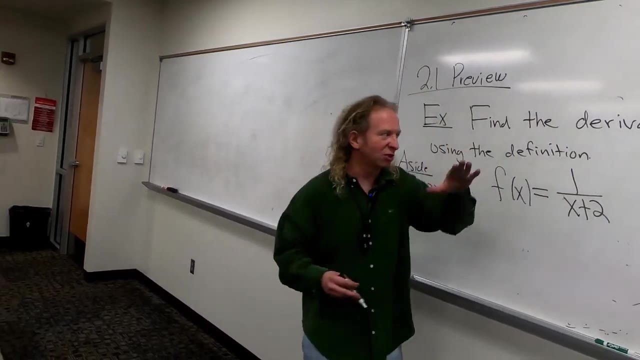 So we have random functions And so we want to find out what the slope of is of a random function. Well, the slope is going to change, right, So it's going to be like a slope function. So, to find the slope for a function, it's going to change. 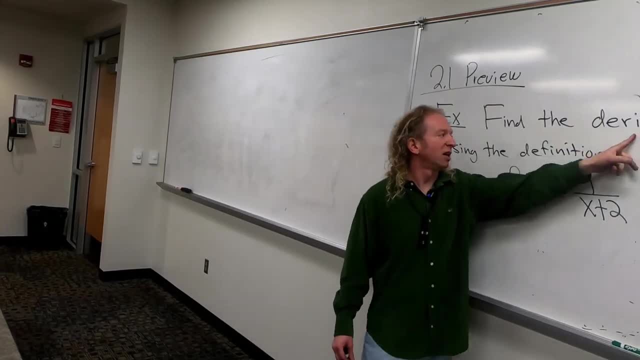 It's not constant. It's not a constant slope, So the derivative is the slope of the function. So the derivative is the slope. So we're going to construct it from scratch next time at the beginning of class. It's really beautiful. 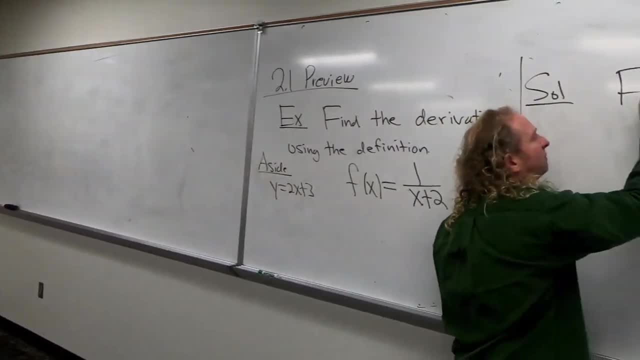 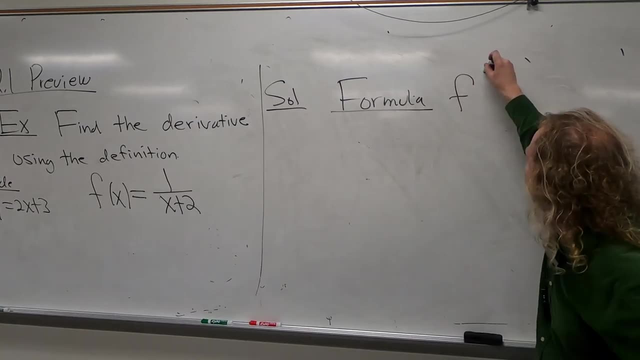 For now we're just going to use the formula. So the formula for the derivative is f, And then you put- I'll do it here- f, And then you put a symbol. here It's f, prime, P-R-I-M-E. 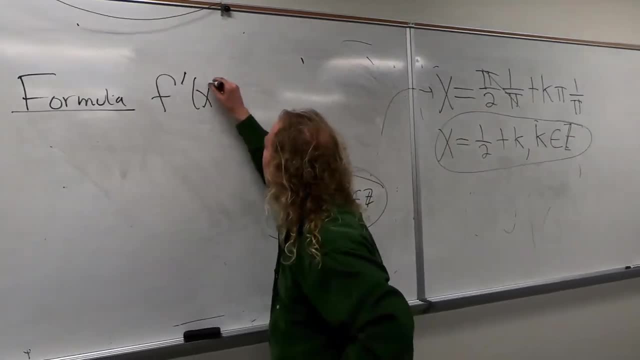 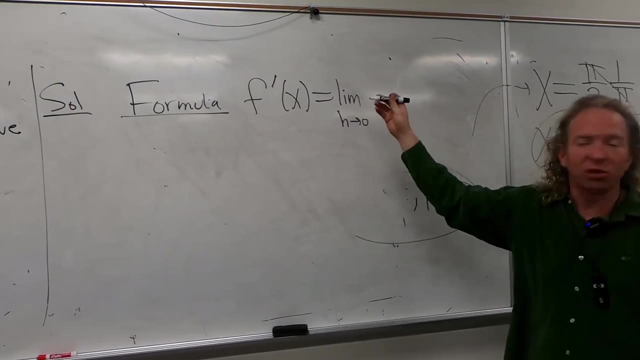 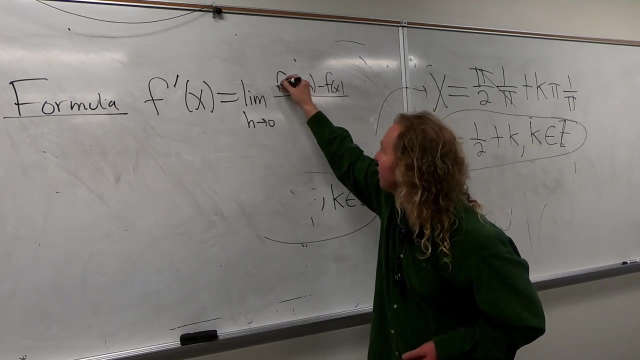 Like prime F, prime of x, And it's equal to the limit, as h approaches zero, of what's called the difference quotient, which you learn, which you study briefly in college algebra. In college algebra they make you compute this. It's like on a test. 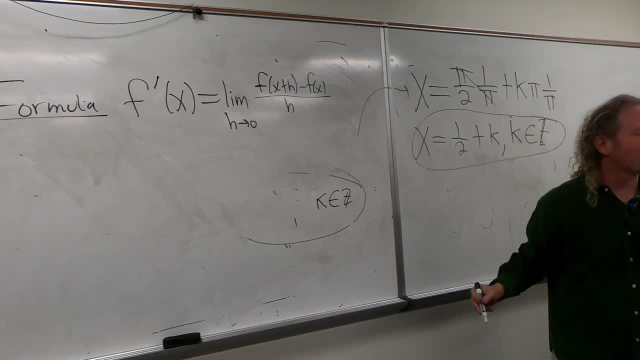 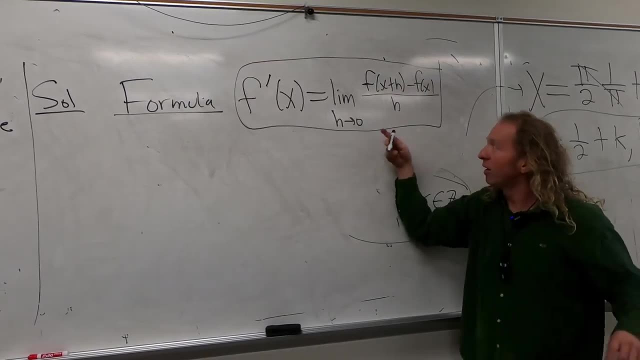 And you compute it And you work it out. In this class we do the same thing, except at the end of the problem we just plug in zero for h. So this is the formula for the derivative right. You may have seen this in the homework before, except instead of h it had something else notorious. 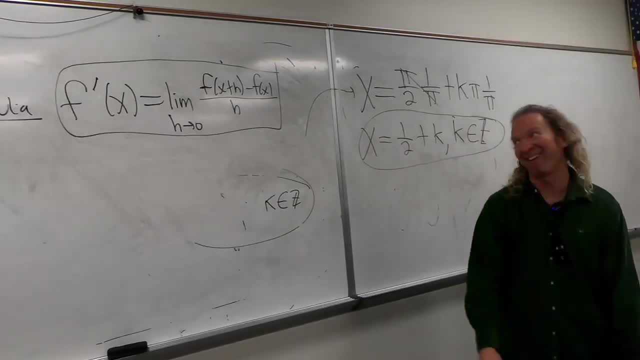 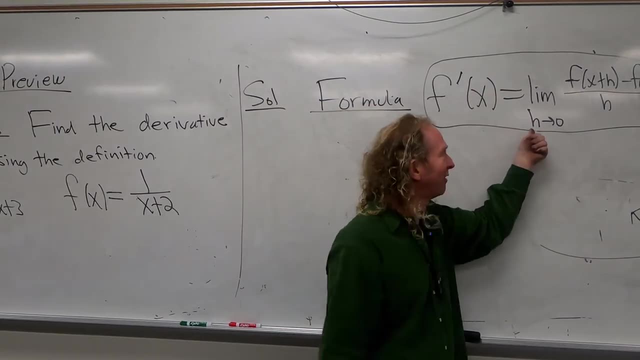 Do you remember what it was? The delta x? I know It was like. oh, I recently. I recently, this morning, I posted a video from the homework, The one over x plus three. when I did it, I finally posted it. 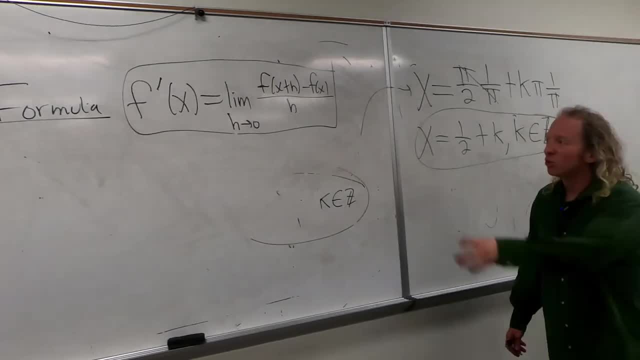 And it's got a delta x in it. I'm like: oh, The delta x makes it so much harder, So we'll be using h, All right, So let's do this problem. So all you have to do is work this out. 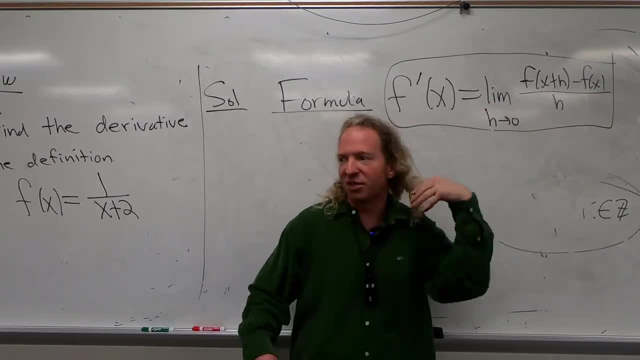 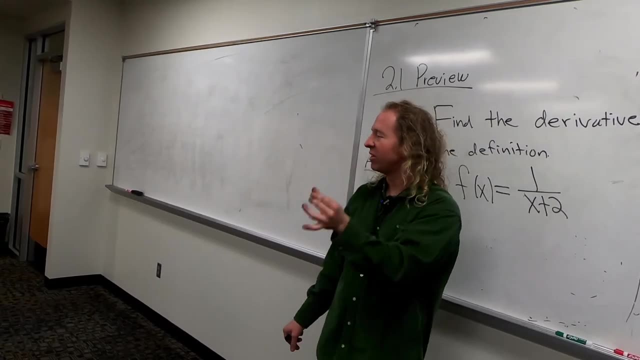 Okay, So keep in mind whenever you write the limit sign. you have to continue. You have to continue to write it. So you have a choice: You can write it every single time from the beginning, or you can wait to the very end to write it. 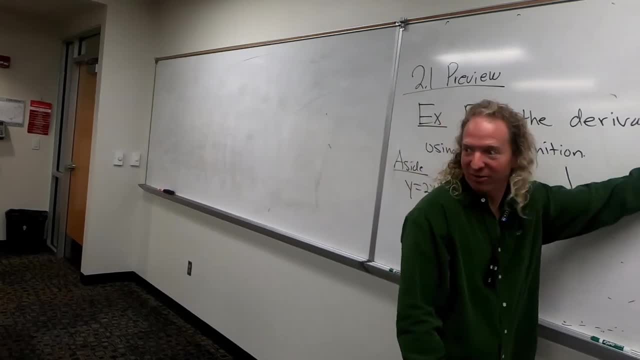 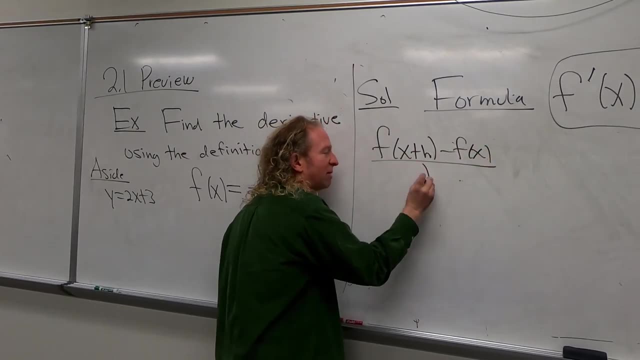 Let's wait to the very end to write it, So I'm not going to write it first, I'm just going to start with this. It's really important to show the work correctly, So maybe, step one, write the formula down. 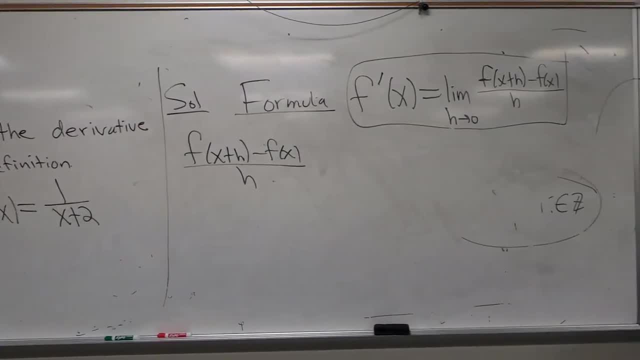 So the formula. you'll have to memorize it, but you'll know it. There's a gazillion of these in the homework, So I'll show you. After this, I'll show you how to get the answers to the homework using the internet, in case you don't want to. 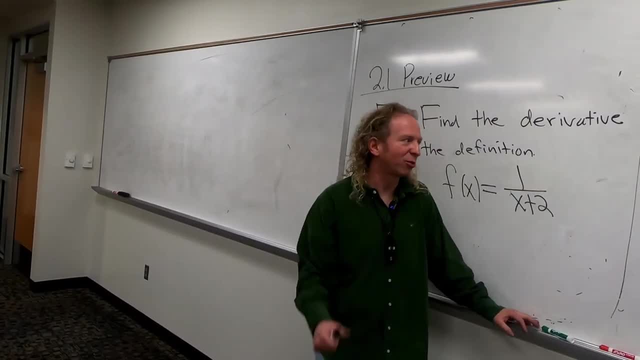 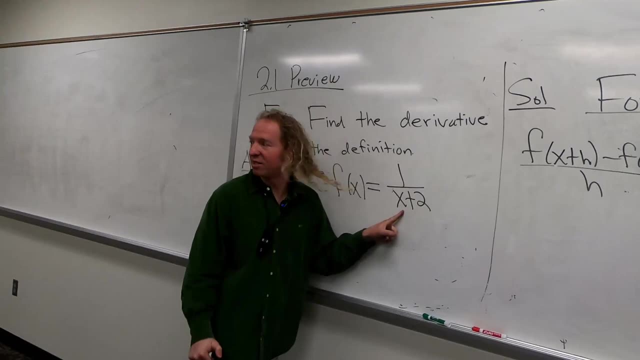 You don't want to do them all right. Because there's so many right, Your hand will burn out. So this is equal to: So f of x plus h means we replace all of the x's here with x plus h's. 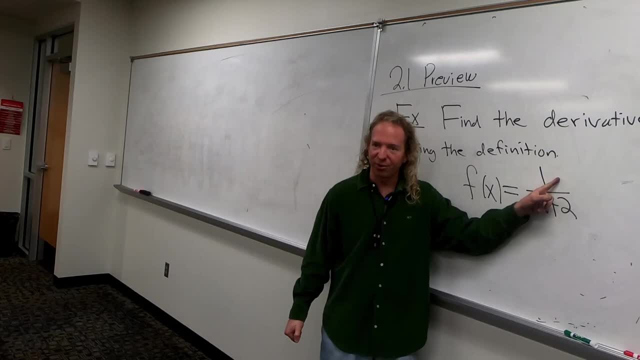 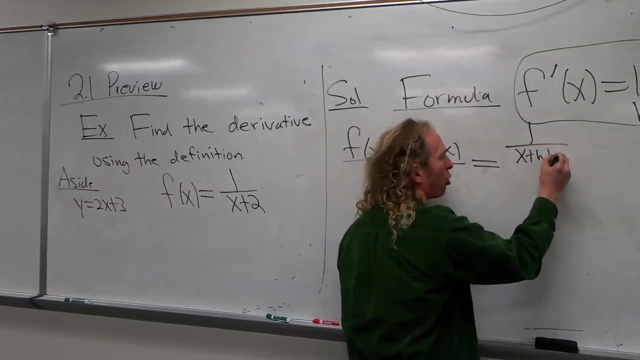 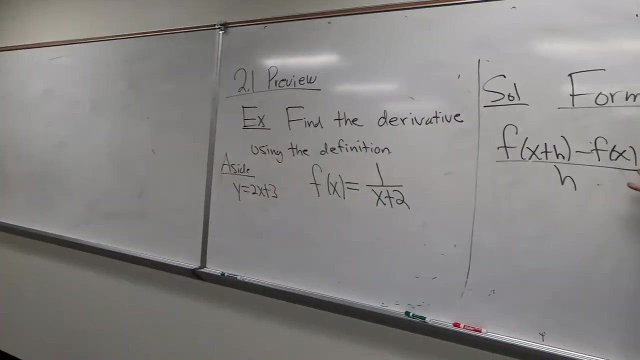 So instead of 1 over x plus 2, it's 1 over x plus h over 2.. Very good, Yes, So all we've done is replace x with x plus h. So this is this Everyone see. 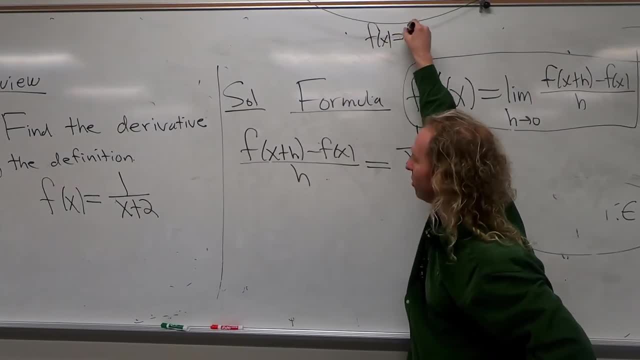 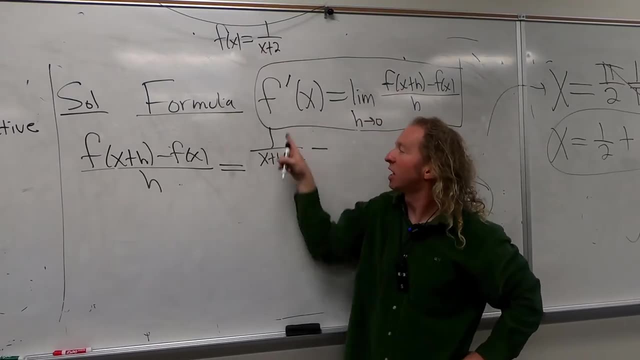 Because f of x. I'll write it up here: F of x, which was taller. is this So f of x plus h? you just put an x plus h there. See X plus h. X plus h. Does everyone see it? 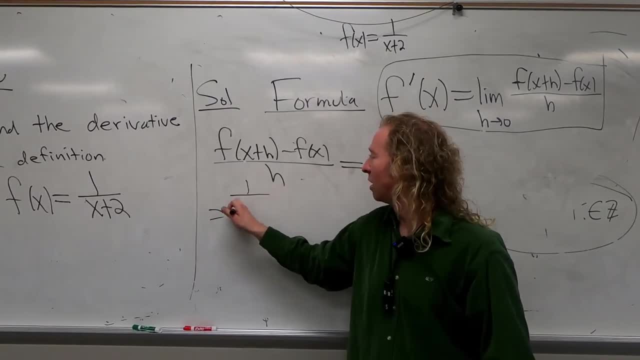 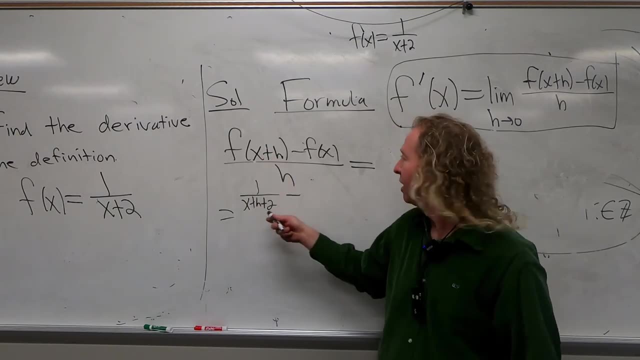 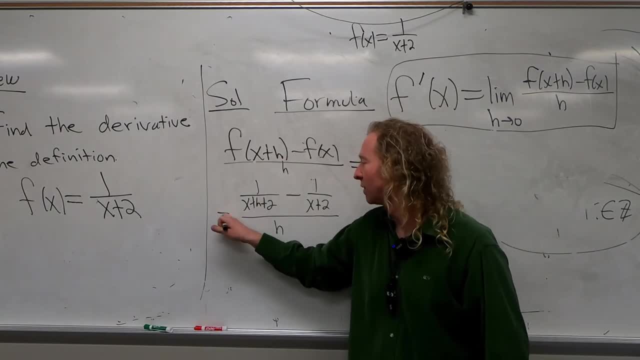 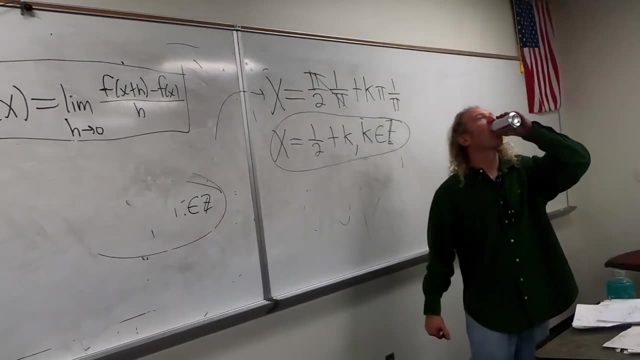 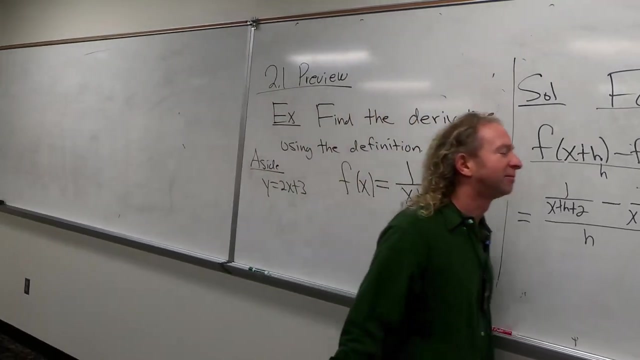 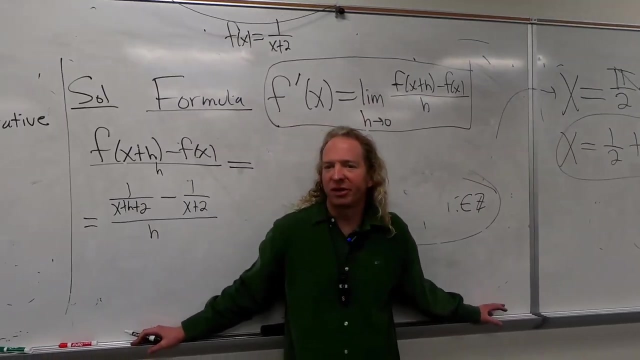 Let me catch up. So this is this. This is this. I'll pause. I'll pause. Hey, Welcome back. Welcome back. Any questions on that? That's a hard thing in college algebra for people to grasp. So f of x is 1 over x plus 2.. 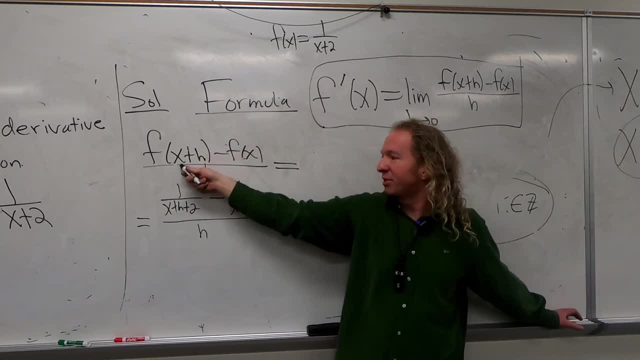 So f of blah is 1 over x plus 2.. So f of x plus h is 1 over x plus h plus 2.. You're just replacing the x's with the x plus h. Everyone get it. Everyone get that step. 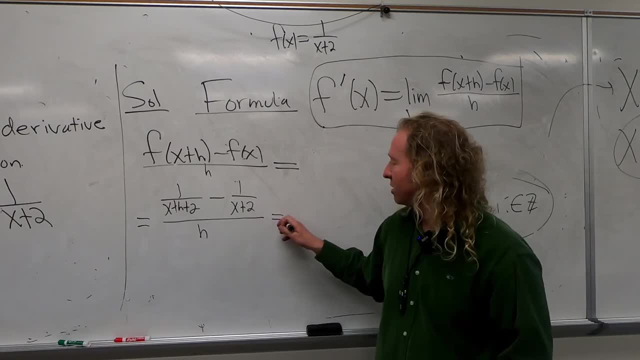 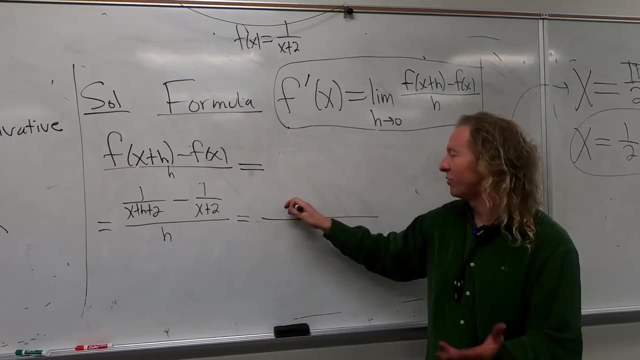 Yeah, Okay, All right. So now we have to subtract these. The way I do it is, it's kind of cheap. I just write down the product because that's going to be the LCD, Okay, So I just know that that will work. 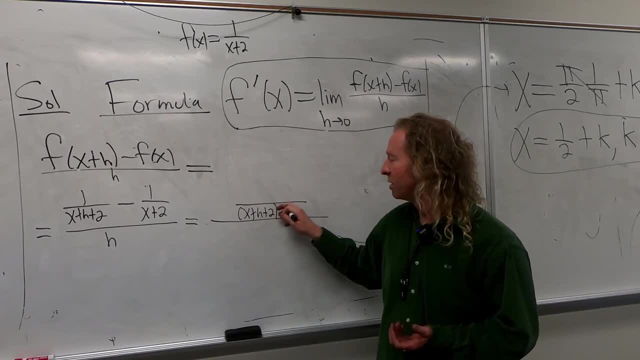 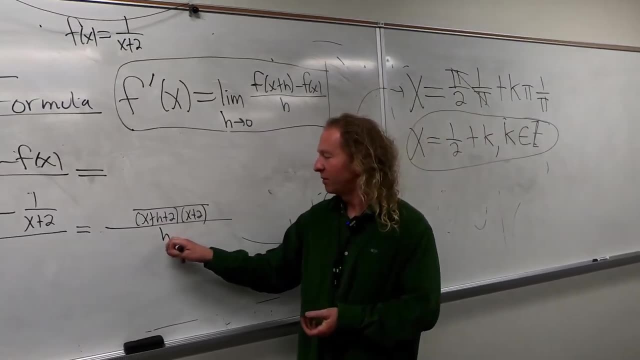 So it's going to be x plus h plus 2 times x plus 2.. Okay, And then we still have the h here. So we haven't figured this out yet. I just write it down first. I just know it's this times this on the bottom. 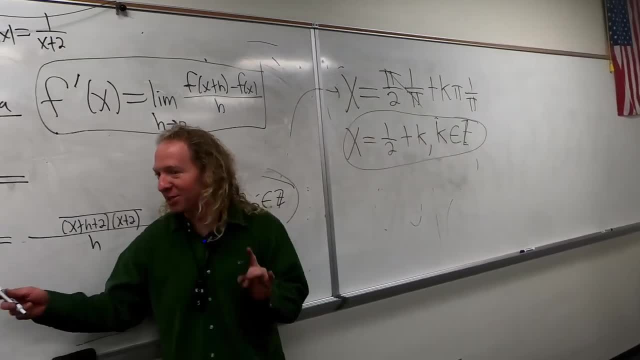 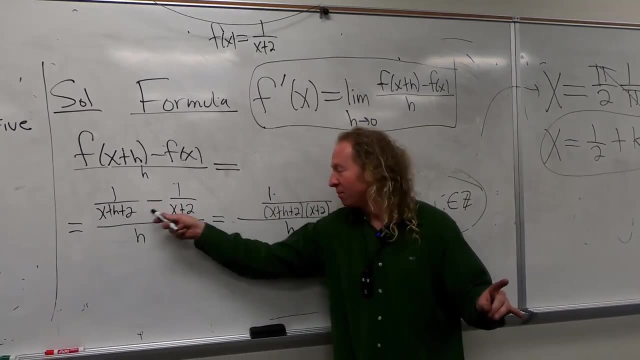 That's good water, Okay, So then it's going to be 1 times, and then here you have this, but you want this What's missing here? x plus 2. So it's 1 times what's missing. 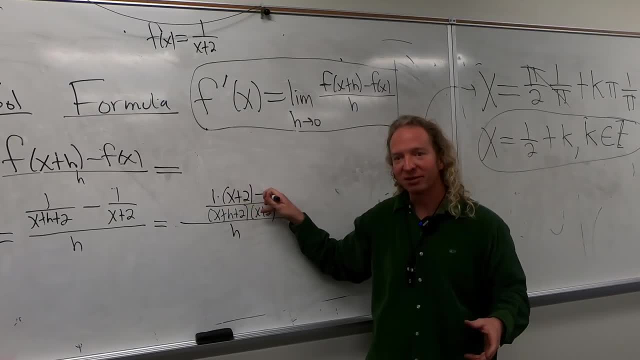 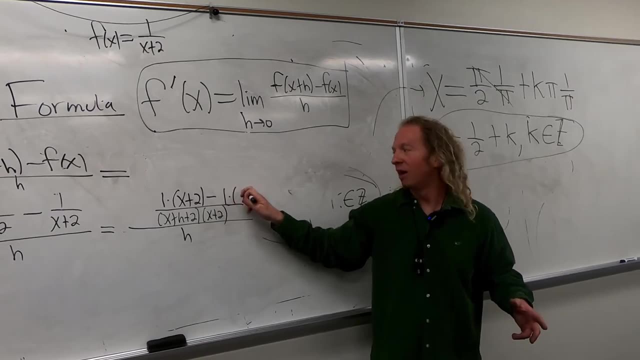 I don't know where I learned that, but it works Minus And then it's 1 times what goes here. Good, Very good. This is so. there's a lot of points on your test. Okay, It's like final exam type stuff. 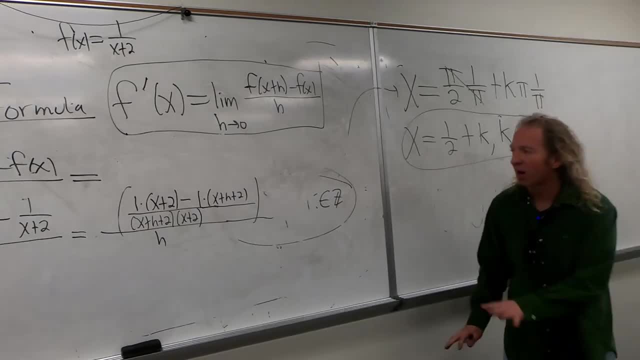 So you usually have one in your final like this too. So it's really important. Let me pause here. I'll go over it again. Notice, I added those parentheses there. They were already there. It's just no one ever talks about it. 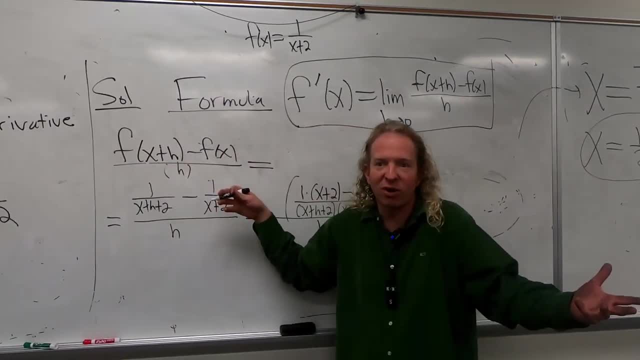 Right, They're here. Look, there's parentheses here. There's really a parentheses here, but no one ever does it. Why? Because it's weird, Right, But there is. If you were, If I write 2 over 3, there's really parentheses there. 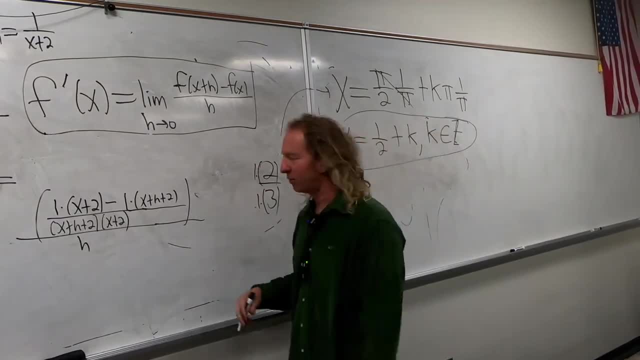 And you can put a 1 there, Right, You can do that. It's the same thing Like they're implied. Okay, So again, it's 1 times what's missing: x plus 2.. Minus 1 times what's missing. 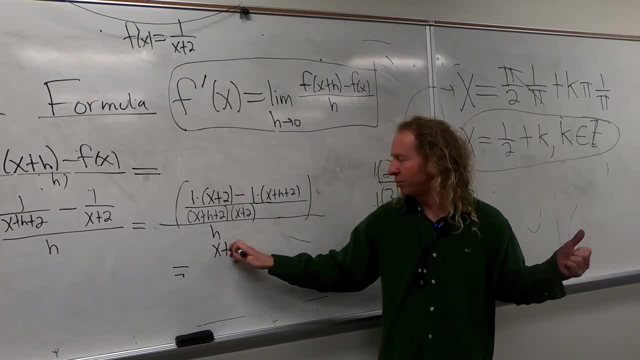 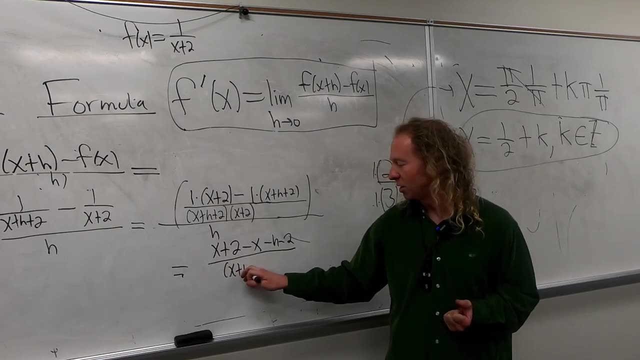 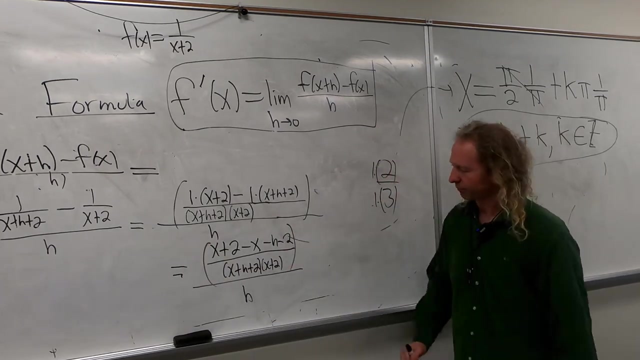 x. So here we can distribute. So it'll be x plus 2 minus x minus h minus 2 over. Then we have x plus h plus 2.. x plus 2 over h. I'm going to show you something really cool after this. 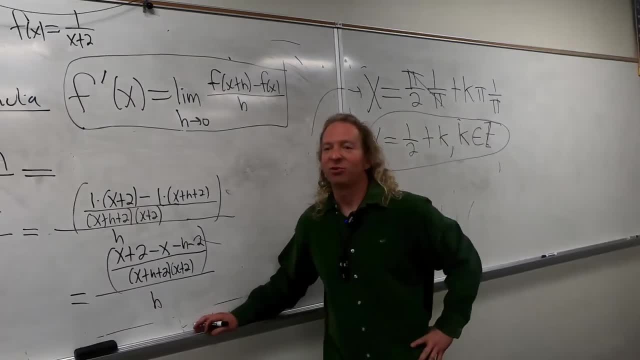 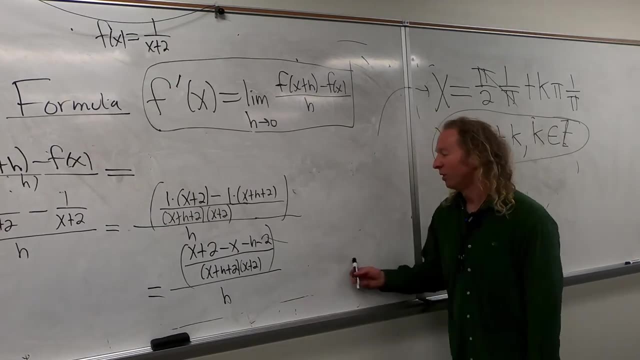 Like how to get the answers. It's really exciting, It's a really cool website, It's free. Oh, I've got to show you something else too. Okay, So stuff goes away. Boom, boom, boom boom. 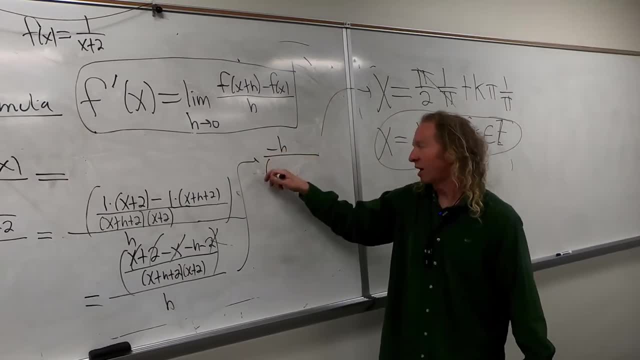 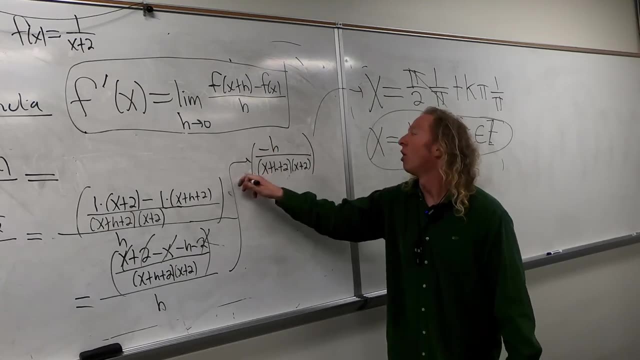 So we have negative h over x, plus h plus 2, x plus 2.. And it's still in parentheses: Choo choo, All over h, All over h. Take your time, It's a lot of writing. 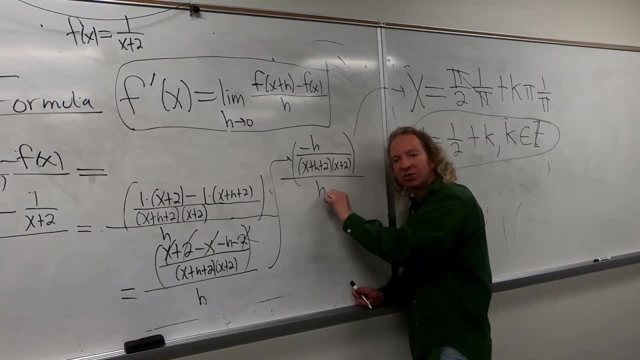 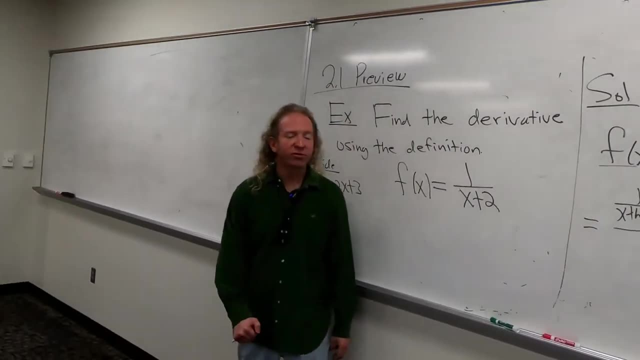 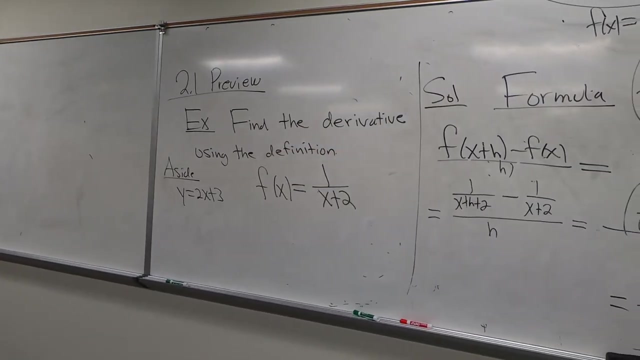 The parentheses are important because it's this entire thing divided by h. Right, This entire thing divided by h. When you divide by h, what do you really multiply by The reciprocal? Very good, Which is 1 over h. So this is equal to: 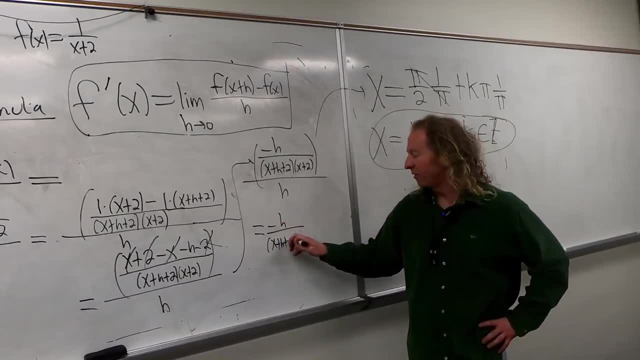 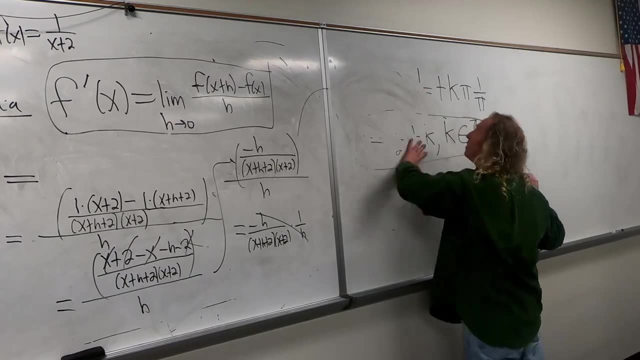 This is why I assigned that annoying delta x problem. I figured most people would get stuck on it, But it's good, because eventually you'll get it. and then when we do it on Monday, which is when we're doing this, We're not really doing it today. 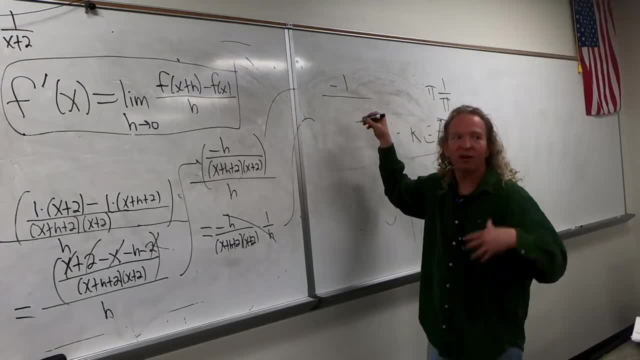 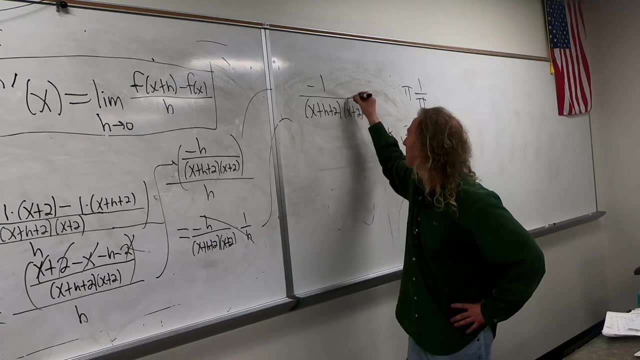 This is not really happening. It'll be like: oh yeah, okay, I've seen it before. So then this is x plus h plus 2, x plus 2.. So in college algebra this would be like a hard college algebra problem. 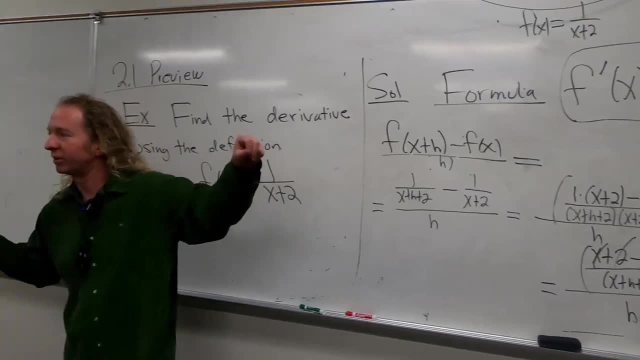 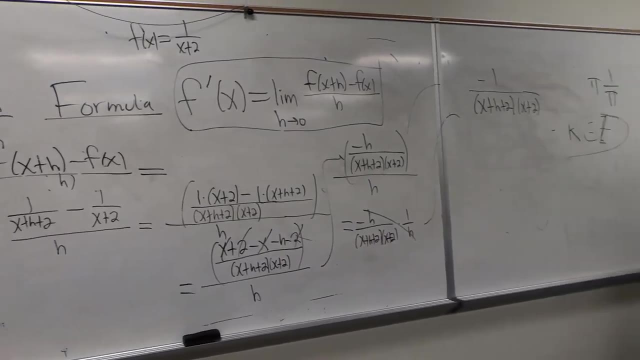 You would stop here, right, And you would call that the difference quotient. Okay, We're almost done. We're almost done. The next step is just a formality, And it's very easy. It's very simple. I'm just going to wait. 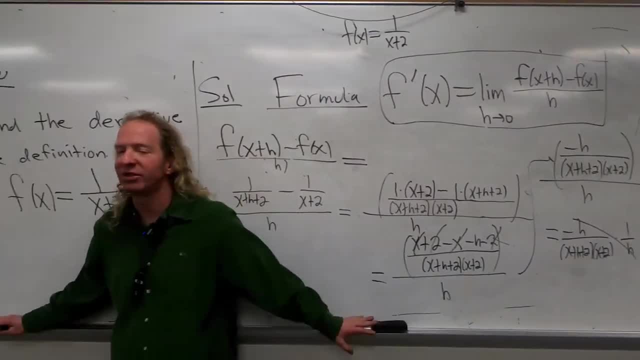 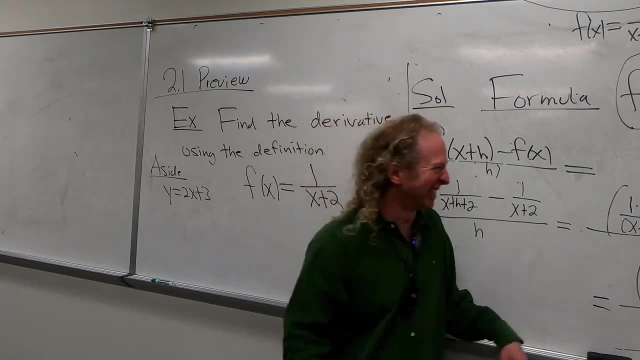 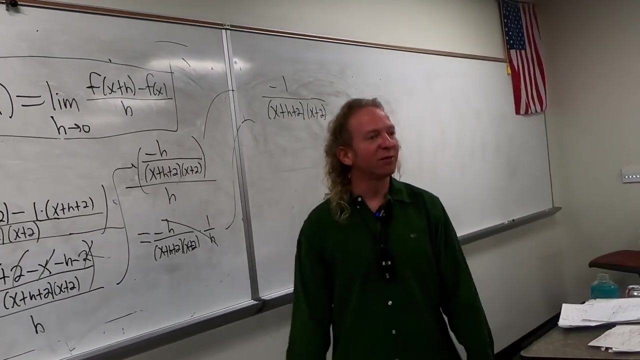 I need any questions. People are writing still, So I'll wait. I forgot that thing was there. I just I was like what Forget? like yeah, okay, No questions, No questions, All right. So we worked out this piece, right. 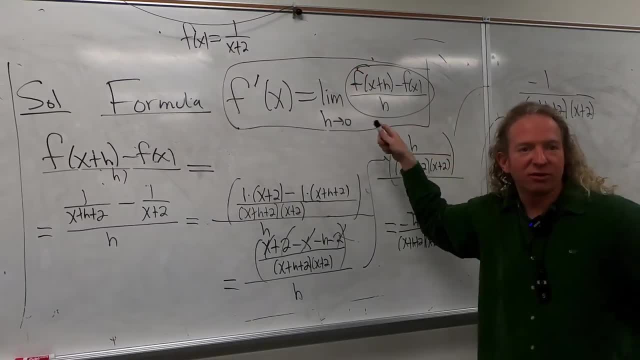 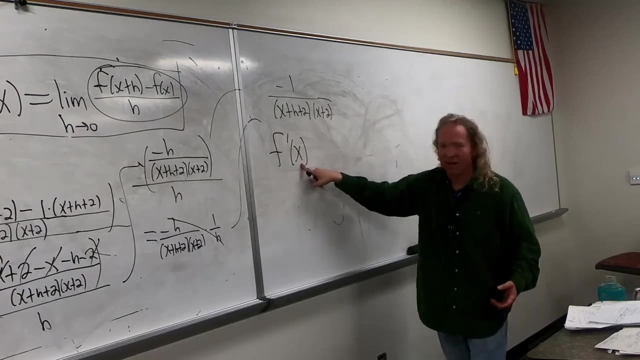 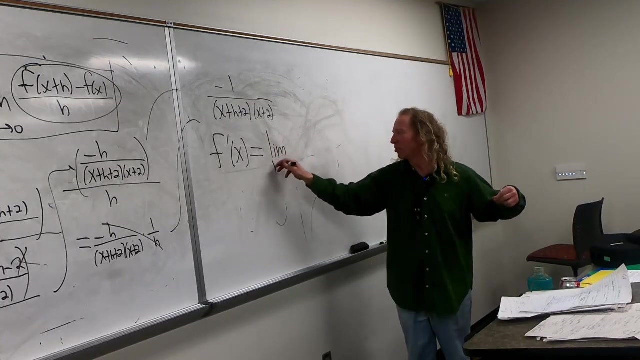 So now we just got to take the limit. So it's a formula. So to finish, f prime of x. right, that's what we have to find. the derivative of f at x- this is the slope of the function at x- is equal to the limit as h approaches 0. of this, 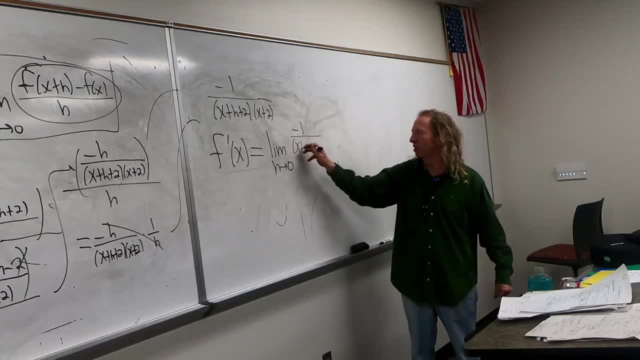 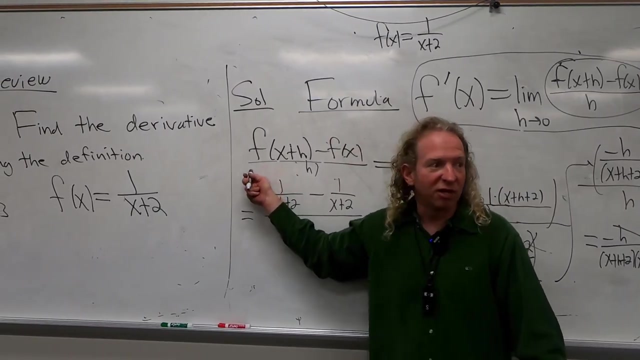 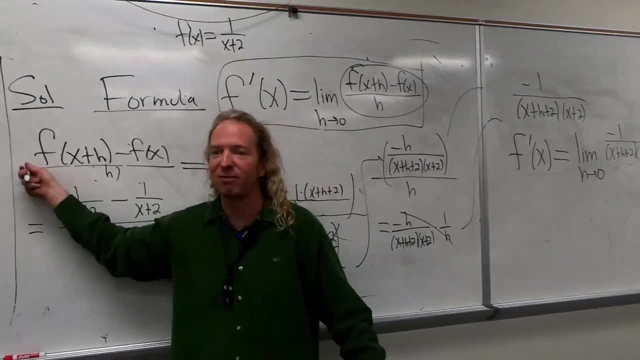 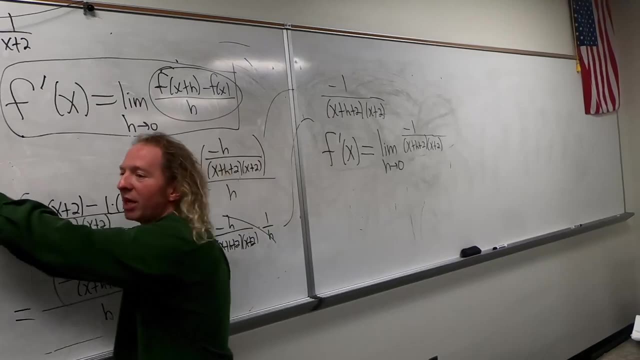 That's 1,, 2,, 3,, 4,, 5,, 6,, 7 times. So it's 7 times more work. I have to write it 7 times, so I wanted to avoid that. So it's better to not write it and wait to the very end, okay, and then write it. 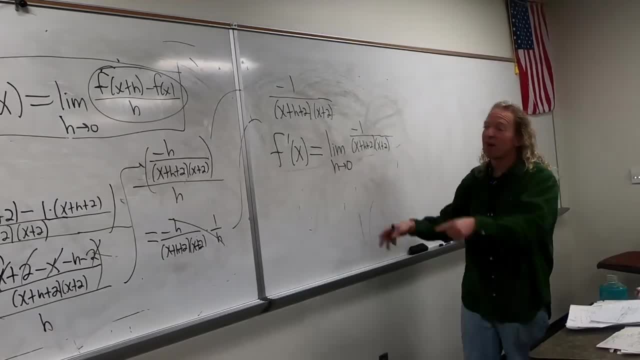 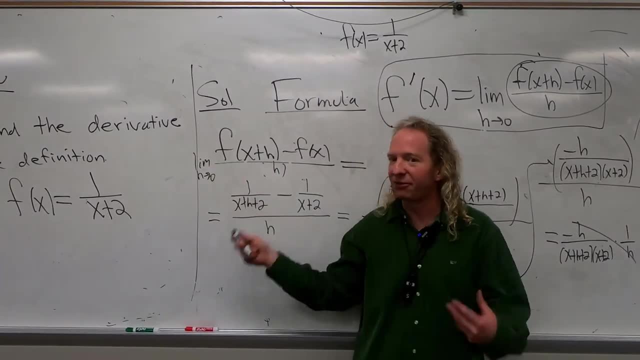 And that way you can't get it wrong, because I can't take points off because it's correct. But if you write it once, like if you write it here, like if you do this and then you don't write it here, I have to take points off because it's wrong. 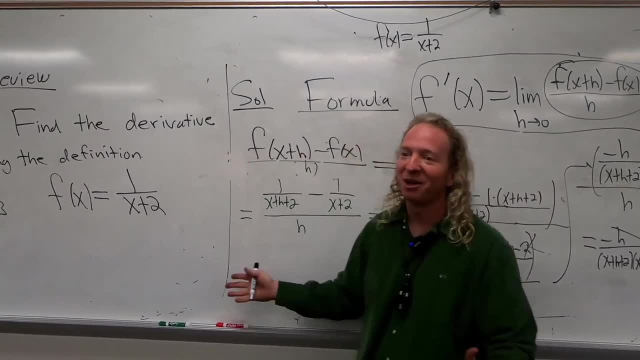 Like I can't. it's like, oh, it's whatever. no, it's wrong. it's a math class like: right, it's got to be right to mark it right, Even if I want to mark it right and I can't unless it's right. 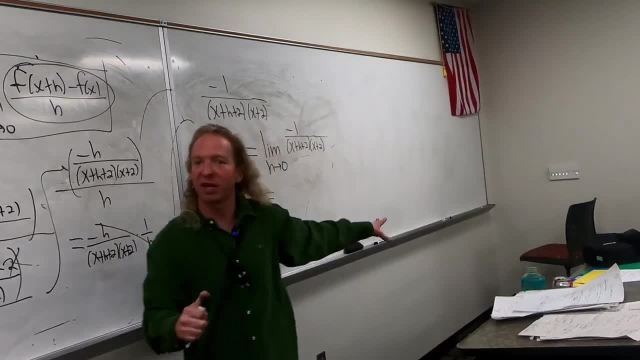 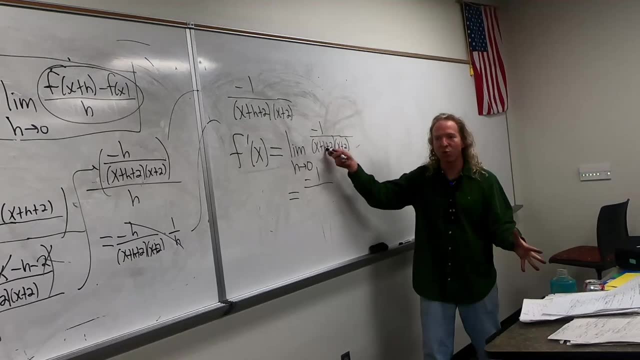 So now we're going to take the limit, so we're going to plug in the 0.. Do we write the limit again now? No, we drop it right. good, good, So this is going to be negative 1 over. so this is 0, right. 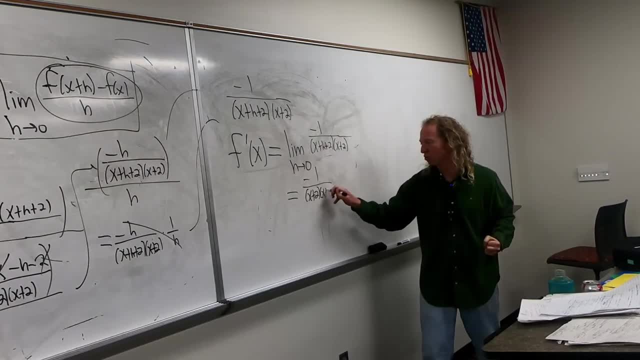 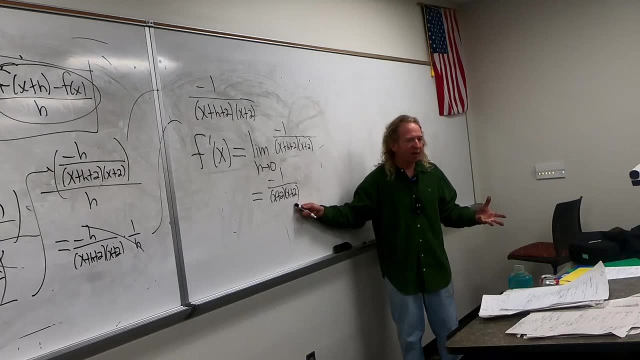 So it'll be x plus 2, x plus 2.. So it'll be x plus 2 times x plus 2 is x plus 2 squared. Yeah, and just leave it like that. A lot of times when people first see calculus they're like: oh, should I multiply it out? 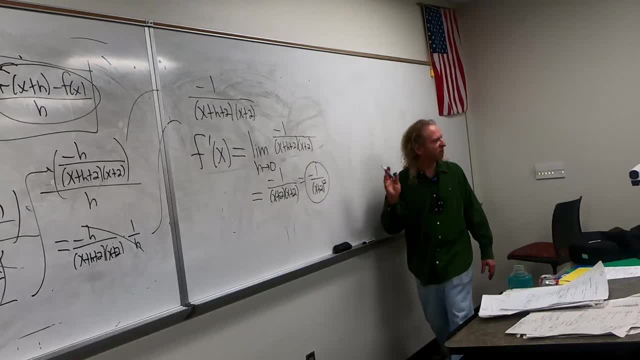 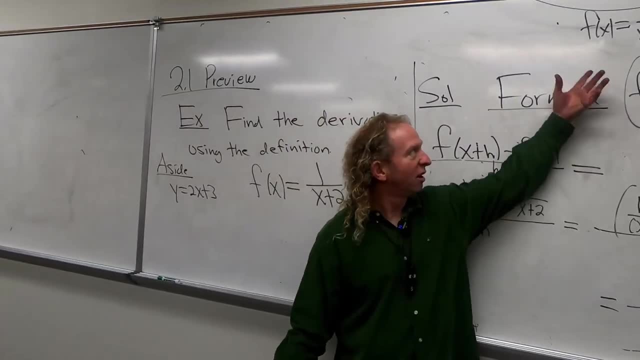 No, no, just leave it. that's beautiful. That's better that way. Just leave it. That's it. That's it. That's called the derivative of the function. On the second test, you'll be able to do this if you're really ready for this in your head. 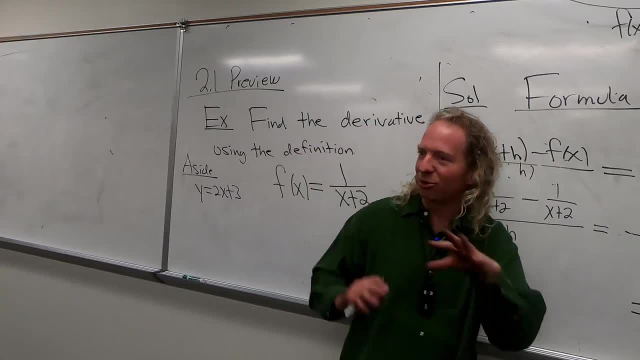 Like using some formulas and stuff, Like oh yeah, yeah, like you'll be able to do some math, Like I can do it in my head, Not this, there's another, there's shortcuts. Yeah, you get really good at it. 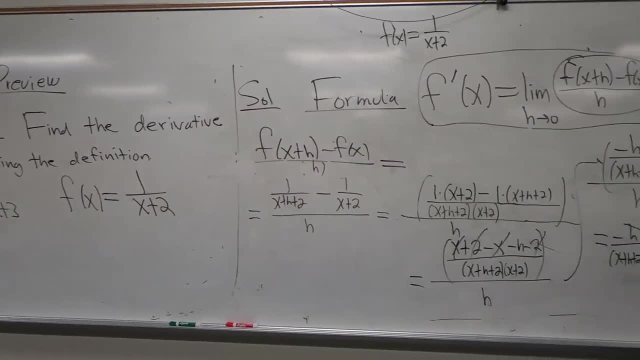 Yeah, you get really good at it, And if you take Calc 2, you become even better. If you take all of them, you're like, yeah, it's really good. Any questions on this one? So this is pretty much, yeah, yeah, Jordan. 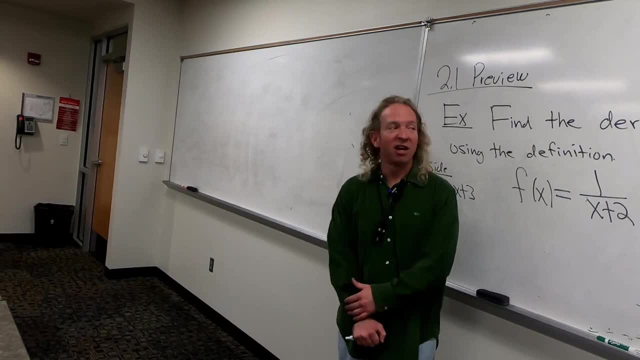 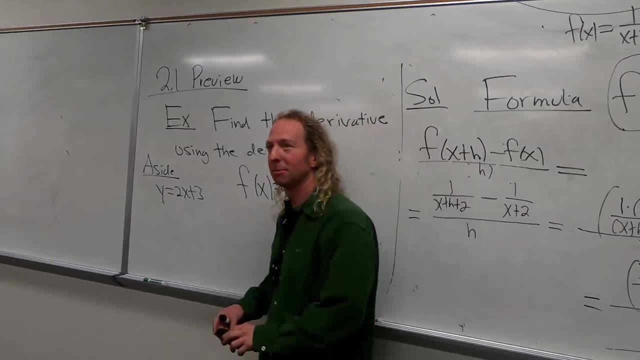 I was going to ask, like, where do we get this from? Like why is this true? What is this? Why is it true? Why is this true? Yeah, like how do we? How did we get that? How does it work out if we were to have a 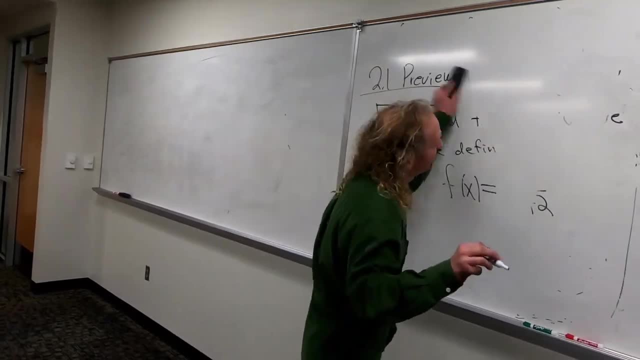 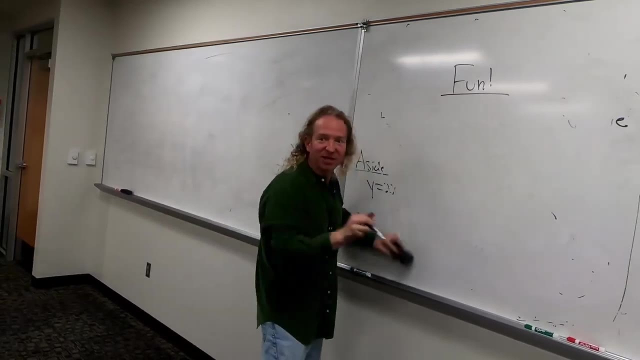 I'm going to show you really quick, I'm going to do it really fast, Okay, Just like five minutes, Okay. So I'll do it again next time. Five minutes, So, no three minutes, Okay. so you have a graph like this: 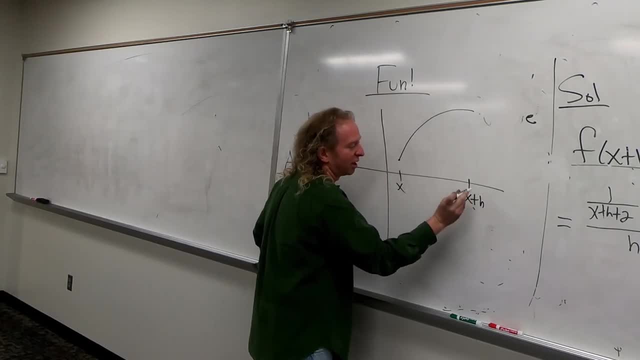 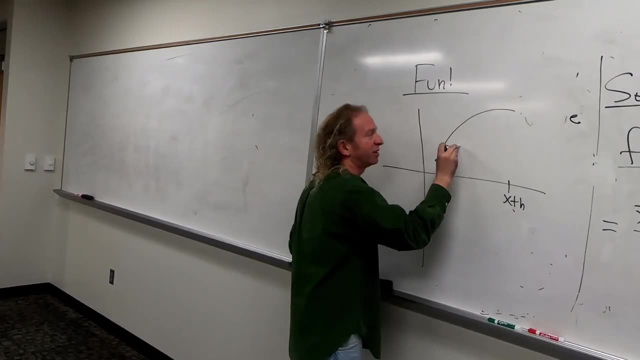 I'm going to call this x. I want to call this x plus h. And the goal here? the goal is to find the slope at x. Okay, So what you do is you connect, You connect these dots and you draw a triangle. 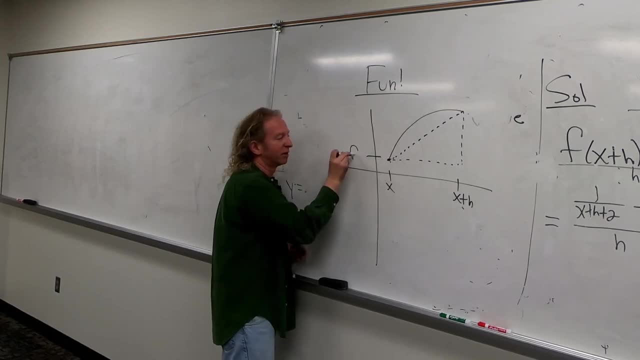 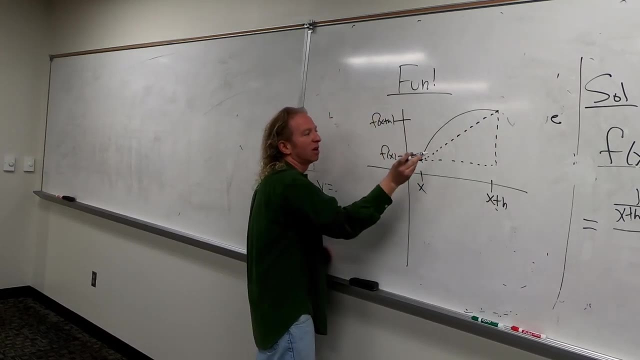 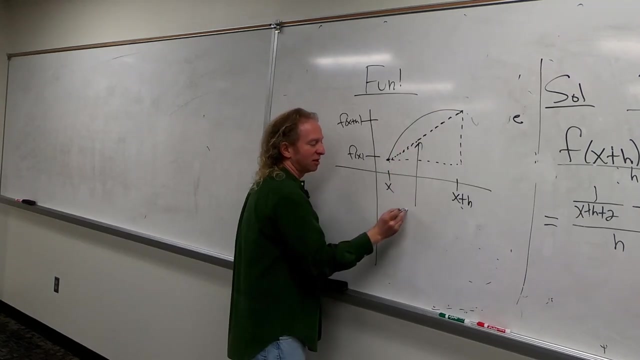 So the y value at x is f of x. The y value at x plus h is f of x plus h. Now the run, the slope of this line. this line has a name. This line is called the secant line. 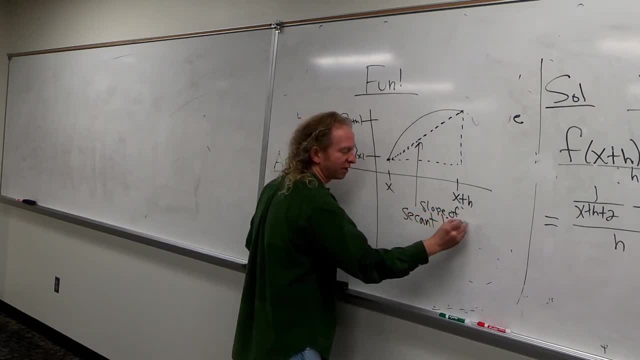 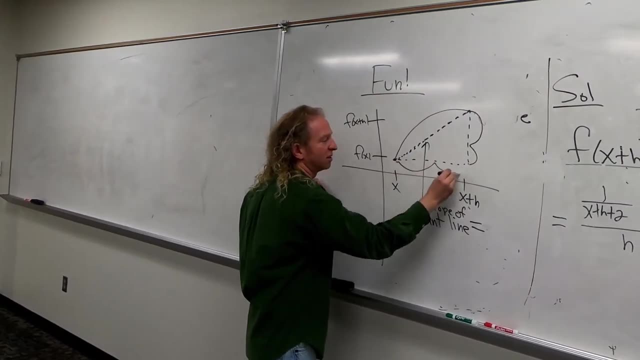 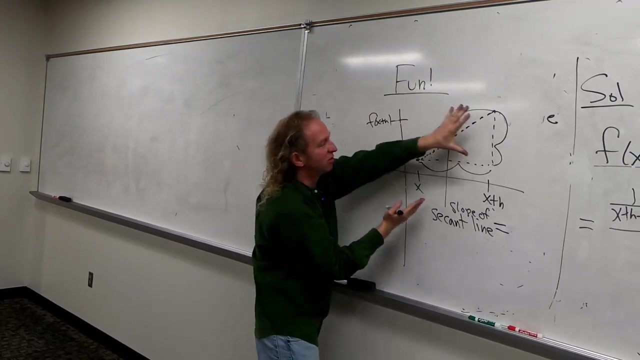 And the slope of the secant line. it's rise over run. So the rise is this, The run is this. The rise is this minus this, This minus. this gives you this, This minus this gives you this. So the rise is f of x plus h minus f of x. 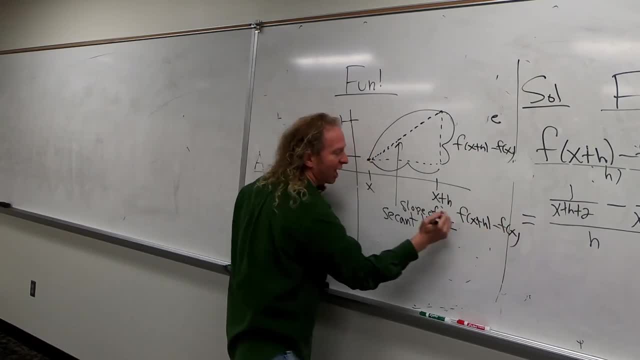 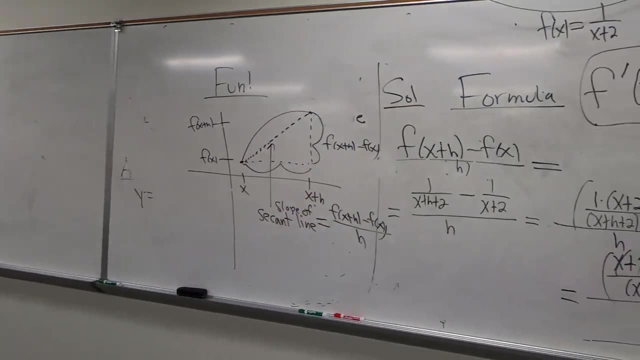 So it's f of x plus h minus f of x, And the run is this minus this or just this distance, which is h. So this monster is the slope of the secant line. What's the secant line? You can do anything like this. 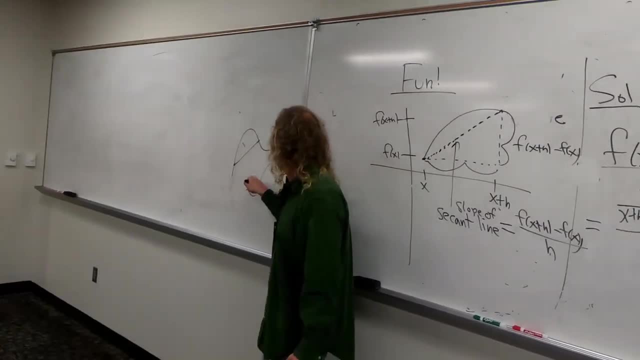 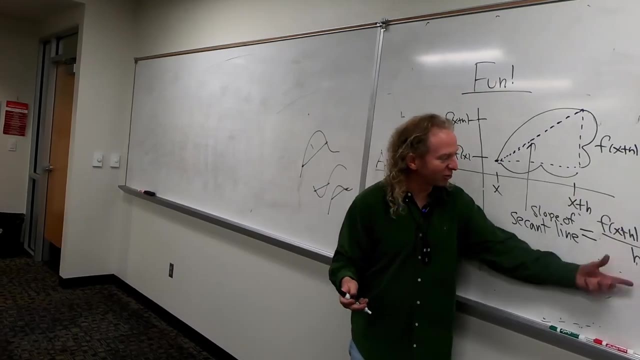 Take any two dots and connect them. It's a secant line, Secant line. Secant line, Secant means it cuts in Latin, according to this guy I met once. So the slope, yeah, yeah, No, yeah. 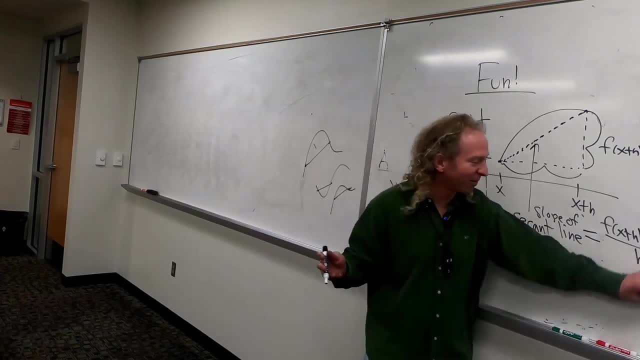 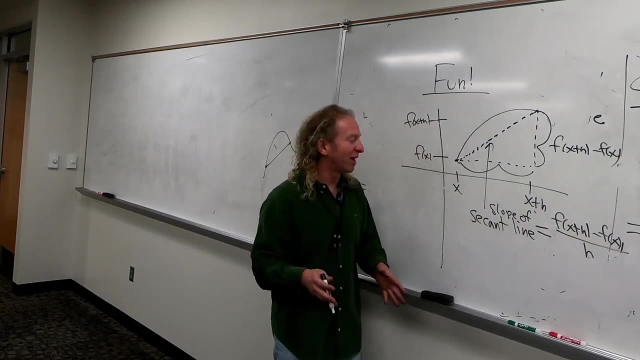 I met him at, like this high school competition in Oviedo or something. He's like: yeah, he was really cool. He used to be a math major, but he couldn't. that doesn't matter. Yeah, He couldn't get through advanced calculus, so he decided to teach Latin. 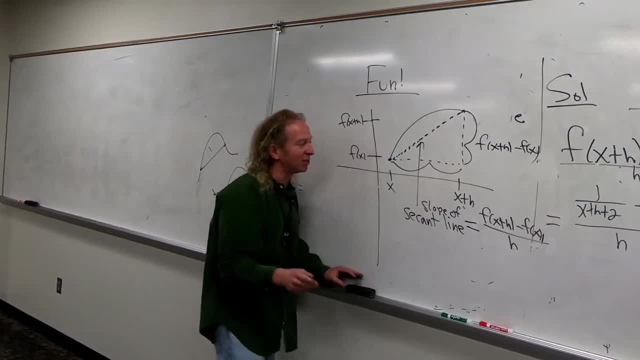 Anyways, secant means it cuts, So that's the slope of the secant line. So here's where you have to use your imagination. If you let h go to zero, what happens? So h is getting small, so it's going this way, right? 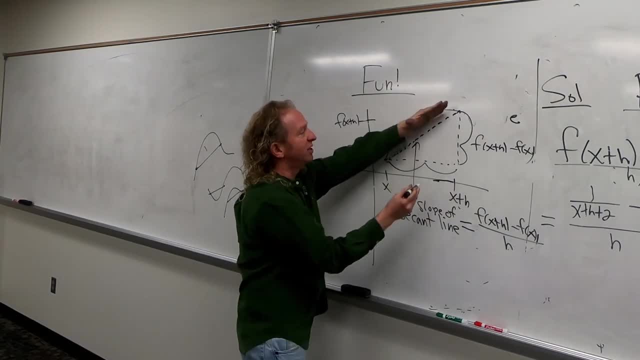 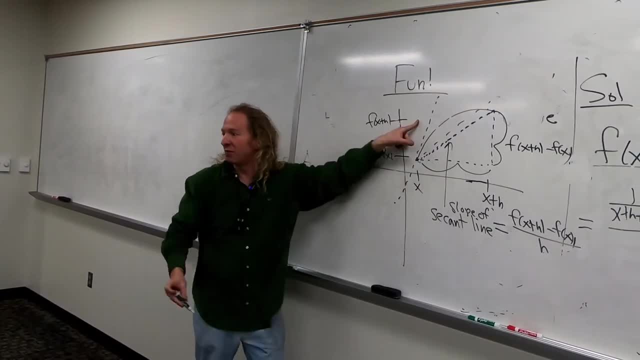 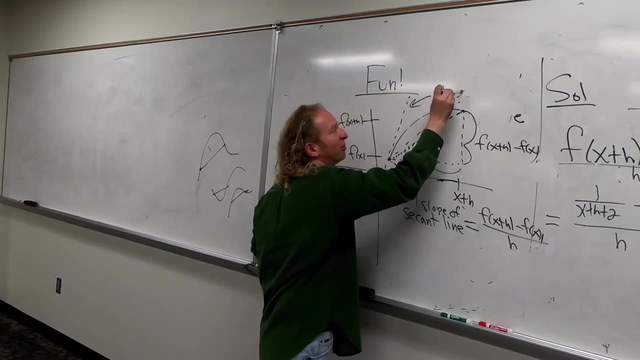 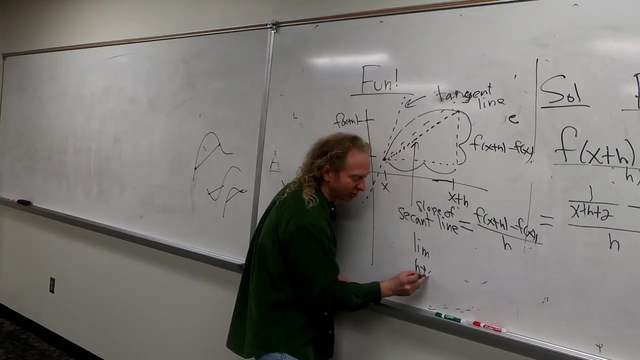 The secant lines approach a line that just touches at this point. That line is called the tangent line. okay, So when you take the limit- ah, I can't spell- When you take the limit, When you let h approach zero. so if you take the limit as h approaches zero of the slope of the secant line, 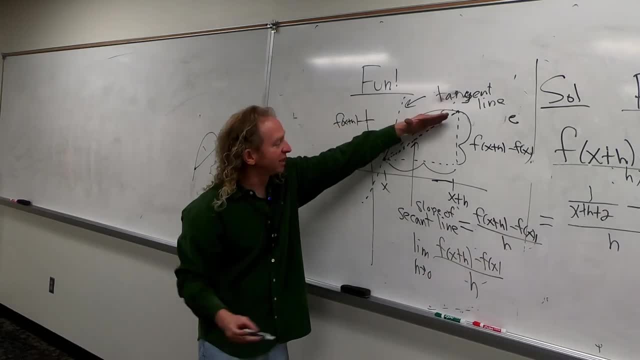 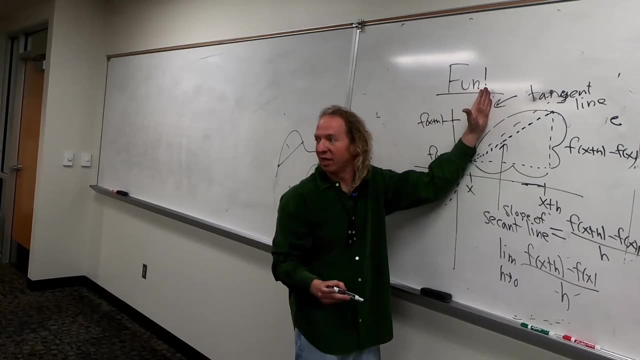 what happens is you have infinitely many secant lines because h is going this way, h is getting small, so this point is going this way, So you have secant line secant, So the secant lines approach the tangent line, So the slopes of the secant lines approach the slope of the tangent line. 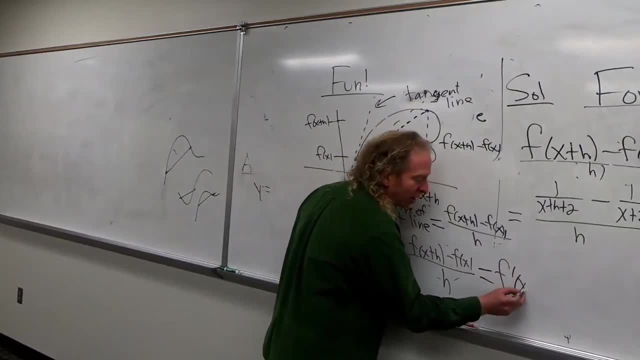 Now we say that this is the slope of the tangent line. So, loosely speaking, it's the slope of the function. We call it the derivative. So that's the derivation It's really. It took three minutes. Does that make sense at all? 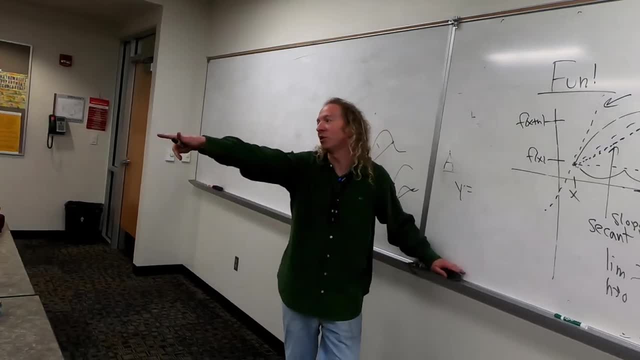 It did, Even just a little bit. Did it make any sense? A little bit, Okay, We'll do it next time, but it'll take us 20 minutes, Yeah, 15.. So what you're saying is: the derivative is the tangent line of the function. 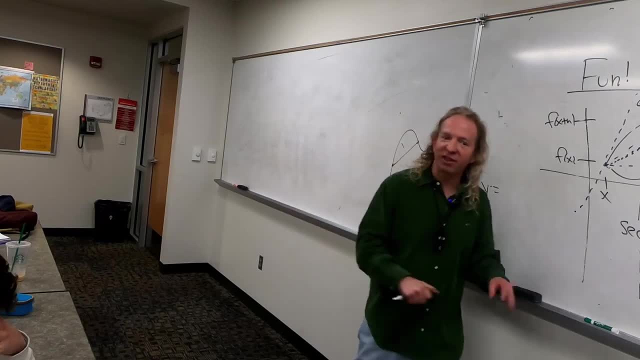 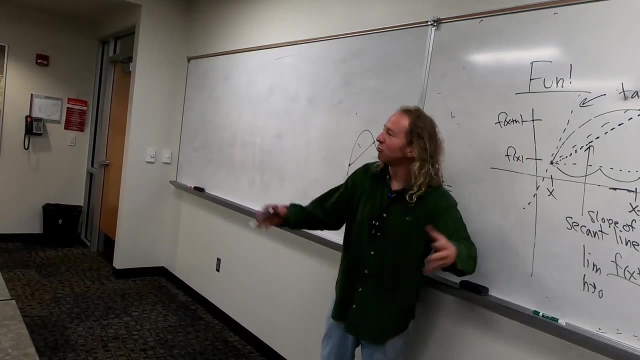 It's the slope of the tangent line. Okay, slope of the function. Yep, That's the most important thing. That's calc one. If you can go home and explain this to like your friends correctly, like: do you know calculus? 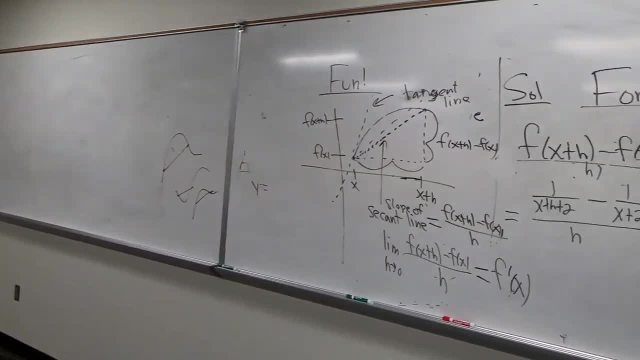 Like shkene right, Like most people can't right. I mean because? why? Because I mean you have to homework and stuff to do right, And like you have to focus on that Because that's your grade. 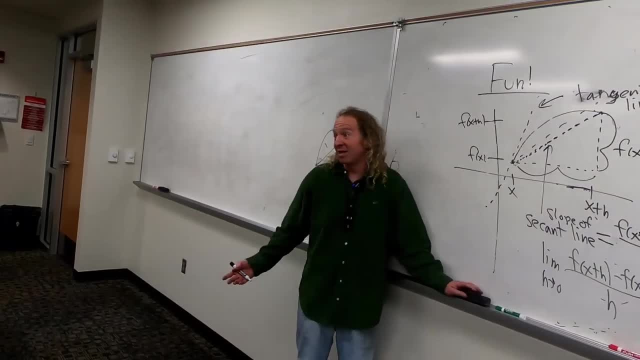 This is not your grade, right? It's just you know. But yeah, Yeah, it's fun, But it's interesting. This is really calculus. So this is called differential calculus. So calculus back in the day used to be two parts. 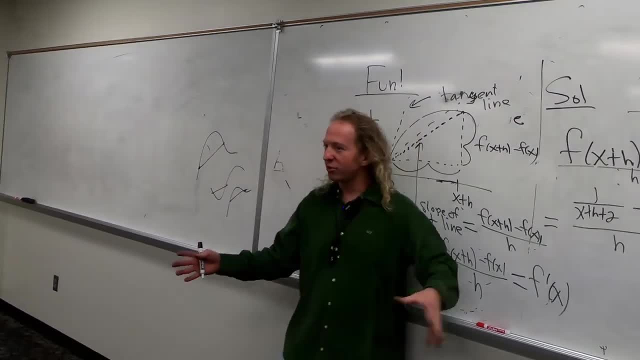 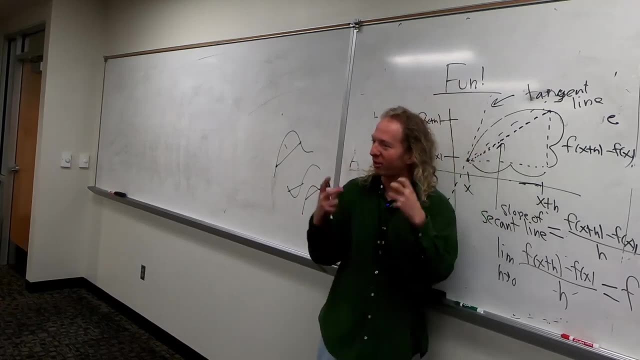 It used to be differential calculus and integral calculus. So this is the beginning of what's called differential calculus, Like the old school books, like differential calculus volume one, Like these really old school books that are like really hard to read and they smell good.